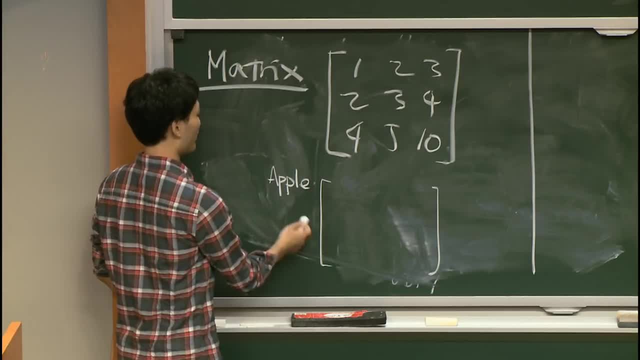 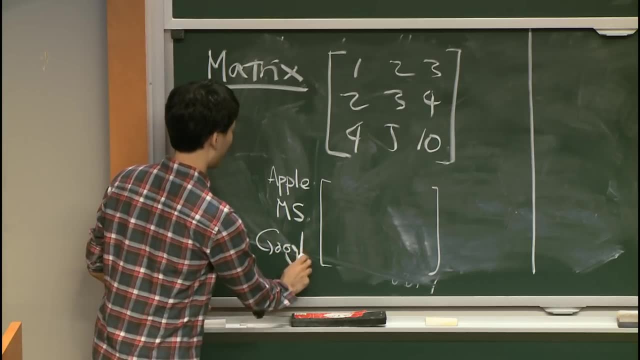 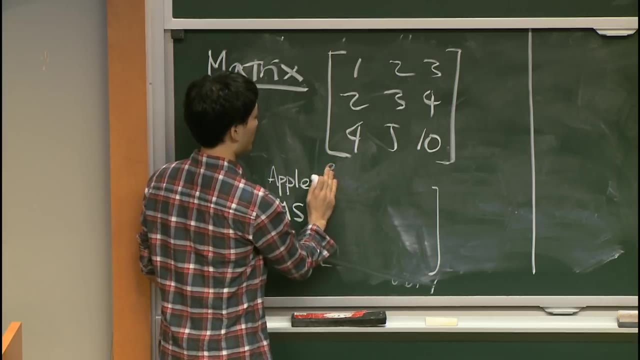 like Apple, I don't know Morgan Stanley should be there, What else? Google, And then maybe we can index a column by dates. So R, yeah, I'll say July 1st, October 1st, September 1st. 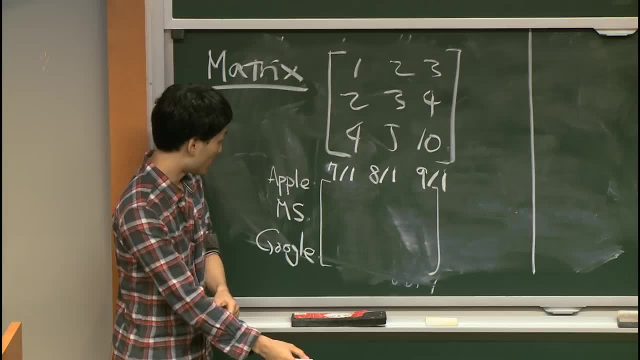 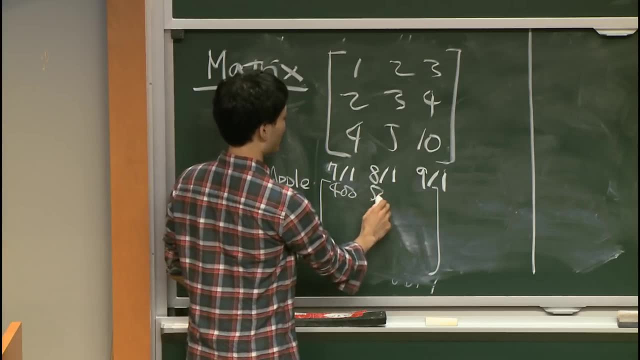 And the numbers. you can pick whatever data you want, but probably the sensible data will be the stock price on that day- I don't know- for example, $500, $500, and $5,000, that would be great. 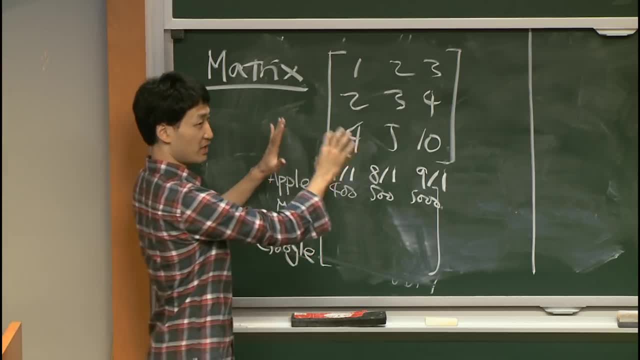 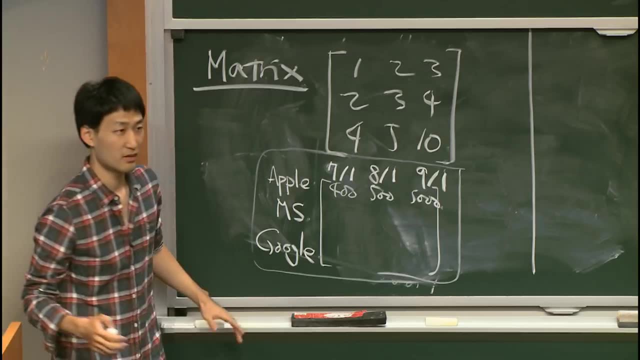 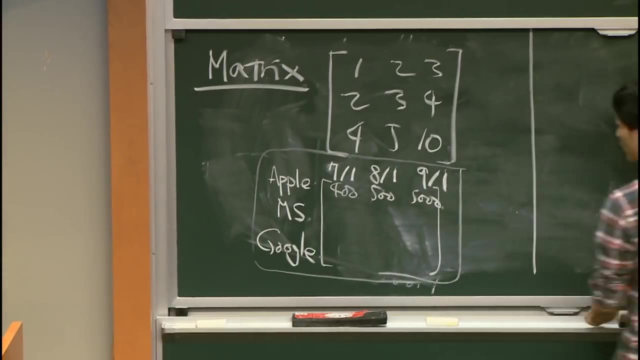 So these kind of data, that's just the matrix. Okay, so defining a matrix is really simple, but why is it so powerful? So that's an application point of view, just as a collection of data, but from a theoretical point of view. 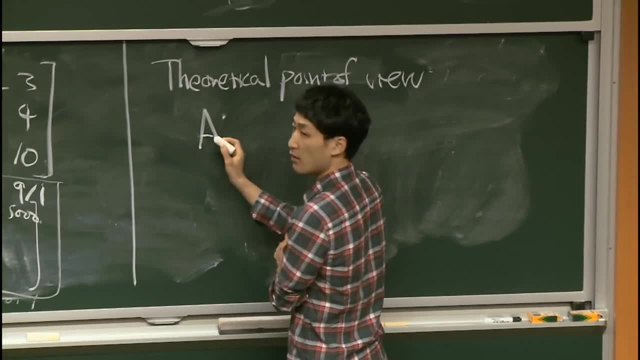 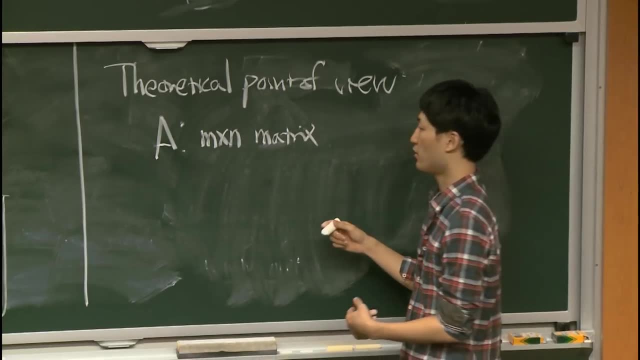 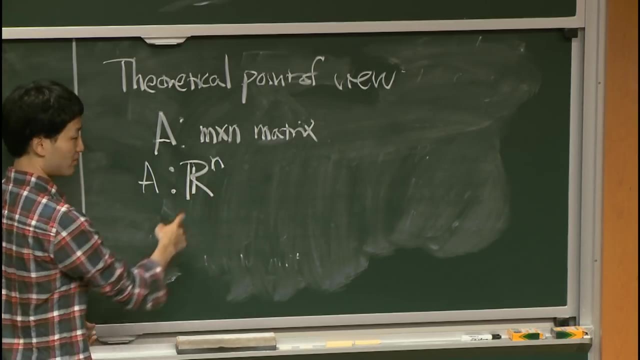 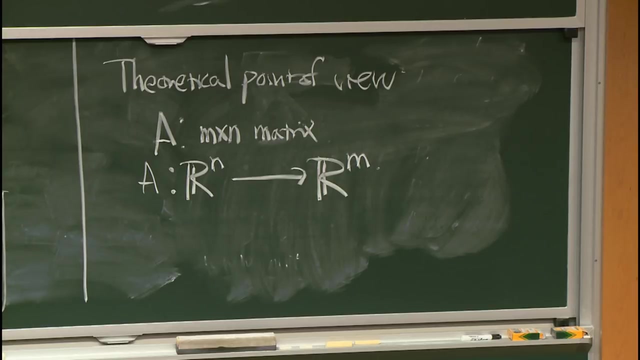 a matrix. an M by N matrix is an operator. It defines a linear transformation. A defines a linear transformation from the vector space- N dimensional vector space- to the M dimensional vector space. That sounds a lot more abstract than this right. Okay so, for example, let's just take a vector space and we'll get an M by N vector space, right? Okay so, for example, let's just take a vector space and we'll get an N dimensional vector space, right. 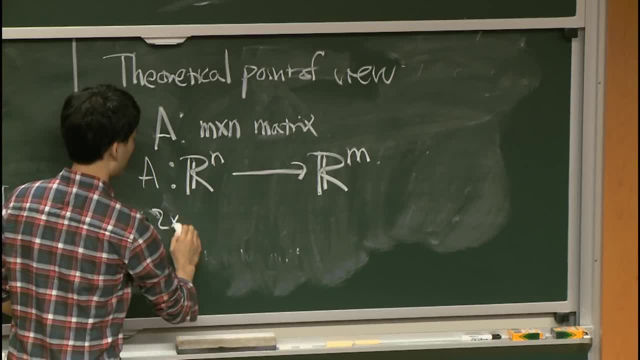 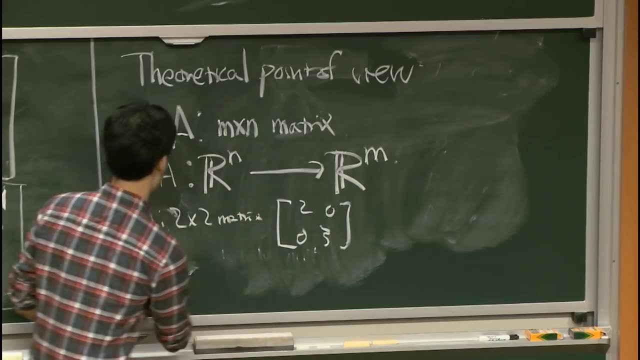 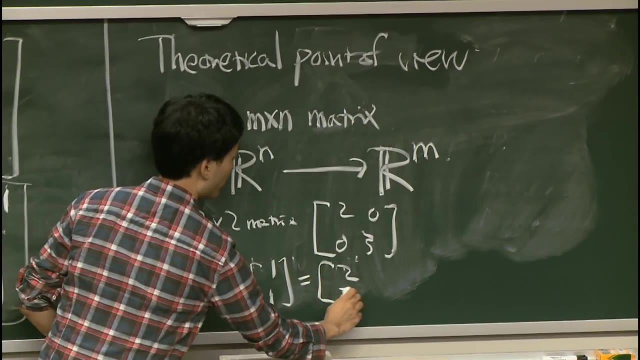 a very small example: if A is a 2 by 2 matrix 2, 0, 0, 3, then 2, 0, 0, 3 times, let's say 1, 1, is just 2, 0, 3.. 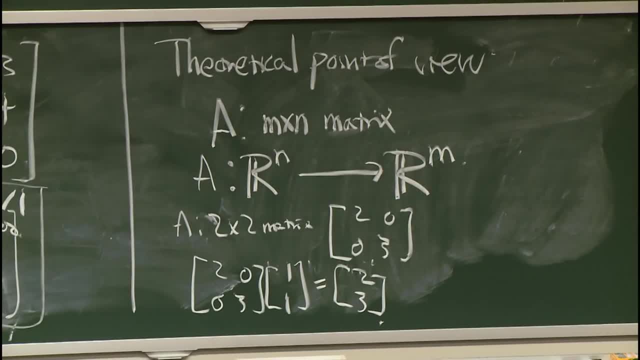 Right, OK, Does that make sense? It's just matrix multiplication, So now try to combine the point of view. What does it mean to have a linear transformation defined by a data set, And things start to get confusing. What is it? 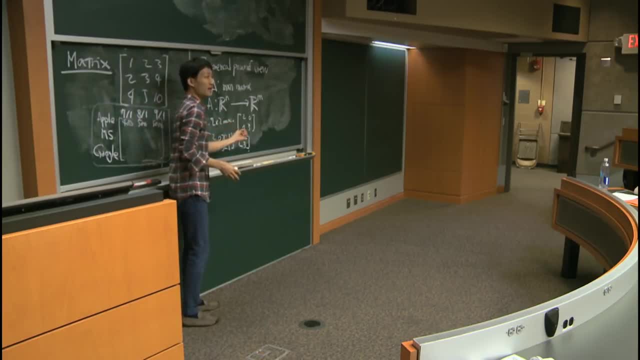 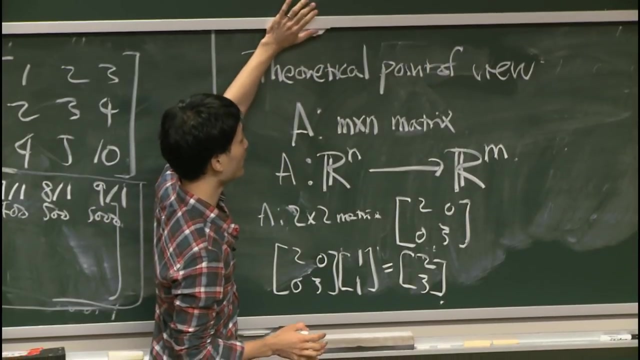 Why does a data set define a linear transformation And does it have any sensible meaning? So that's a good question to have in mind today And try to remember this question, because today I will try to really develop a theory of eigenvalues and eigenvectors. 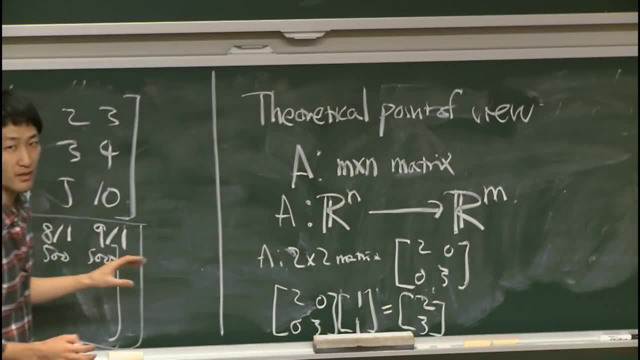 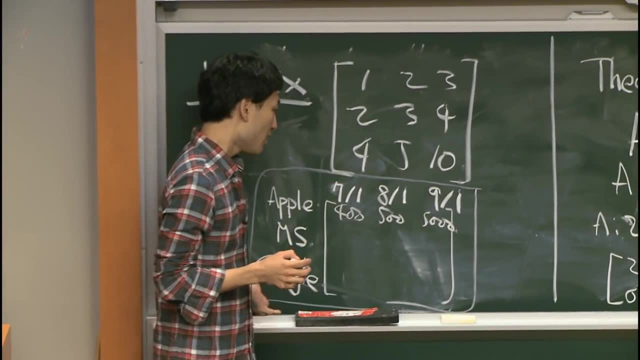 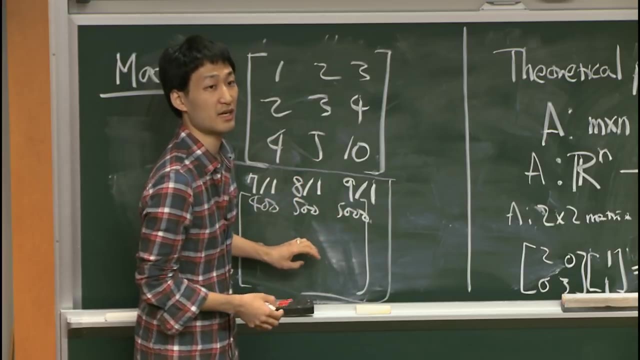 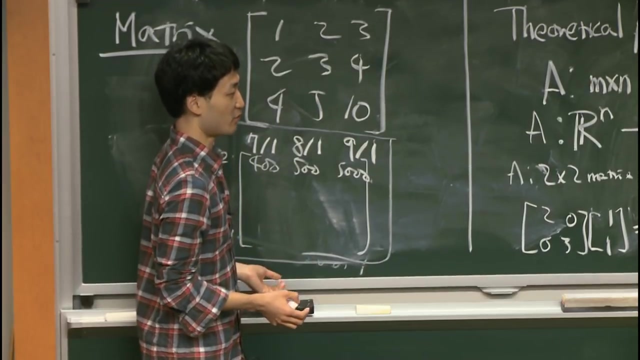 in a purely theoretical language, But it can still be applied to these data sets and give very important properties and very important quantities. You can get some useful information out of it. Try to make sense out of why it happens. So that will be the goal today. 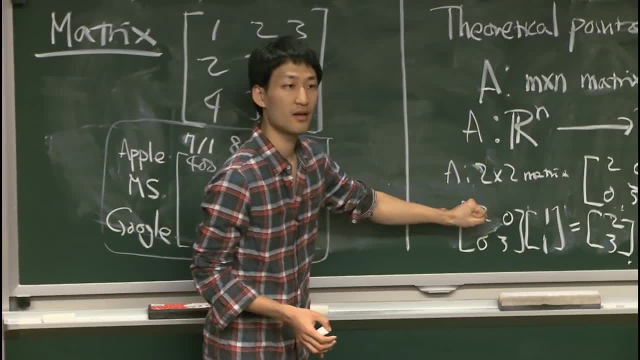 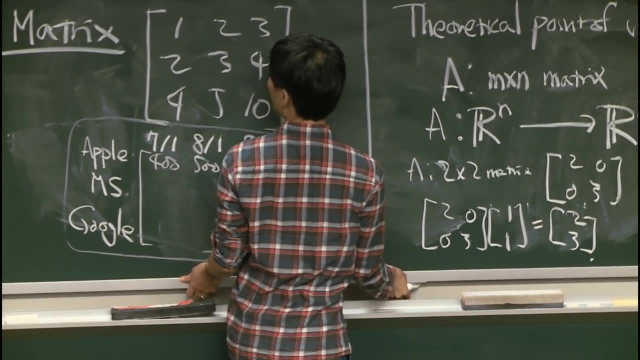 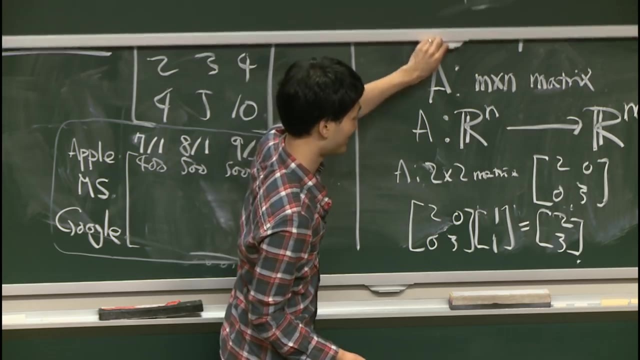 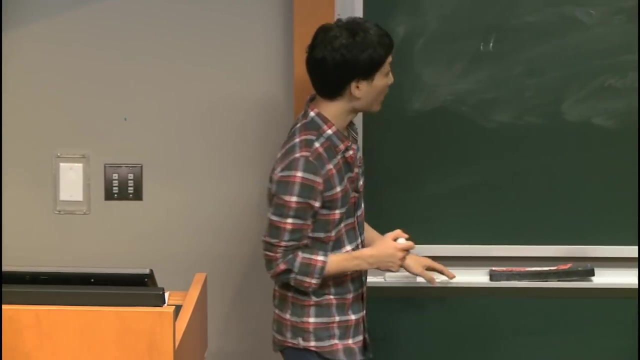 So really treat linear algebra as a theoretical thing, But remember that there's some data set like really data set underlying. OK, this doesn't go up. That was a bad choice for my first board. Oops, sorry, OK, So. 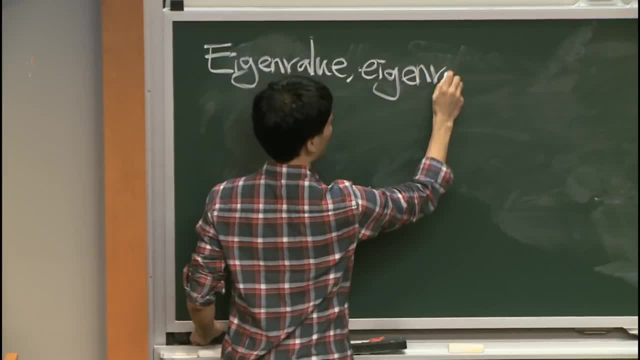 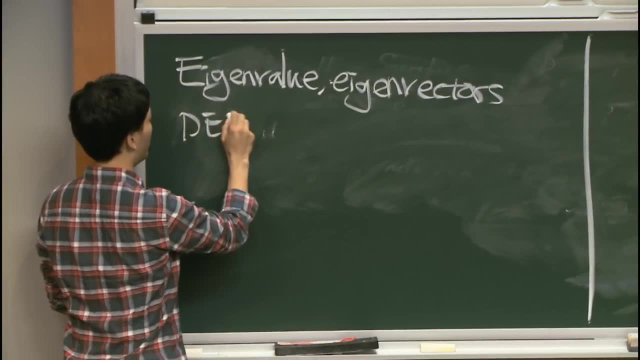 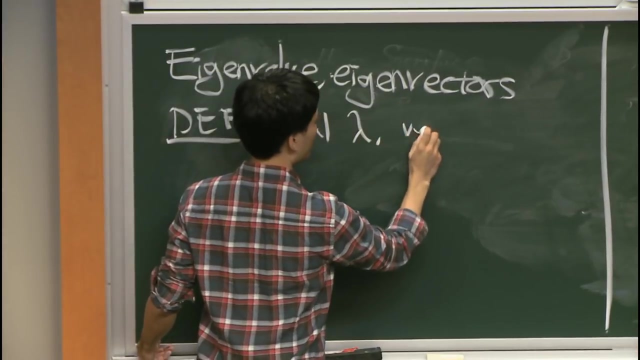 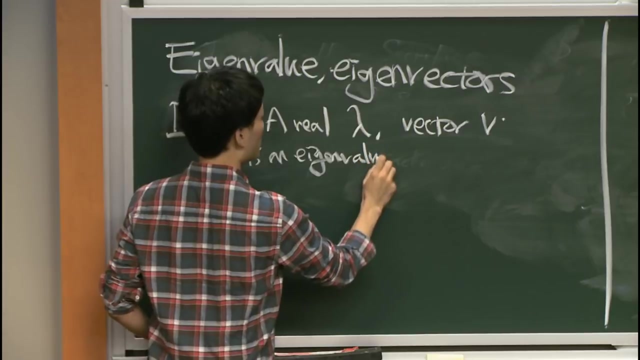 the most important concepts for us are the eigenvalues and eigenvectors of a matrix which is defined as a real number lambda and a vector. phi is an eigenvalue and eigenvector. OK, OK, OK, OK. 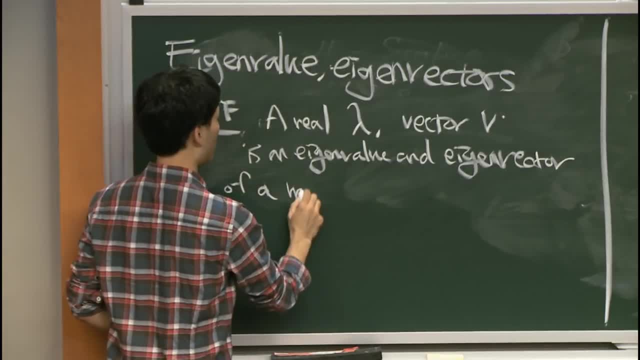 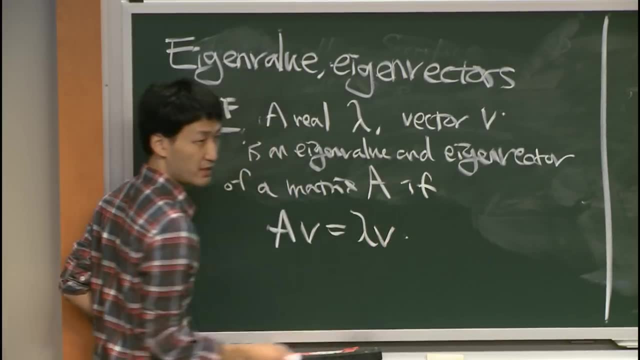 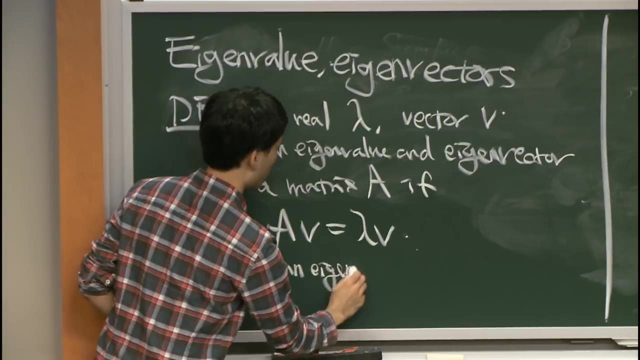 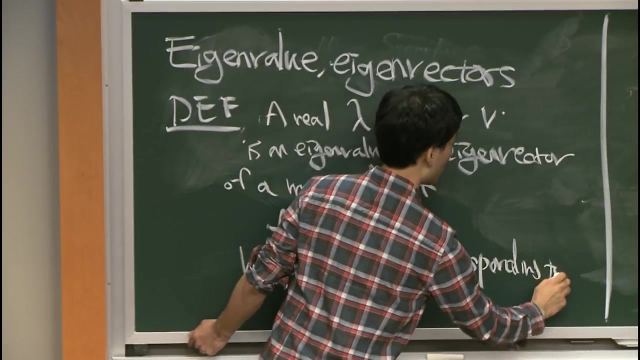 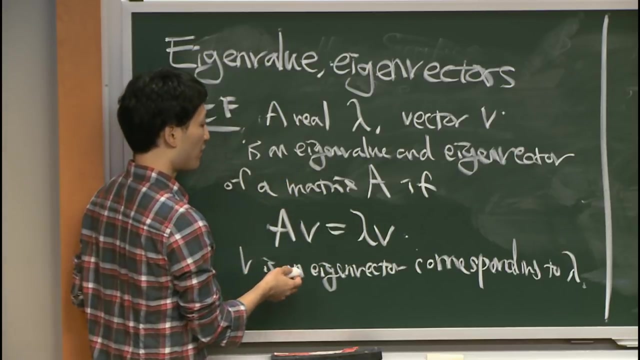 OK, OK, OK, So we have a matrix A. if A times V equals lambda times V, We also say that V is an eigenvector corresponding to lambda. So remember, eigenvalues and eigenvectors always come in pairs And they are defined by the property. 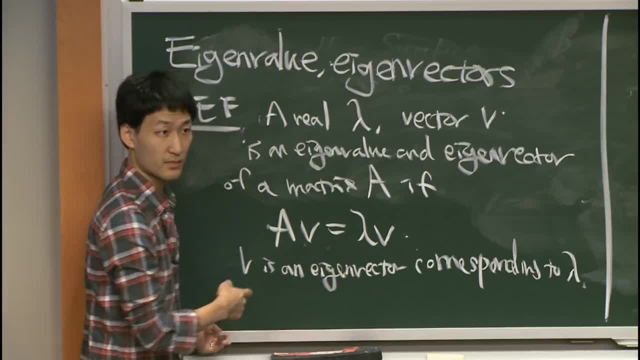 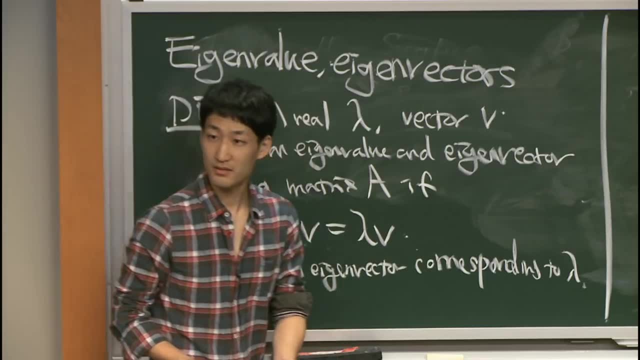 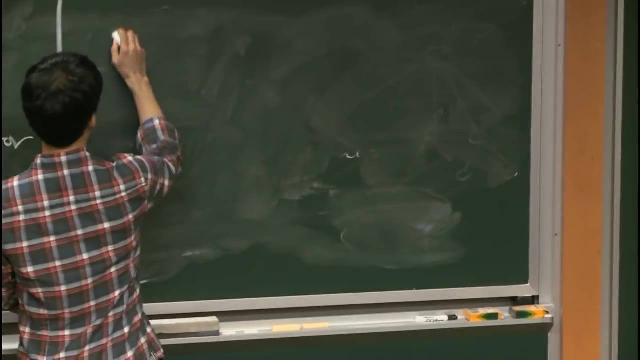 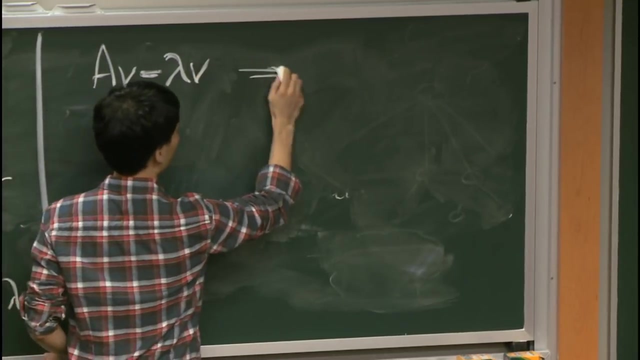 that A times V is equal to lambda times V. First question: Does all matrix have eigenvalues and eigenvectors? No, It looks like this is a very strange equation to satisfy, But if you change it in this form, A minus lambda I V equals 0,. 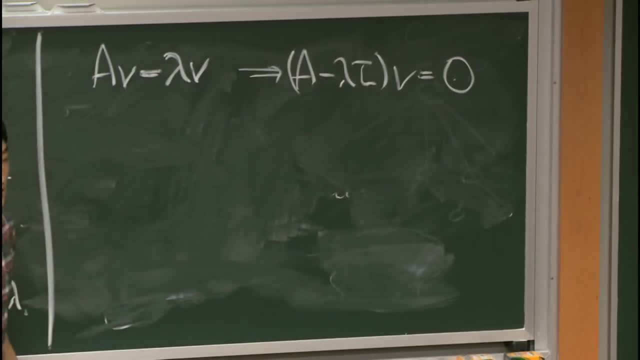 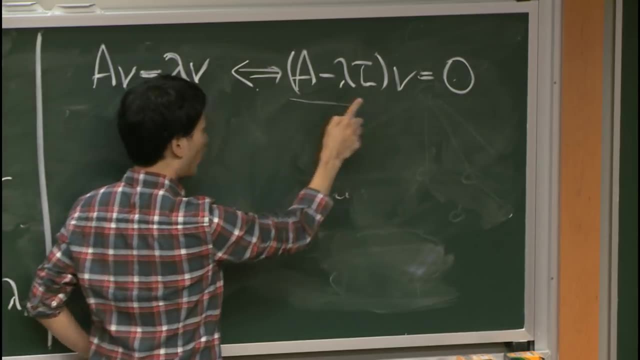 it's a very strange equation to satisfy, But if you change it in this form, A minus lambda I V equals 0, it still looks strange, But at least you understand that it's if, and only if. This can happen, only if. 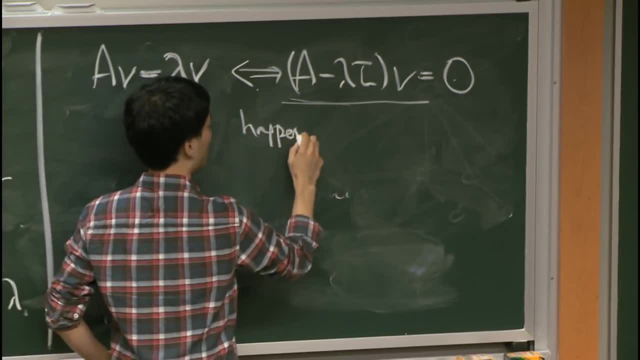 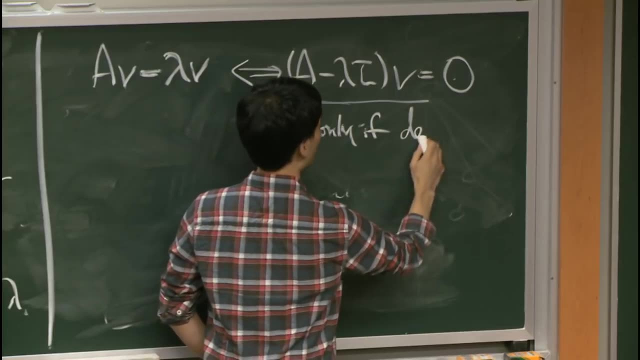 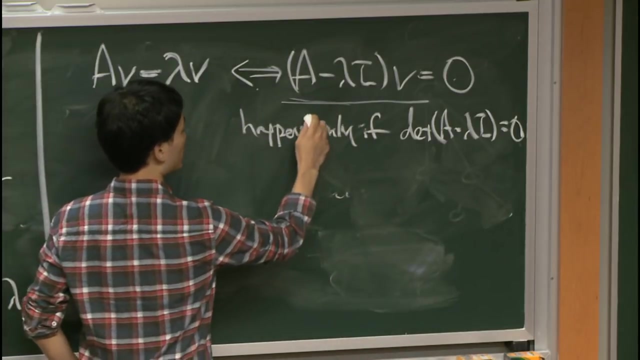 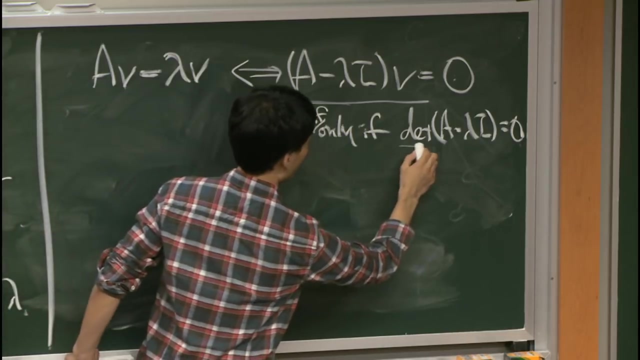 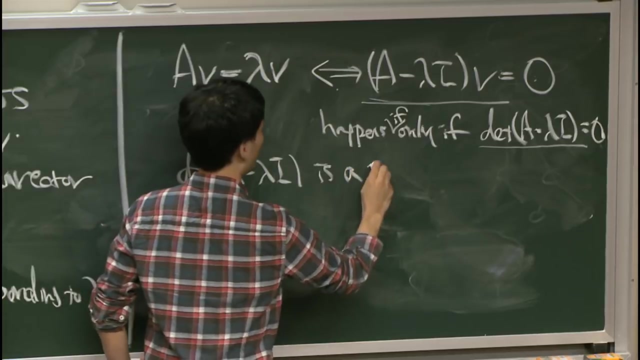 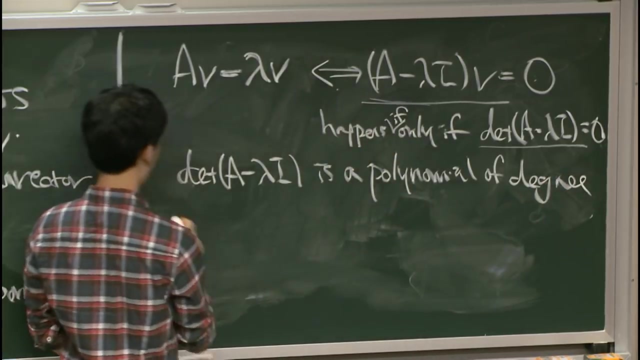 This can happen only if A minus lambda I does not have full rank. So determinant of A minus lambda I is equal to 0., If and only if, in fact. OK, So now comes a very interesting observation. Determinant of A minus lambda I is a polynomial of degree N. 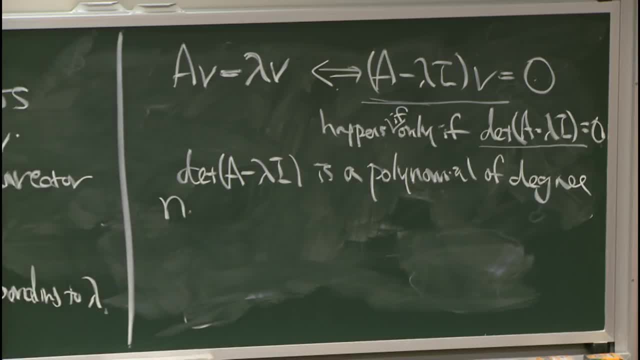 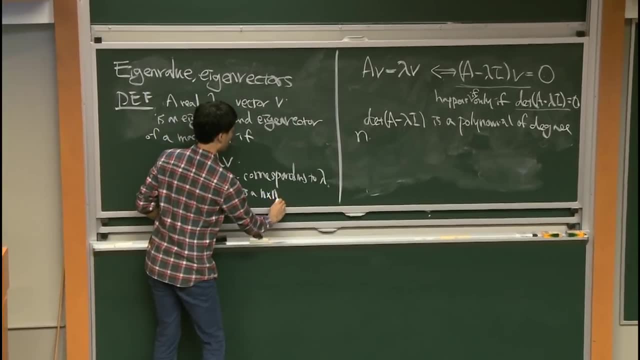 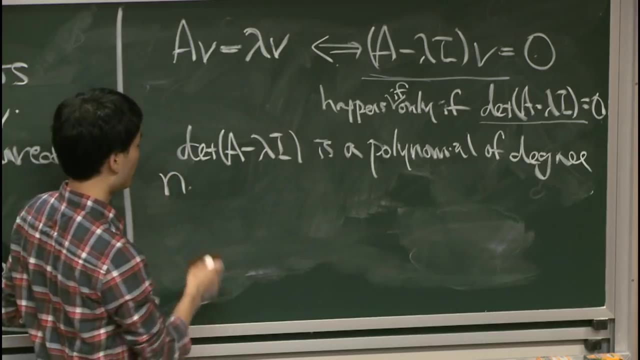 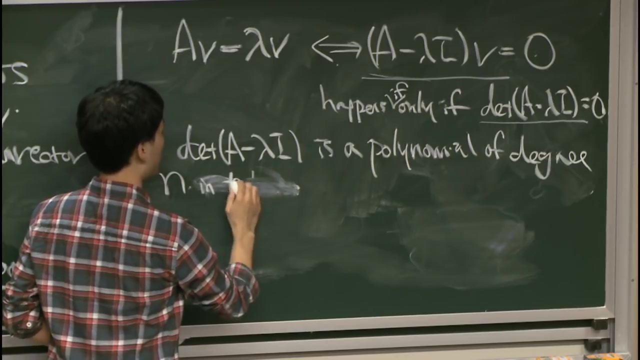 OK, I should have said this is only for N by N matrices. This is only for square matrices. sorry, It's a polynomial of degree N, That means it has a solution, Has to give N in terms of lambda, So it has a solution. 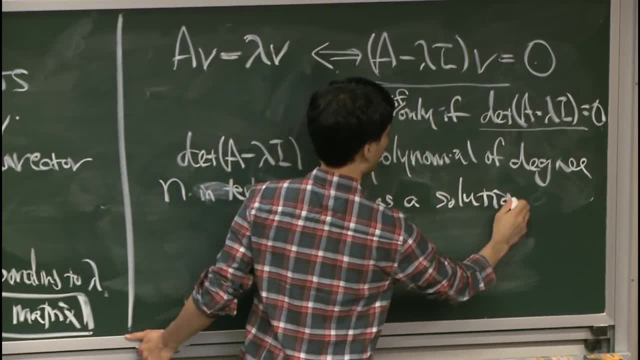 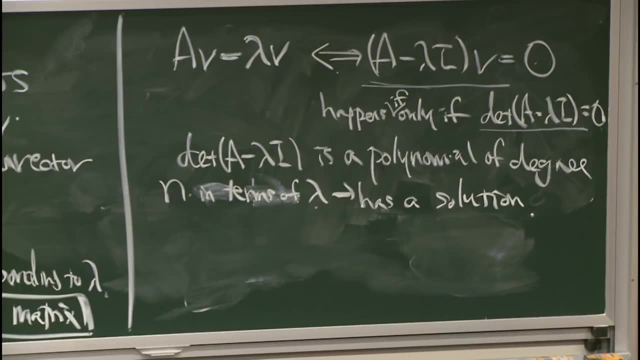 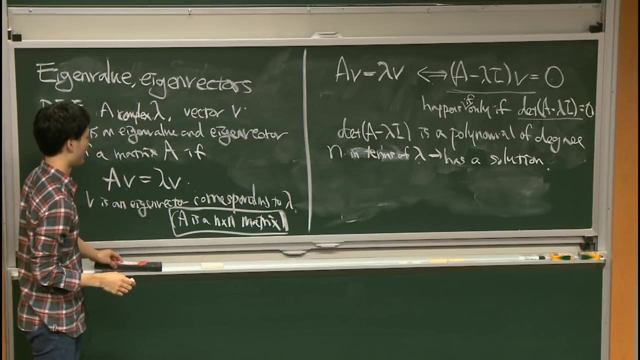 It might be a complex number. I'm really sorry. I'm nervous in front of the video. It's a complex. I understand why you were saying that it doesn't necessarily exist. Let me repeat. I made a few mistakes here, so let me repeat here. 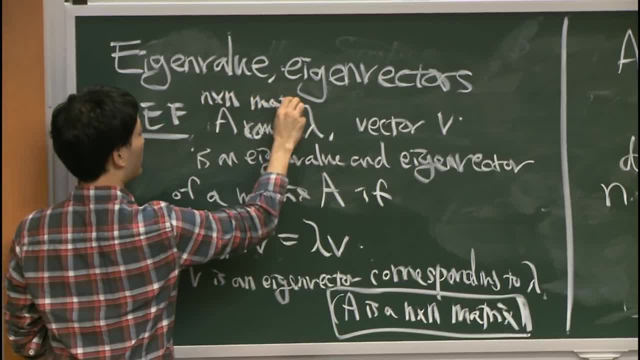 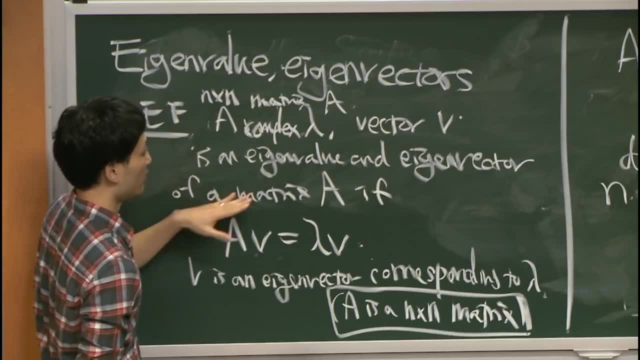 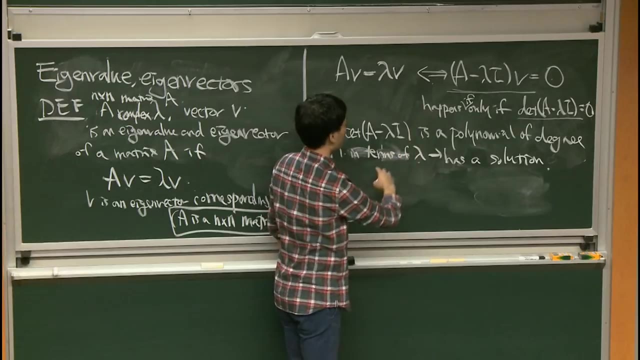 For a N by N, matrix A, a complex number, lambda, and the vector V is an eigenvalue and eigenvector. if it satisfies this condition, It doesn't have to be real. Sorry, Sorry about that. And now, if we rephrase it this way: 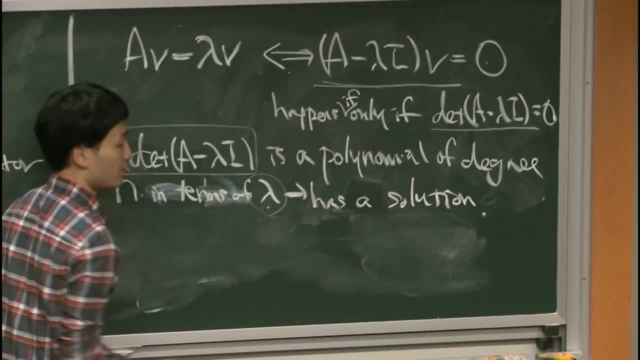 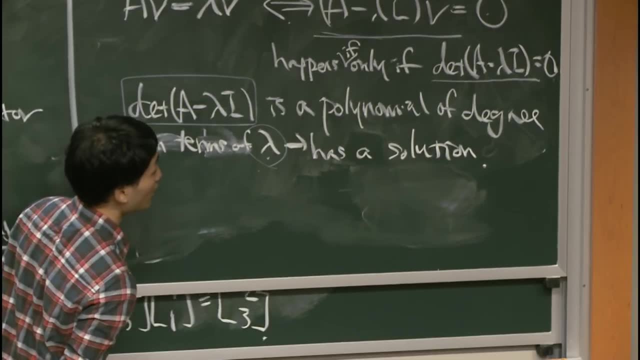 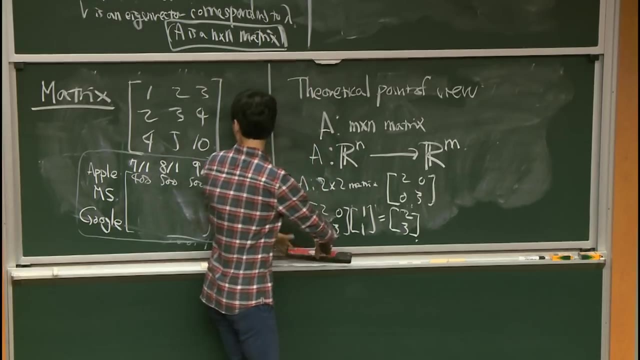 because this is a polynomial, it always has at least one solution. OK, That was just a side point, very theoretical. So we see that there always exists at least one eigenvalue and eigenvector. Now, we saw its existence. What is the geometrical meaning of it? 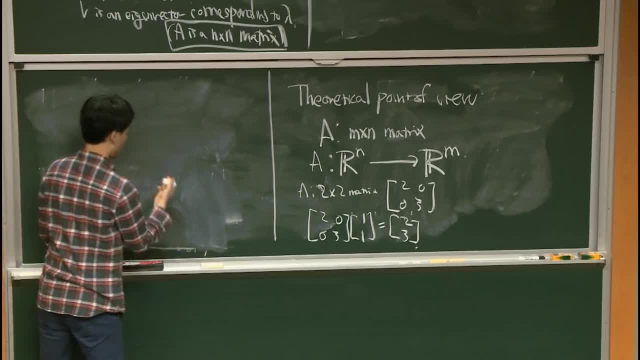 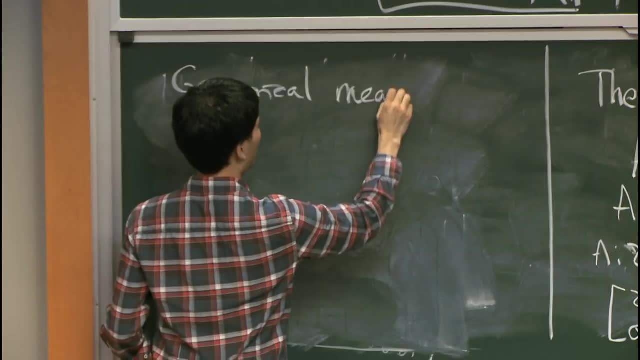 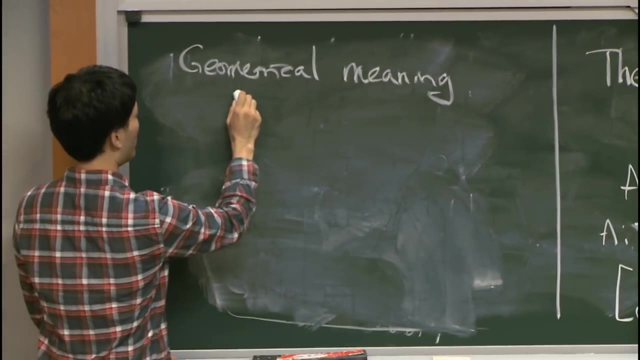 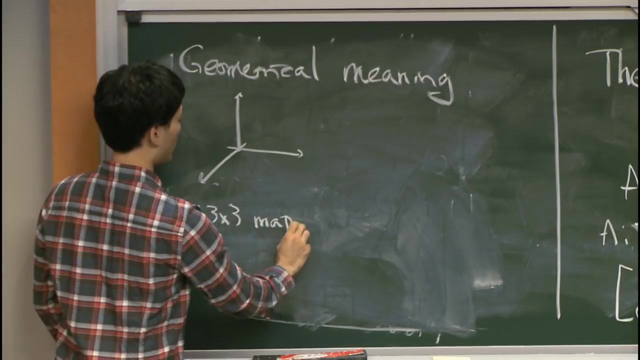 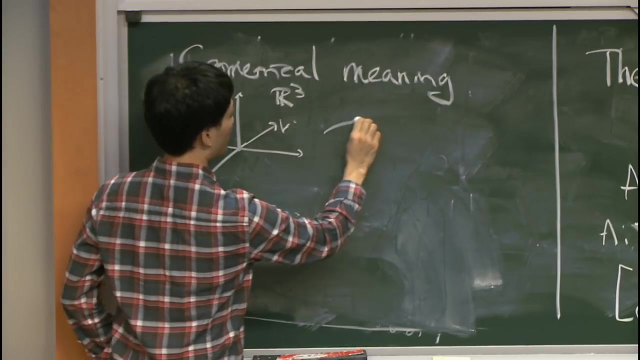 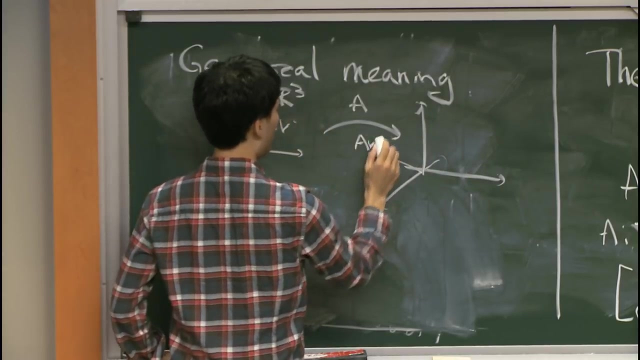 We will see. Now let's go back to the linear transformation point of view. So suppose A is a 3 by 3 matrix, Then A takes a vector in R3. and transforms it into another vector in r3. but if you have this relation, what's? 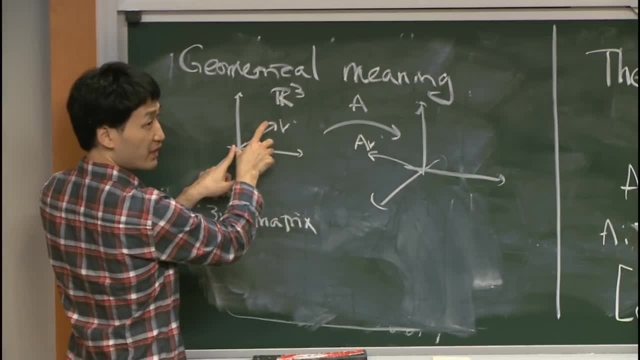 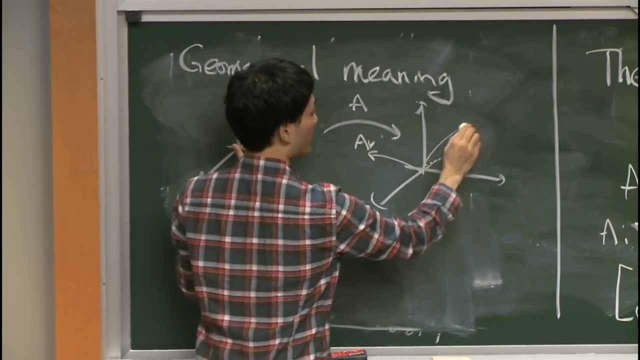 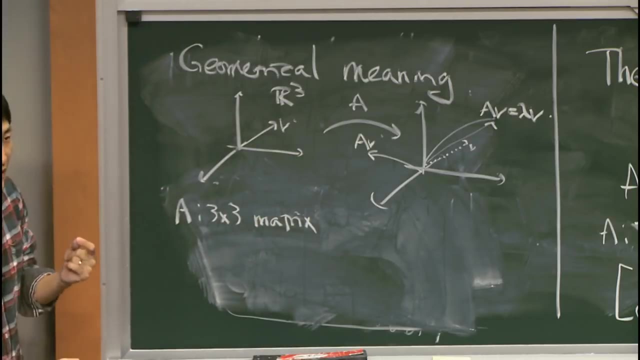 going to happen is a. when applied to V, it will just scale the vector V. if this was the original V, a of V will just be lambda times this vector. that will be our a of V, which is equal to lambda V. so eigenvectors are those special vectors. 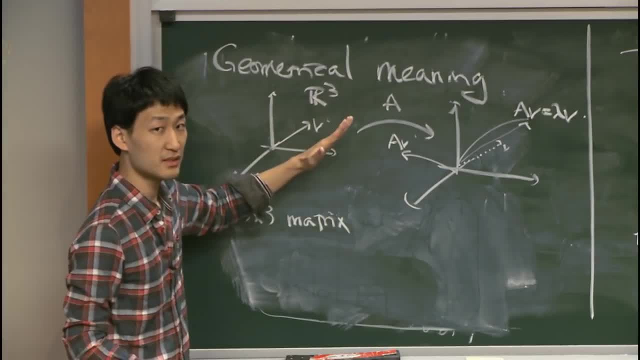 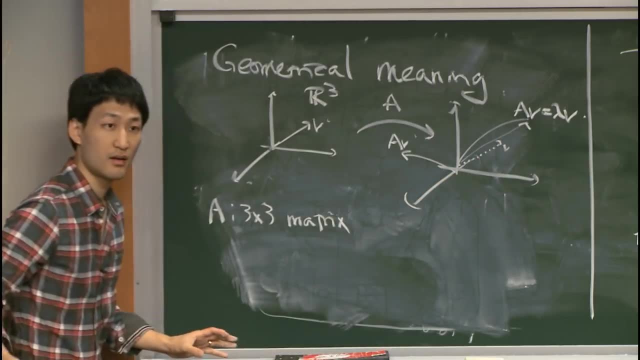 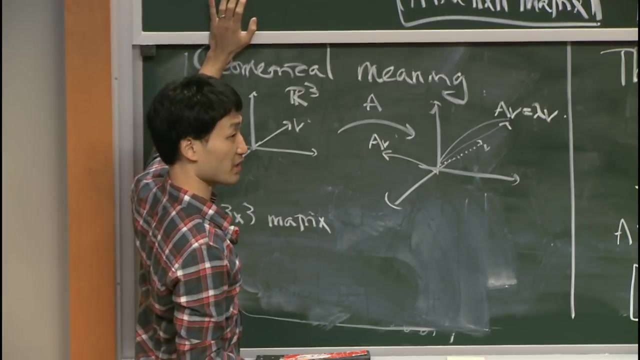 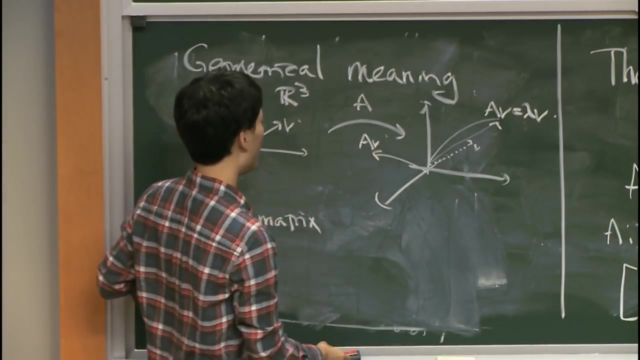 which, when applied, this linear transformation just gets scaled by some amount, which, where that amount, is exactly lambda. so what we established so far, what we recall so far, is every m by n matrix has at least one such direction. there is some vector where the, the linear transformation defined by a, just scales that vector, which is quite 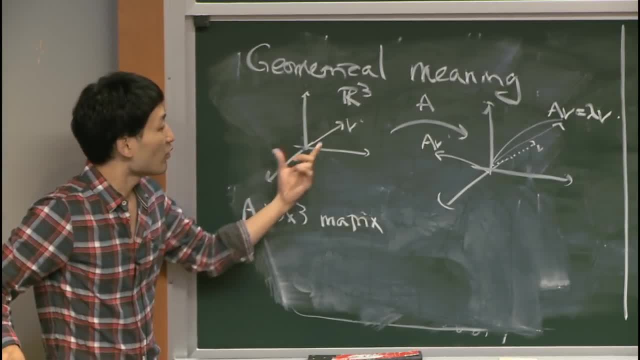 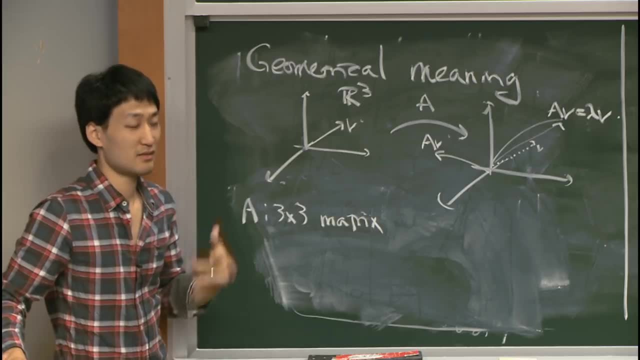 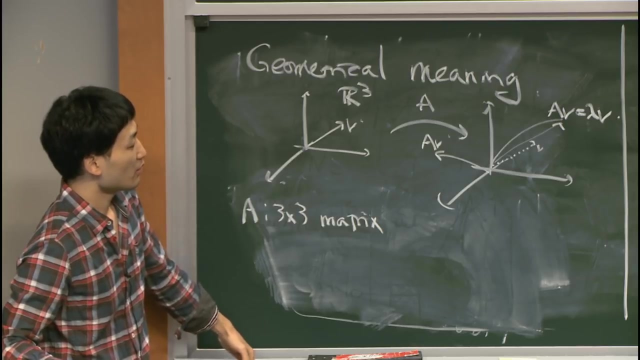 interesting if you'd never thought about it before. there's no reason such vector should exist. of course I'm lying a little bit because this- these might be complex vectors, but at least in comp, in the complex word is complex world is true. so if you think about this, this is very helpful. it gives you 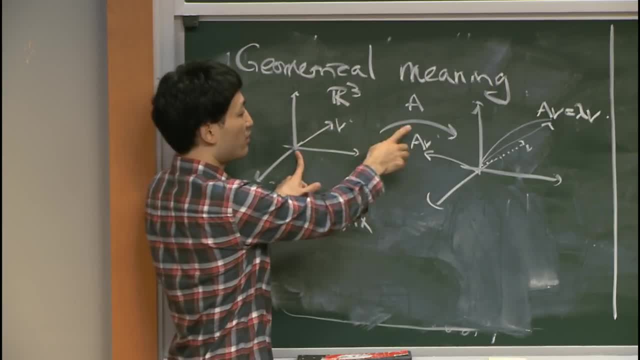 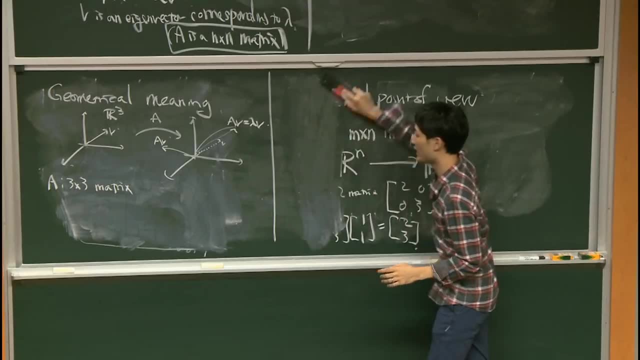 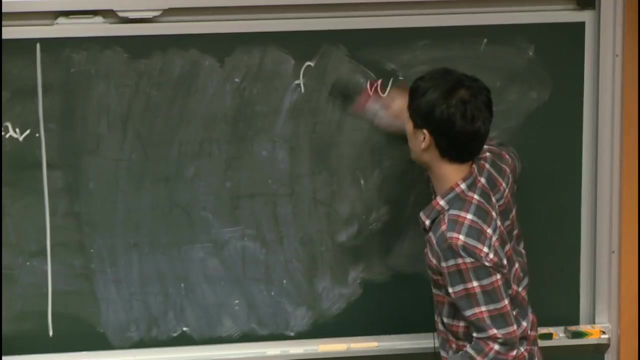 an idea of what a linear transformation is going to look like. okay, so from these vectors, from these vectors point of view, this linear transformation is really easy to understand. okay, that's why eigenvalues and eigenvector are so good. it breaks down the linear transformation into really simple operations. what? let me make that? 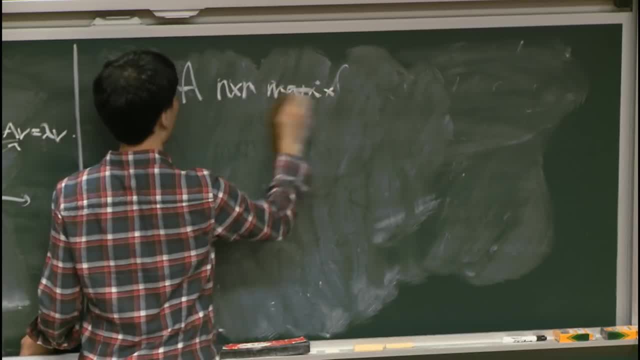 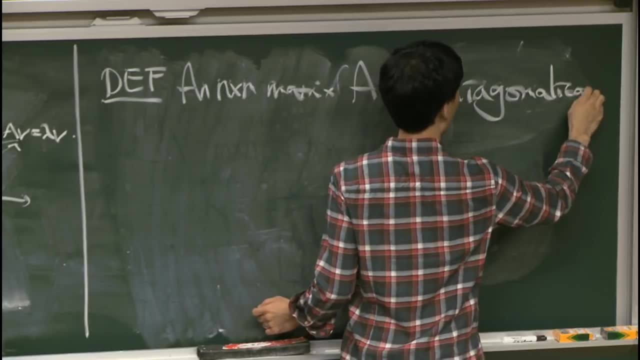 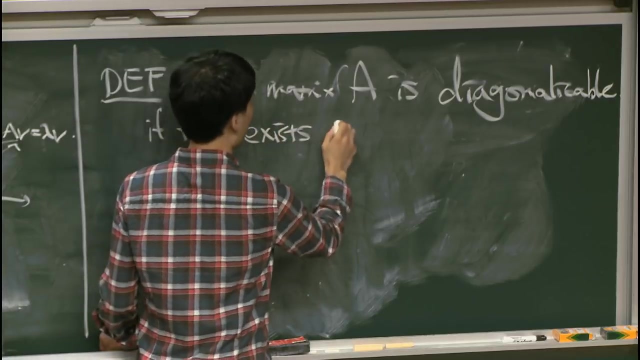 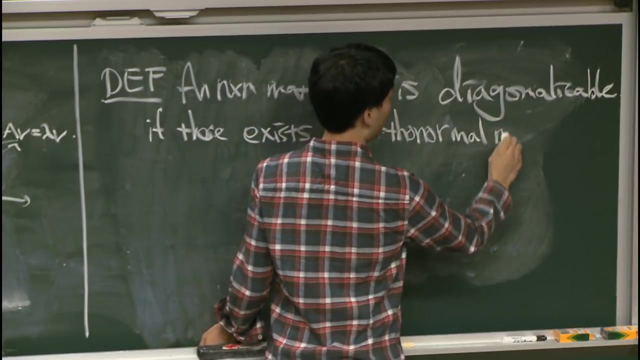 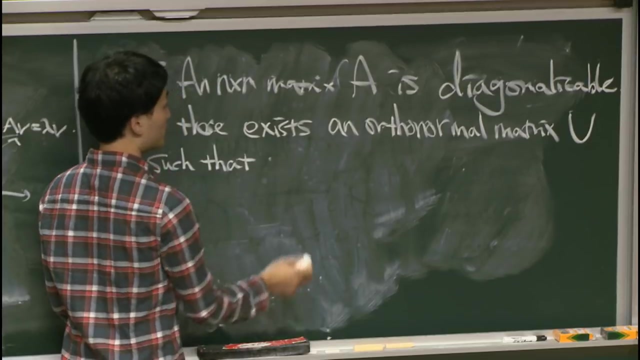 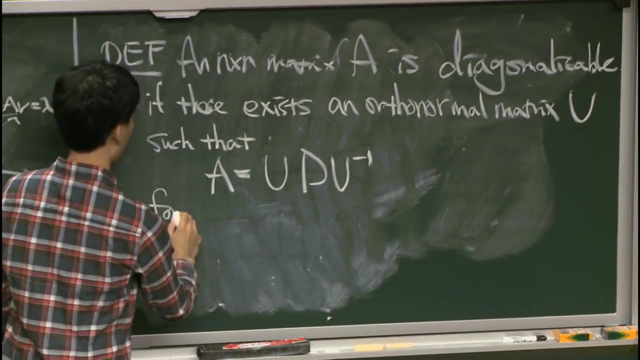 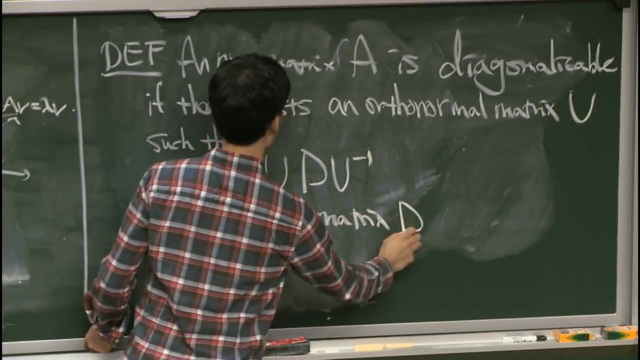 formalize that a little bit more. so in an extreme case We call it diagonalizable. if there exists an orthonormal matrix, I'll call what that is, u, such that a is equal to u times d times u, inverse for a diagonal matrix: d. 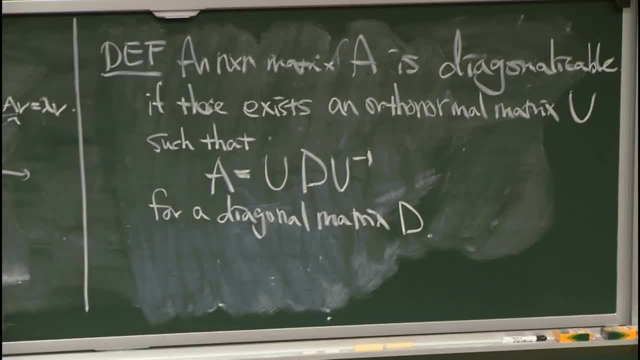 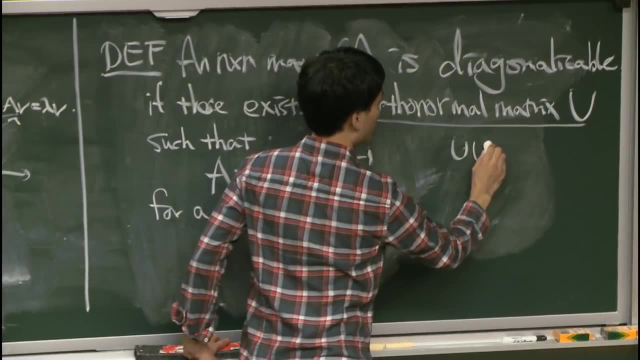 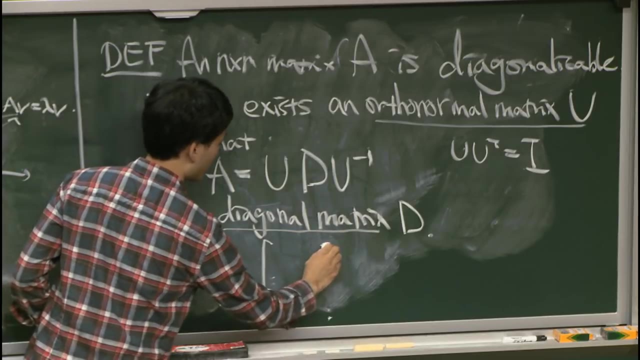 Let me iterate through this a little bit. What is an orthonormal matrix? It's a matrix defined by the relation u times u transpose is equal to the identity. What is a diagonal matrix? It's a matrix whose non-zero entries are all. 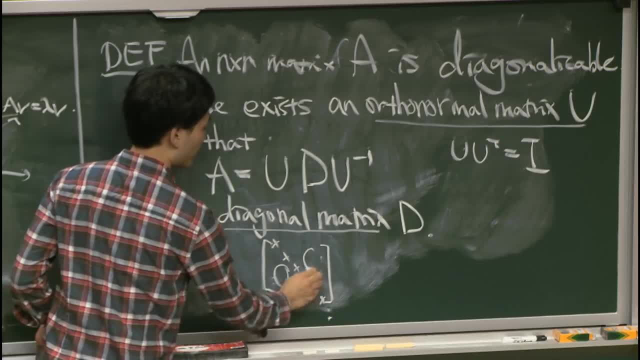 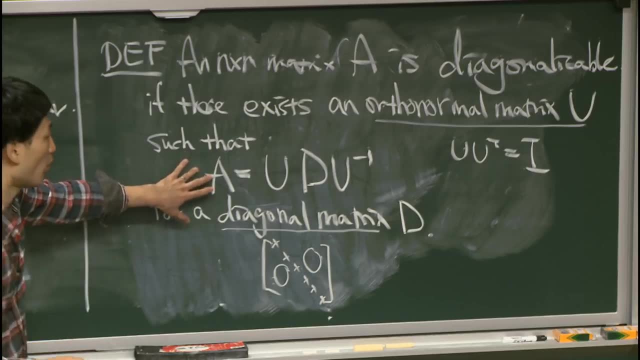 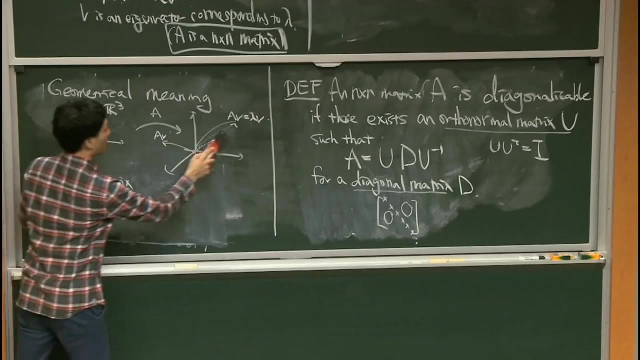 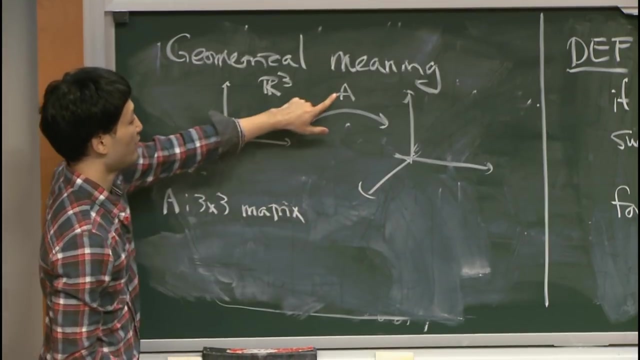 on the diagonal. all rest are 0.. Why is it so good to have this decomposition? What does it mean to have an orthonormal matrix like this? It means, basically I'll just explain what's happening If that happens: If a matrix is diagonalizable, if this a is diagonalizable. 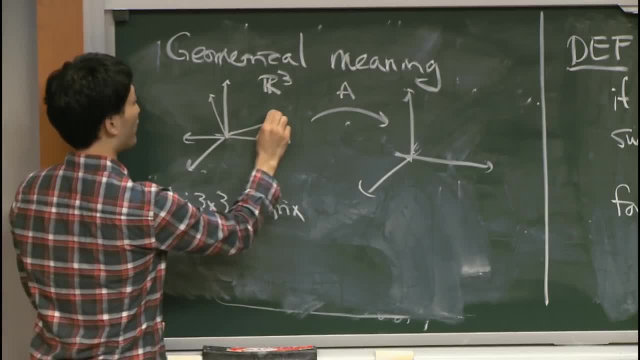 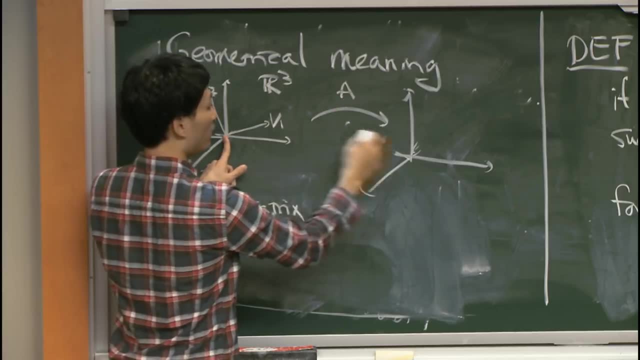 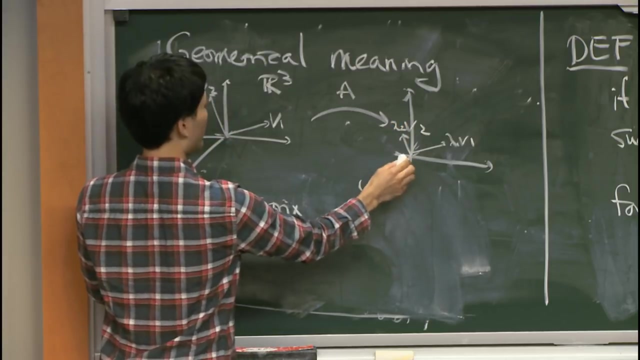 there will be three directions: v1,, v2, v3,, such that, when you apply this, a v1 scales by some lambda 1, v2 scales by some lambda 2, and v3 scales by some lambda 3.. 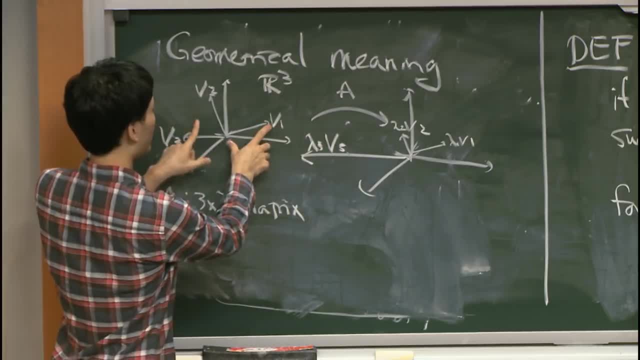 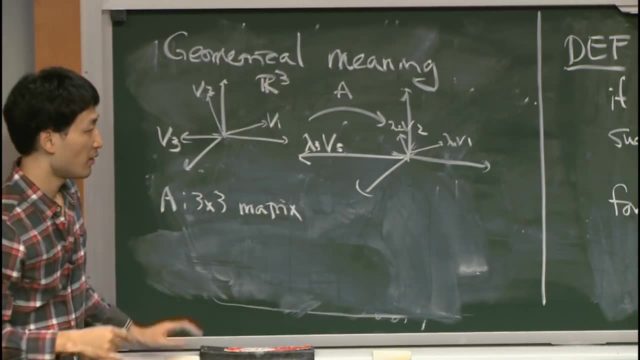 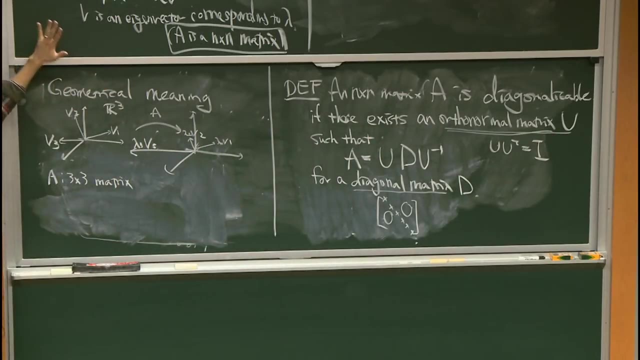 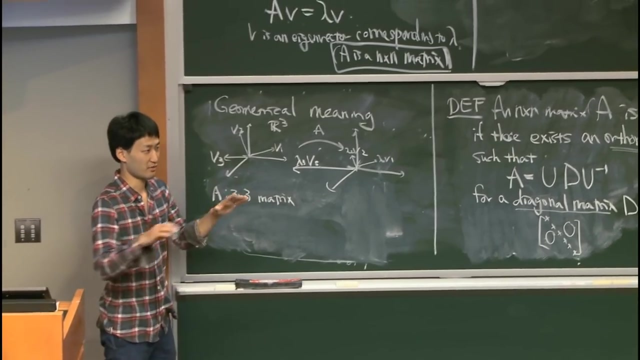 So you can completely understand the transformation a just by looking, just by, just in terms of these three vectors. OK, So this, the stuff here, will be the most important thing that you'll use in linear algebra throughout this course. So let me repeat it really slowly. 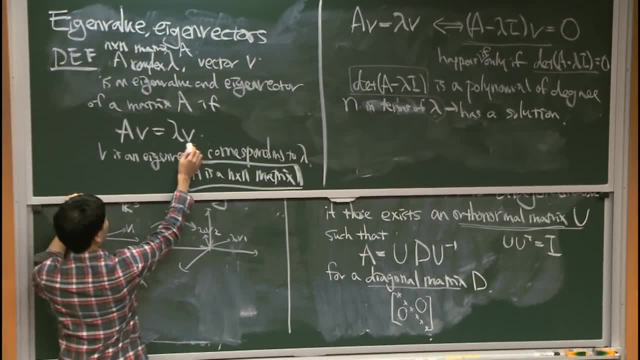 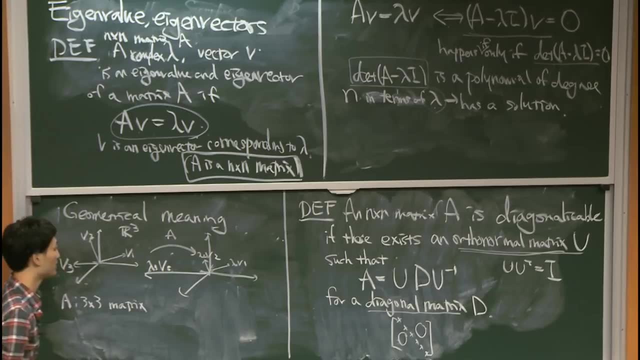 OK, So an eigenvalue and eigenvector is defined by this relation. OK, We know that there are at least one eigenvalue for each matrix and there is an eigenvector corresponding to it, And eigenvectors have this geometrical meaning. 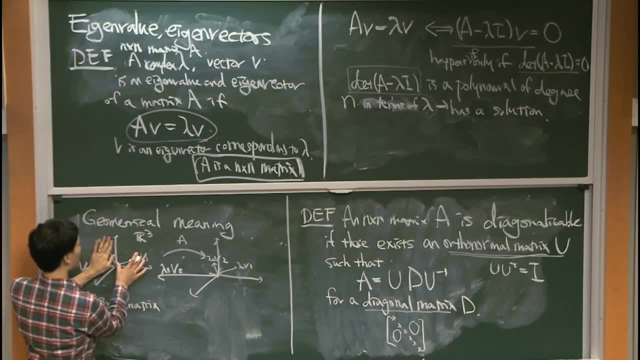 where a vector is an eigenvector if the linear transformation defined by a just scales that vector. So in R for R setting, the real good matrices are the matrices which can be broken down into these directions. OK, And those directions are defined by this u. 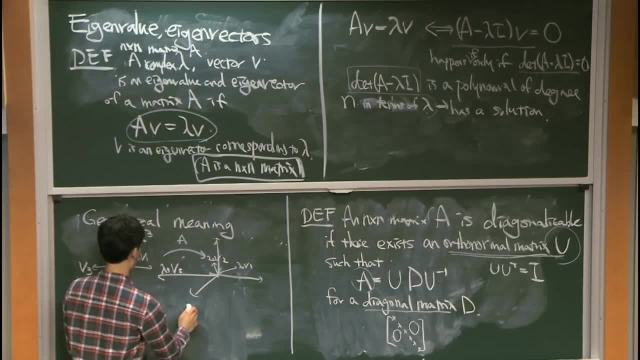 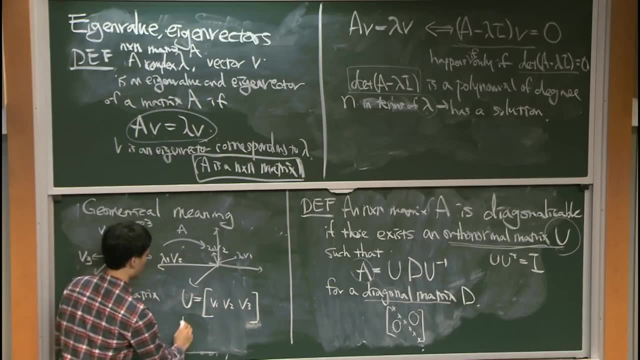 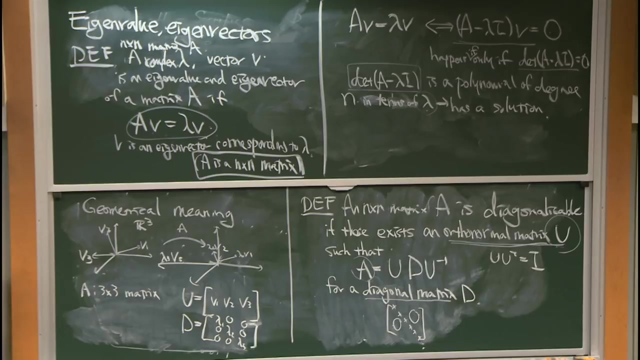 And d defines how much it will scale. So in this case u will be our v1, v2, v3.. And d will be our lambda 1, lambda 2, lambda 3, all 0.. Any questions so far? 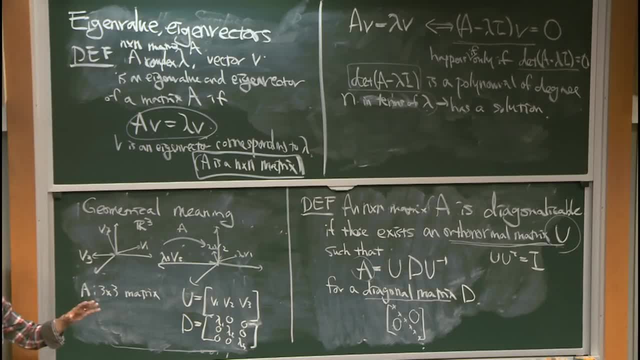 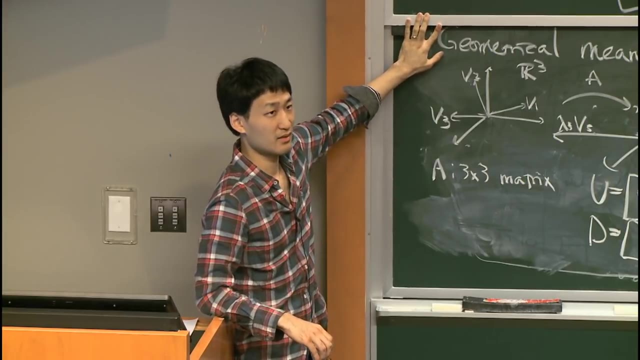 OK, So that is abstract. Now remember the question I posed in the beginning. So remember that matrix where we have stocks and dates and stock prices and entries. What will an eigenvector of that matrix mean? What will an eigenvalue mean? 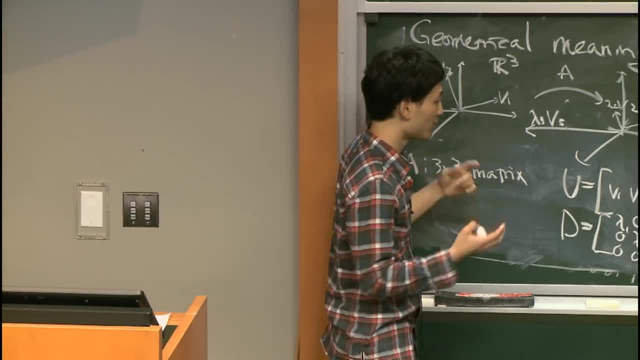 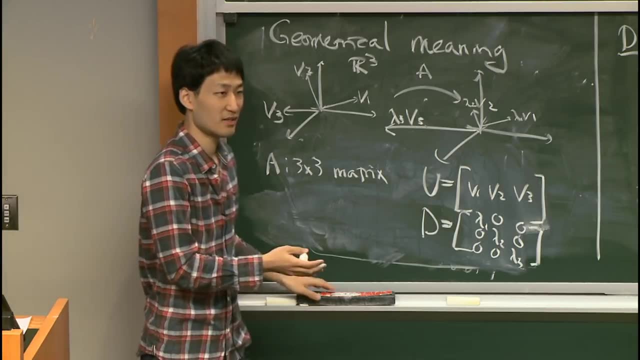 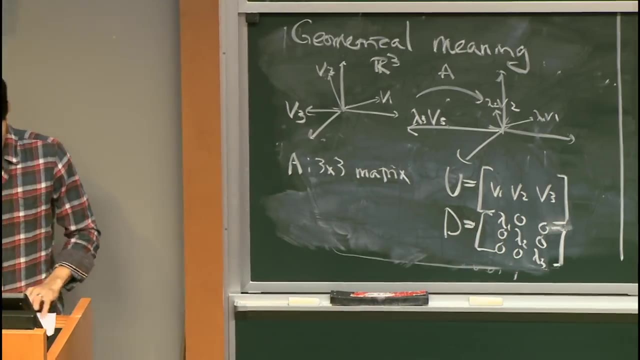 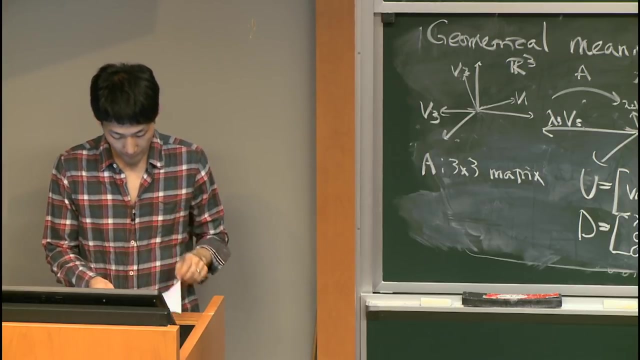 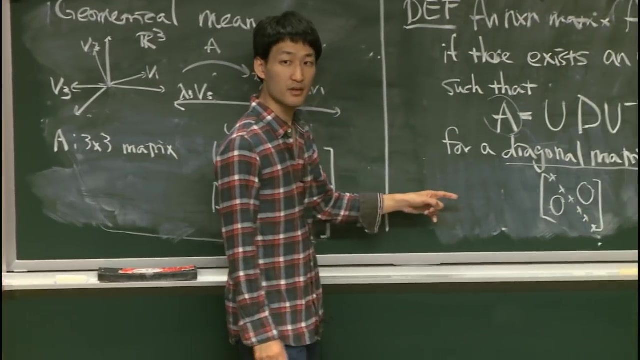 OK, So try to think about that question. OK, So try to think about that question. It's not like it will have some physical counterpart, but there's some really interesting thing going on there. OK, The bad news is that not all matrices are diagonalizable. 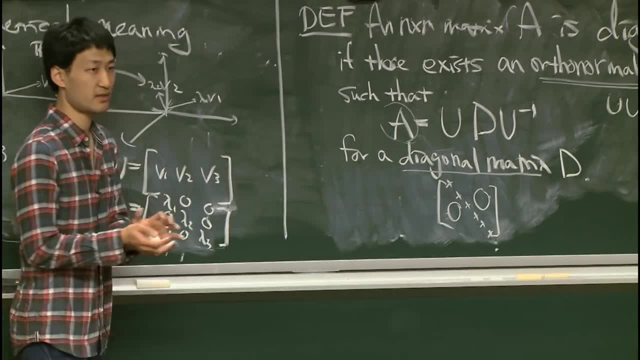 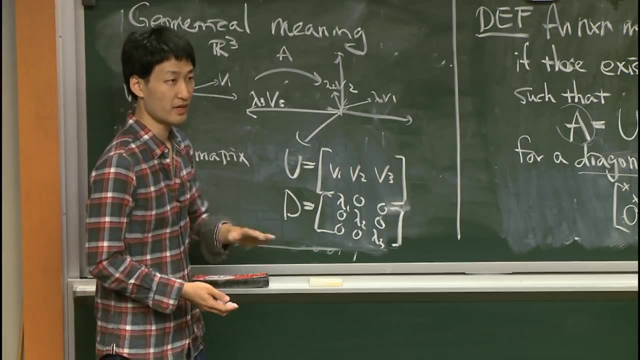 OK, If a matrix is diagonalizable, then it's going to be a vector. OK, If a matrix is diagonalizable, it's really easy to understand what it does, because it really breaks down into these three directions, if it's a 3 by 3.. 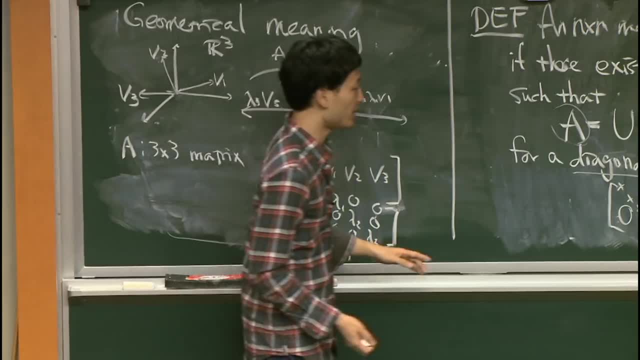 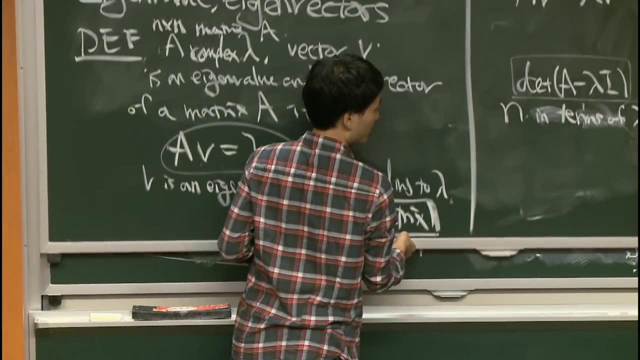 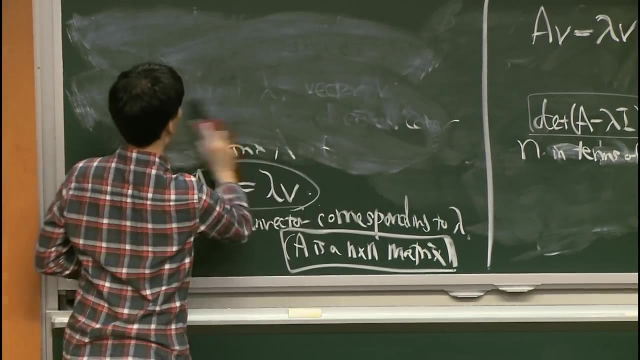 It's an n by n. It breaks down into n directions. Unfortunately, not all matrices are diagonalizable, But there is a very special class of matrices which are always diagonalizable And fortunately we will see those matrices throughout the course. Most of the matrices n by n matrices we will study. 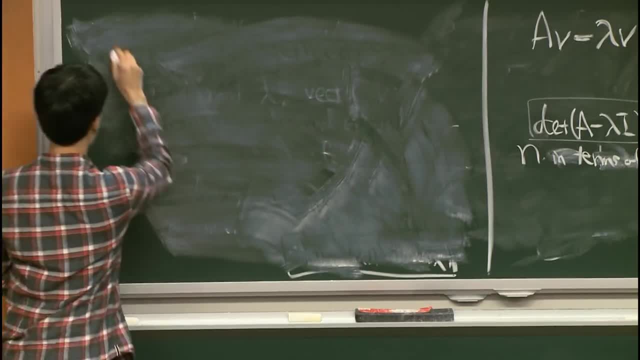 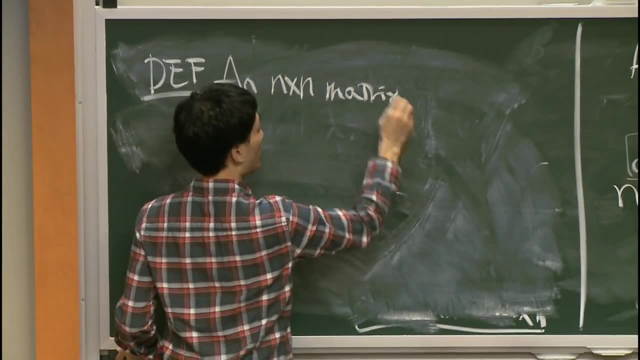 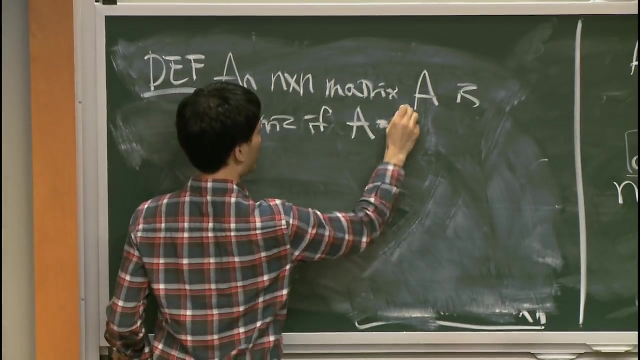 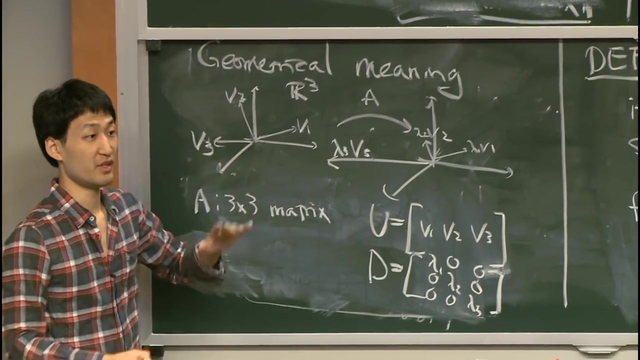 They fall into this category. So an n by n matrix A is symmetric if A is equal to H. OK, Before proceeding, please raise your hand if you're familiar with all the concepts so far, OK, Good, I have a feeling. 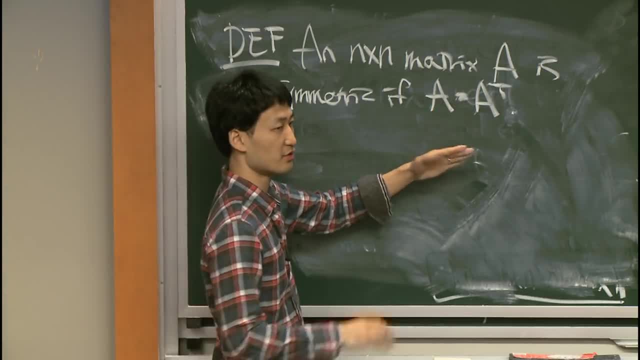 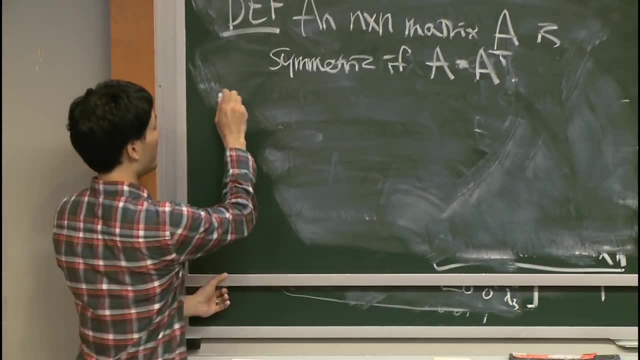 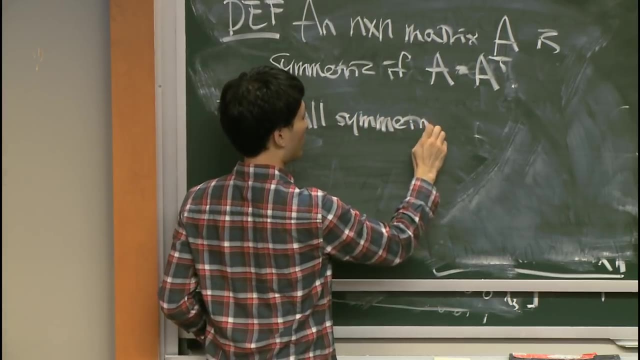 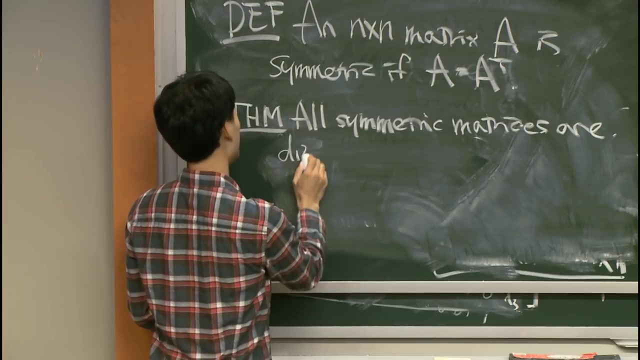 OK, So a matrix is symmetric if it's equal to its transpose. A transpose is obtained by taking the mirror image across the diagonal, And then it is known that all symmetric matrices are diagonalizable. Ah, I made another mistake. Orthonormally. 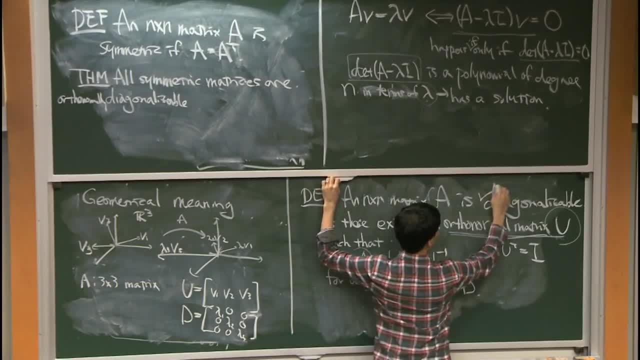 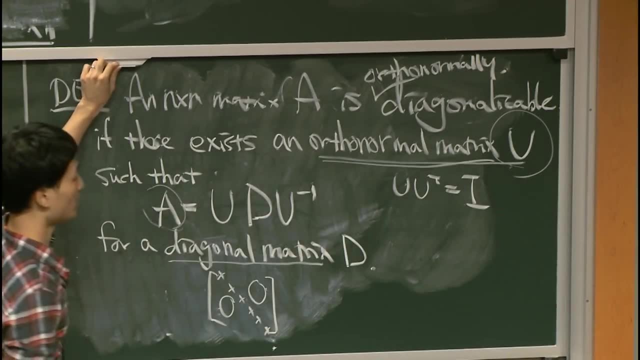 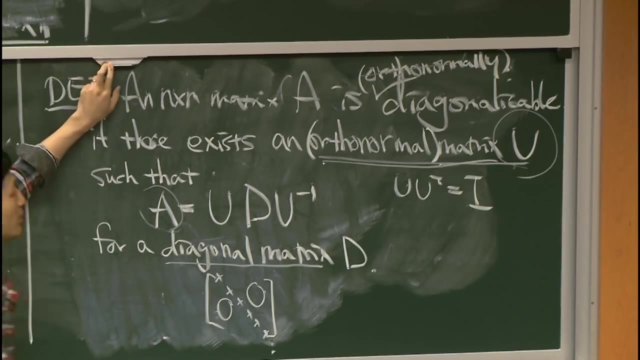 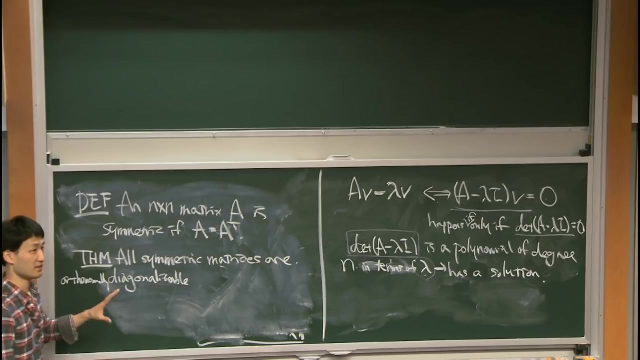 So this I missed. Matrix is orthonormally diagonalizable, So it's diagonalizable if we drop this condition. OK, Then replace it with an inverse, An invertible, OK. So symmetric matrices are really good And fortunately, most of the n by n matrices. 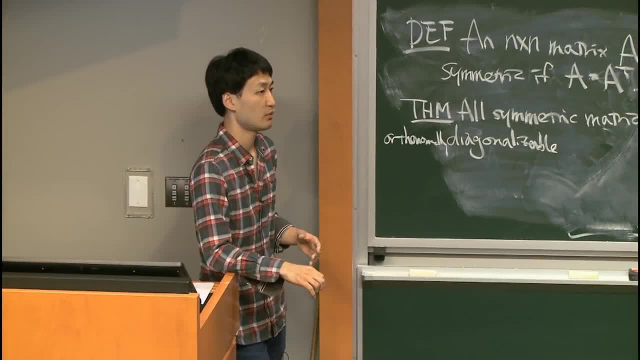 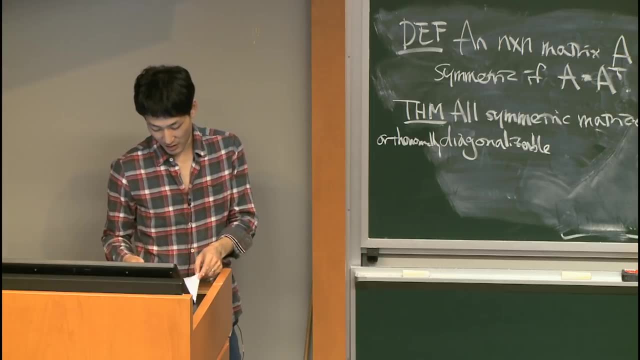 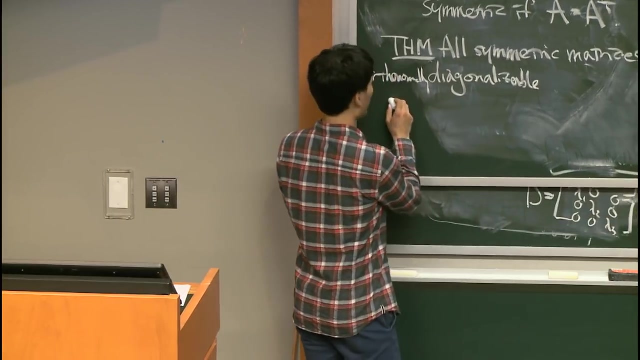 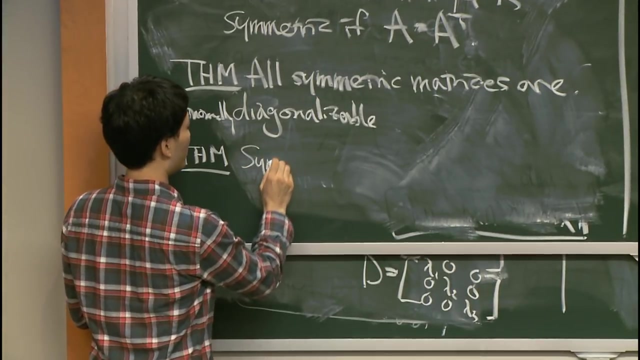 that we will study are symmetric. Just by the nature of it, it will be symmetric. The one I gave as an example is not symmetric. It's not symmetric, OK, OK, But I will address that issue in a minute. And another important thing is symmetric matrices. 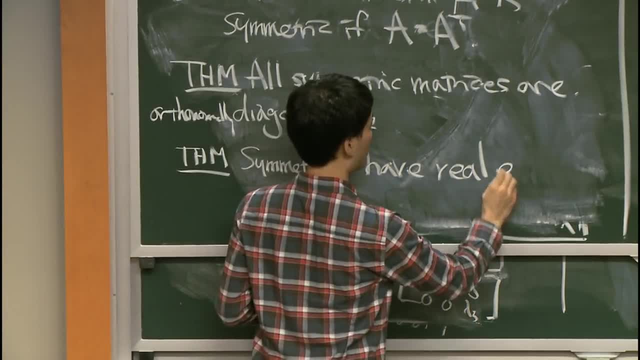 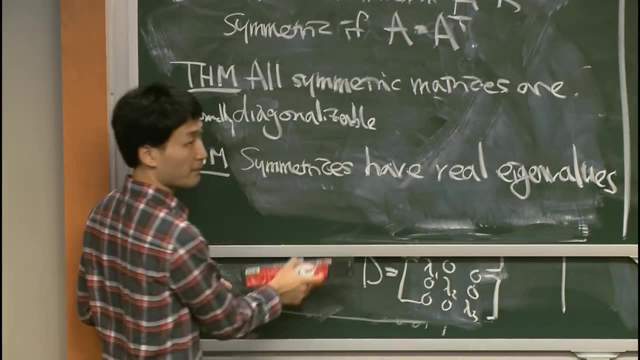 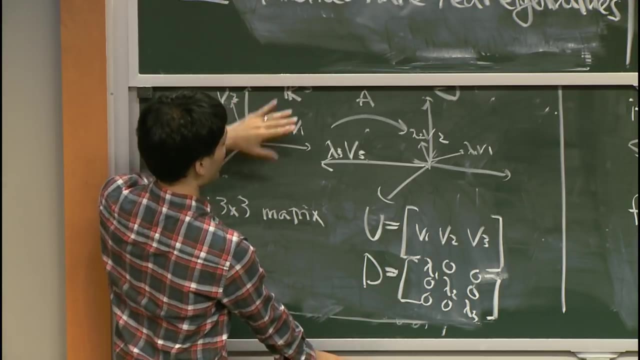 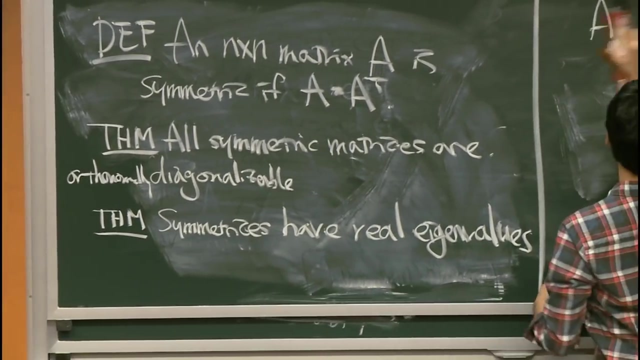 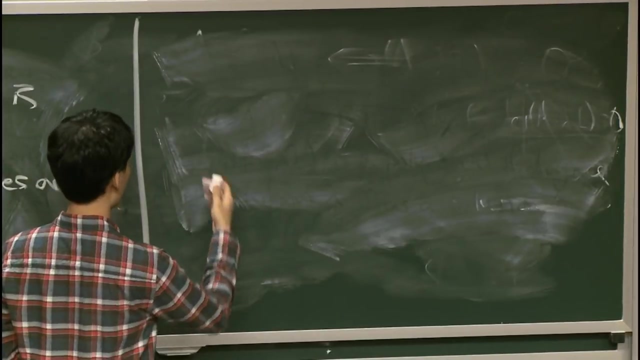 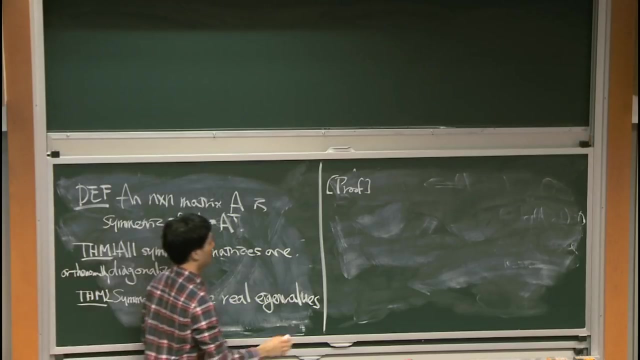 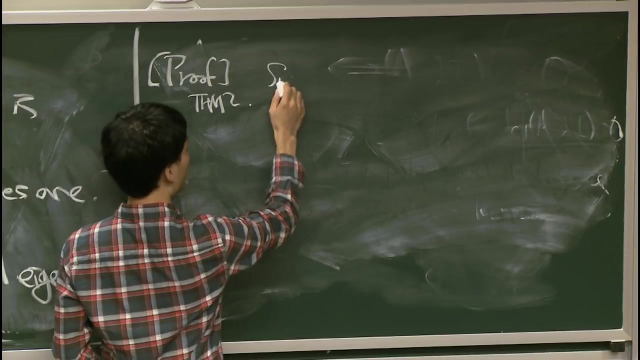 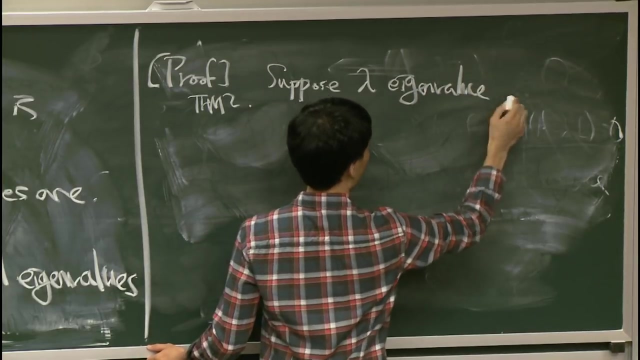 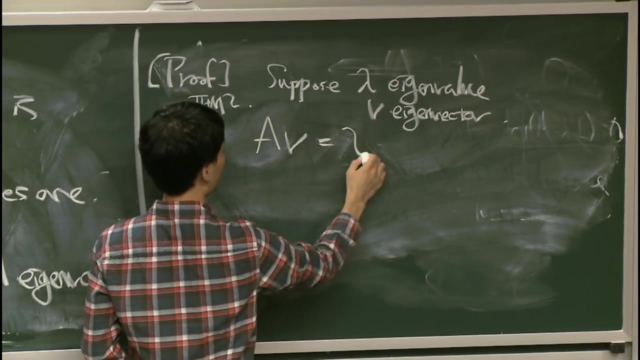 have real eigenvalues. So really, This geometrical picture for symmetric matrices, this picture is really the picture you should have in mind. OK, So proof of theorem two: Suppose lambda is an eigenvalue with eigenvector v, Then by definition we have this: 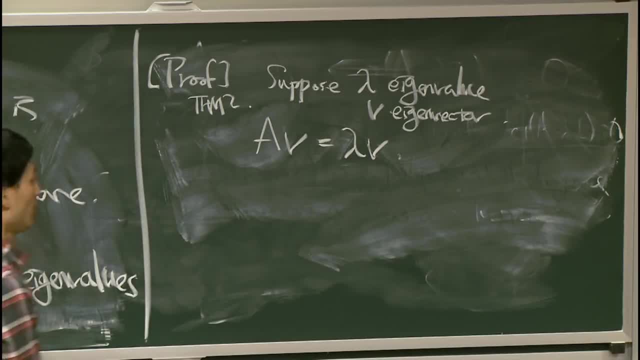 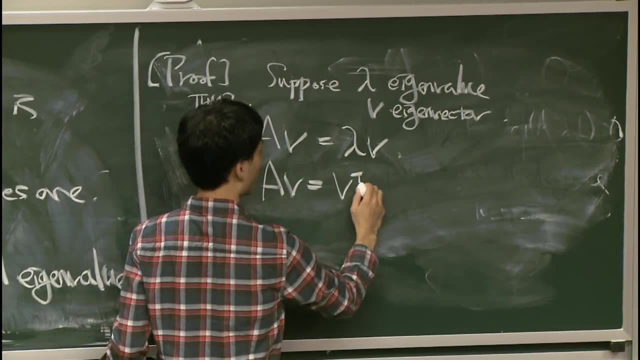 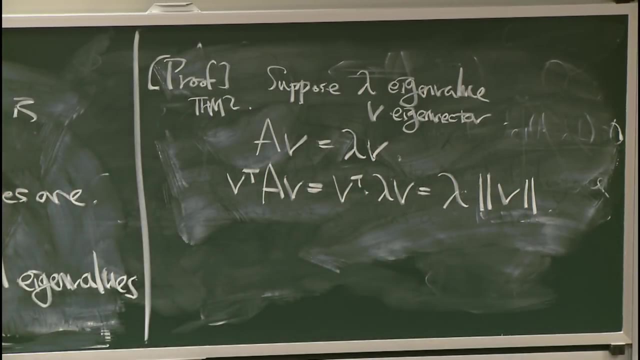 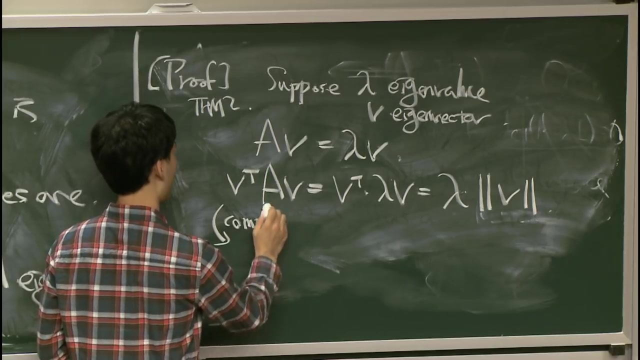 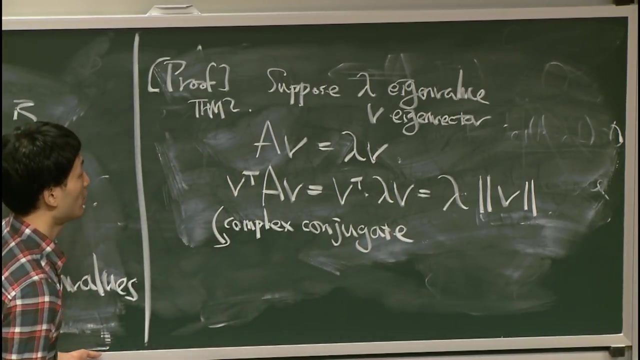 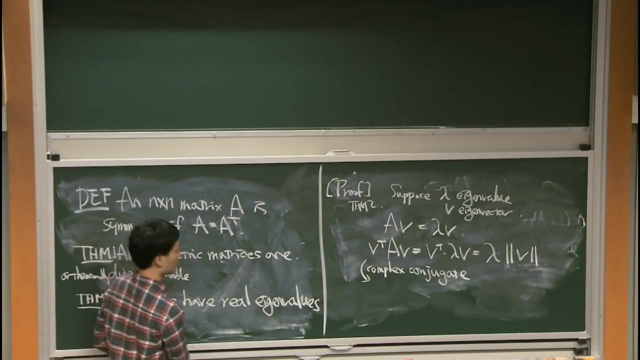 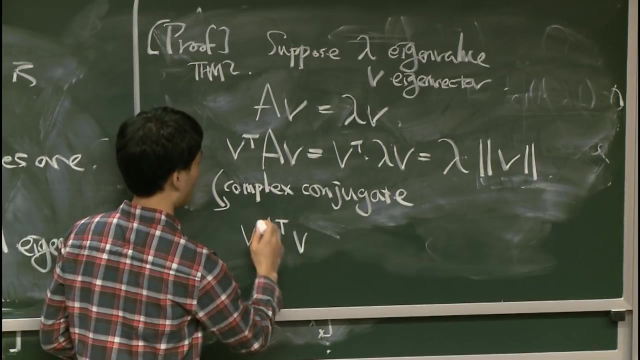 OK. Now multiply v, transpose on both sides, OK. And multiply v, transpose on both sides, OK. And multiply v, transpose on both sides. It is, lambda times, the norm of v. Now take the complex conjugate. Then first to conjugate, we have v a, t, v, t a t v. 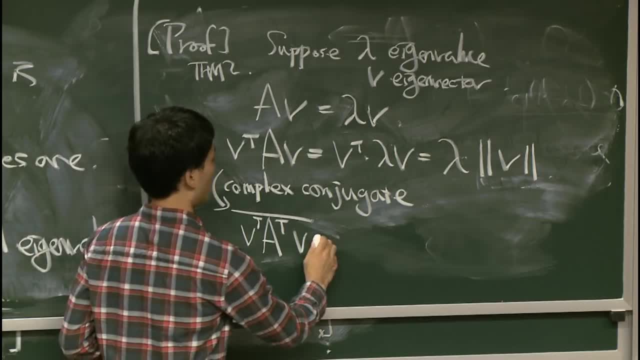 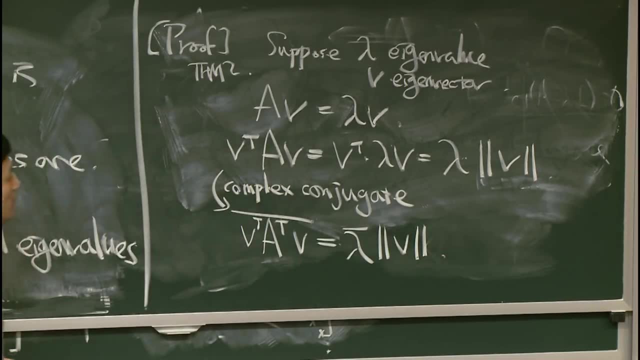 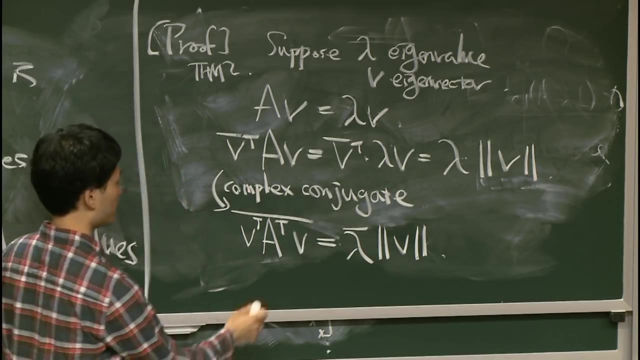 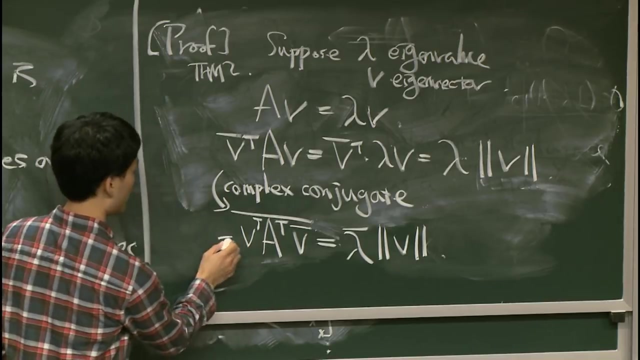 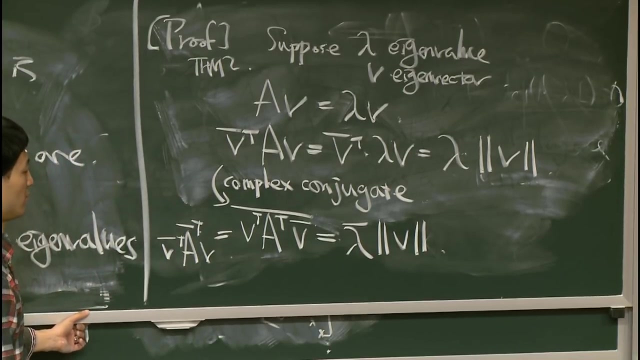 And then take the conjugate of it And we get this. OK, We get lambda v a t, v, t a v. OK, And this side is equal to v t a v. But because a is real, 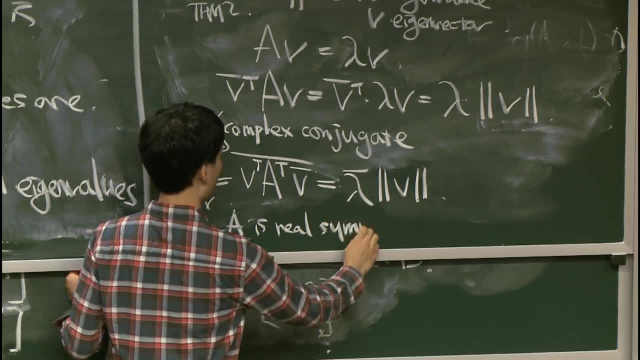 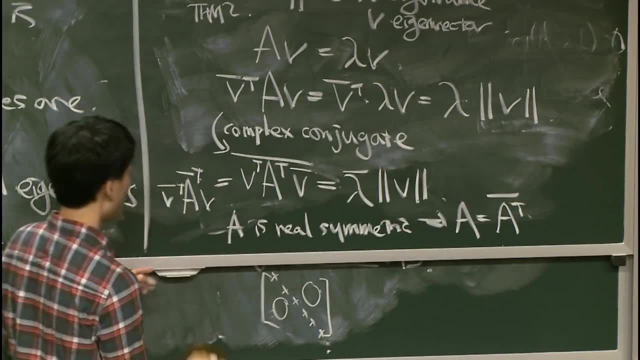 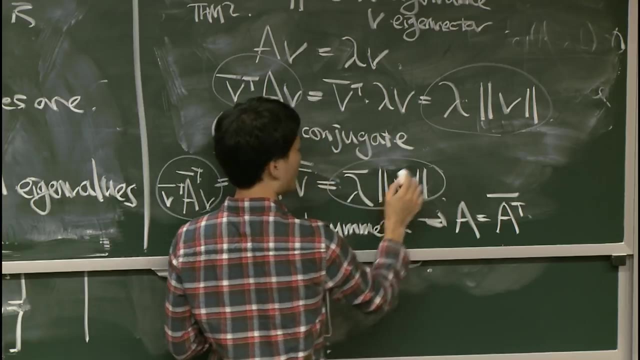 symmetric. We see that a is equal to the conjugate of A, So this expression and this expression is the same. The right side should also be the same. That means lambda is equal to the conjugate of lambda, So lambda has to be real. 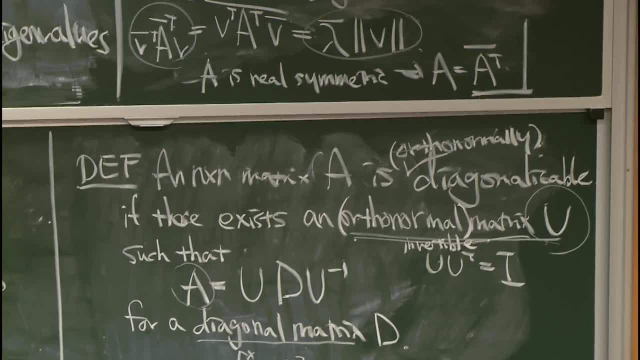 And the other side should also be the same. We still have to multiply v transpose. We just have to multiply v transpose to get the integration. So this expression is 2.. And we have that, And now we're going to compute the balance. 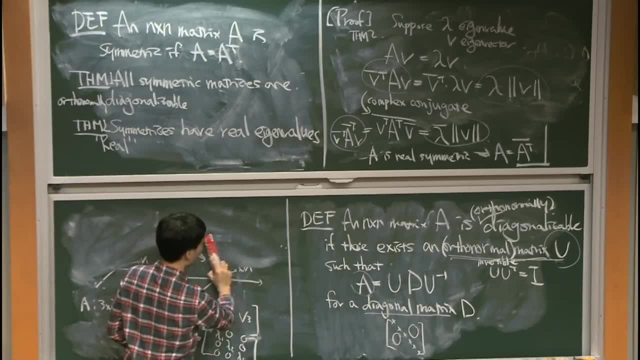 So we're going to compute And we just have to calculate the full function of this, And I just want to say that we just do this one. We just know that this is our 0, we just have to x minus 1.. 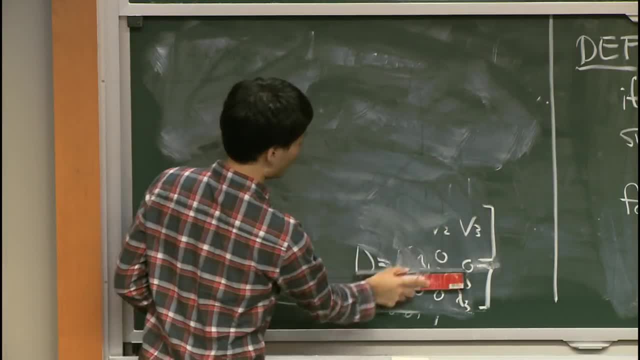 And we're going to do the same thing for this one. We do this one and we do this one, And we do this one and we do this one. So that's다 and i's equal to 1.. And we know that v transpose is 0 and we know that it's 0.. 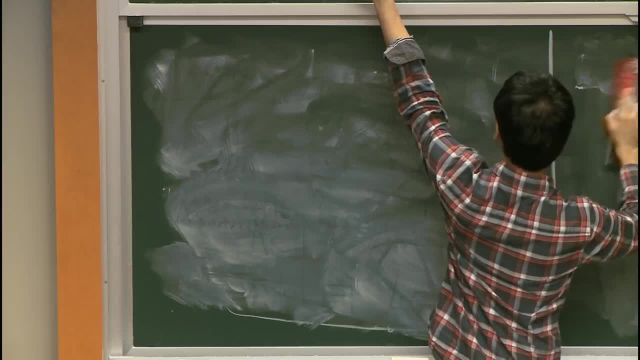 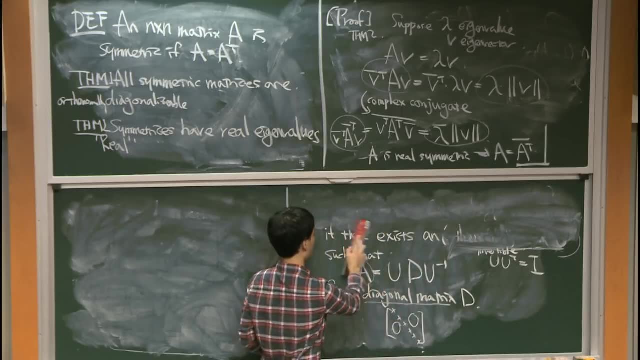 And we know that v transpose is zero. So the derivative of the matrix is going to be 1.. important to remember these two theorems. Whenever you see a symmetric matrix, you should really feel like you have control on it because you can diagonalize it. 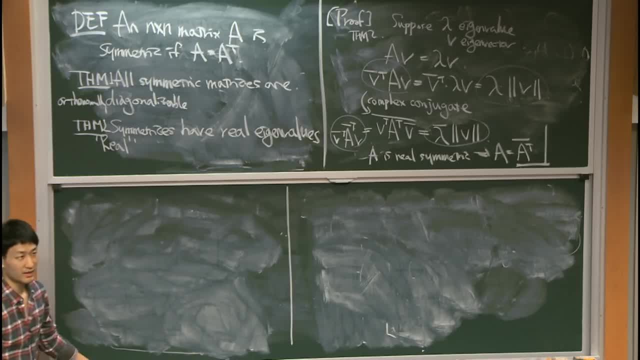 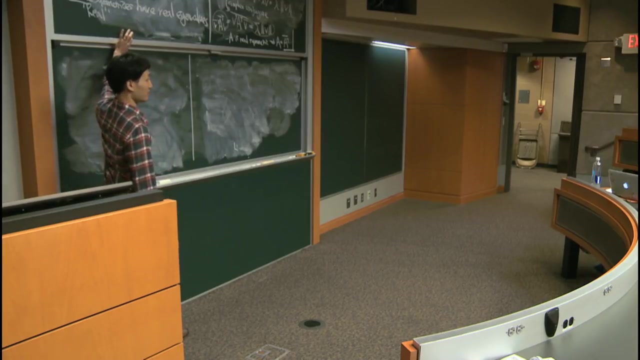 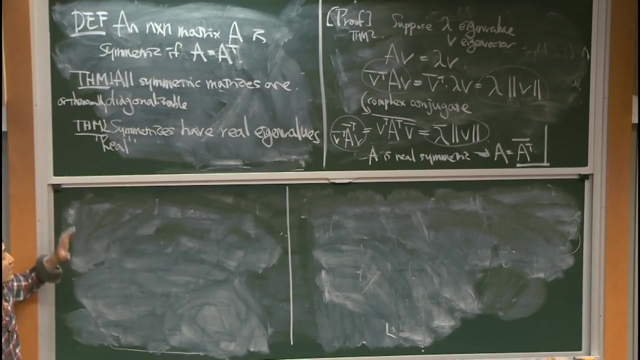 And, moreover, all eigenvalues are real and you have really good control on symmetric matrices. OK, that's good. That was when everything went well. We can diagonalize it. So so far, we saw that for a symmetric matrix, we can diagonalize it. 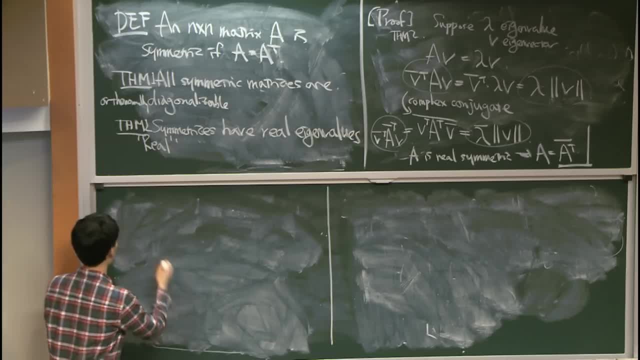 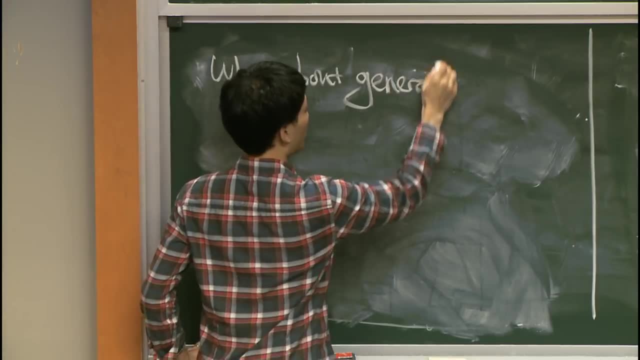 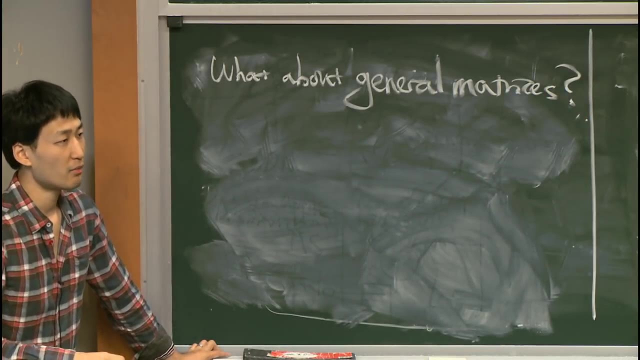 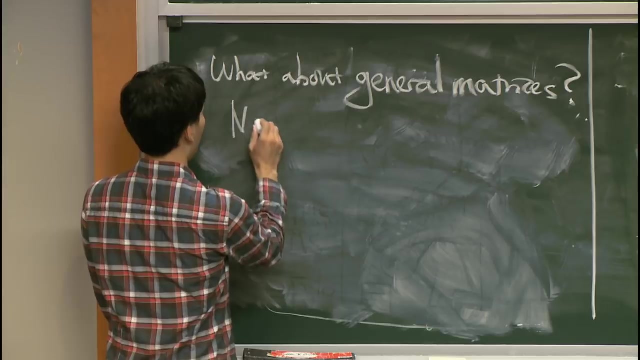 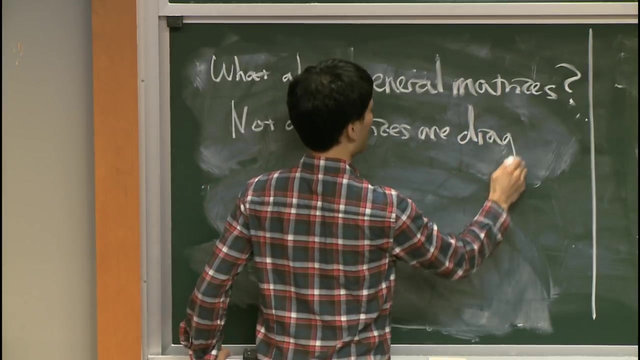 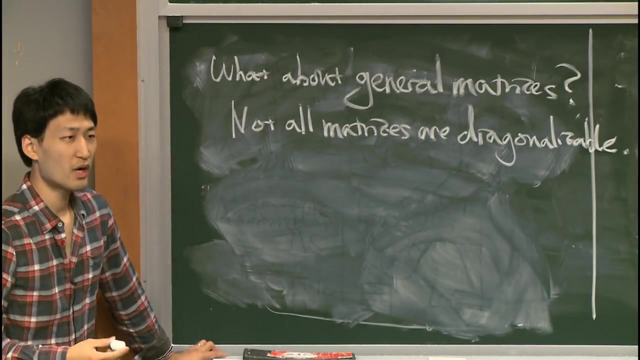 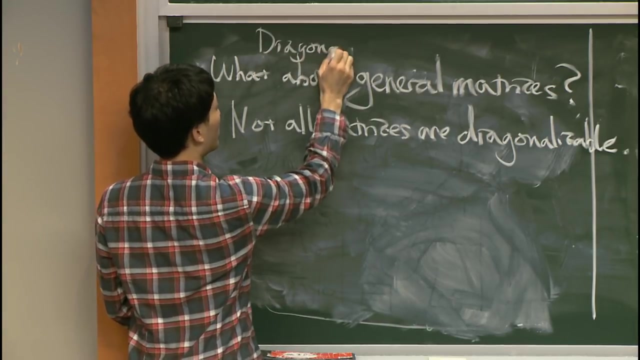 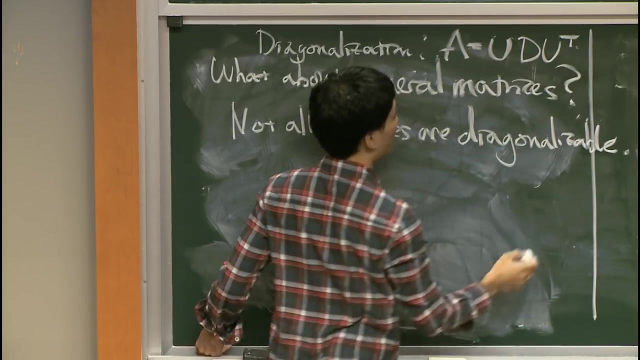 It's really easy to understand. But what about general matrices? In general, not all matrices- Marriages- are diagonalizable first of all, But sometimes we still want a decomposition like this. So diagonalization was So: a equals u times d times u transpose or u inverse. 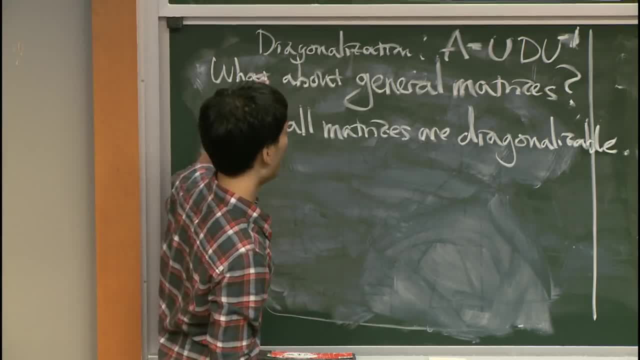 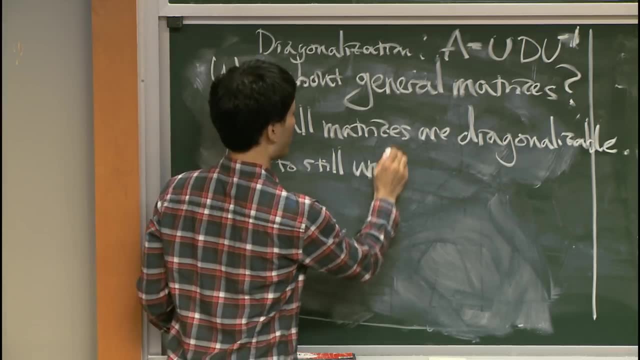 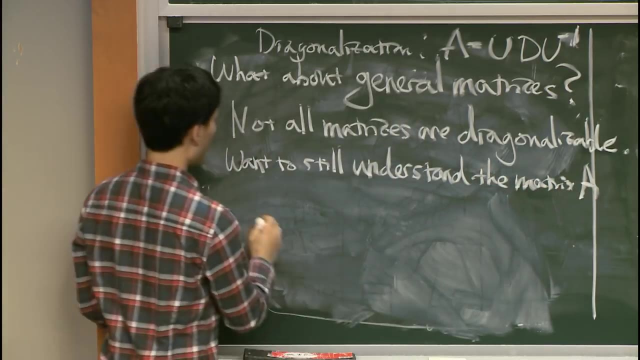 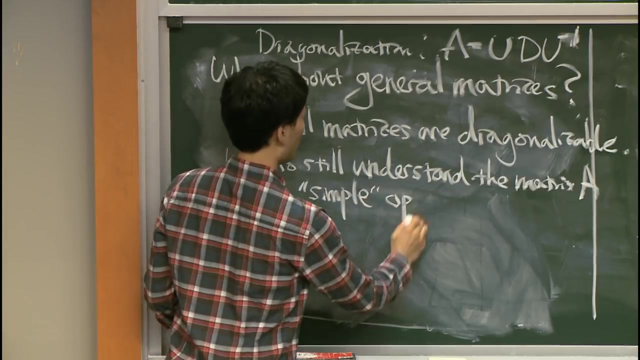 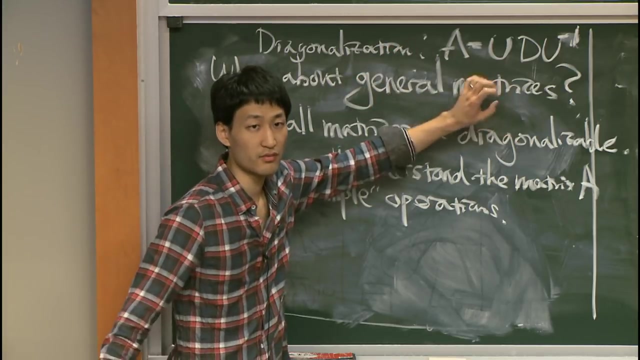 Oh, we want something similar, We want to understand. So our goal: we want to still understand the matrix given matrix A through through simple operations such as scaling. When the matrix was a diagonalizable matrix, this was done. 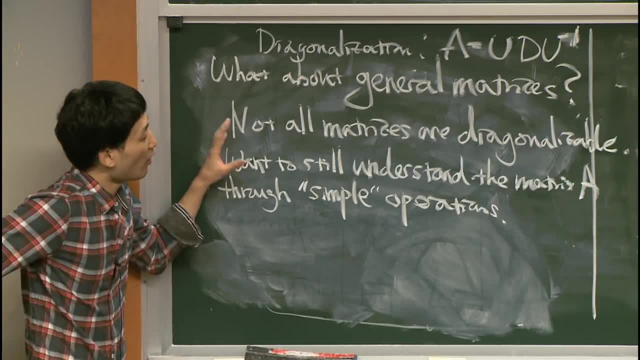 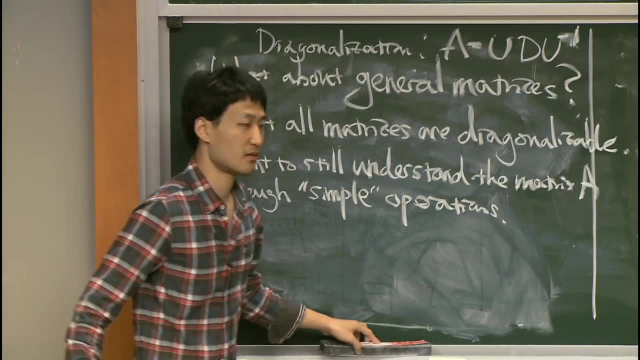 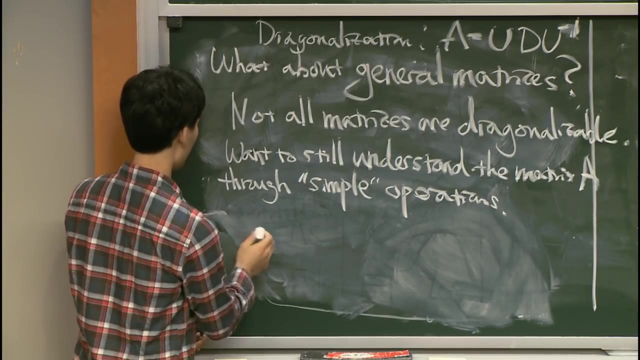 This was possible. Unfortunately, it's not always diagonalizable, So we have to do something else. So that's what I want to talk about, And luckily, the good news is there is a nice tool we can use for all matrices, even though it's slightly weaker. 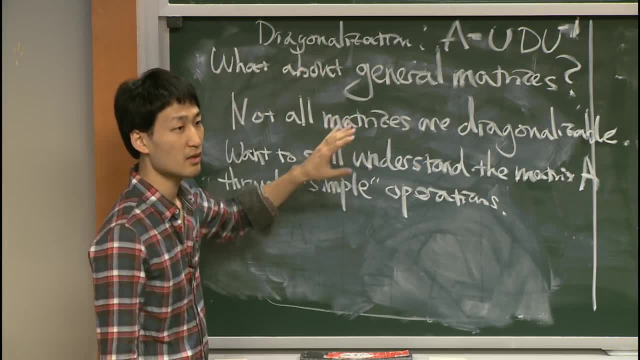 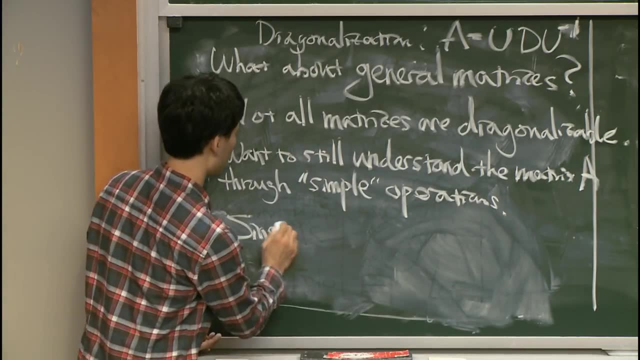 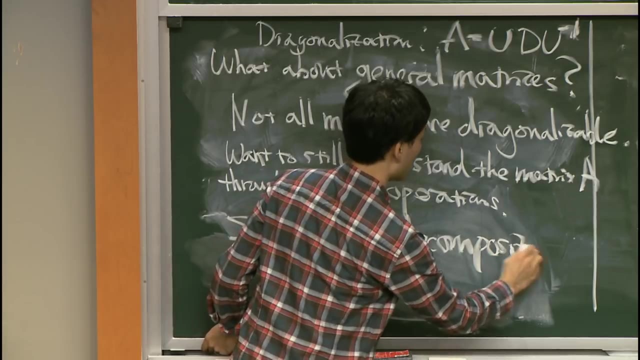 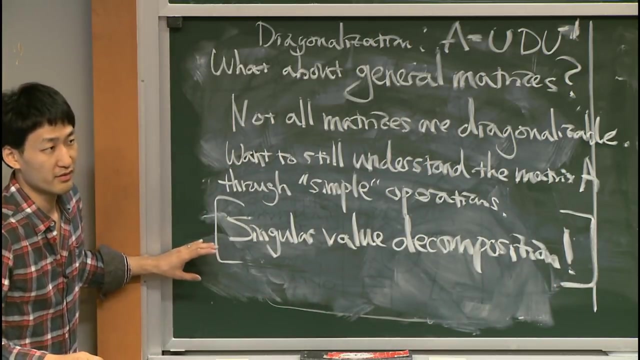 In fact a little bit more weaker than this diagonalization, But still it distills some very important information of the matrix. So it's called singular value decomposition. So this will be our second tool of understanding matrices. It's very similar to this diagonalization. 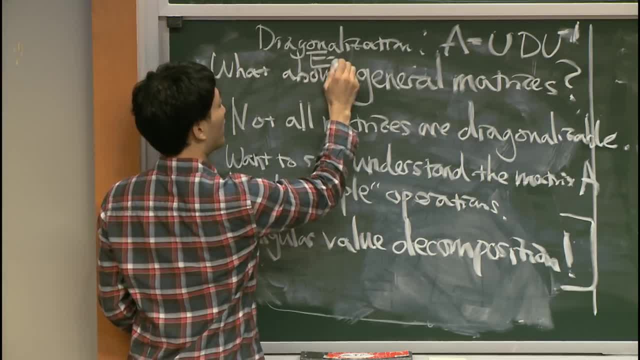 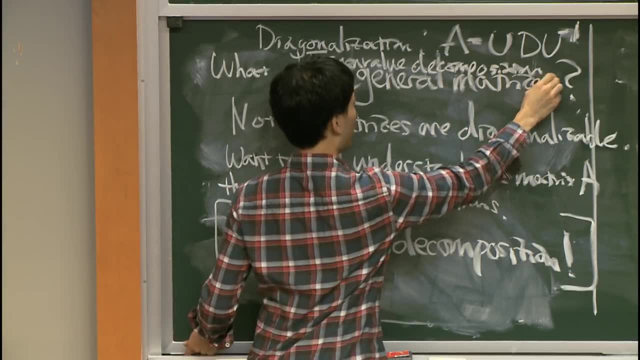 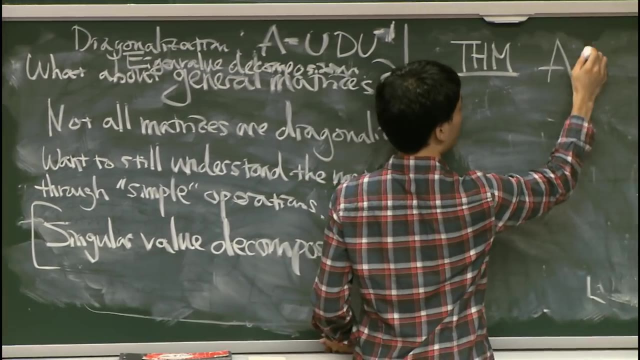 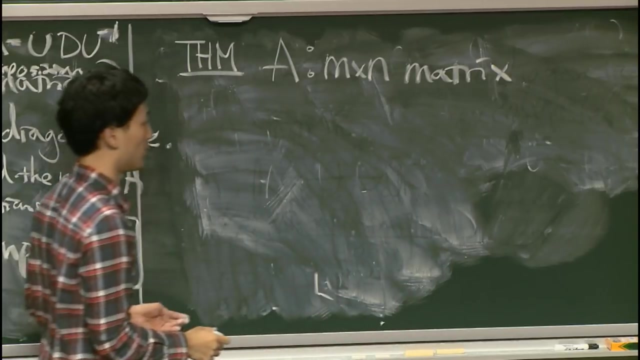 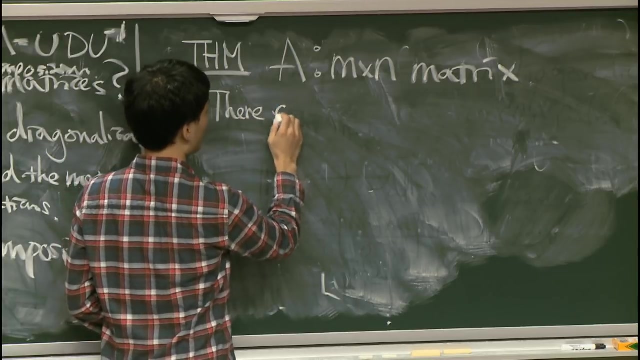 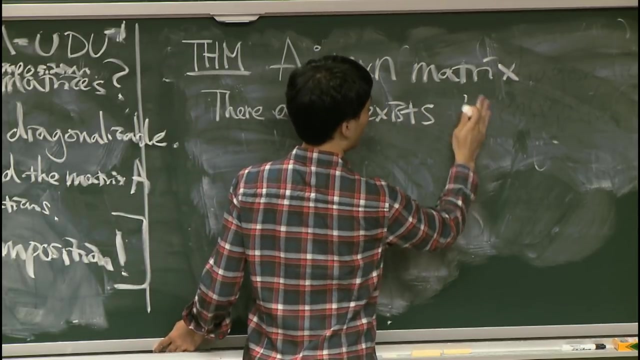 or in other words, I call this eigenvalue decomposition. But it has a slightly different form. So what is its form? So it's theorem. So let A be an m by n matrix, Then there always exists u orthonormal matrices. 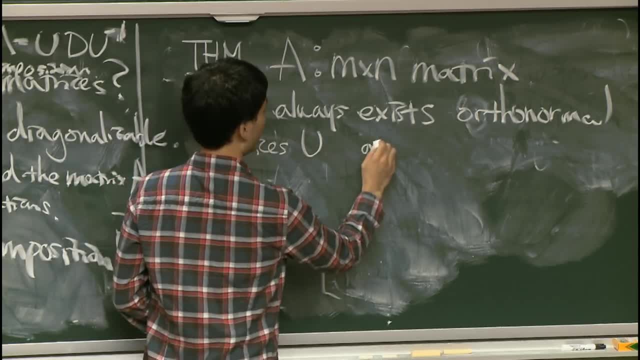 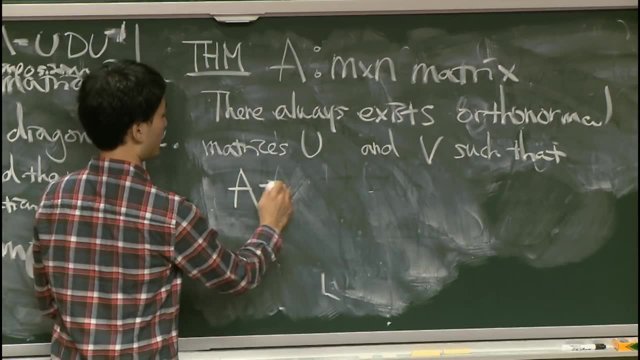 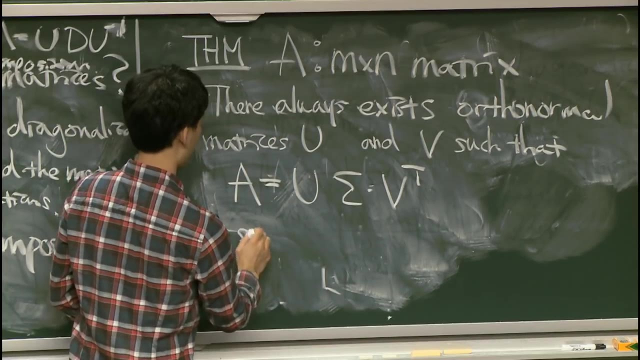 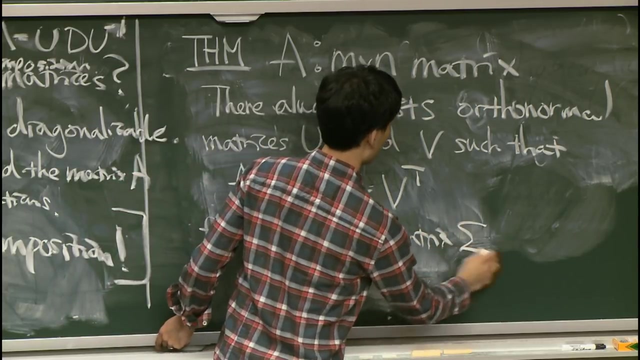 So we have u and v such that A is equal to u times sigma times v. transpose for some diagonal matrix sigma. Let me parse through the theorem a little bit more. Whenever you have a matrix that's diagonalizable. whenever you're given a matrix, it. 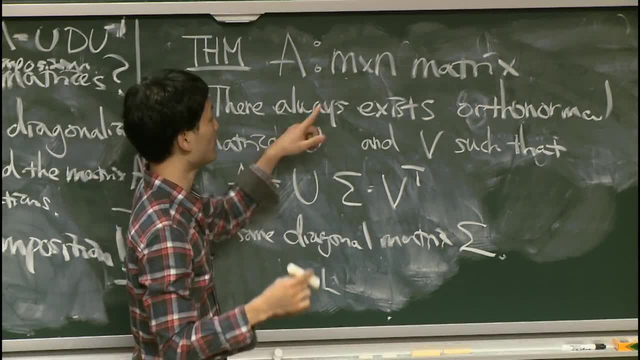 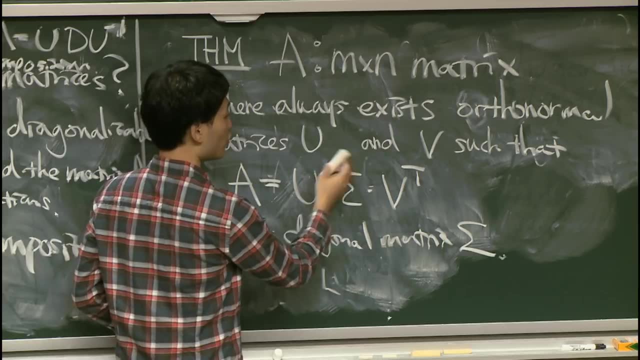 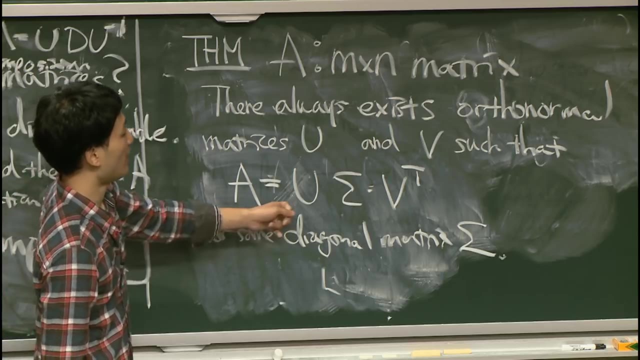 doesn't even have to be a square matrix anymore, It can be non-symmetric. So whenever you're given an m by n matrix, in general there always exists two matrices, u and v, which are orthonormal, such that A can be decomposed as u times sigma times v transpose. 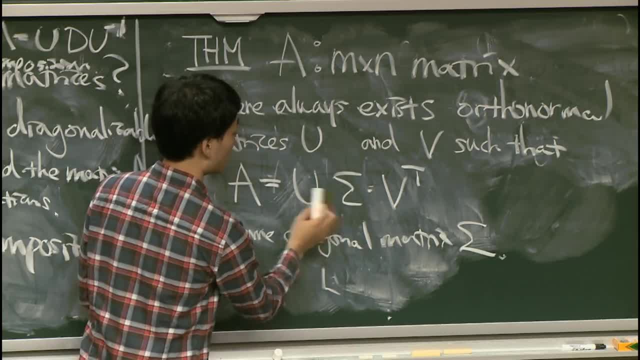 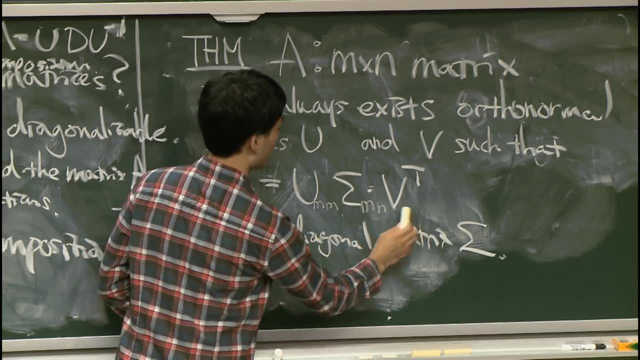 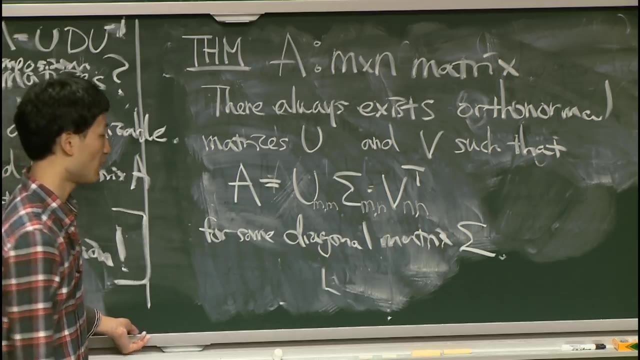 where sigma is a diagonal matrix. But now the size of the matrices are important. So u is an m by n matrix, Sigma is an m by n matrix And v is an n by n matrix. That just denotes the size, dimensions of the matrix. 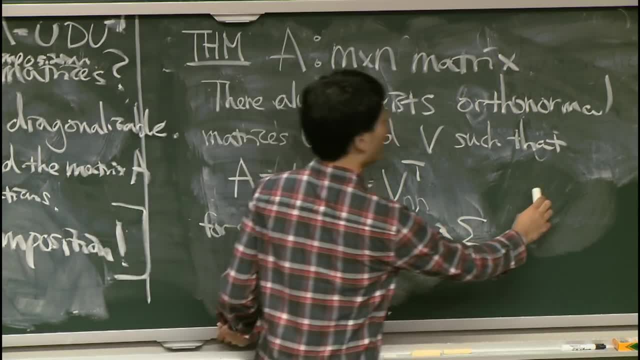 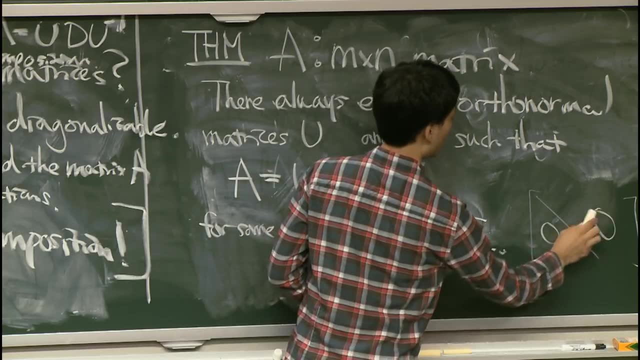 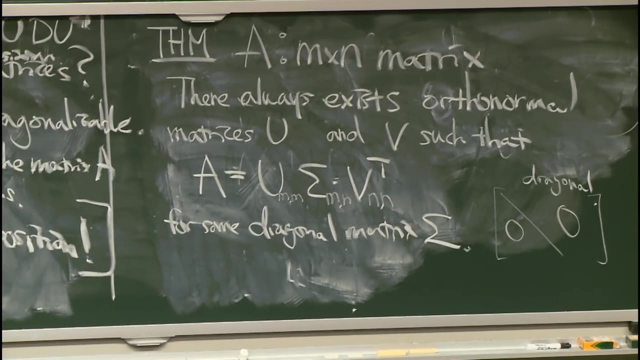 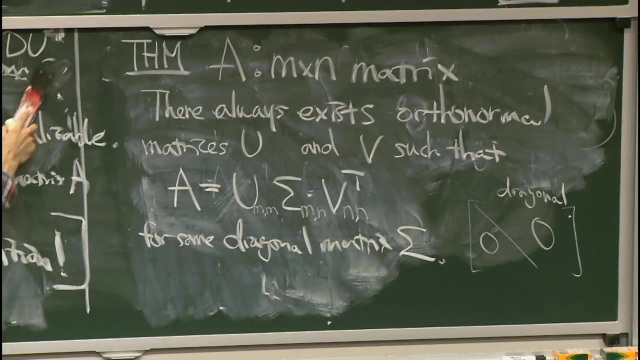 So what does it mean for an m by n matrix to be diagonal? It just means the same thing. So only the ii entries are allowed to be non-zero. So that was just a bunch of words. So let me write this: Eigenvalue decomposition. we'll do that part later. 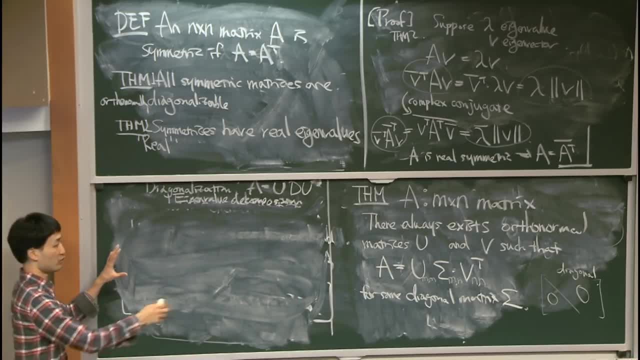 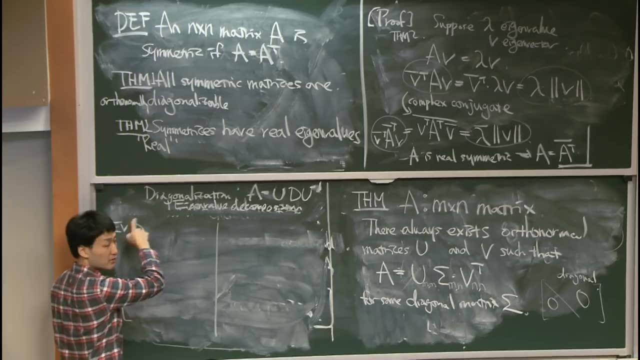 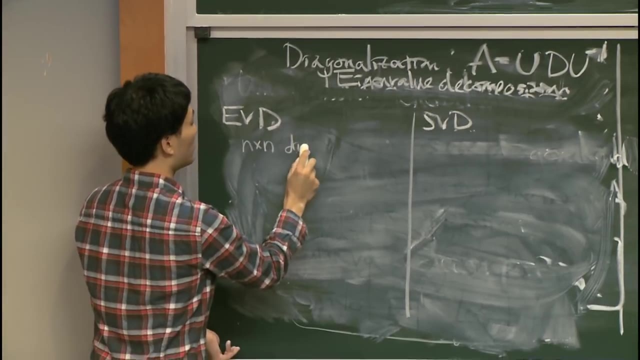 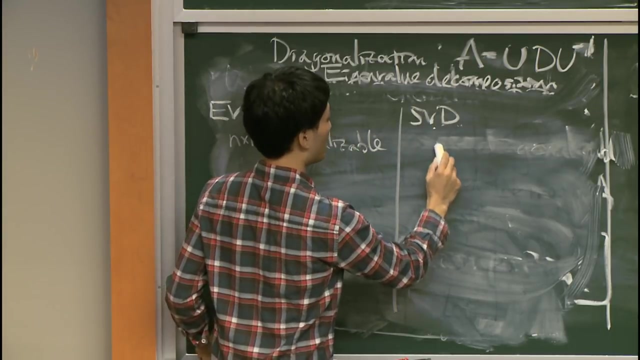 OK, So let me compare now eigenvalue decomposition with singular value decomposition. So this is EVD. what we just saw before, It's only SVD. This only works for m by n matrices which are diagonalizable. SVD works for all general m by n matrices. 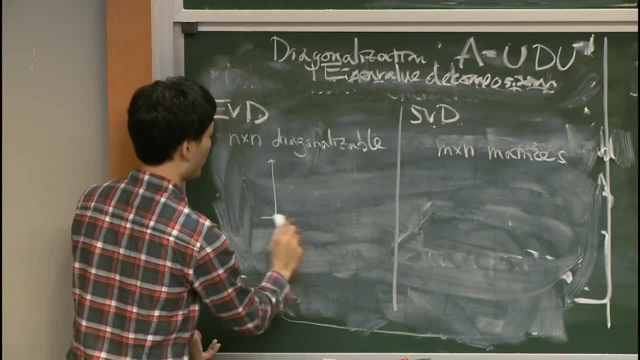 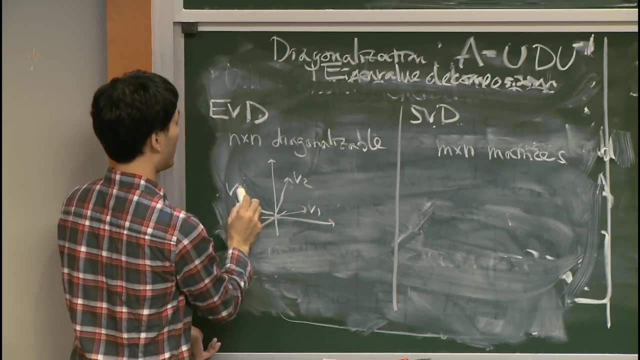 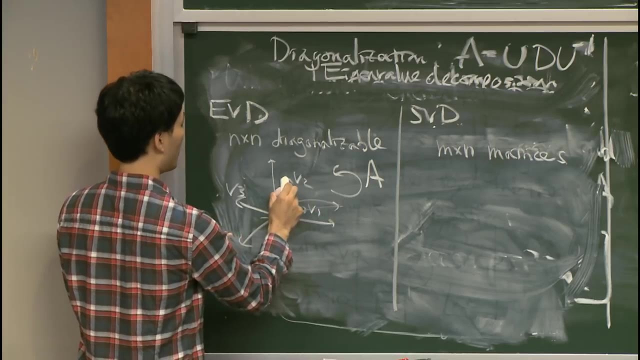 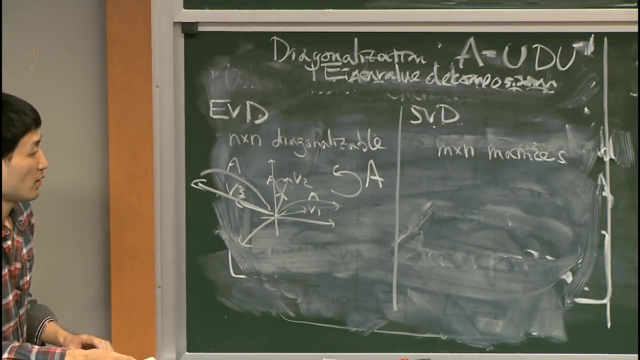 However, this is powerful because it gives you one frame, so v1,, v2,, v3, for which A acts as a scaling operator. OK, So this is just one frame. So v2., v3., v3. And, like that, A. that's what A does. A does, A does OK. 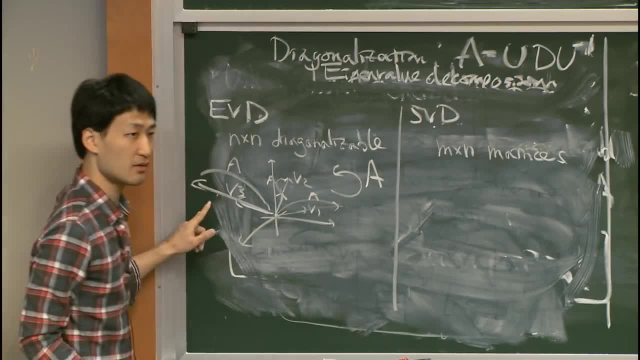 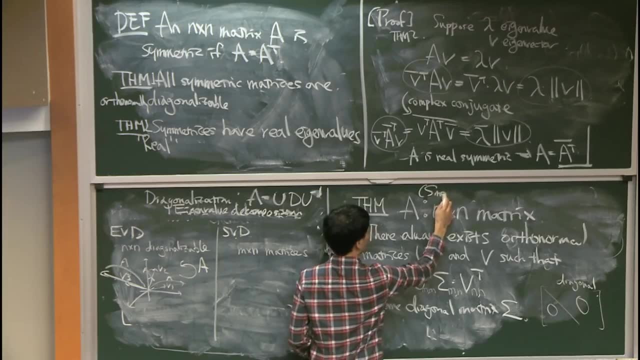 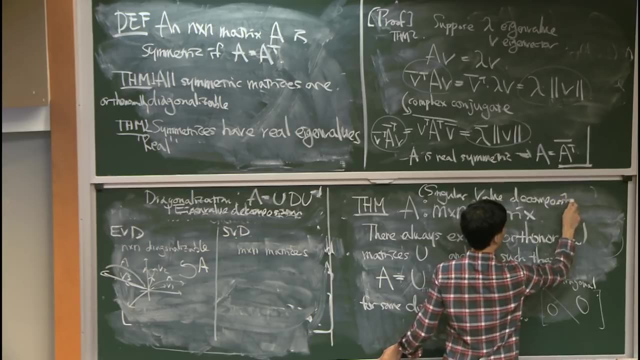 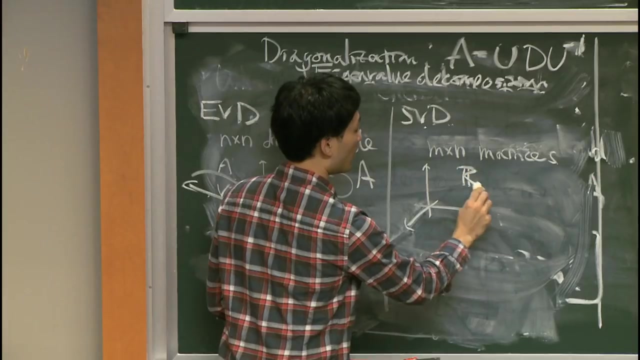 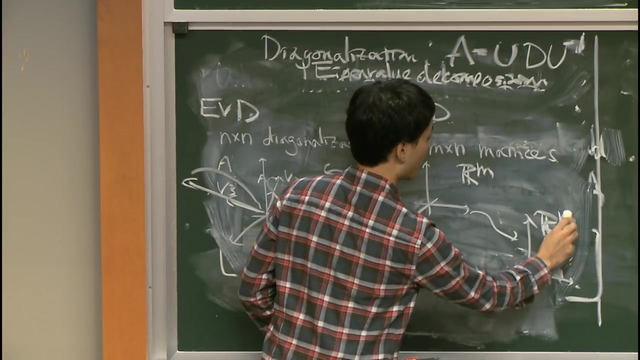 That's because these U on the both sides are equal. However, for singular value decomposition, this is called singular value decomposition. I just erased it. What you have instead is, first of all, the spaces are different. You take a vector in r to the m and bring it to r to the n. 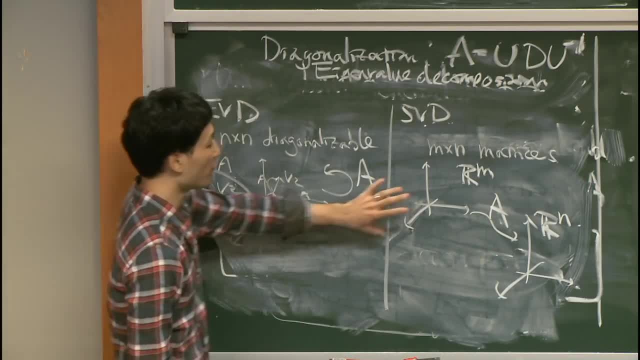 by this operation A. What's going to happen here is there will be one frame in here and one frame in here, So there will be vectors v1, v2, v3, v4,, v5,, v6,, v7,, v8,, v9,. v10, v11, v12, v13, v14, v15, v16, v19, v20,, v21, v22, v23, v23,, v24, v26,, v27, v28, v29, v30, v31, v32, v33, v33, v34, v35, v36, v37, v38, v39,, v40,, v44,, v41, v42, v43, v44, v45, v46, v48, v49, v49,, v50,, v50,, v50,, v50, v50. 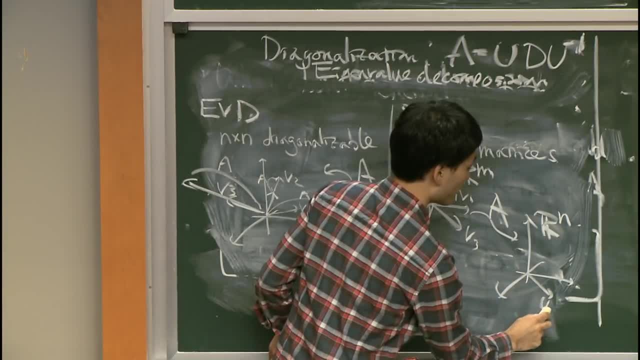 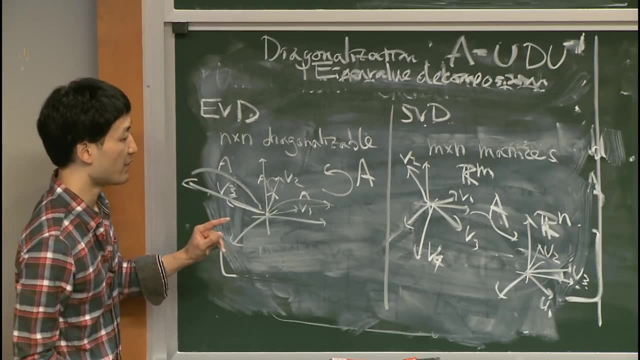 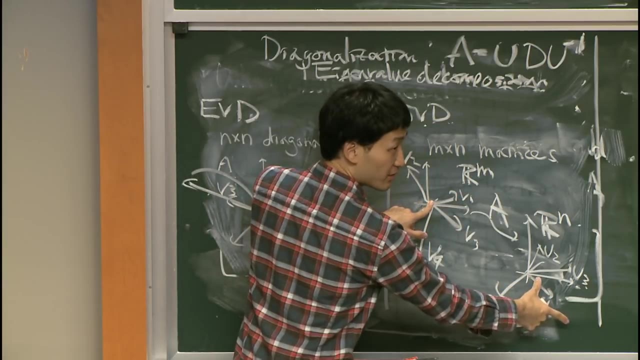 v4, like this, And there will be vectors u1, u2, u3, like this here, And what's going to happen is when you take v1, A will take v1 to u1 and scale it a little bit according to that diagonal. 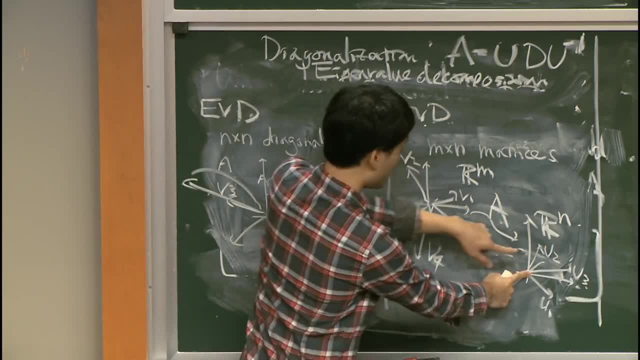 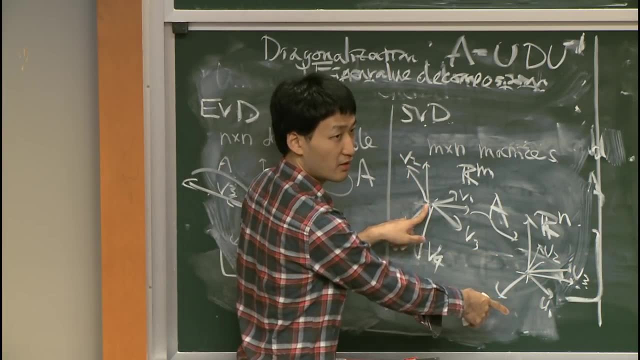 A will take v2 to u2, we'll scale it. A will take v3 to u3, scale it. Wait a minute, but for v4, we don't have v4. What's going to happen is this is just going to disappear. 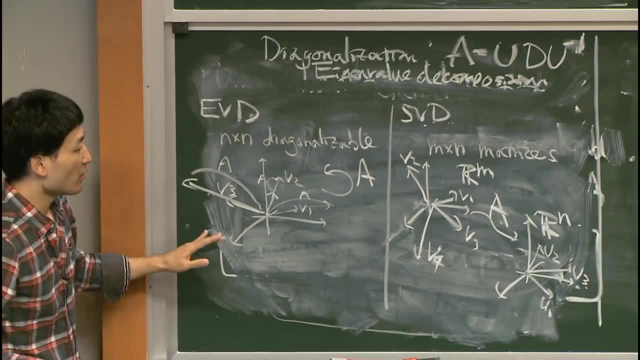 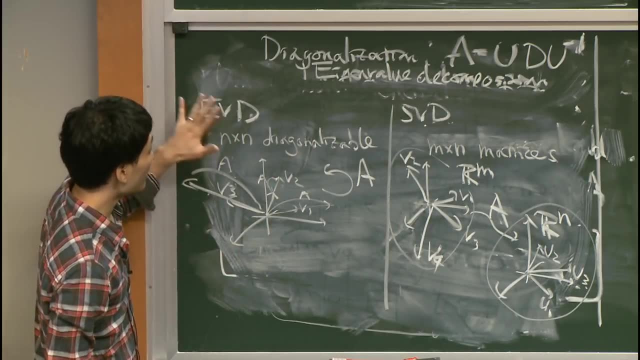 v4,, when applied, A will disappear. So I know it's a very vague explanation, but this geometric picture- try to compare them. A diagonalization, eigenvalue decomposition works within its frame, So it's very, very powerful. 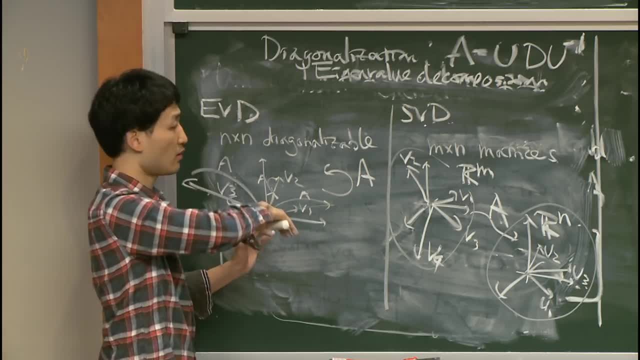 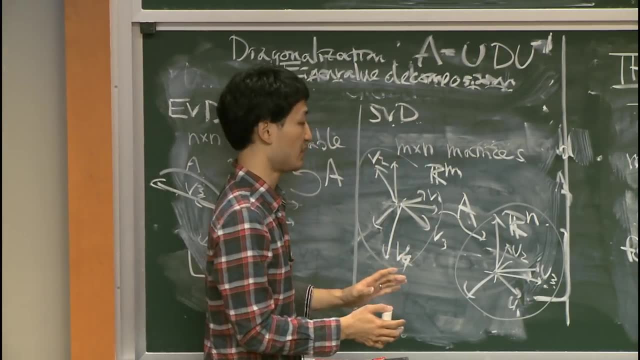 You just have some directions and you scale those directions. But the singular value decomposition. it's applicable to more general class of matrices but it's rather more restricted. You have two frames, one for the original space, one for the target space. 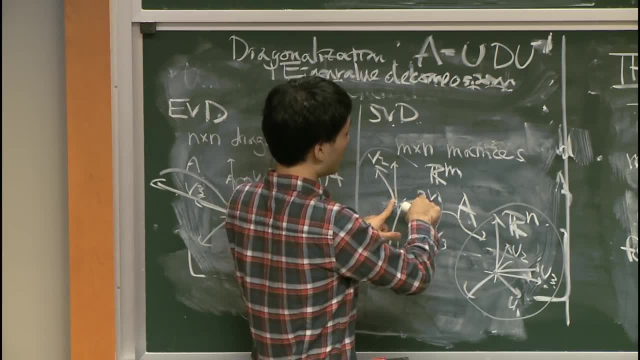 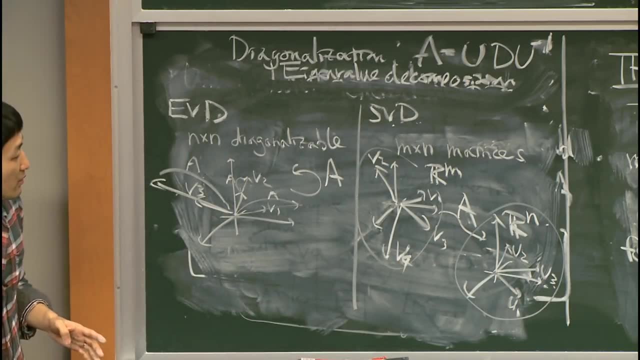 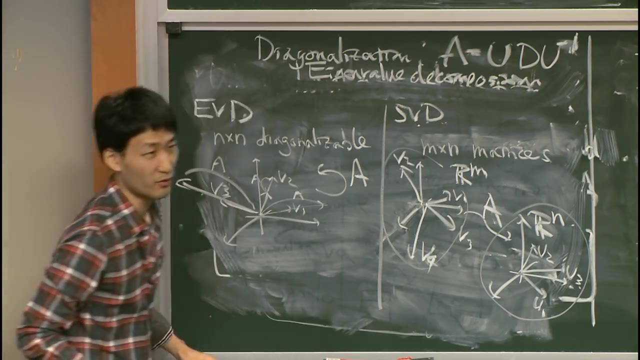 And what the linear transformation does is it just sends one vector to another vector and scale it a little bit. OK, So now there's another good example, OK, OK. So this is a good time to go back to that matrix in the very beginning. 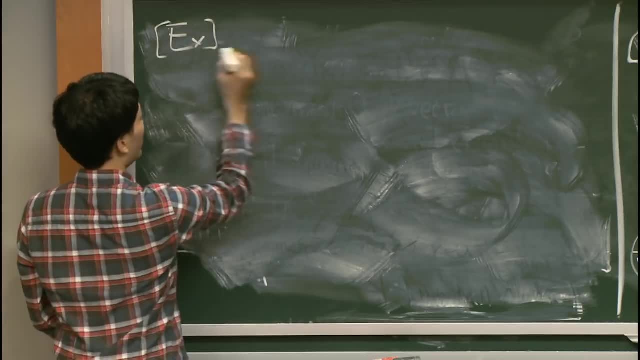 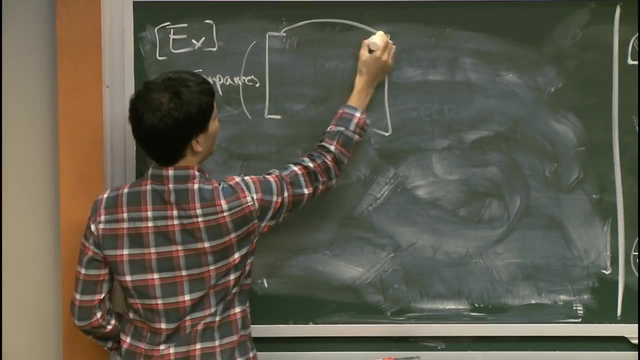 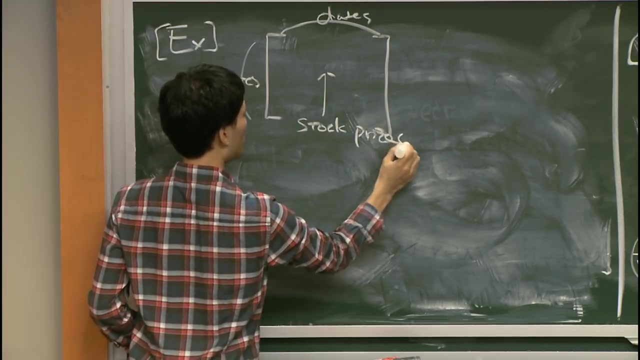 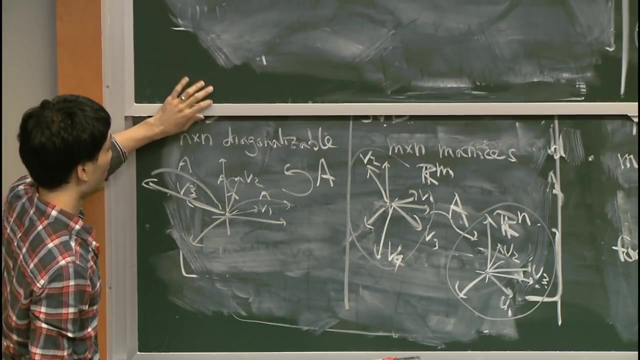 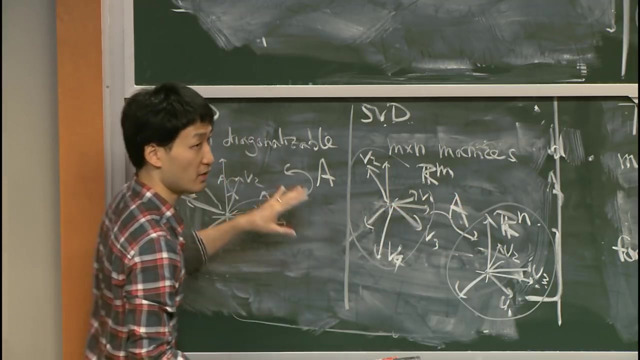 So remember that example where you had a vector of companies and dates and the entry was stock prices. OK, So if it's a n by n matrix, you can try to apply both eigenvalue decomposition and singular value decomposition, But what will be more sensible is singular value. 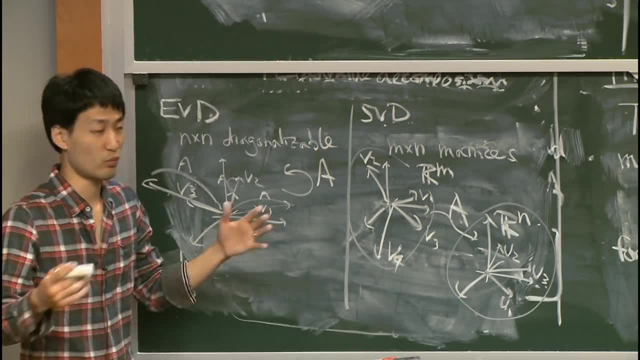 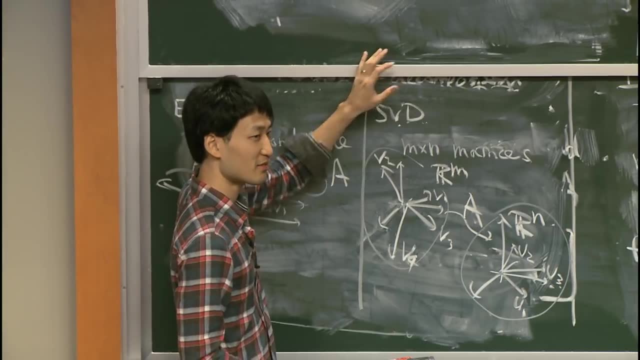 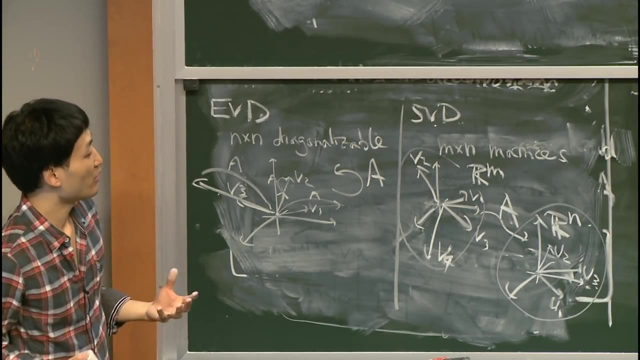 decomposition in this case. I won't explain why and what's happening here. Peter will probably. yeah, You will come to it later, But just try to do some imagining before listening what's really happening in real world. So try to use your own imagination, your own language. 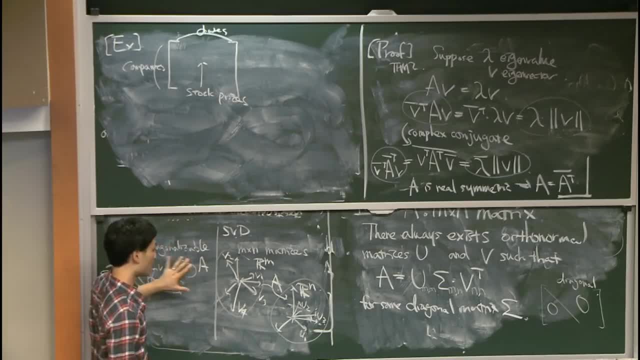 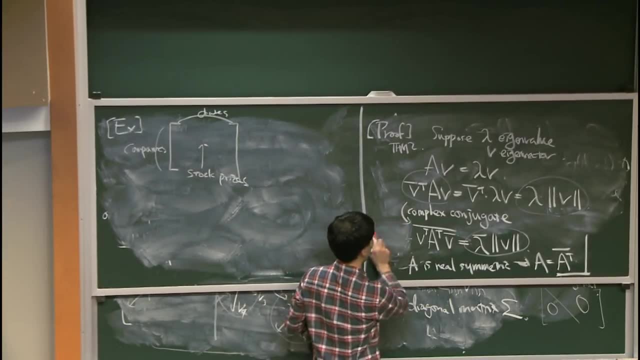 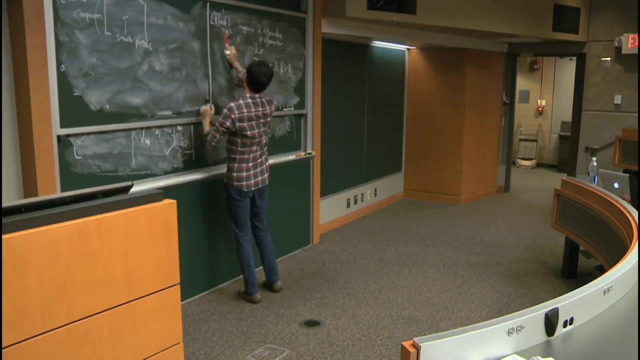 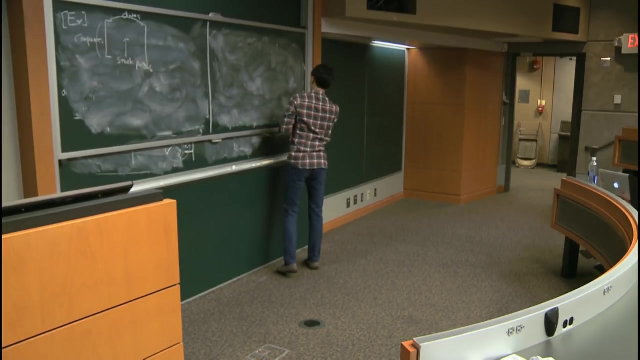 to express. see what happens for this matrix. what this decomposition is doing Just looks like totally nonsense. Why does this have even a geometry? Why does it define a linear transformation, And so on? It's just a beautiful theory which gives many useful information. 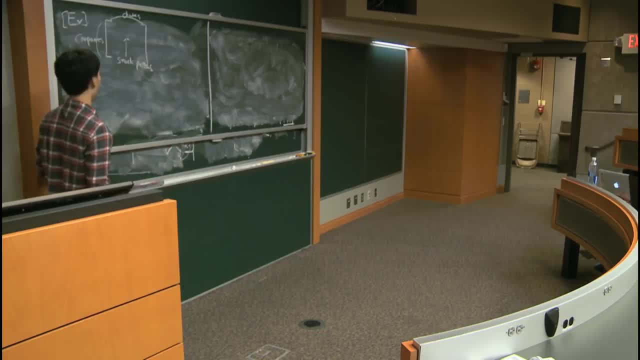 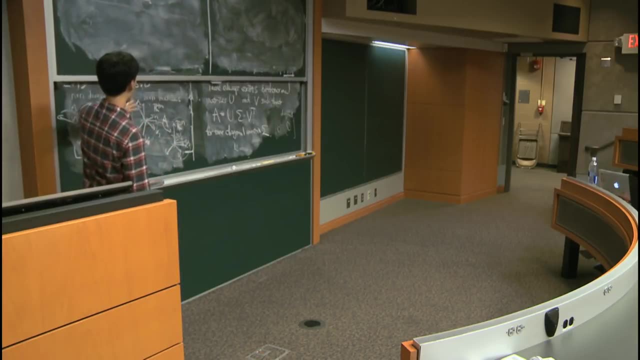 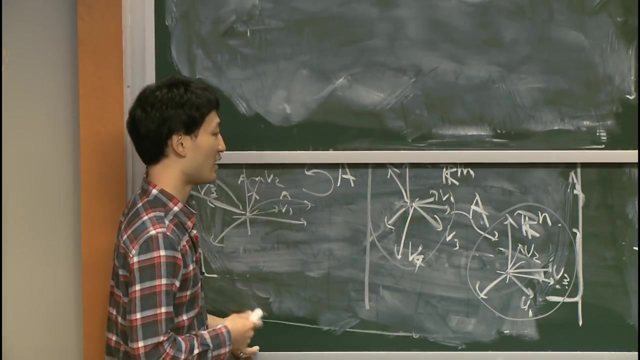 I can't really emphasize more because emphasize enough, because really this is just universal, being used in all science, these eigenvalue decomposition and singular value decomposition, Not just for this course but pretty much, it's safe to say, in every engineering. 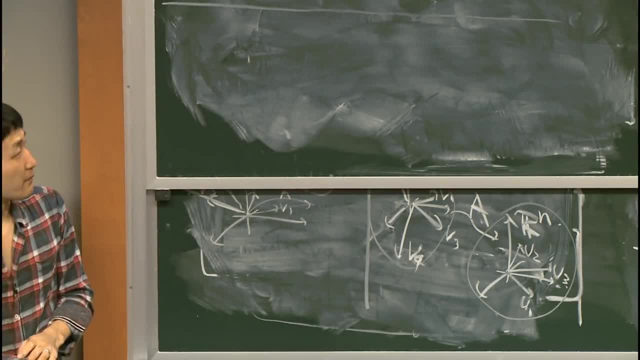 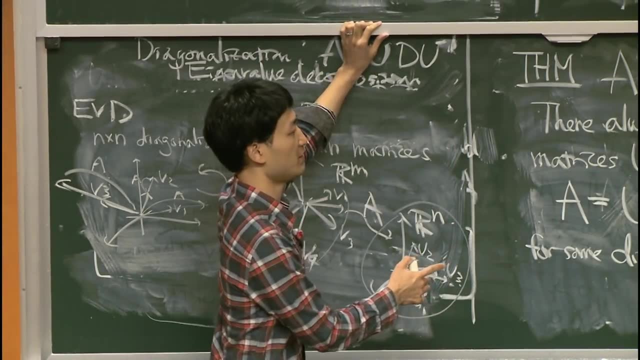 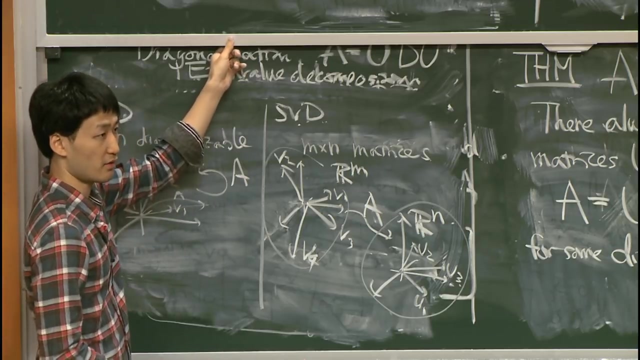 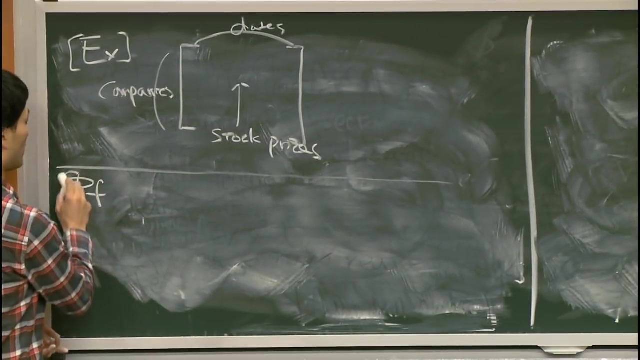 you'll encounter one of the forms. OK, So let me talk about the proof of the singular value decomposition And I will show you an example of what singular value decomposition does for some example matrix, the matrix that I chose. Proof of singular value decomposition. 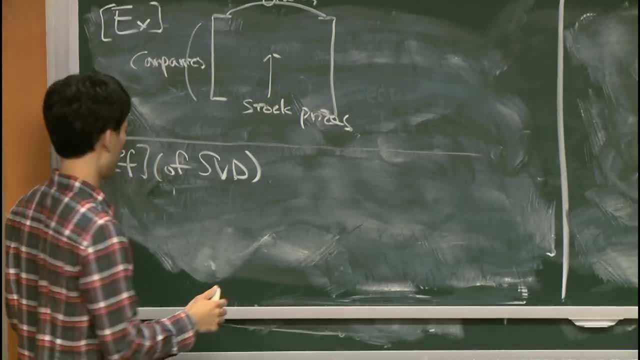 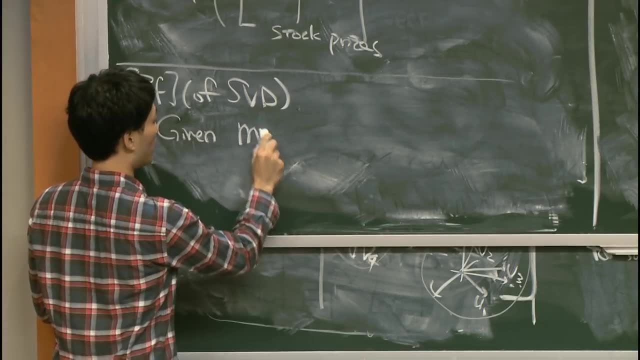 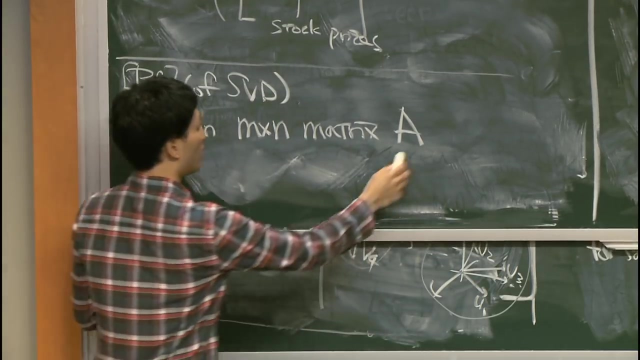 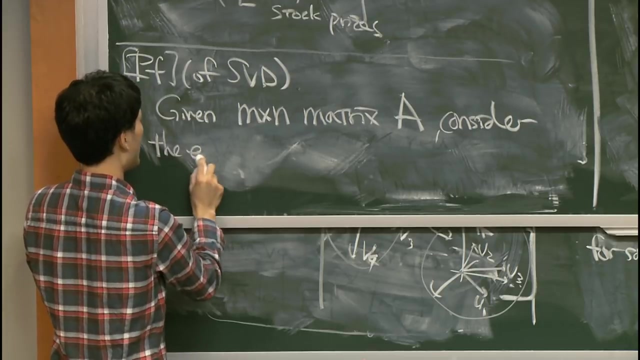 which is interesting. It relies on eigenvalue decomposition. So, given a matrix A, consider the eigenvalues of A times A, which is the most common matrix. What's it going to be? So I'm going to call that A times A, times A. 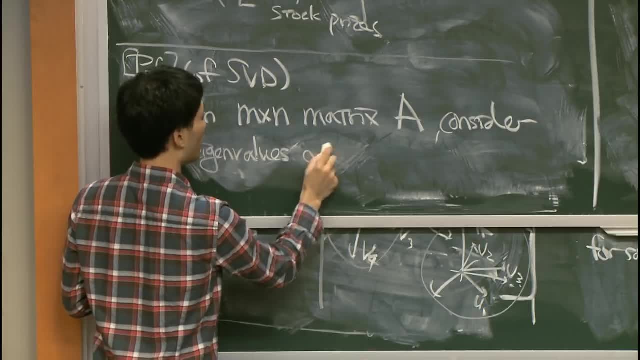 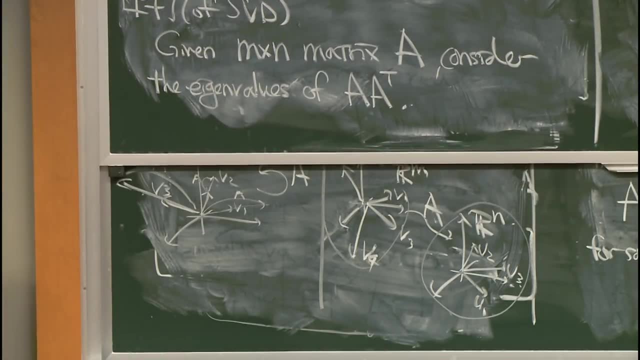 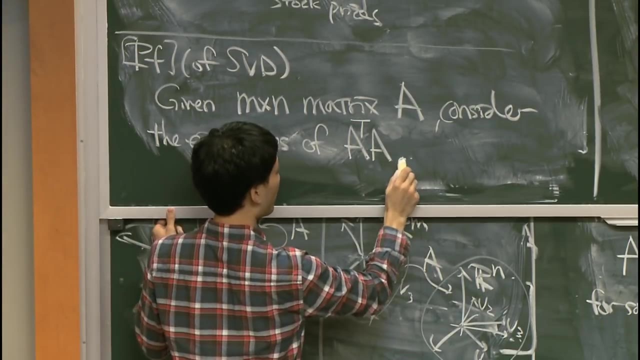 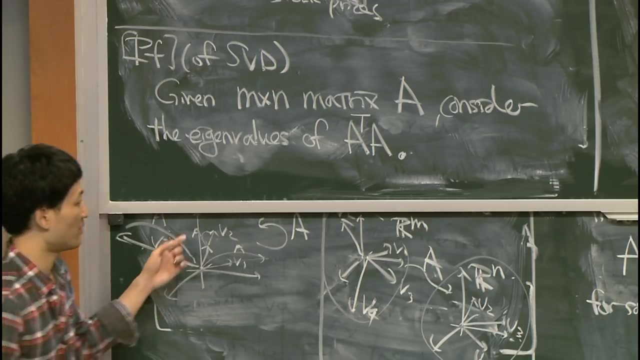 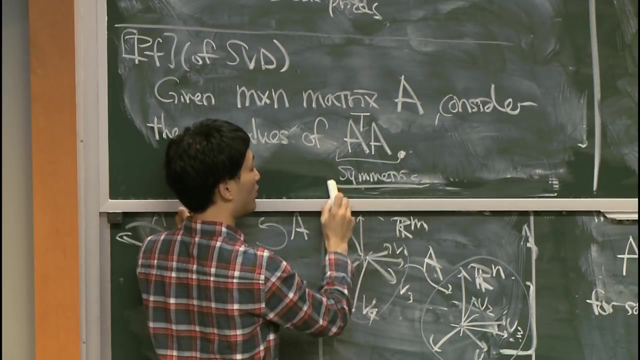 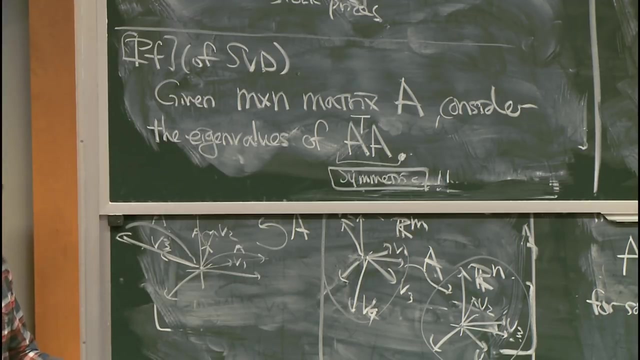 It's going to be A times B minus B, So in this translation A is the only radical which times A transpose A. First observation: That's a symmetric matrix, So, if you remember, it will have real eigenvalues and it's diagonalizable. 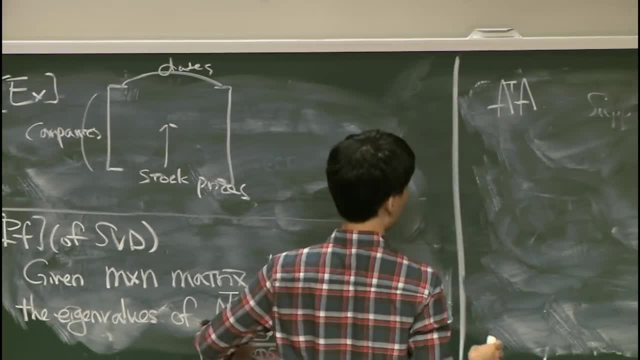 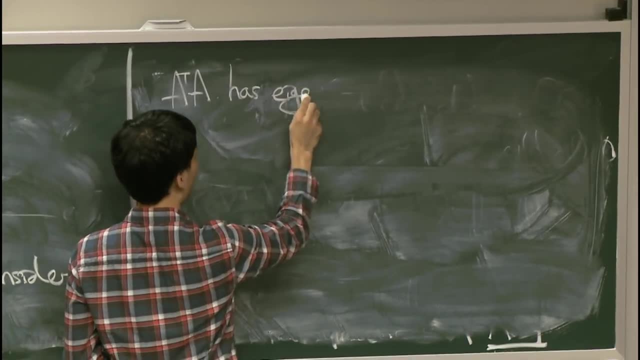 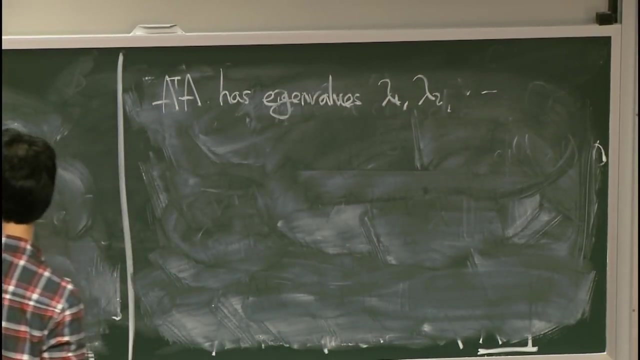 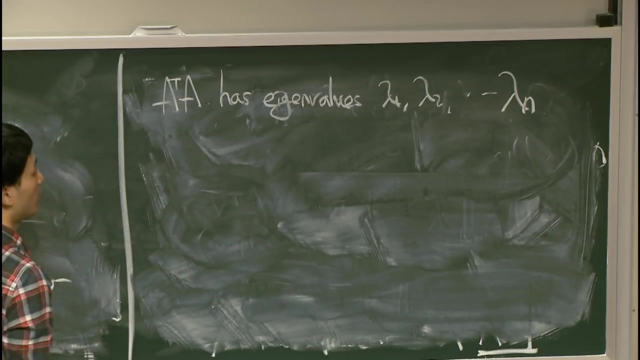 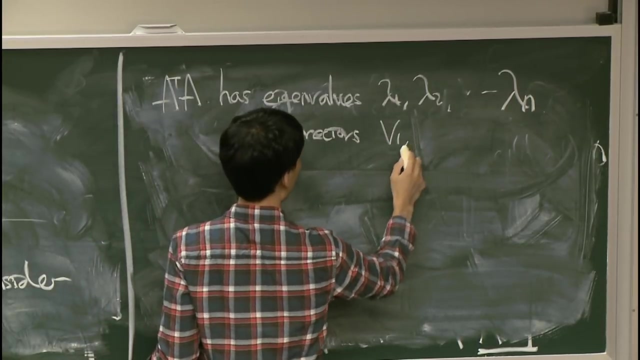 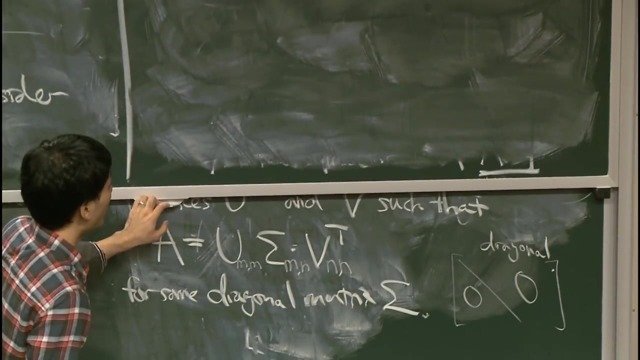 So A T of A has eigenvalues, So lambda 1, lambda 2, up to an m by n matrix, so lambda n And corresponding eigenvectors v1, v2, up to vn. And so, for convenience, I will cut it at lambda r. 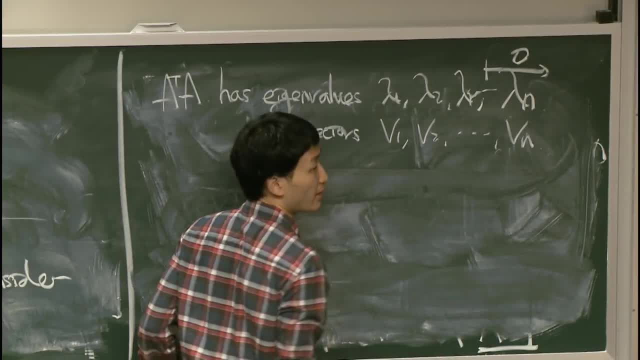 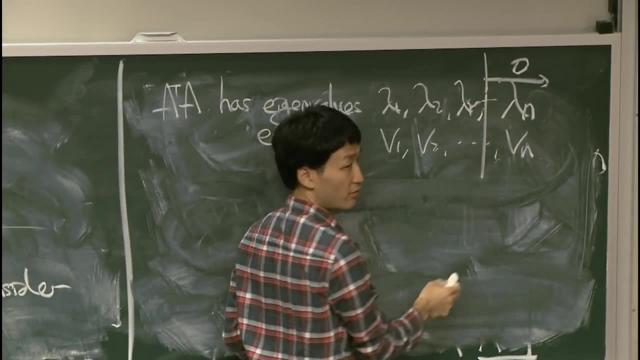 And assume all the rest is 0. So there might be none which are 0. In that case we use all the eigenvalues. But I only am interested in non-zero eigenvalues. So I will say up to lambda r: they're non-zero. 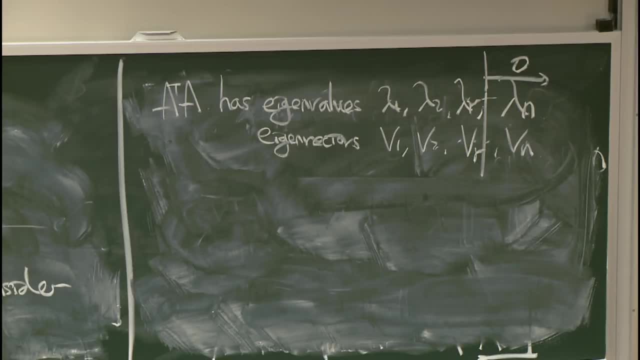 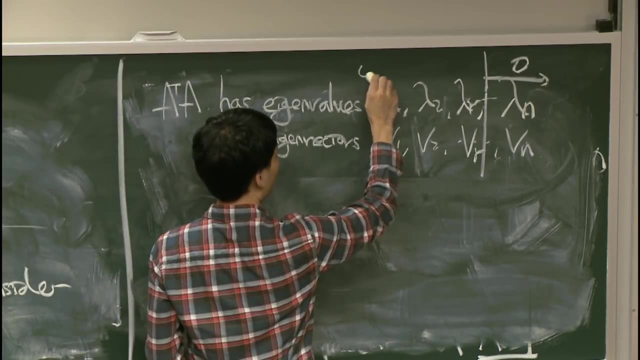 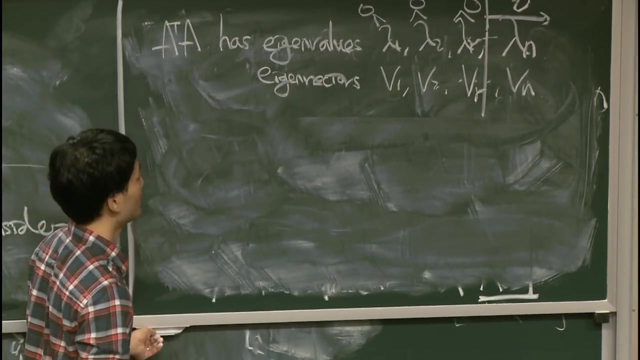 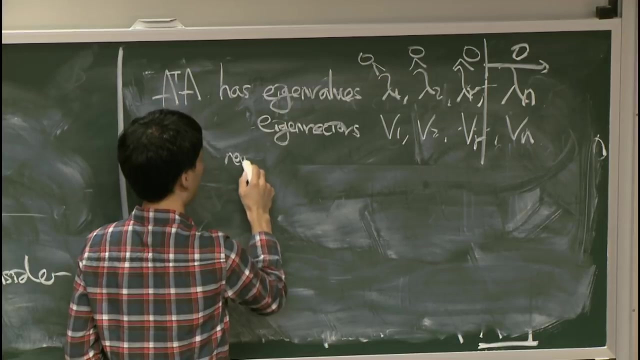 Afterwards 0.. It's just a notational choice, And now I'm just going to make a claim that they're all positive. This part is kind of just. Just believe me, Then, if that's the case, we can rewrite the eigenvalues. 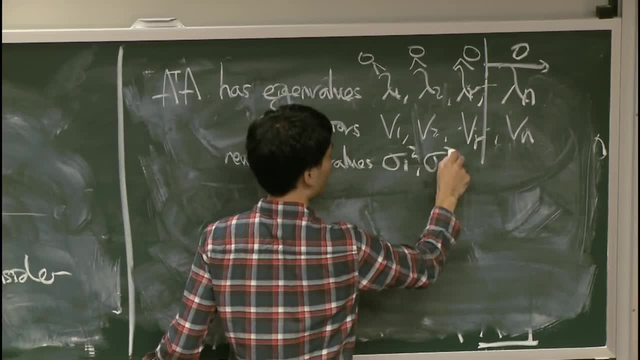 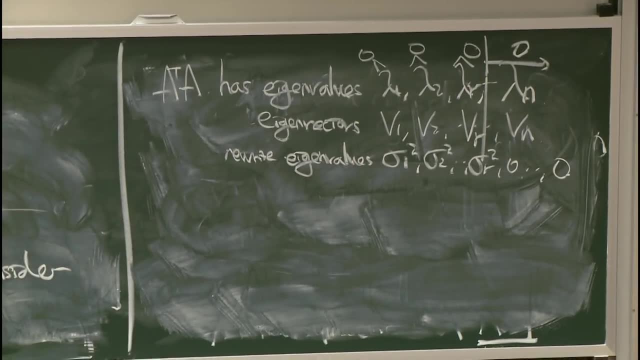 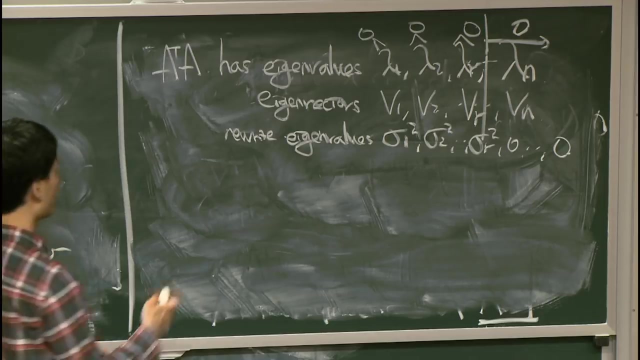 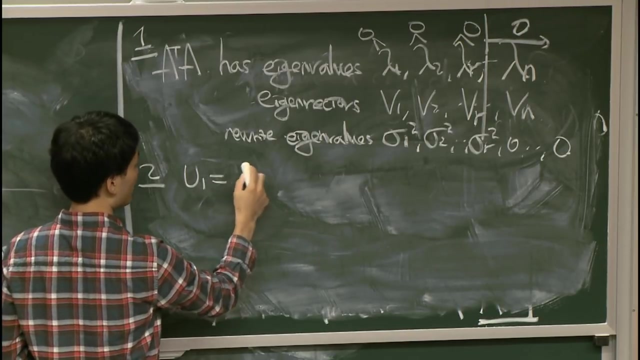 as sigma 1 square, sigma 2 square, sigma r square and 0.. OK, That was my first tip. My second step, that was step 1.. Step 2 is to define u of 1 as a times v1 over sigma 1,. 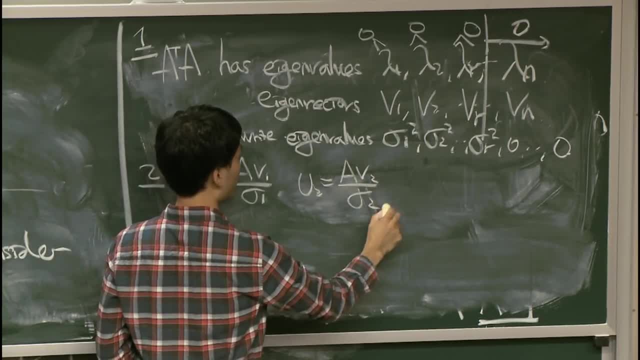 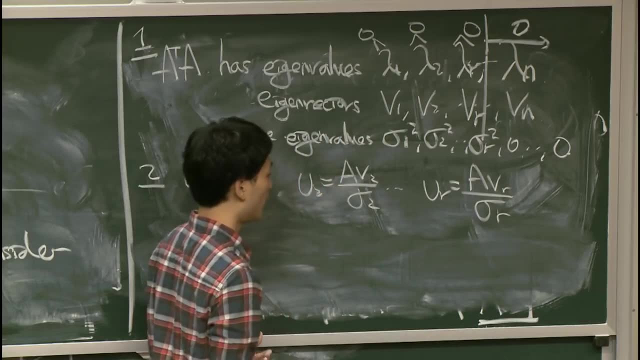 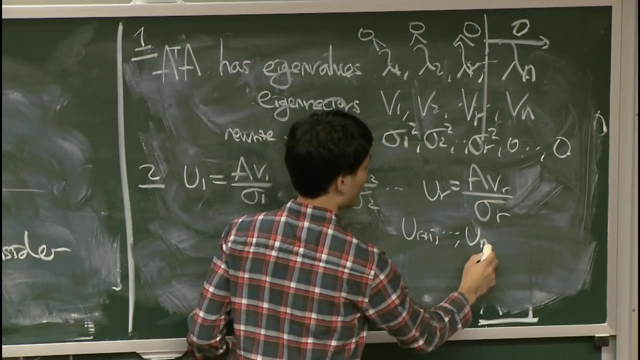 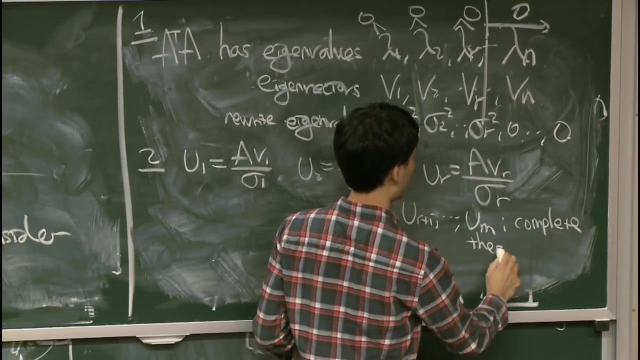 u of 2 as a times v2 over sigma 2, and u of r as a times v of r over sigma r, And then u times r plus 1 as up to u times v2.. And then u times m as complete the above into a basis. 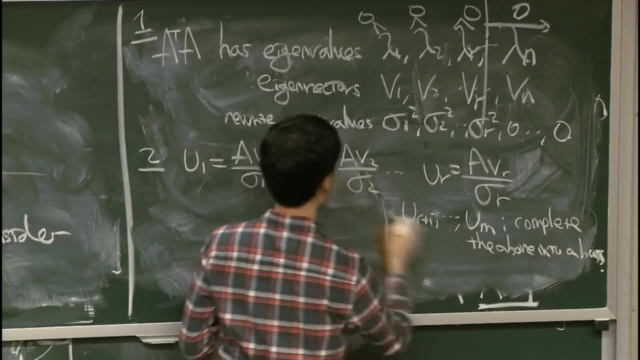 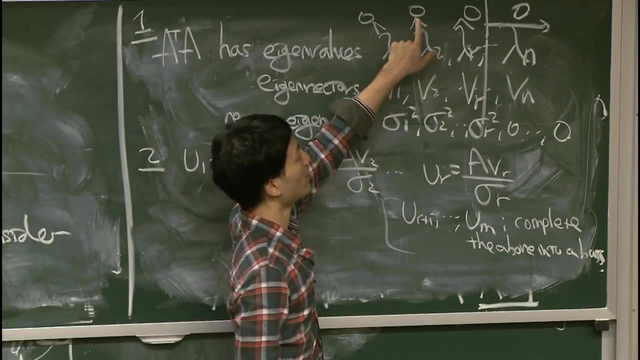 So for those who don't understand, just think of we pick u1 up to u r first and then arbitrarily pick the rest, And you'll see why I only care about the non-zero eigenvalues, because I have to divide by sigma. 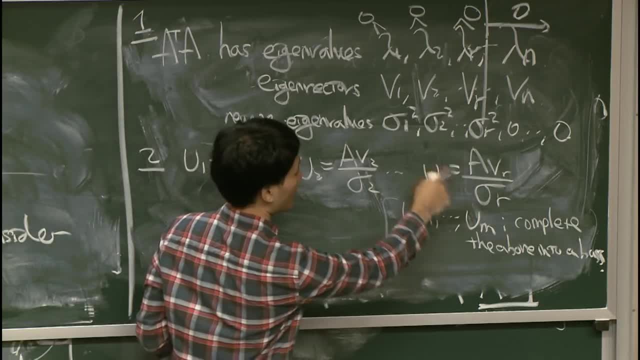 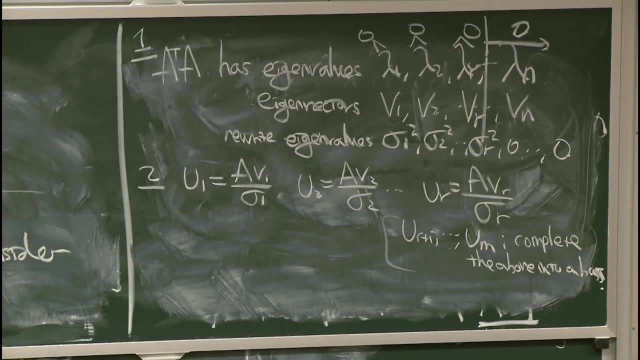 Sigma, Sigma, The sigma values, And if it's 0, I can't do the division. So that's why I identified those which are not 0. Then we're done. OK, So it doesn't look at all like we're done. 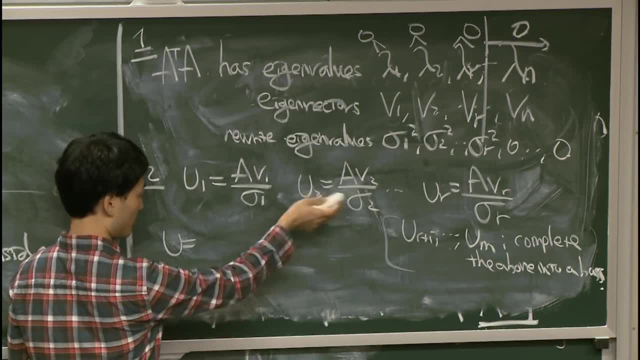 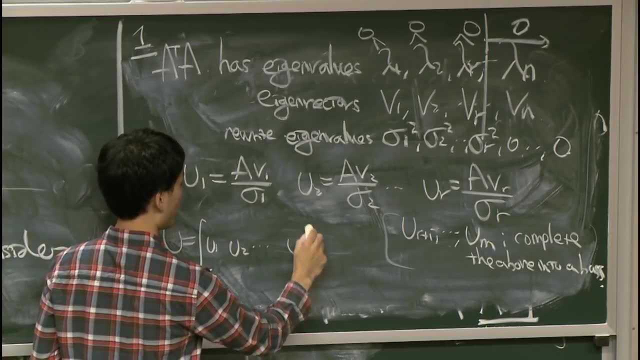 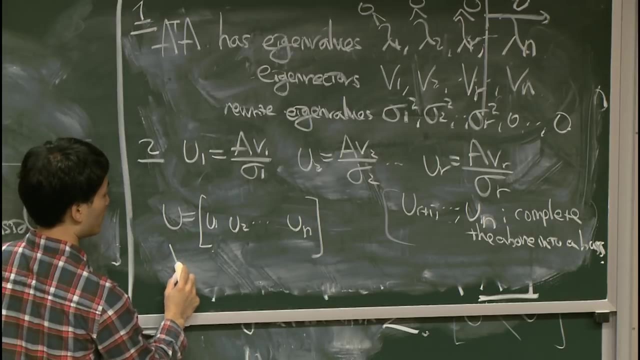 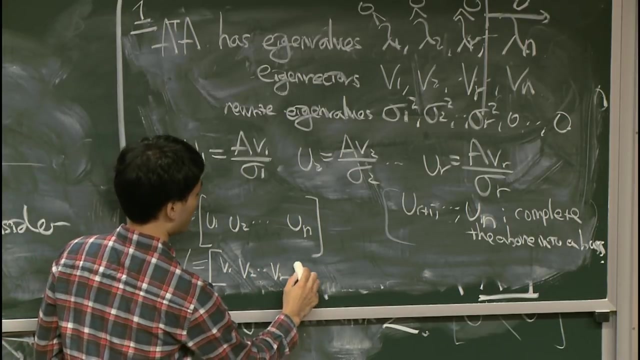 But I'm going to let my u be this: u1, u2, up to un. Sorry, that's dn My v. I'll pick as v1, v2, up to vr And then vr plus 1 up to vm. 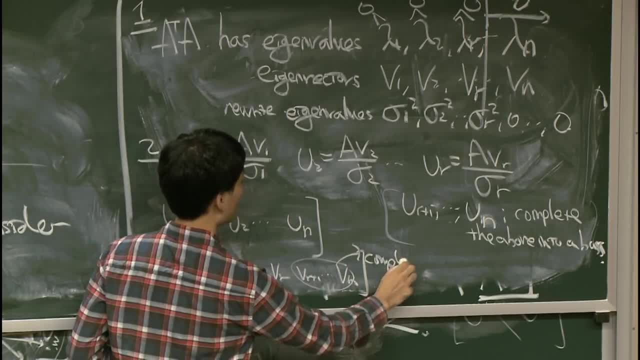 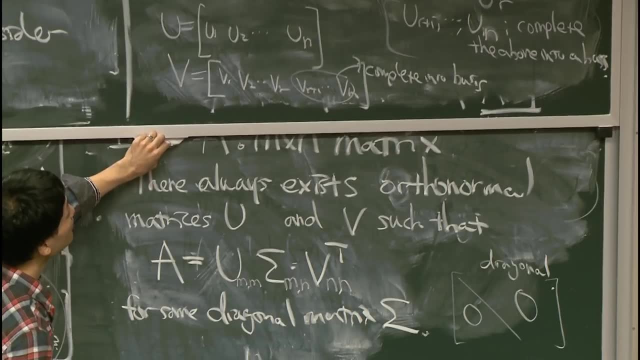 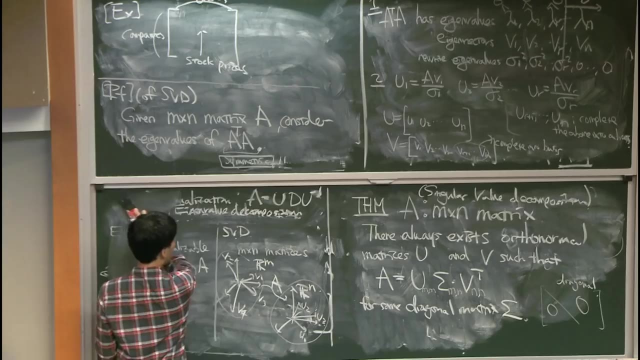 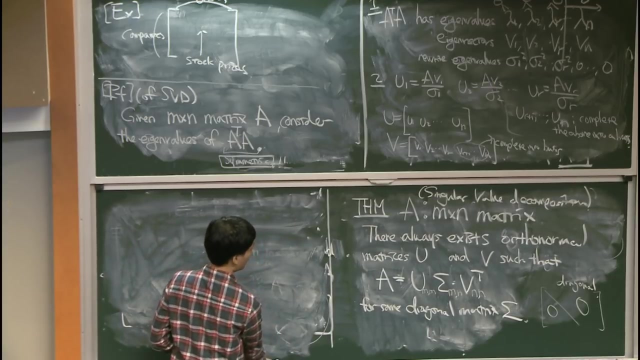 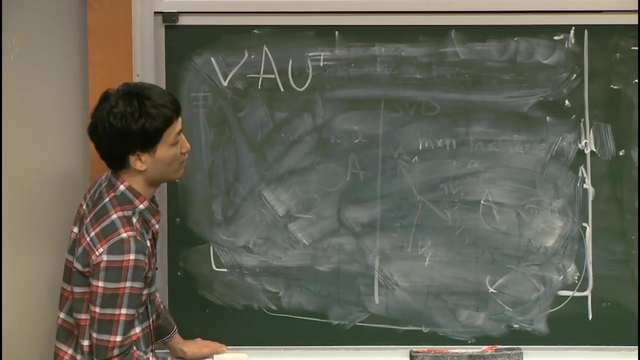 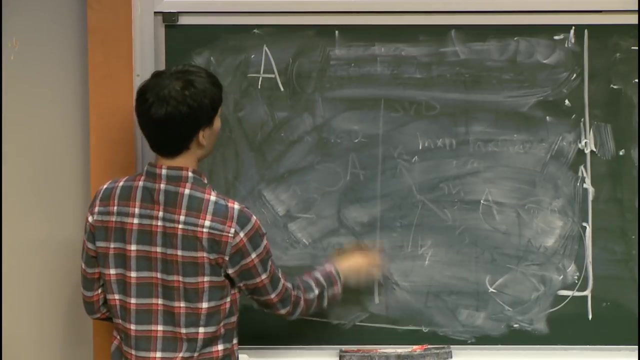 This again just complete into a basis. Now let's see what happens. OK, OK, So a times u transpose times v. Ah, that's why it looks wrong. I have to do u times a times v transpose. So I would write: v is. 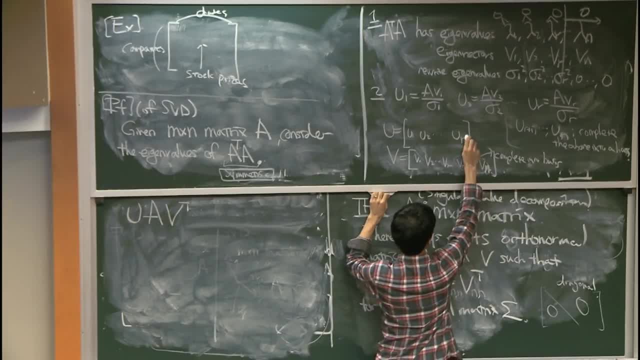 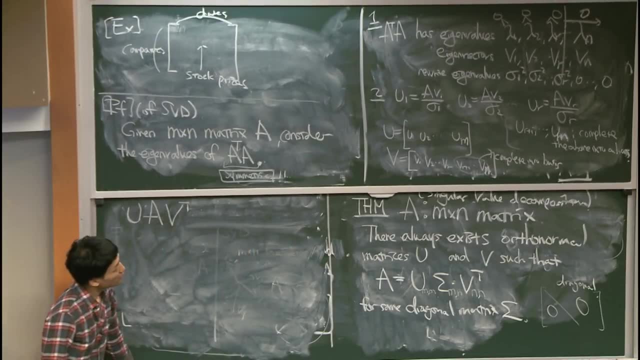 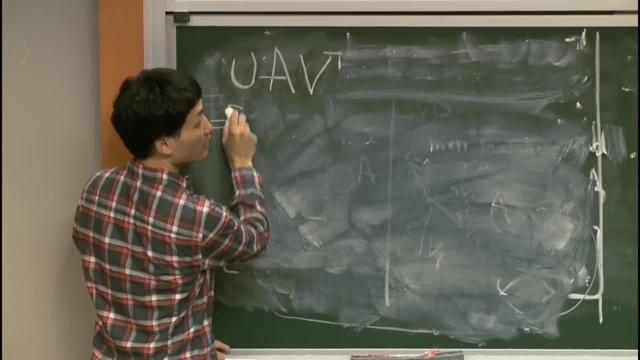 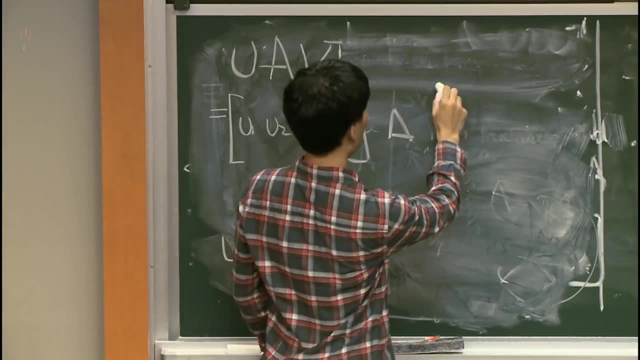 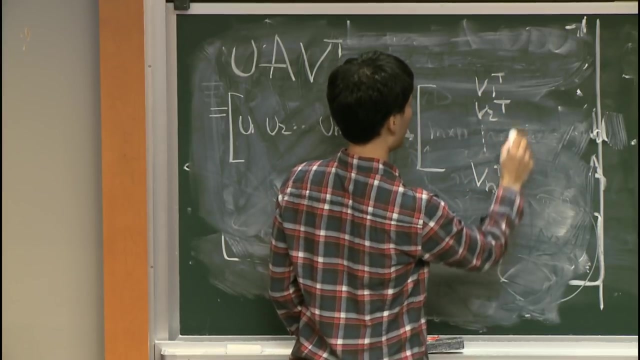 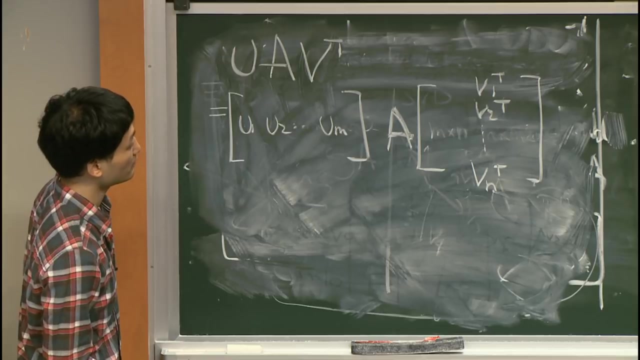 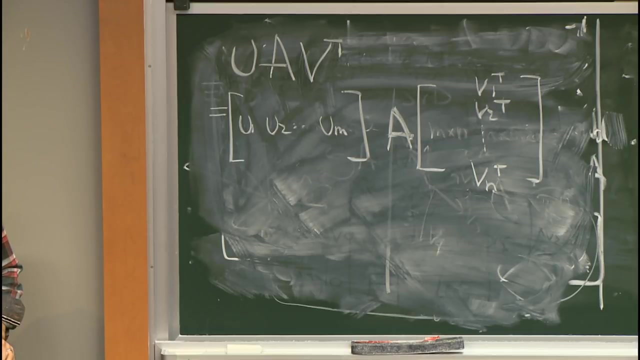 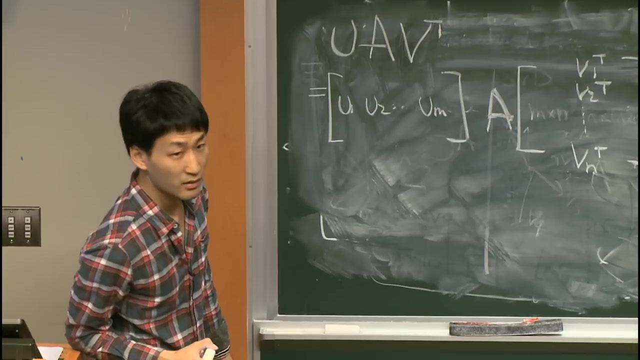 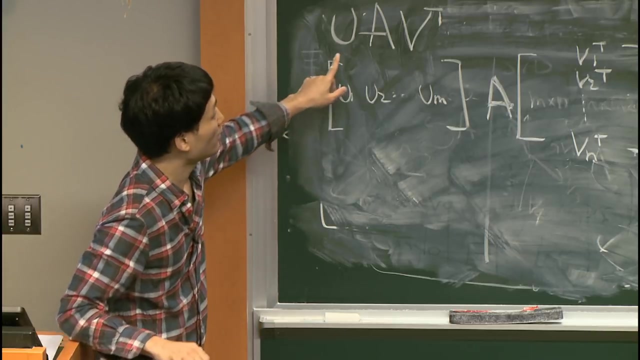 So u times A, times B transpose. yeah, That will be 1, u2, um A B transpose will be B1 transpose, B2 transpose, Bn transpose. All right, I messed up something, Sorry. Oh, that's the form I wanted. 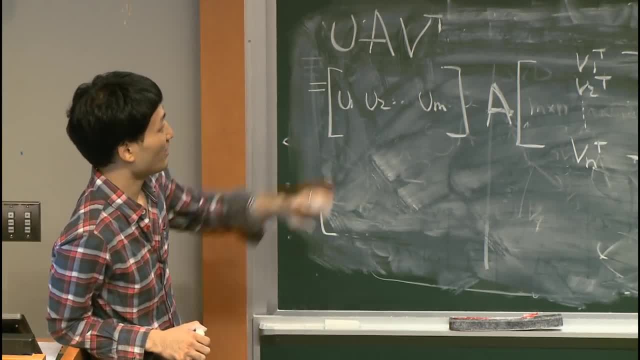 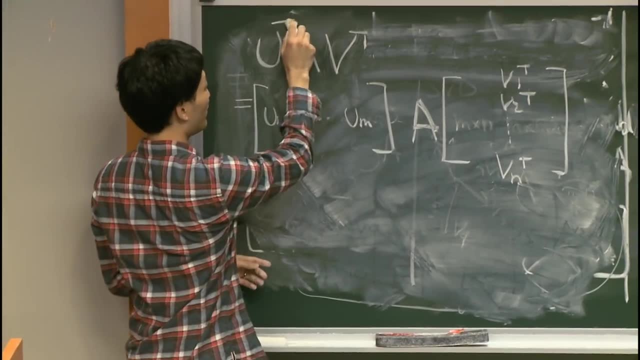 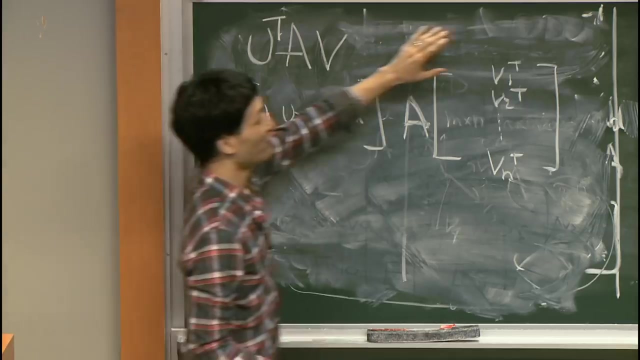 That's what I want, right? Yeah, So I have to transpose u and B there, OK, sorry, Oh, yeah, so thank you. Thank you for the correction. I know this looks different from that, but I mean, if you flip the definition, it will be the same. 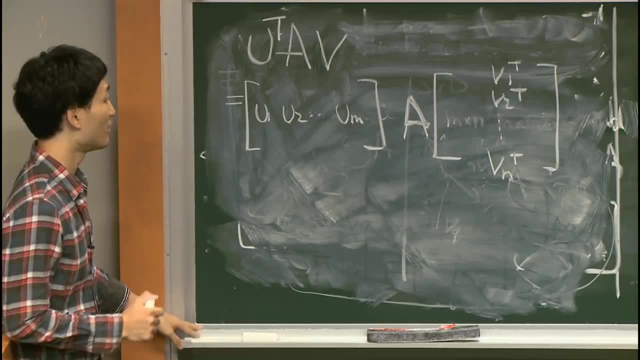 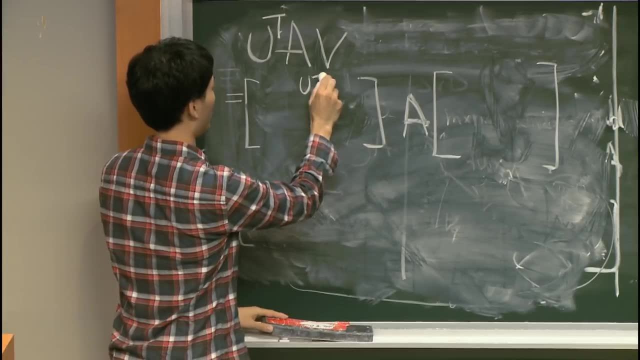 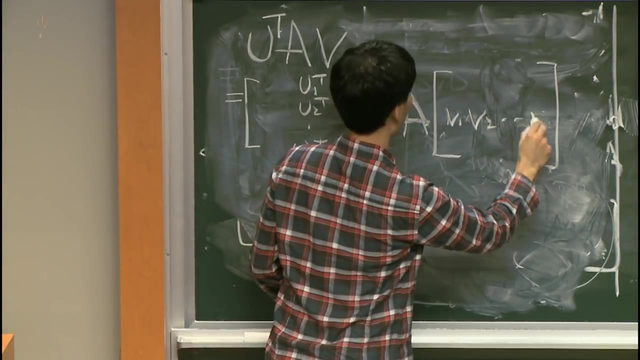 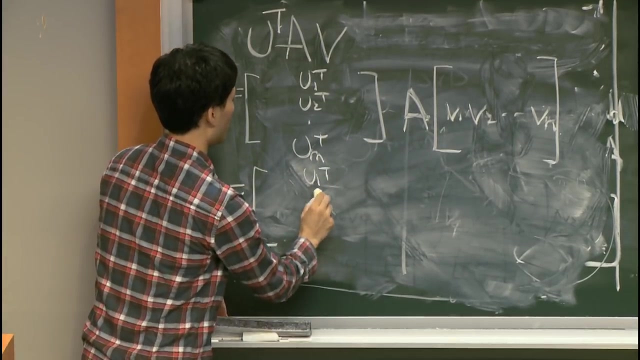 So I'll just not stop making mistakes here. Do you have a question? Yeah, So yeah, thank you. Yeah, that that will make more sense. OK, thank you very much. And then you're going to have u1 transpose up to um transpose. 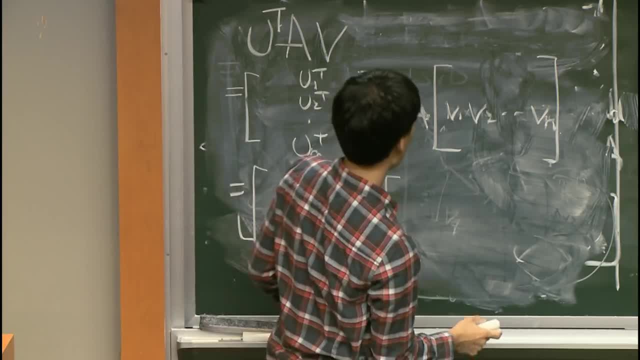 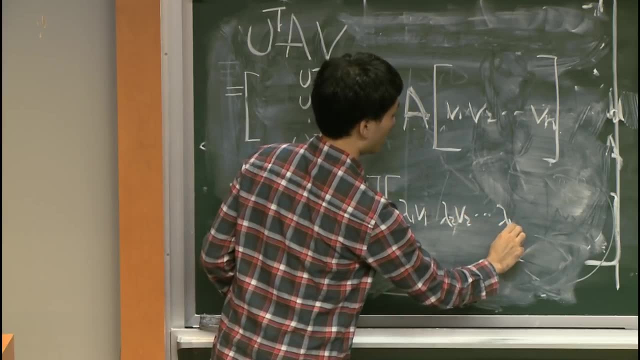 A times B, because of the definition of B, will be lambda 1 of B1.. A times B2 will be lambda 2 of B2 up to lambda r of Vr, And the rest will be 0.. And the rest will be 0. 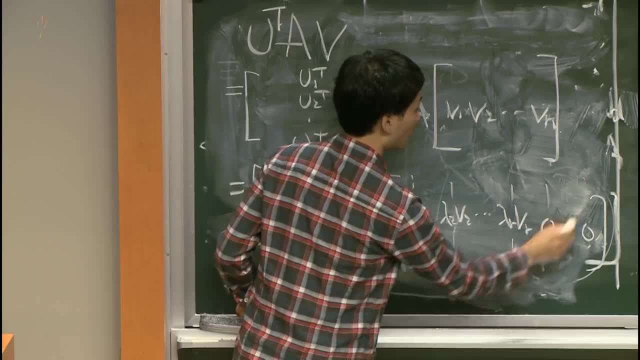 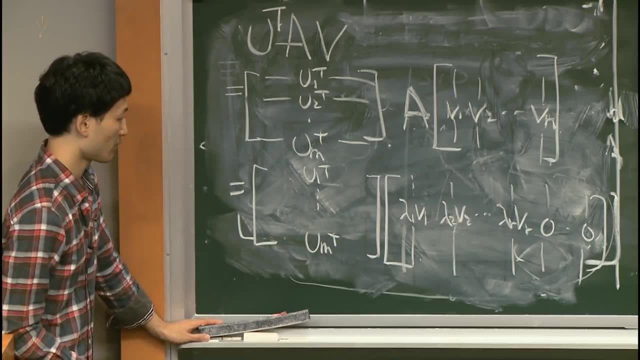 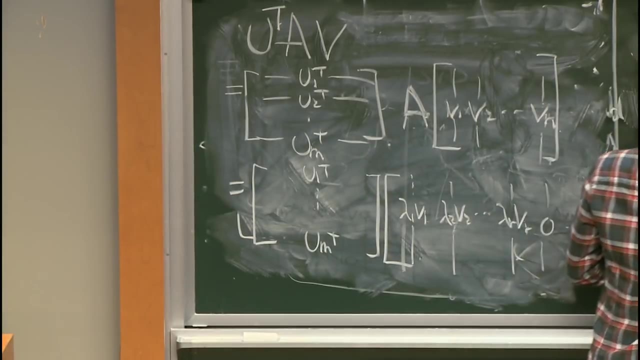 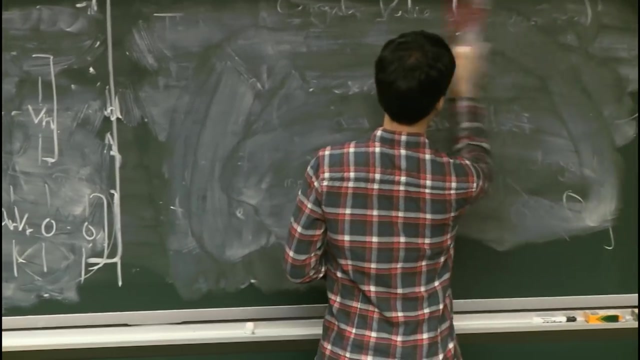 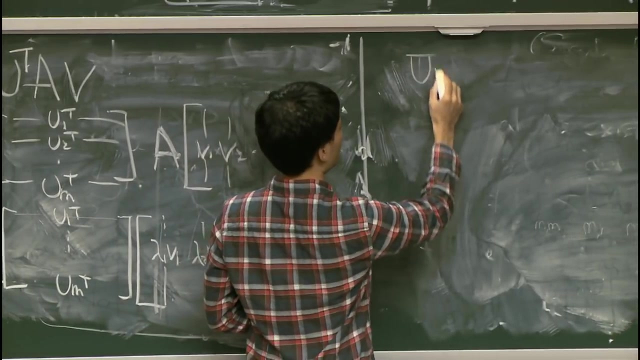 These all define the columns. OK, now let's do a few computations. OK, So u1 t times lambda 1 B1.. u1 t and lambda 1 B1.. When you take the dot product, what you're going to get? 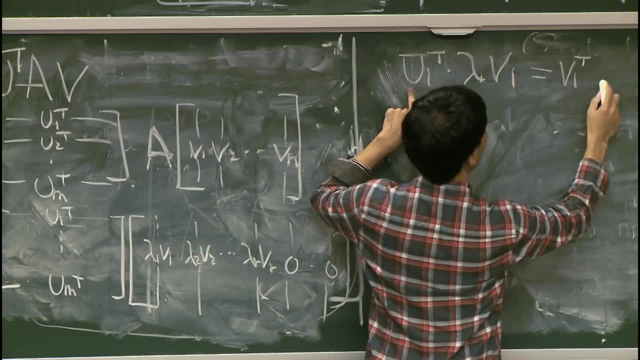 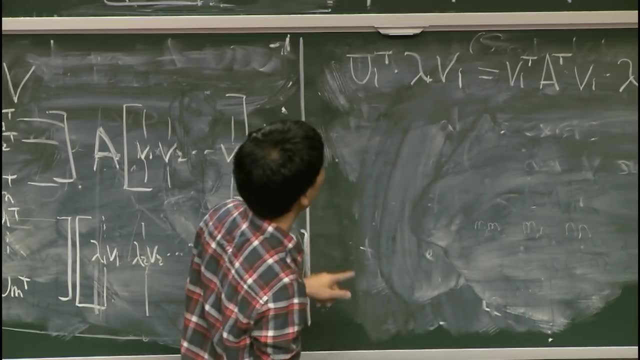 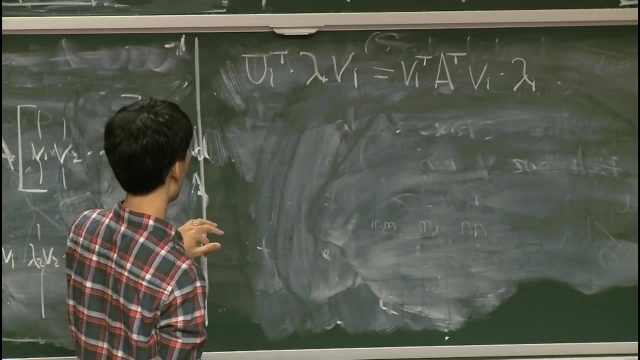 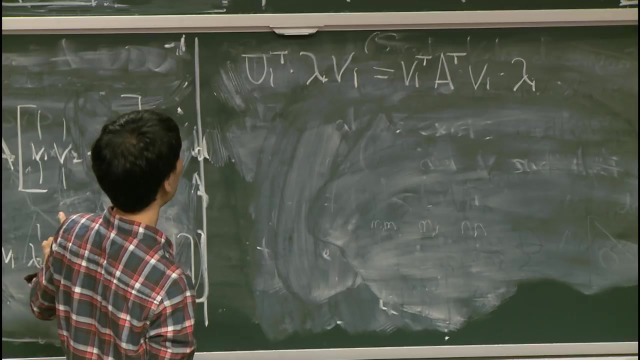 is B1 t. transpose of B1 lambda 1 t. I'm missing something. I'm missing A transpose. You're going to have it Ct. transpose of A transpose. It's just going to Maria, And how many A's does this give? 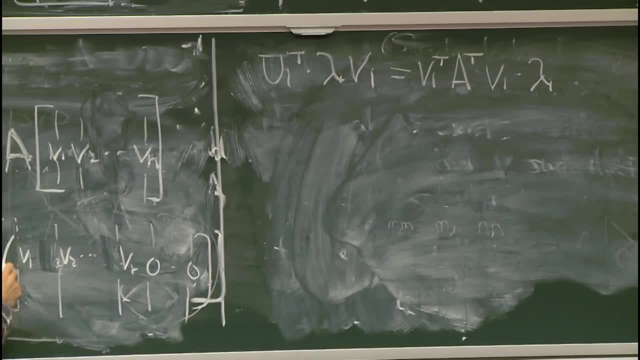 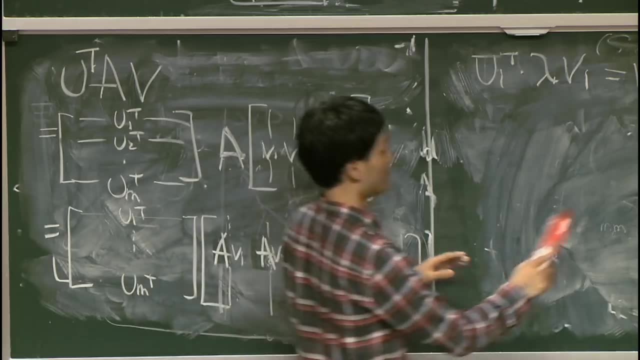 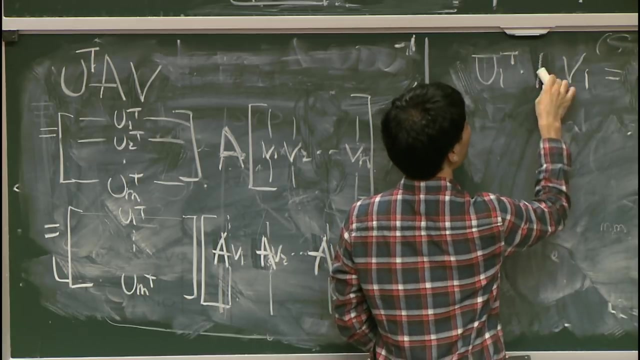 No, it's A transpose of A, transpose A One. Ah, sorry about that. This is not right. These are: As Trying to find the eigenvalue through an amounts to the A transpose. Yeah, Yes, Right, Oh right. 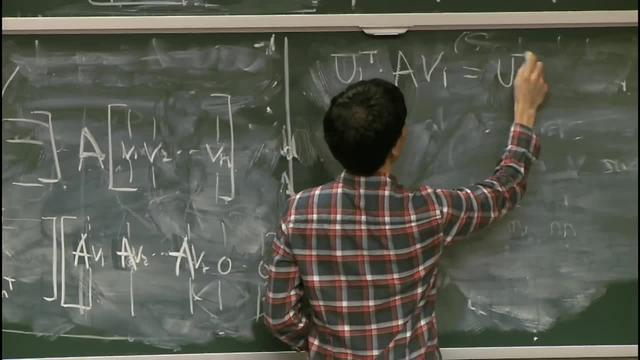 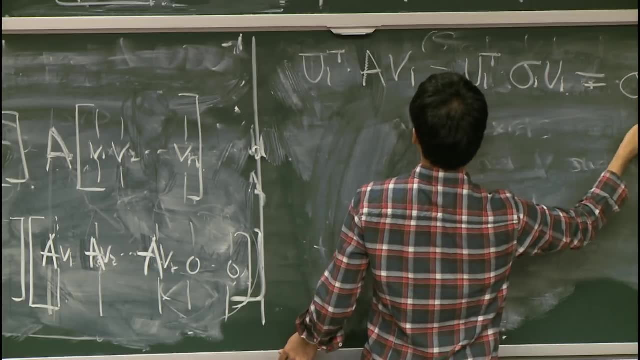 Let me Wait a minute. let me find U1, OK, and that's U1. transpose times sigma 1 times U1.. That will be 1, sigma 1.. Yeah, And then if you look at the second entry, 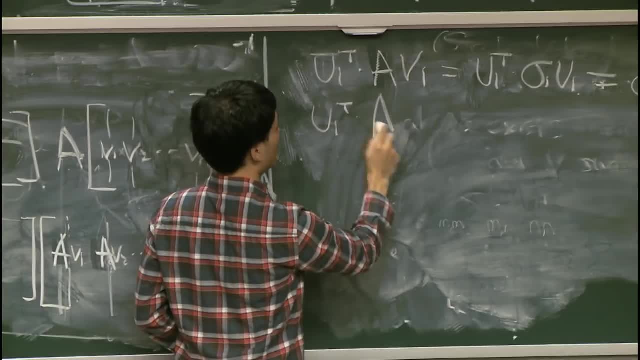 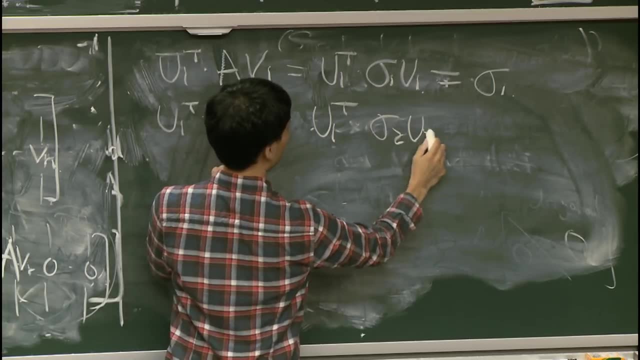 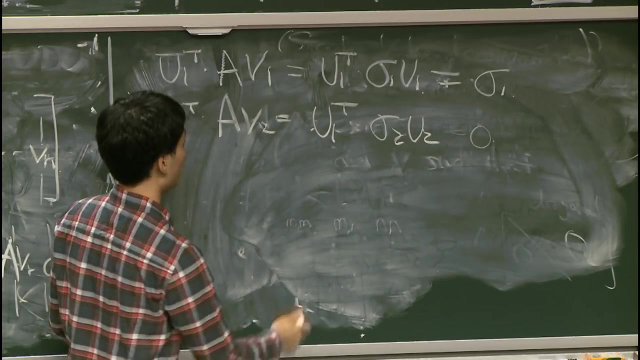 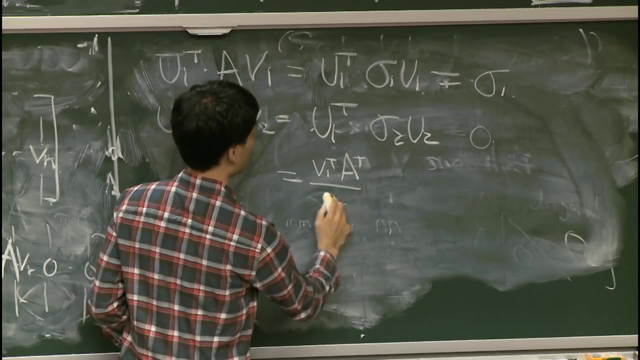 U1 transpose times AB2,. you get U1 transpose times sigma 2 of U2, but I claim that this is equal to 0. So why is that? the case U1 transpose is equal to V1 transpose, A transpose over sigma 1, and we have sigma 2.. 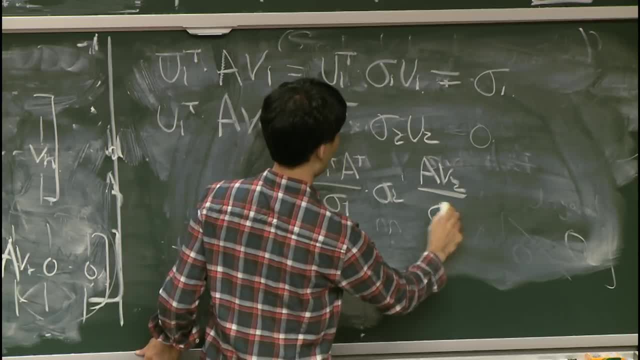 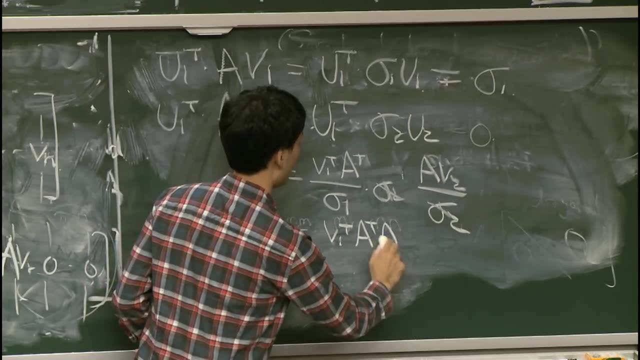 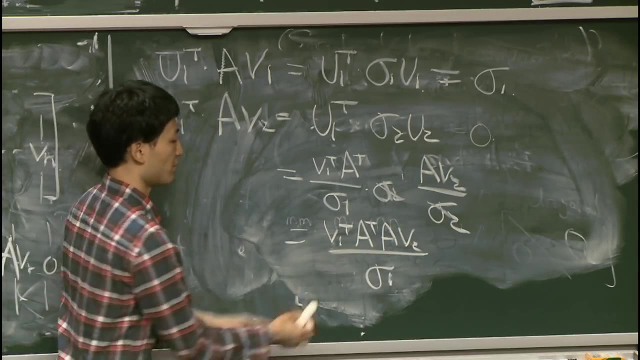 U2 is equal to A times V2 over sigma 2, those two pencils, And we have V1, T, ATA B2 over sigma 1. Sigma 1.. But V1 and V2 are two different eigenvectors of this matrix. 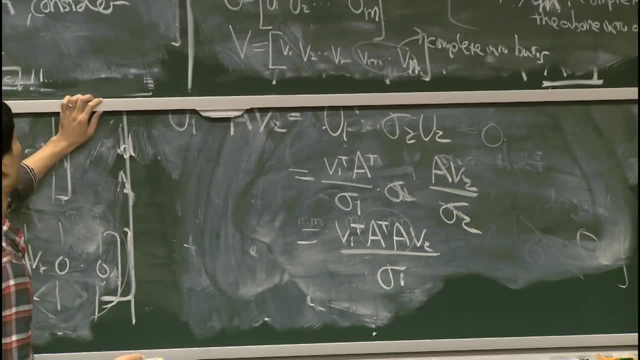 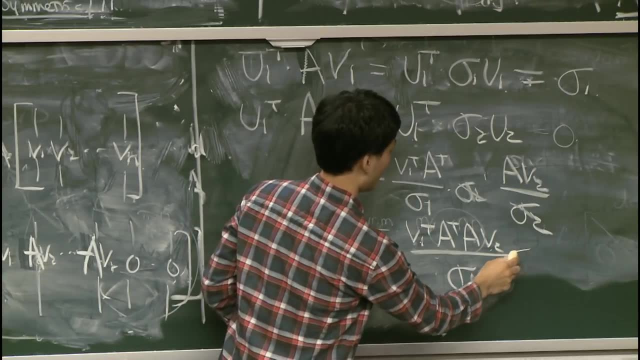 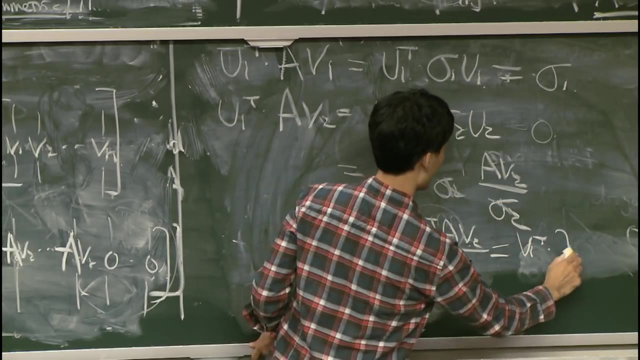 In the beginning. we can have an orthonormal decomposition of A, transpose A. That means V1, T times V2, and that has to be equal to 0, because that's an eigenvalue. We have V1, T times lambda, 2, V2 over sigma 1.. 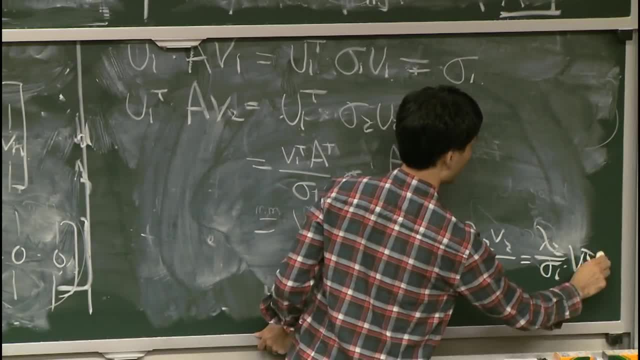 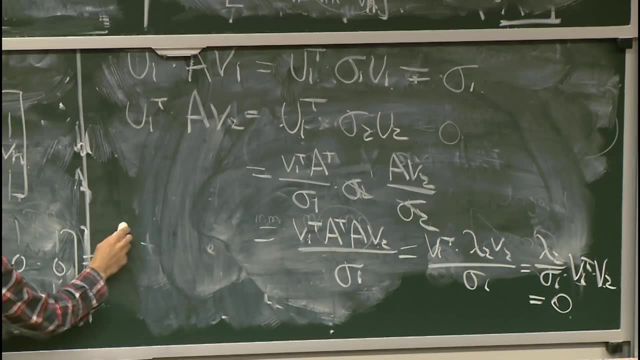 So we have lambda 2.. V2 over sigma 1 times V1 transpose V2.. These two are orthogonal, so we have 0.. So if you do the computation, what you're going to have is sigma 1, sigma 2 on the diagonal up to sigma r. 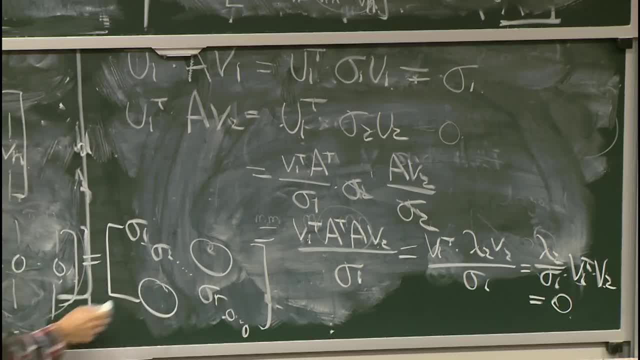 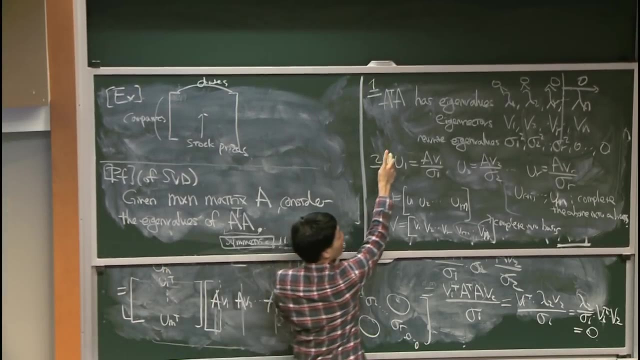 and then 0, 0, rest and 0, 0, rest. Sorry for the confusion. Actually the process is quite simple. I was just lost in the computation in the middle. So the process is: first look at A, transpose A. 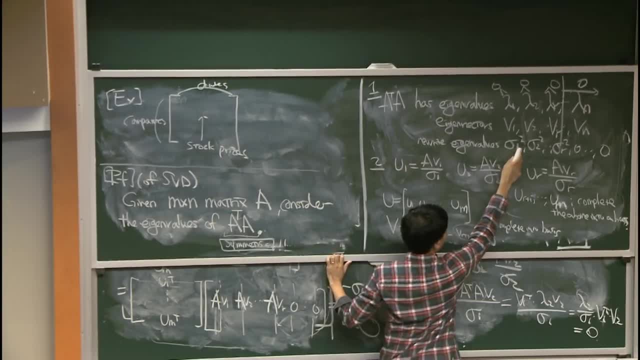 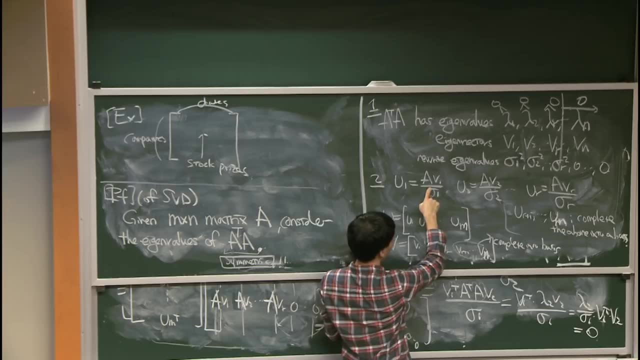 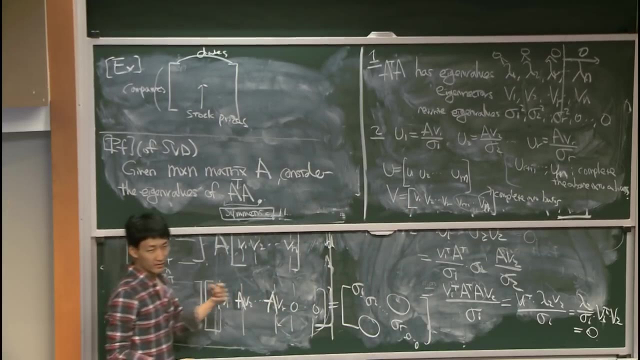 Find the eigenvalues and eigenvectors And using those they define the matrix B. And you can define the matrix U by applying A times B over sigma. Each of those will define the entries of U. The reason I wanted to go through this proof. 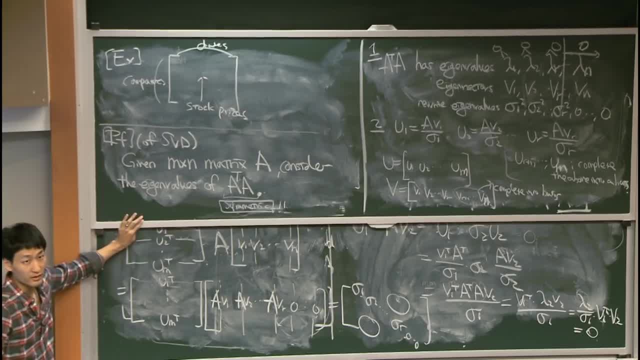 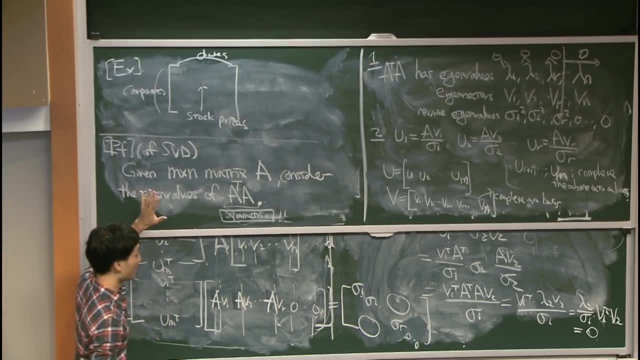 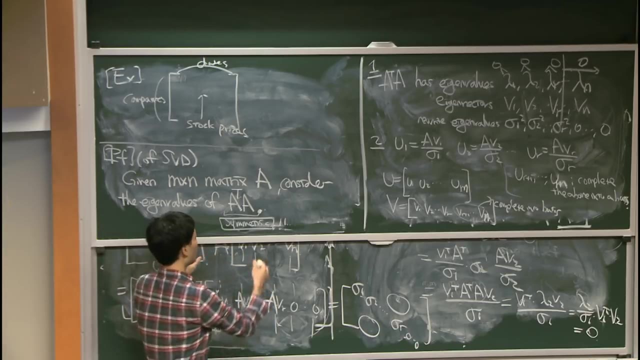 is because this gives you a process of finding a singular value decomposition. OK, It was a little bit painful for me, But if you have a matrix, there's just a simple step you can follow to find the singular value decomposition. So look at this matrix. 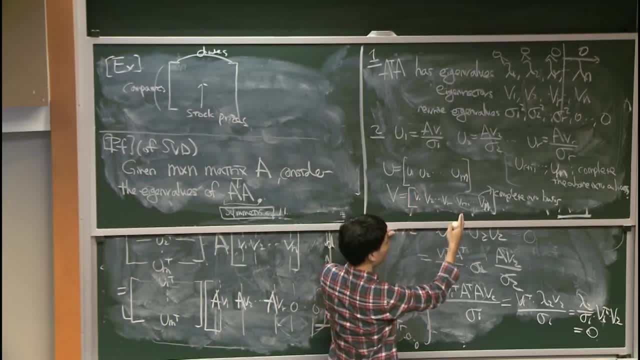 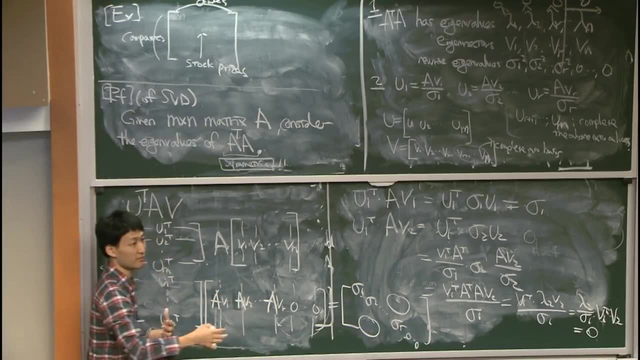 Find its eigenvalues and eigenvectors, Just arrange it in the right way. Of course, the right way needs some practice to be done correctly, But once you do that you just obtain a singular value- decomposition- And really I can't explain how powerful it is. 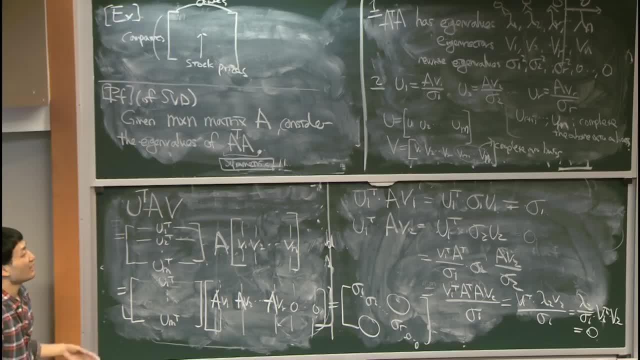 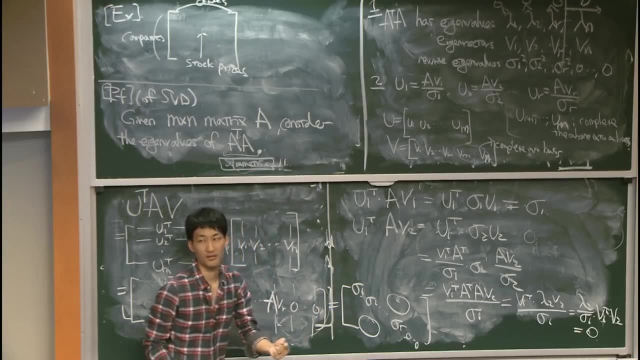 You will only later see it in the course how powerful this decomposition will be, And only then you will be more appreciate how good it is to have this decomposition and be able to compute it so simply. So let's try to do it by hand. 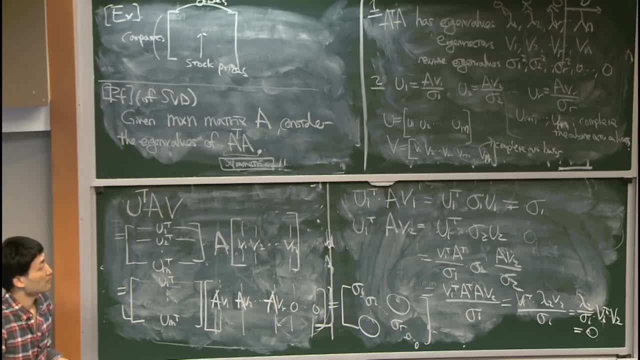 Yes, So when you compute the matrix for the matrix U you apply: Yes, So you could just randomly compute it, or do you need to? It has to be orthogonal. No, It has to be orthogonal Or thurnormal. 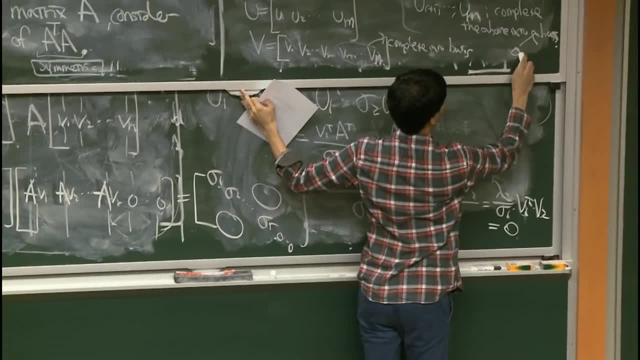 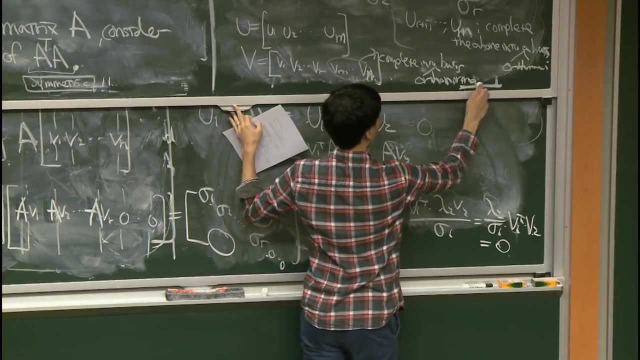 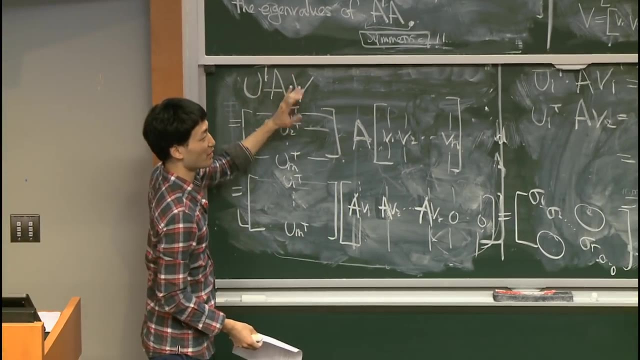 Yeah, It has to be orthogonal. It needs to be orthogonal. It needs to be orthogonal And that's a good point, because that can be annoying when you want to do it by hand. Actually, it's not decomposition, You have to do some Gram-Schmidt process or something like that. 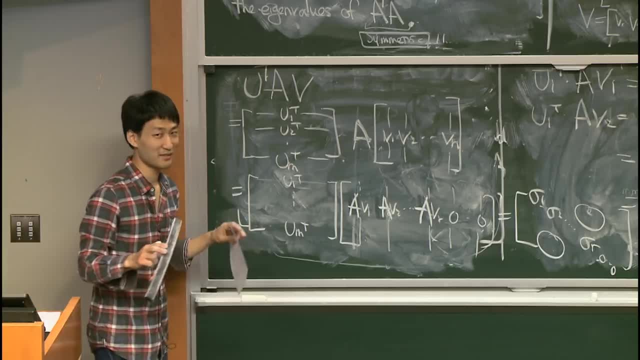 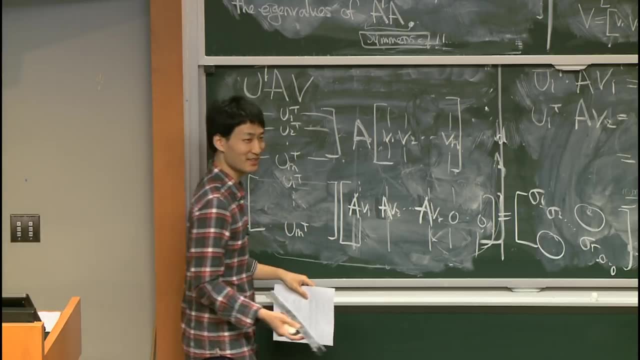 But when I mean by hand, I don't really mean by hand other than when you're doing homework, because you can use a computer to do it. And in fact, if you use a computer, there are much better algorithms than this that are known. 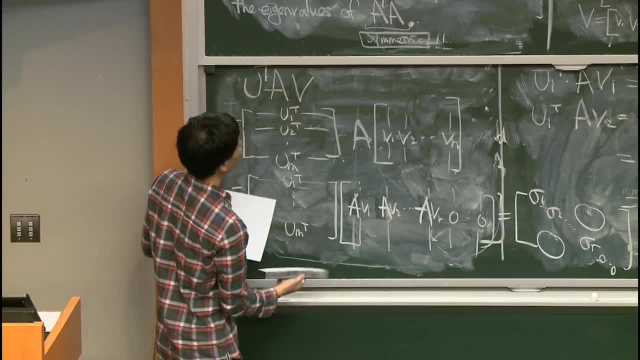 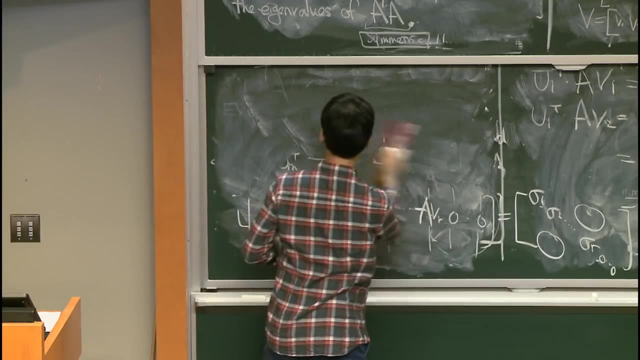 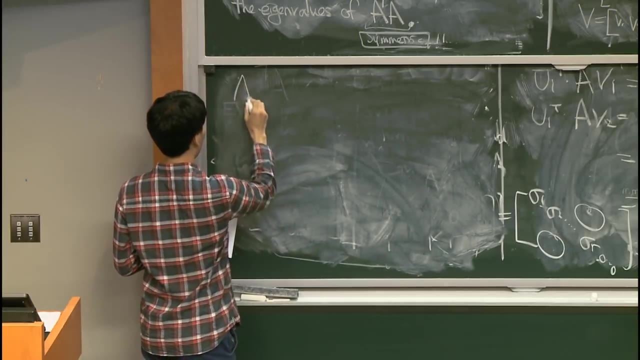 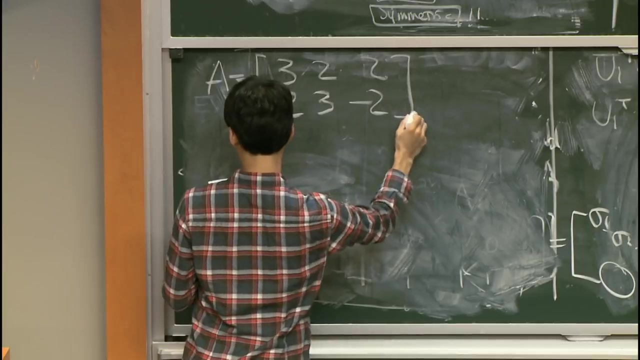 which can do this a lot more quickly and more efficiently. OK, So let's try to do it by hand. OK, So let A be this: matrix: 3, 2, 2, 2, 3, negative 2.. 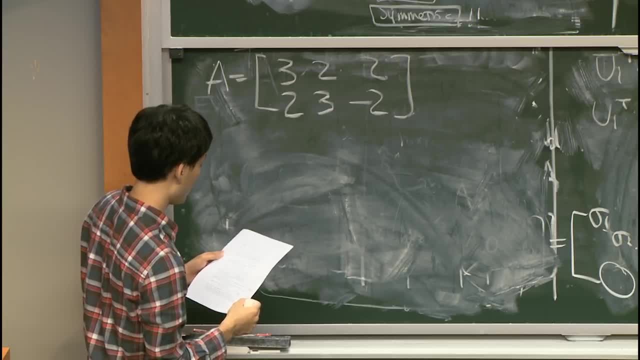 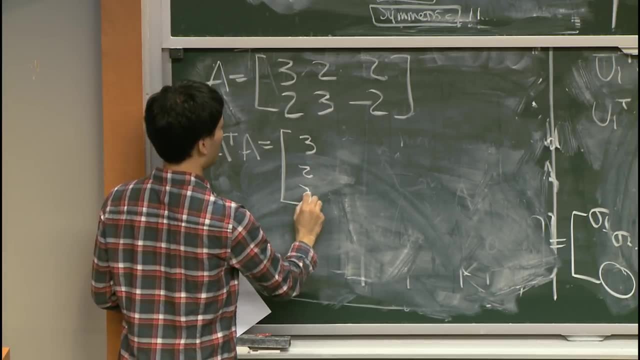 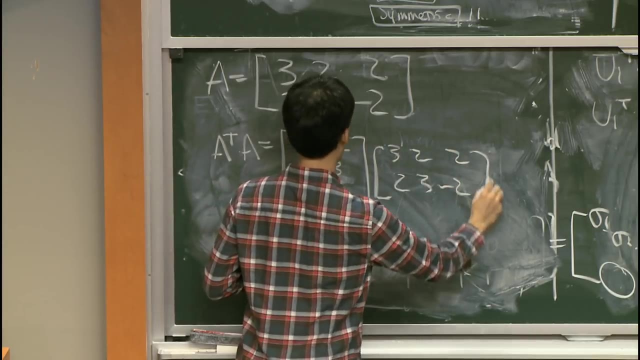 And we want to make the eigenvalues decomposition A, transpose A. we have to compute. that is 3, 2, 2,, 2, 2.. And you'll get 13,, 12, 2, 12,, 13, negative 2, 2, negative 2.. 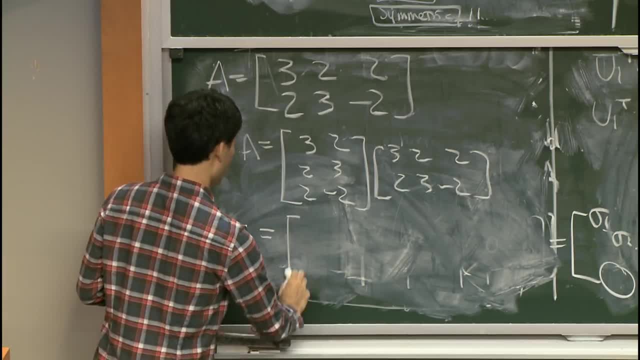 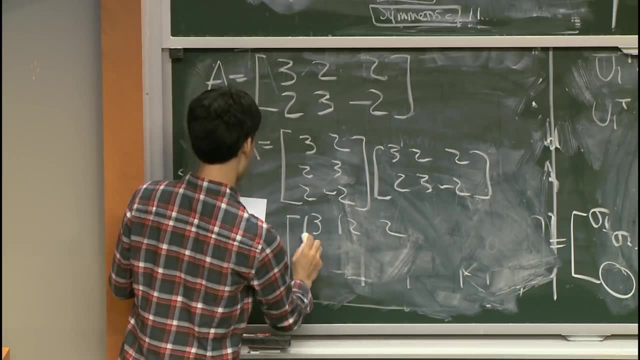 And you'll get 13,, 12,, 2,, 12,, 13, negative, 2, 2, negative 2.. And you'll get 13,, 12,, 2,, 12, 13, negative, 2, 2, negative 2.. 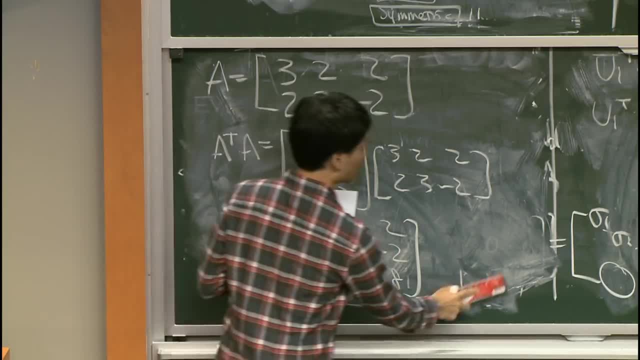 And you'll get 13,, 12,, 2,, 12,, 13, negative, 2, 2, negative 2.. And you'll get 13,, 12,, 12,, 12, 13, negative, 2, 2, negative 2.. 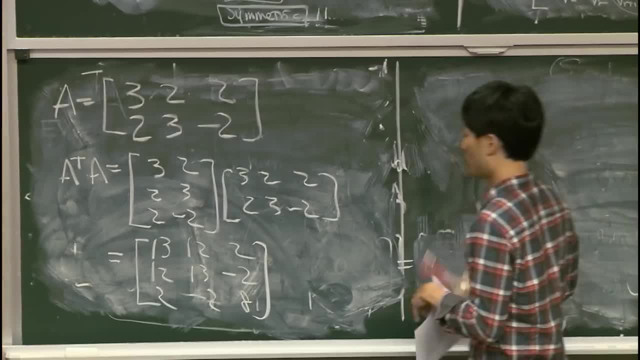 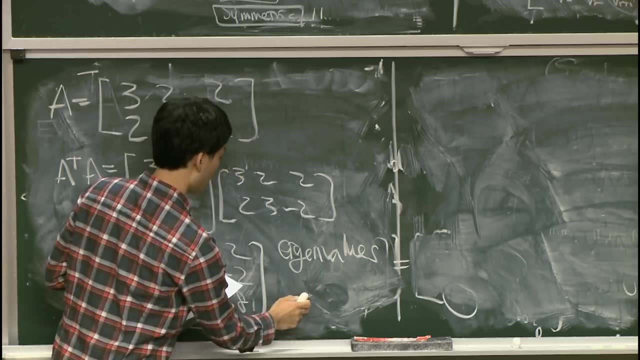 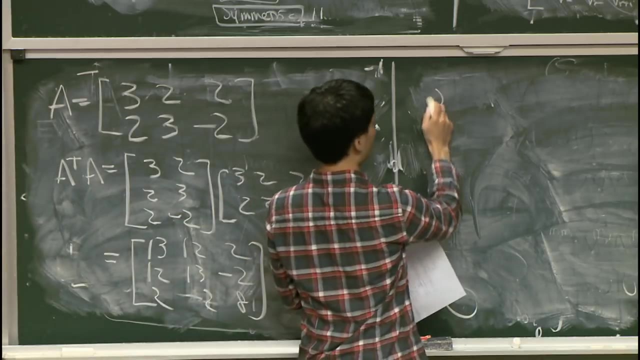 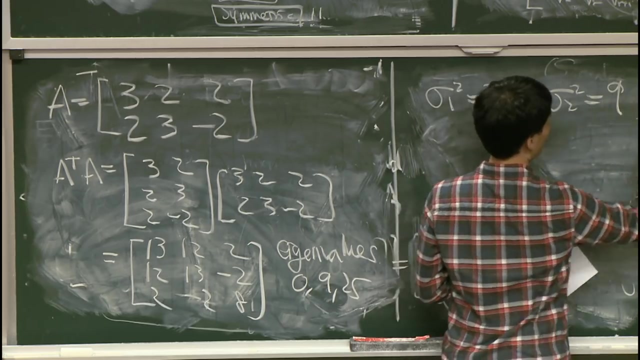 And let me just say that the eigenvalues are 0,, 9, and 25.. So in this algorithm, sigma 1 squared will be 25.. Sigma 2 squared will be 9. And sigma 3 squared will be 0.. 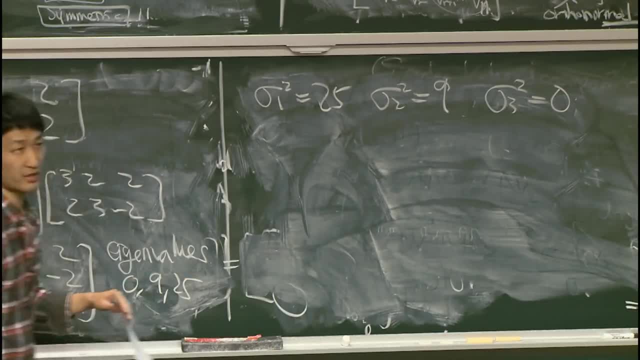 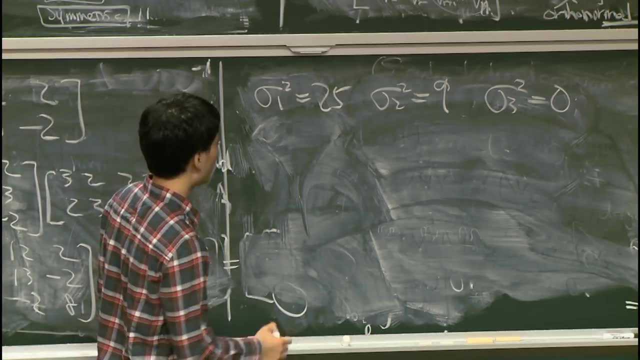 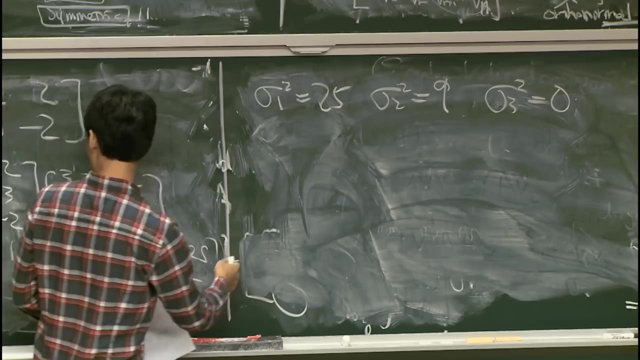 So we can take sigma 1 to be 5, sigma 2 to be 3.. Sigma 3 to be 0.. OK, Now we have to find the corresponding eigenvectors, to find the singular value decomposition. And I'll just do one, just to remind you. 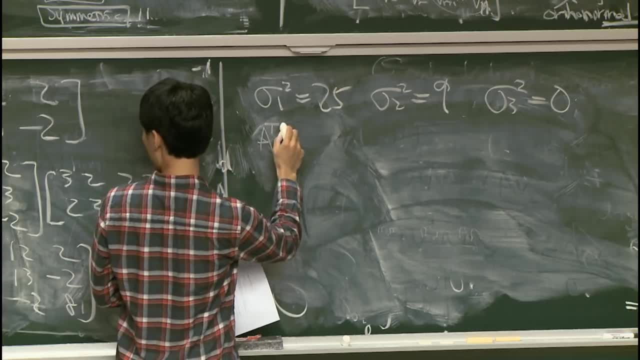 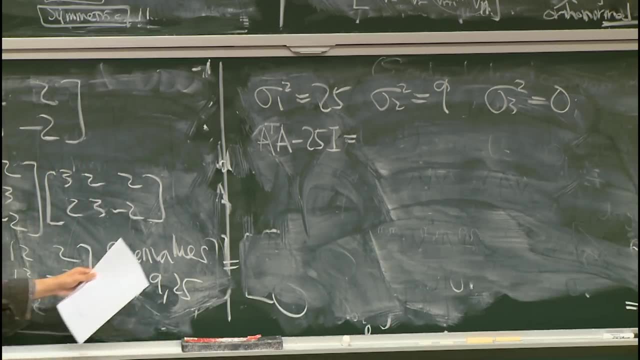 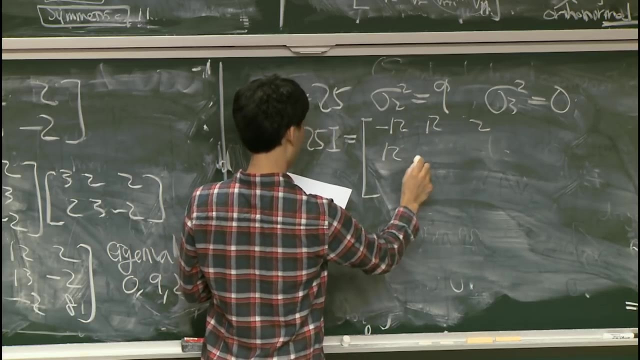 how to find an eigenvector. So A transpose A minus 25i is equal to subtract 25 from these entries You're going to get negative 12, 12, 2, 12, negative 12, 2, 2,. 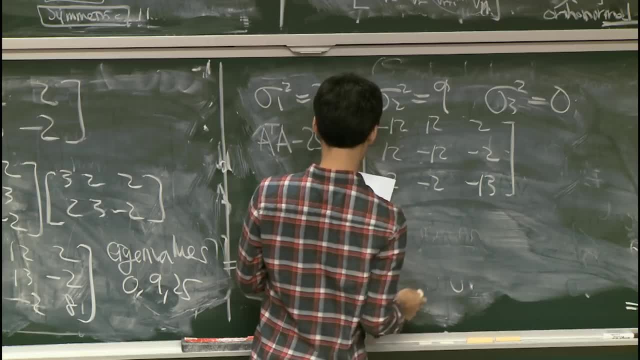 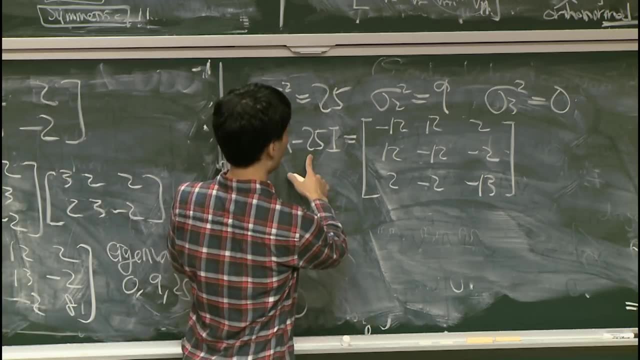 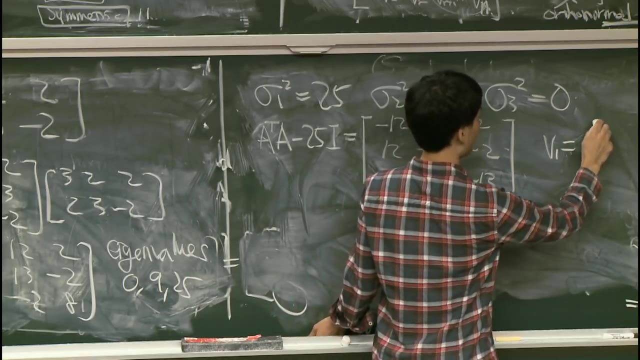 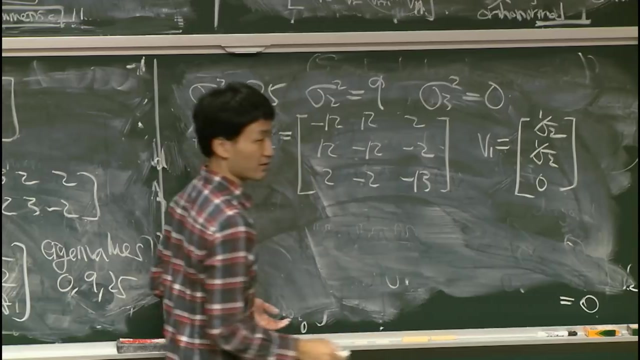 negative, 12,, 13.. And then you have to find the vector which annihilates this matrix, And that will be. you can take one of those vectors to be just 1 over square root, 2.. 1 over square root: 2,, 0,. after normalizing: 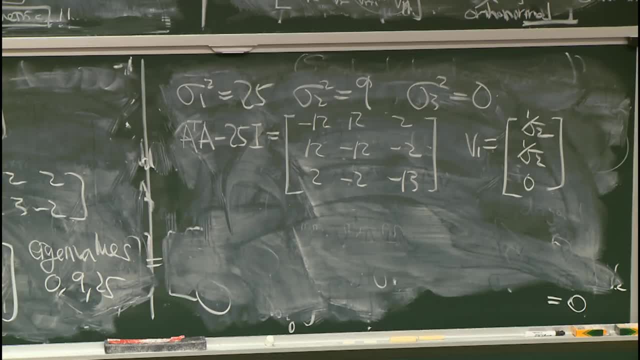 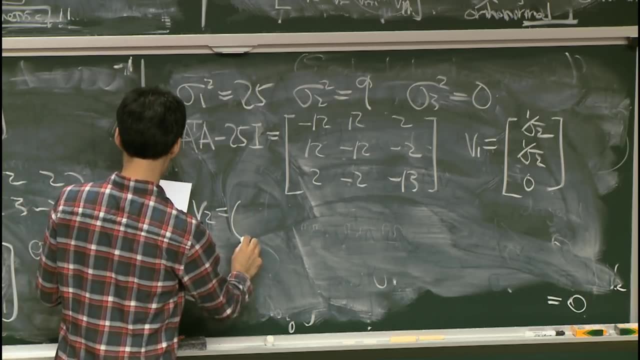 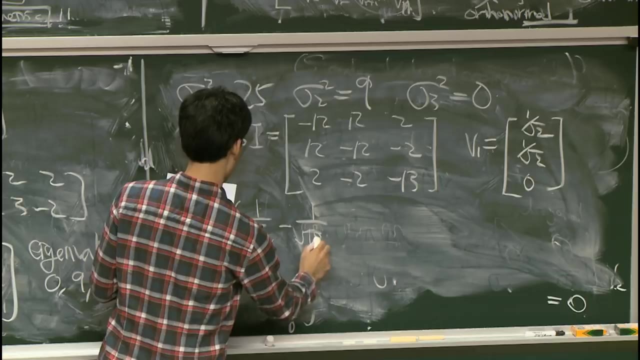 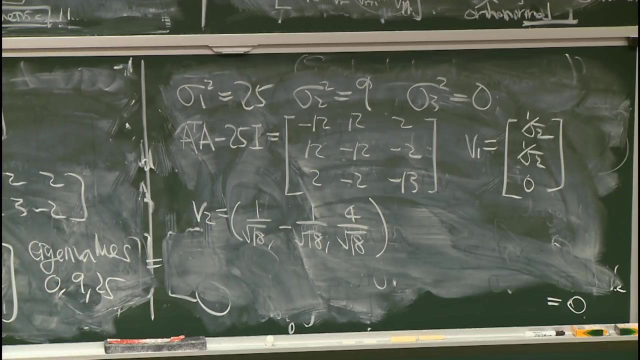 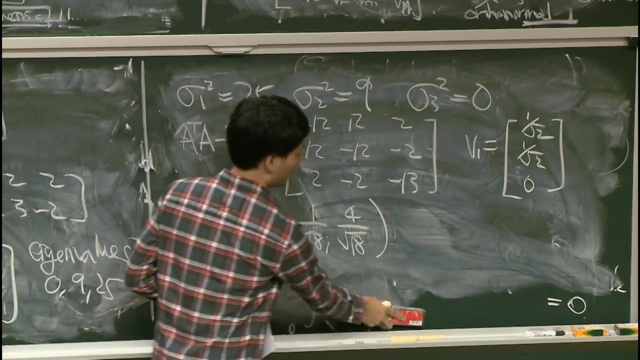 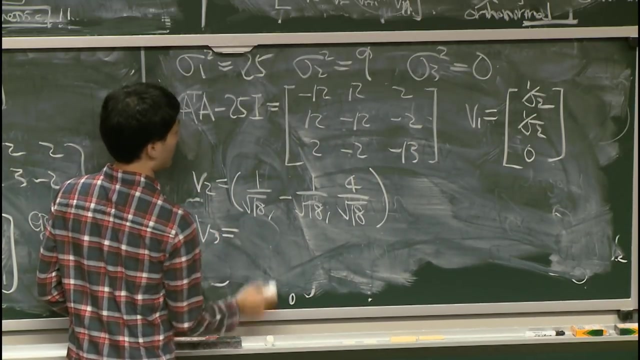 And then just do it for other vectors. You find V2 to be 1 over square root 18, negative: 1 over square root 18, 4 over square root 18.. OK, Now then find V3 to be the one that annihilates this. 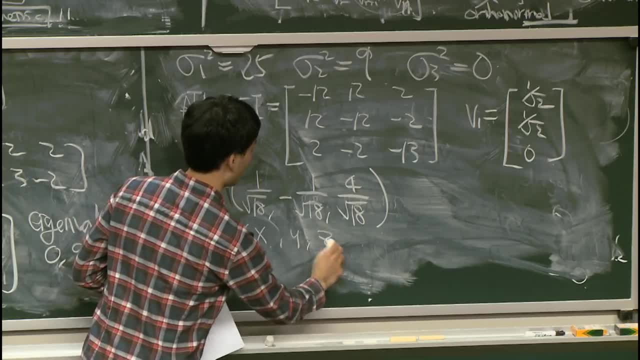 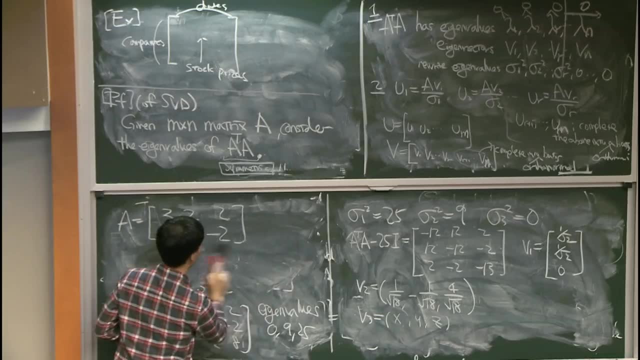 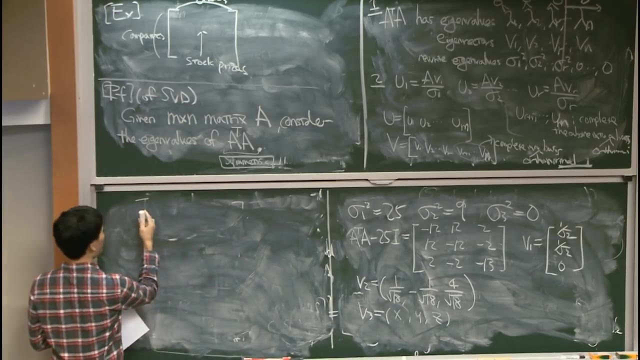 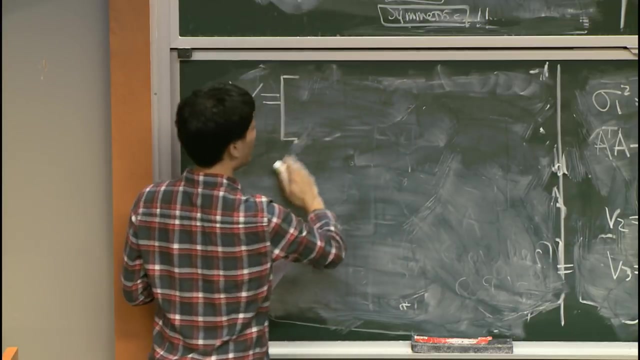 But I'll just say it's x, y, z. This will not be important. I'll explain why it's not that important, OK. OK, Then our V, as written above. actually there, it was transposed, so I will transpose it. 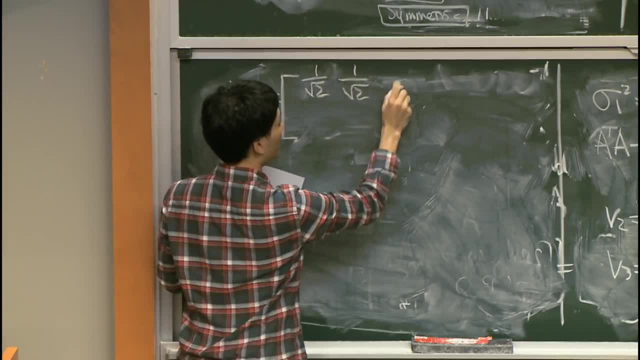 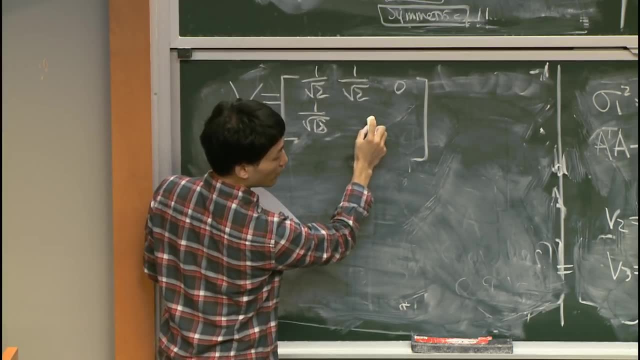 It'll be 1 over square root 2, 1 over square root 2, 0.. V2 is that, So we can write 1 over square root 18.. OK, Negative: 1 over square root 18,. 4 over square root 18.. 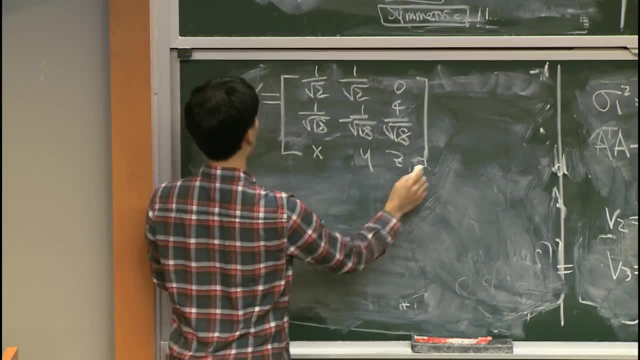 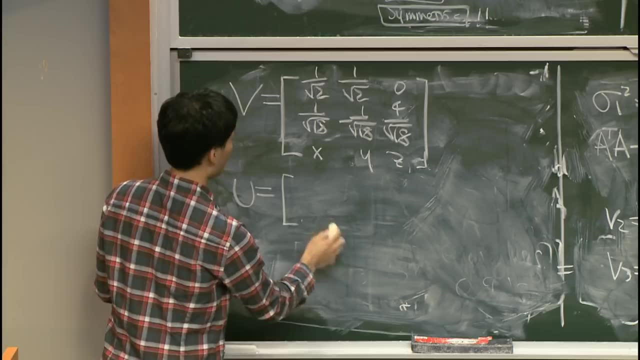 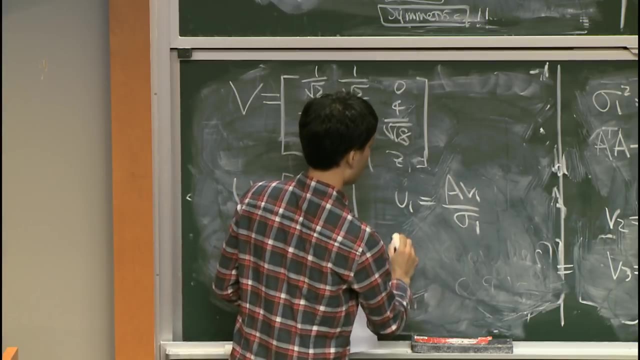 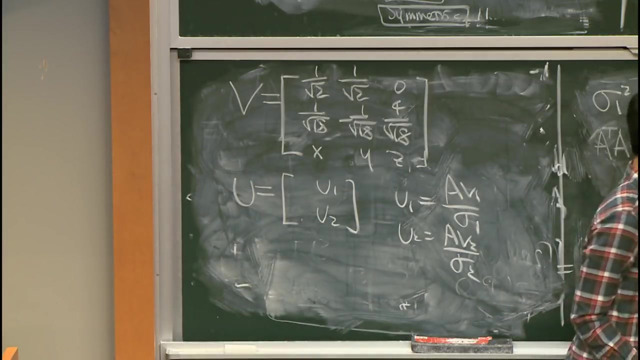 And here just write x, y, z and u will be defined as u1 and u2, where u1 is a times v1 over sigma 1.. u2 is a times v2 over sigma 2.. So multiply a by this vector. 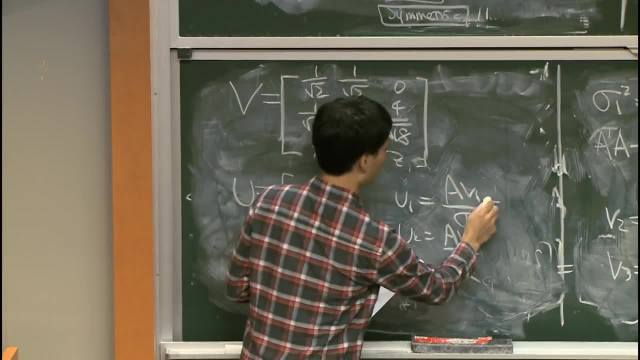 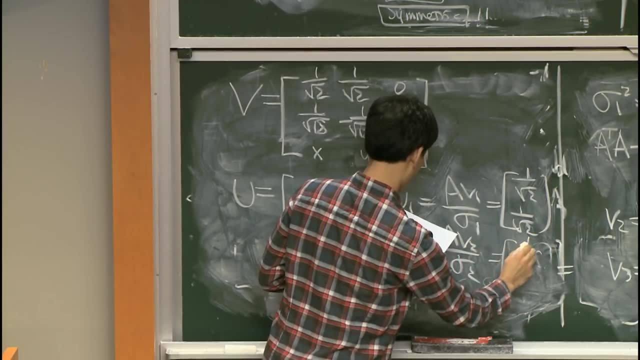 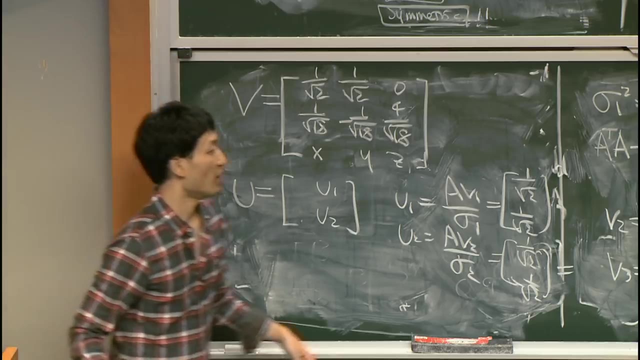 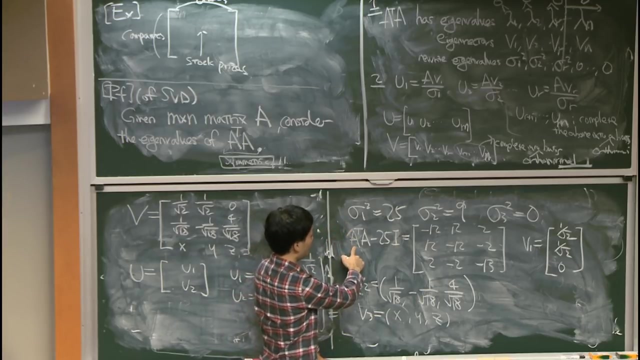 Divide by sigma 1 to get u. I already did the computation for you. It's going to be, and this is going to be, v1.. OK, So if you did the computation right in the beginning to get the eigenvalues, then at a minus 25i this has to be. 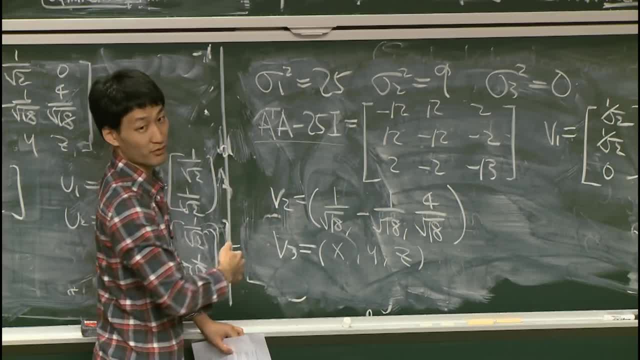 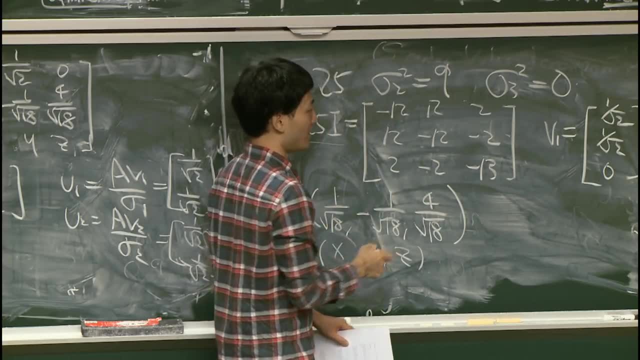 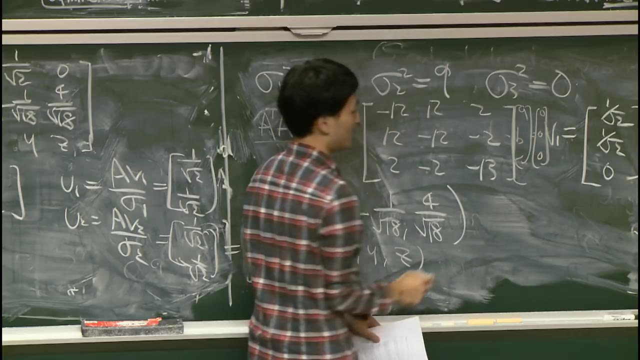 what is? it has to not have full rank. So there has to be a vector v which, when multiplied by this, gives 0, 0, 0 vector. And then you say abc, you set it equal to 0, 0, 0,. 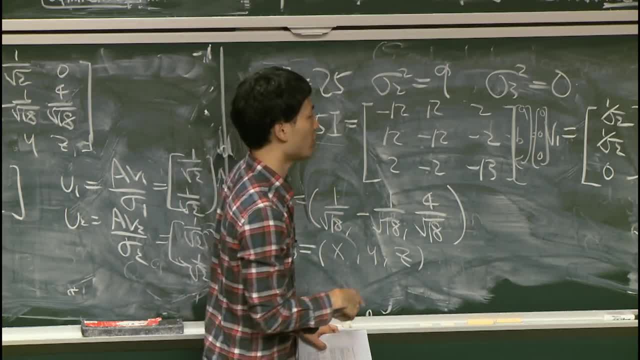 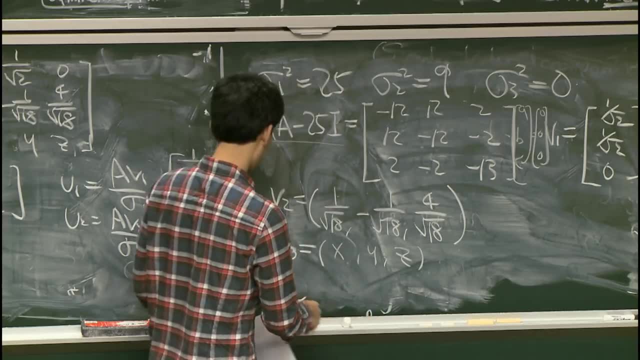 and just solve the system of linear equations. OK, there will be several of them. For example, you can take 1,, 1, 0 as well, but I just normalize it to be half normal. So there is a lot of work involved. 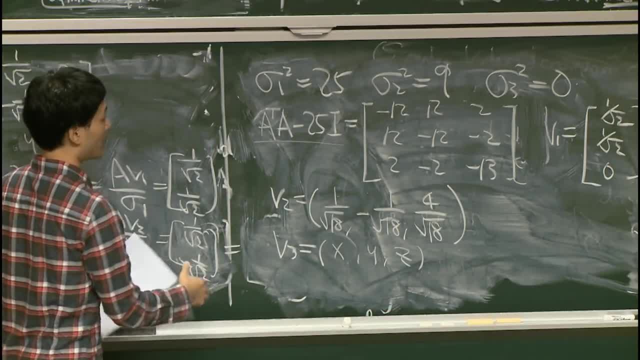 if you want to do it by hand, even though you can do it- You have to find eigenvalues, find eigenvectors. In this case, you have to find three of them- And then you have to do more work and more work. 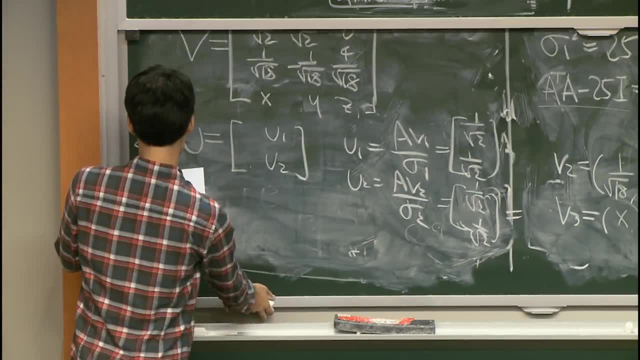 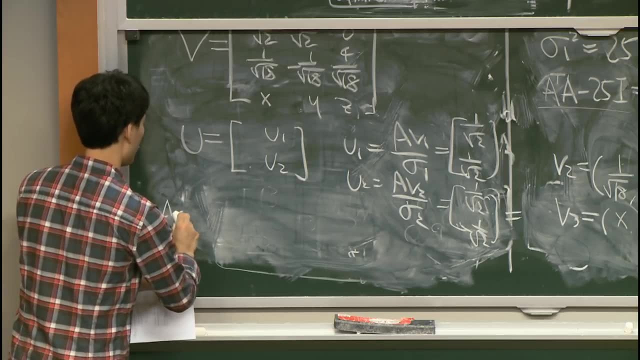 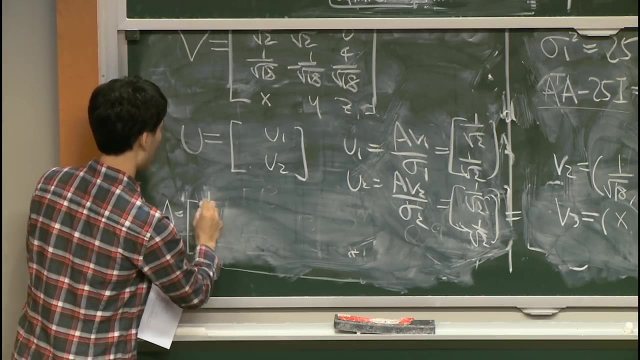 But it can be done And we are done now. So now this decomposes a into u sigma v transformation. So u is given as 1 over sigma OK, OK, 1 over square root of 2, 1 over square root of 2.. 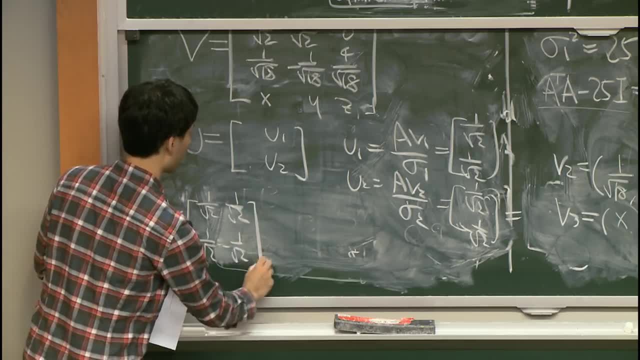 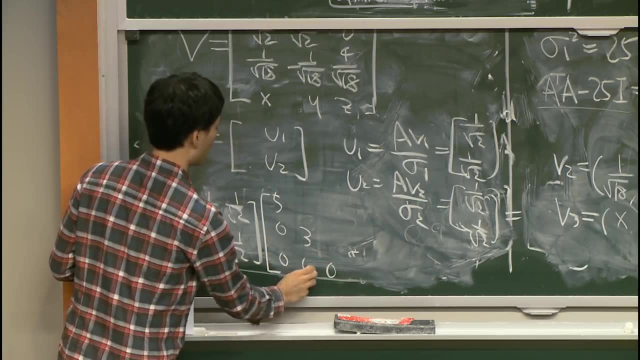 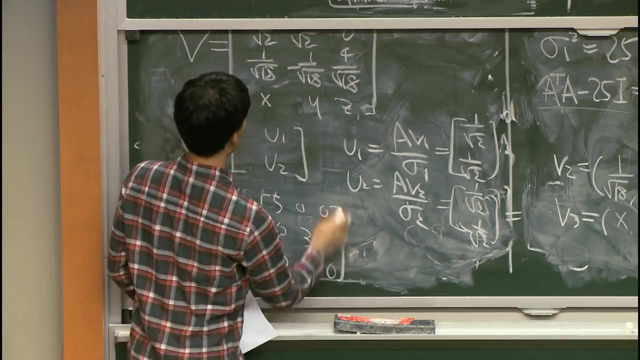 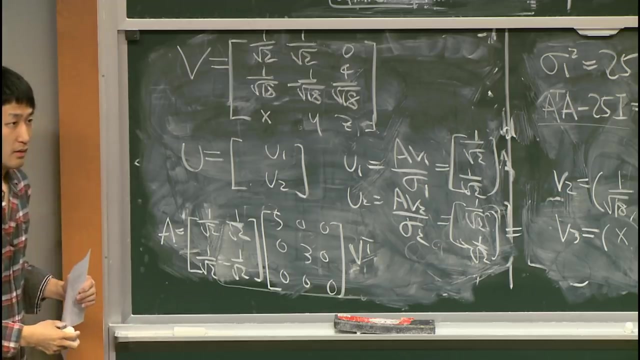 1 over square root of 2 minus 1 over square root of 2.. Sigma was 5, 3, 0.. And v is this. So v transpose is just transpose of that. I'll just write it like that. where v is that. 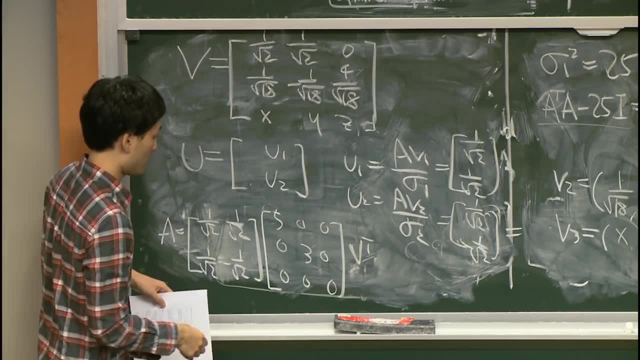 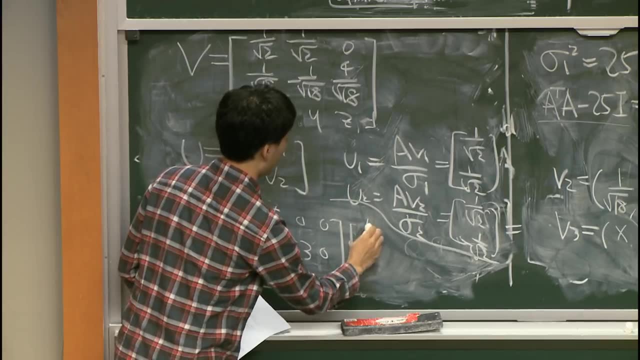 So we have this decomposition, And so let me actually write it, because I want to show you why x, y, z is not important: 1 over square root of 2, 1 over square root of 2, 0.. 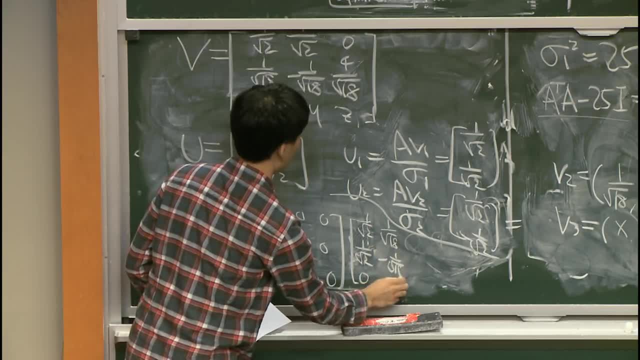 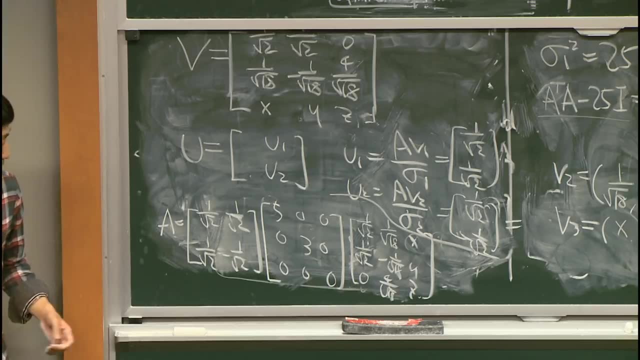 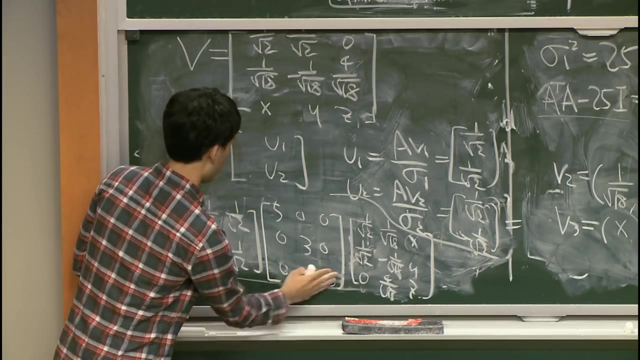 1 over square root of 18 minus 1 over square root of 18, 1 over square root of 18, x, y, z. The reason I'm saying this is not important is because I can just Drop. Oh, what did I do here? 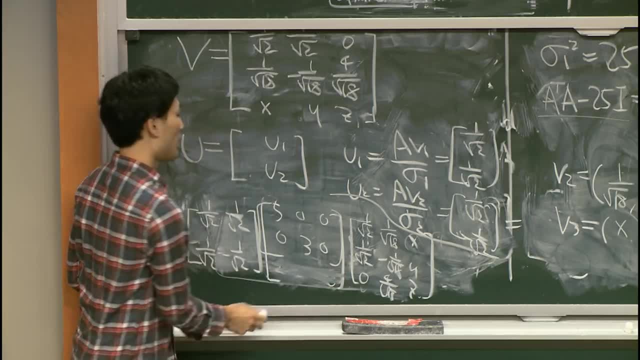 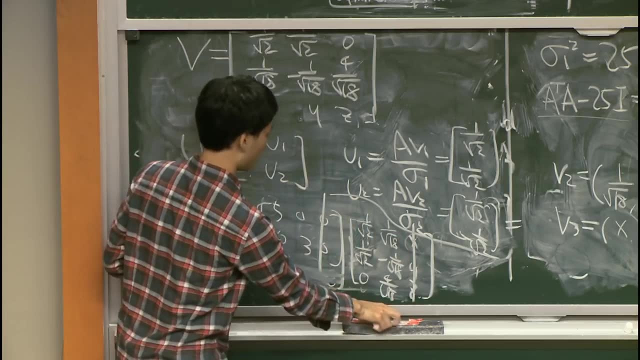 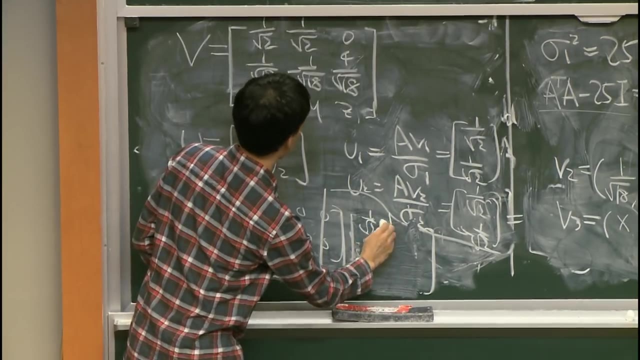 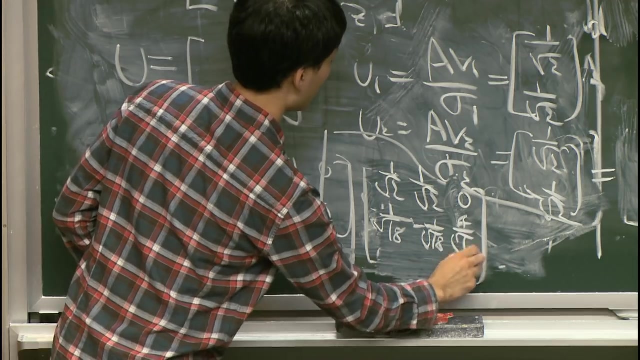 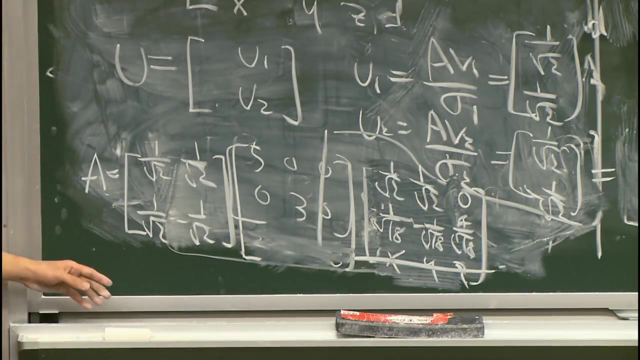 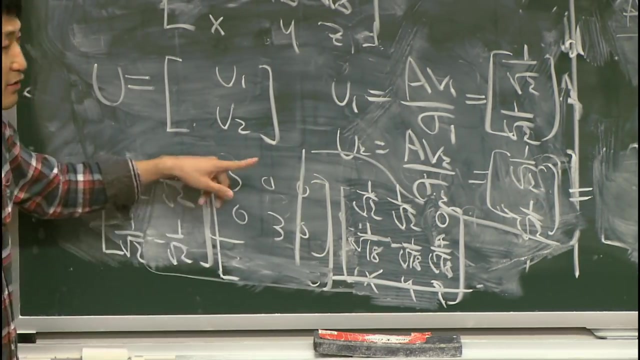 It has to be 2 by 3.. I can just drop this column and drop this column together. Let's leave that for Drop this and drop this all together. So the message here is that the eigenvectors corresponding to eigenvalue 0 are not important. 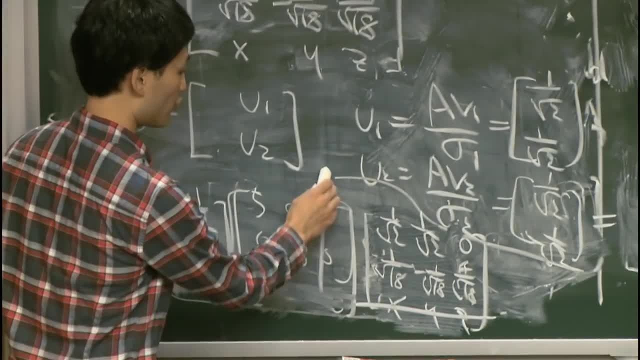 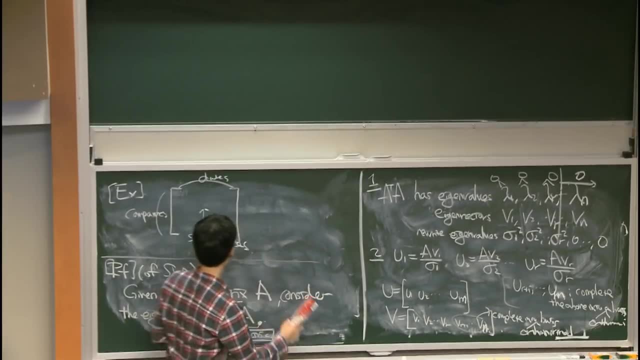 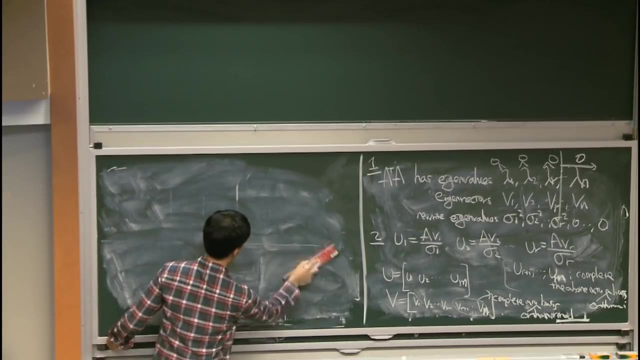 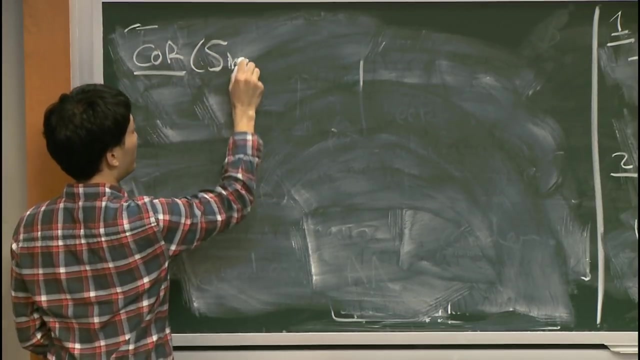 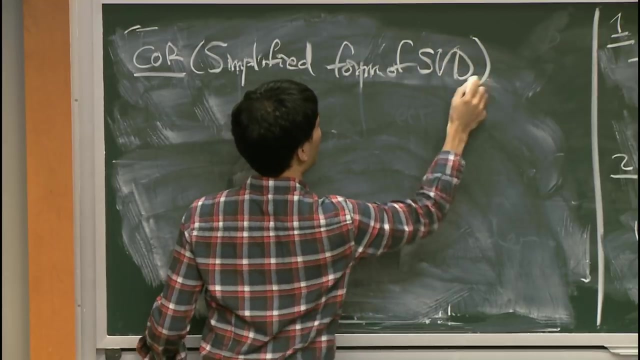 The only relevant ones are non-zero eigenvalues. So drop this and drop this. That will save you some computation. So let me state a different form of singular value decomposition. So this works in general. There's a corollary. We get a simplified form of SPD where 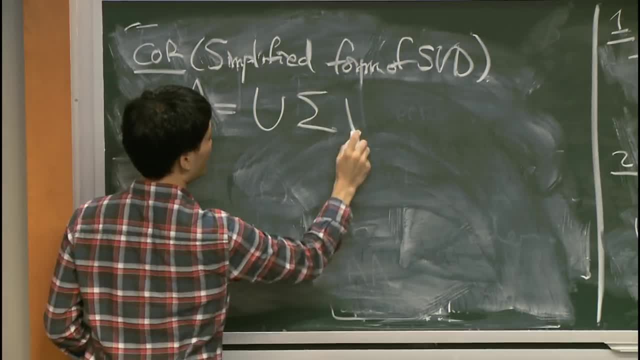 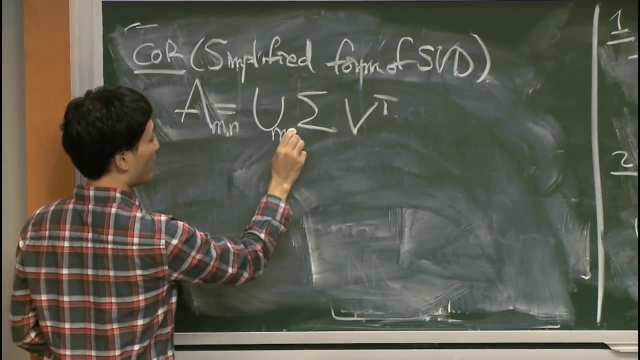 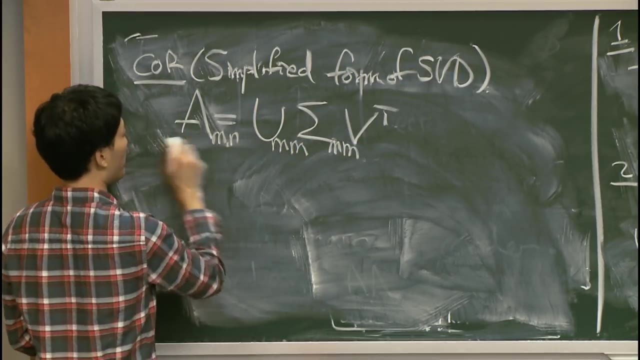 A becomes equal to U times sigma times V transpose: And A was an m by n matrix. U is still an m by n matrix, But now sigma is also an m by n matrix. This only works when m is less than or equal to m. 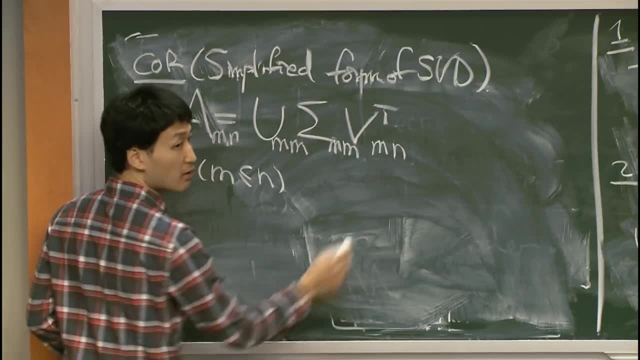 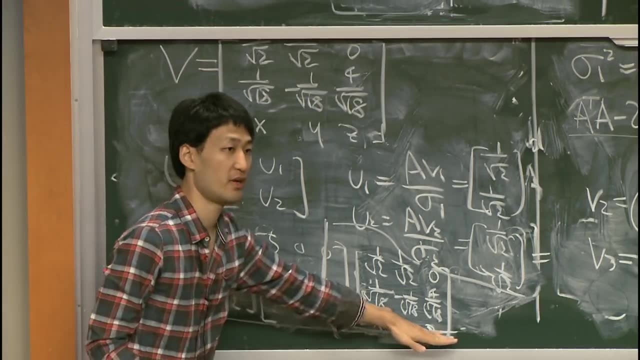 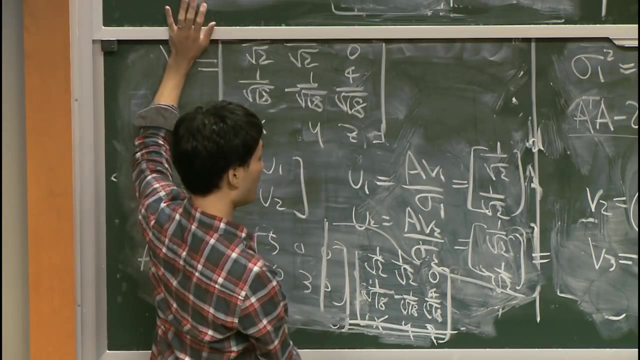 And V is an m by n matrix. So the proof is exactly the same And the last step is just to drop the irrelevant information. So I will not write down why it works, But you can see. if you go through it, you'll see that dropping this part. 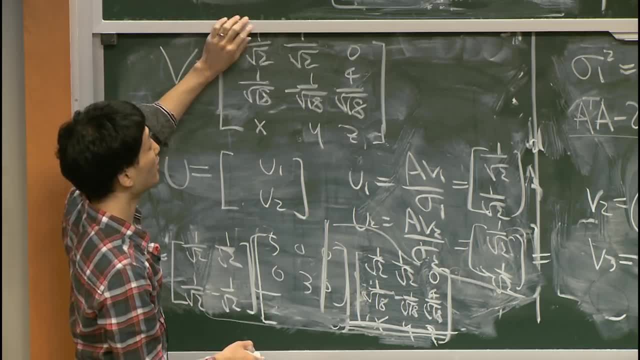 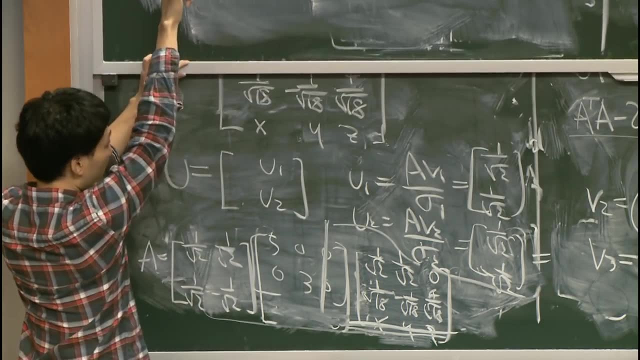 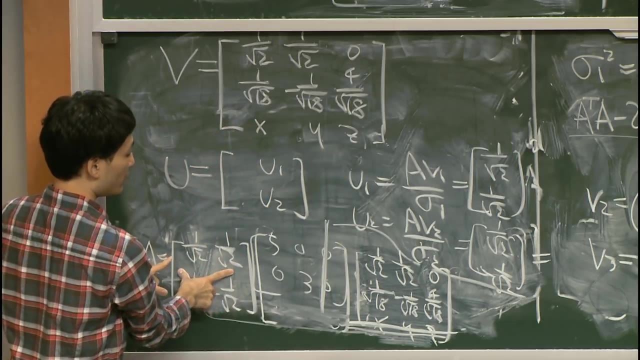 It just corresponds to exactly that information. So that's a reduced form. So let's see: In the beginning we had A. I erased A. A was a 2 by 3 matrix in the beginning And we obtained a decomposition into 2 by 2, 2 by 2,. 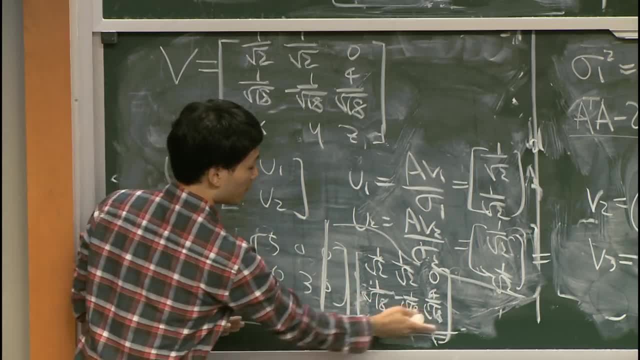 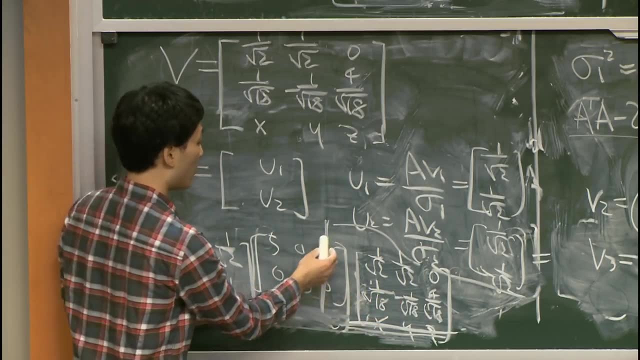 and 2 by 3 matrix. If we didn't delete this column and this row, we would have obtained a 2 by 2 times 2 by 3 times 3 by 3 matrix. But now we can simplify. We can simplify it by removing those. 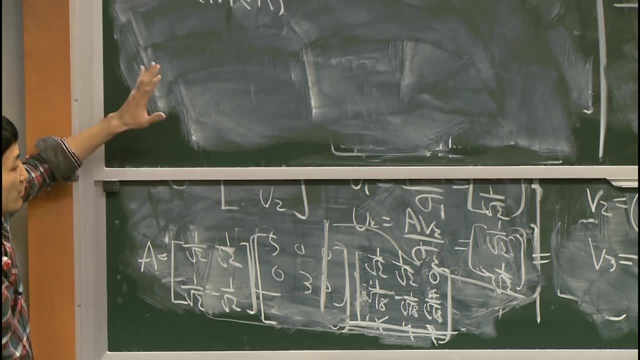 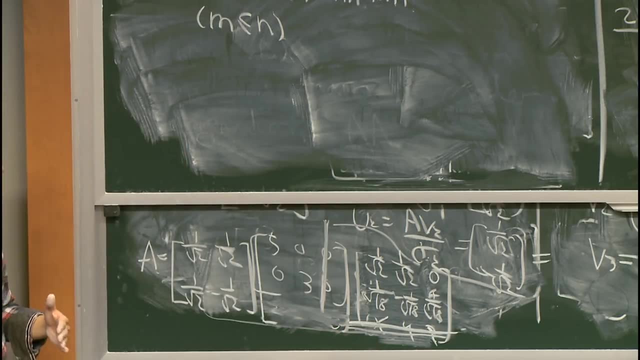 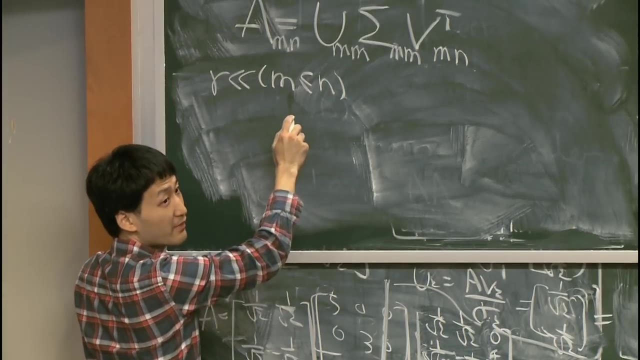 And it might not look that much different on this board because I just erased one row, But many matrices that you'll see in real application have a lot lower rank than the number of columns and rows. So if r is a lot more smaller than both m and n, 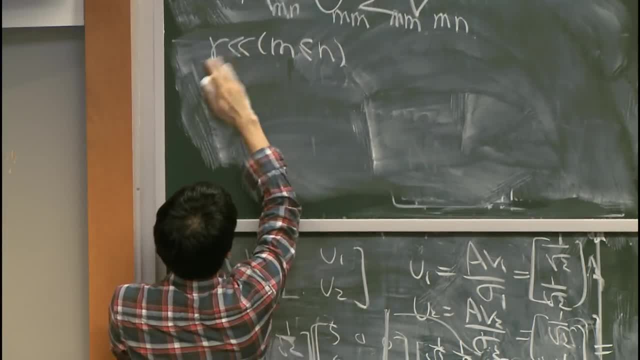 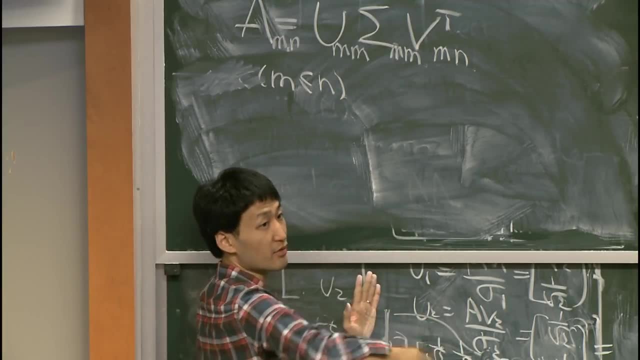 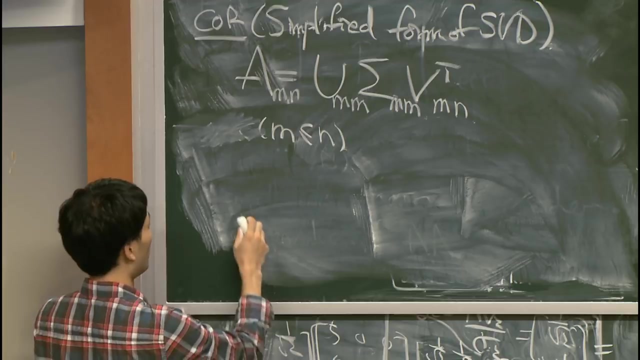 then this part really r. Oh, it's not obvious here, But If M and N has a big gap here, really the number of rows, the number of columns that you're saving, it can be enormous. So to illustrate an example, look at this. 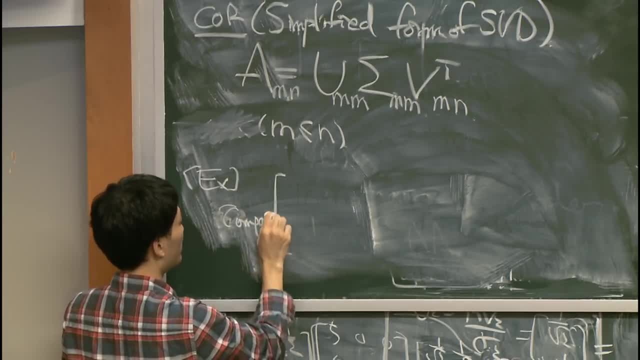 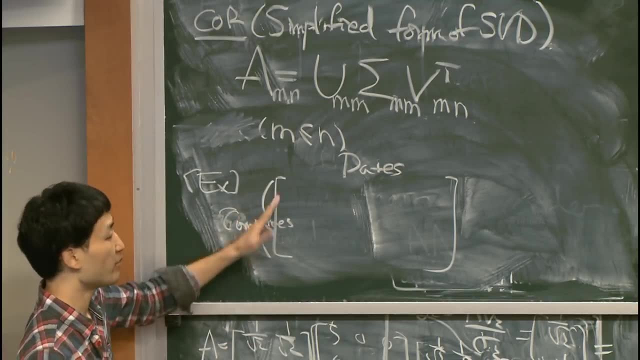 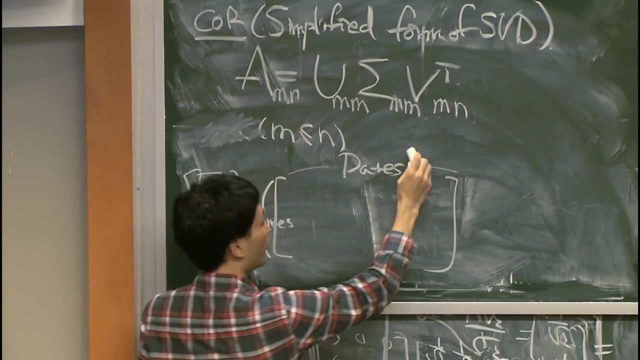 Now look at the stock prices, where you have companies and dates. Previously I just gave you an example of a 3 by 3 matrix, But it's more sensible to have a lot more dates than companies. So let's say you recorded 365 days of a year. 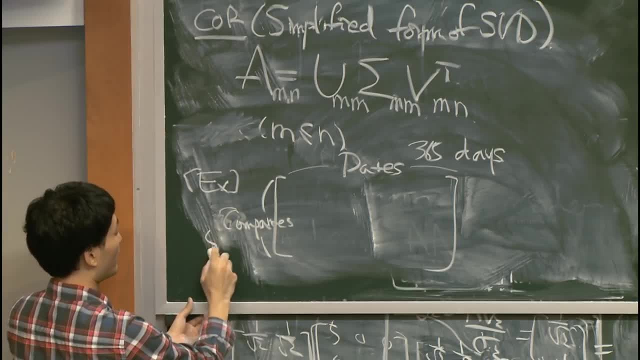 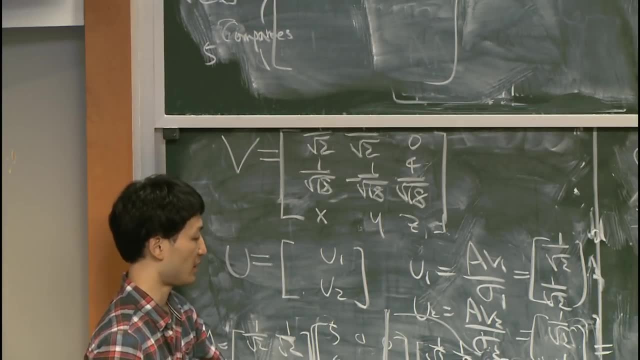 even though the market is not open all days, and just like five companies. If you did a decomposition like this, you'll have a 5 by 5, 5 by 365, 365 by 365 here, But now in the reduced form, you're saving a lot of space. 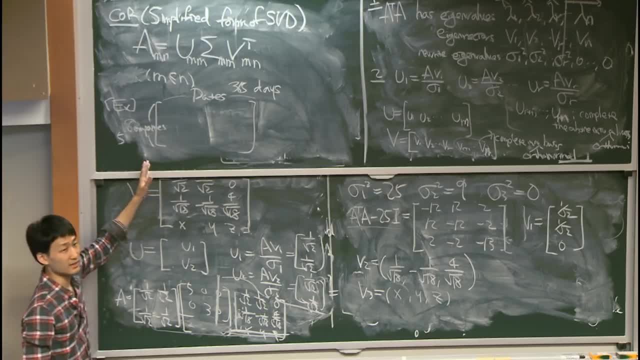 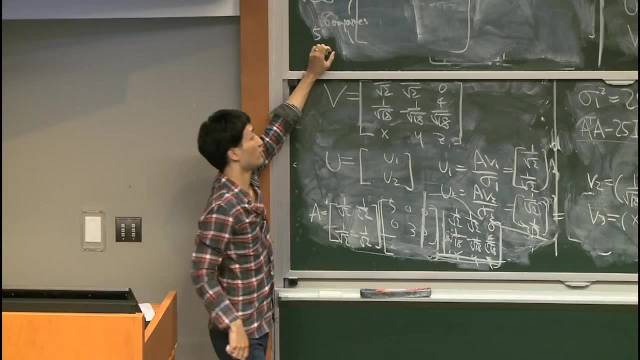 So if you just look at the board, it doesn't look like it's so powerful, But in fact it is. So that's the reduced form, And that will be the form that you'll see most of the time, this reduced form. 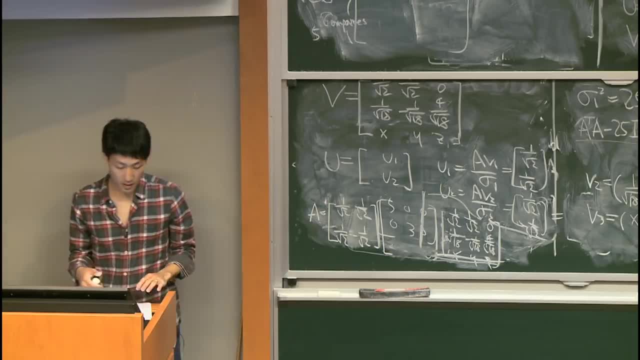 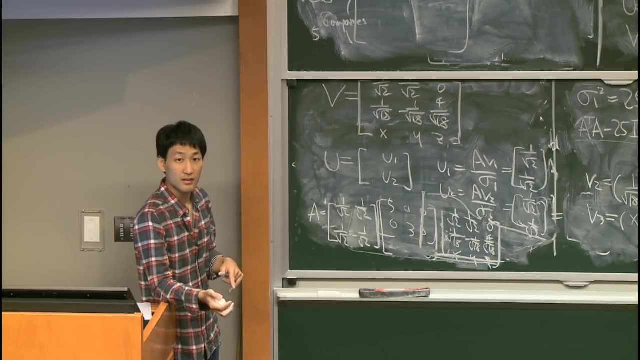 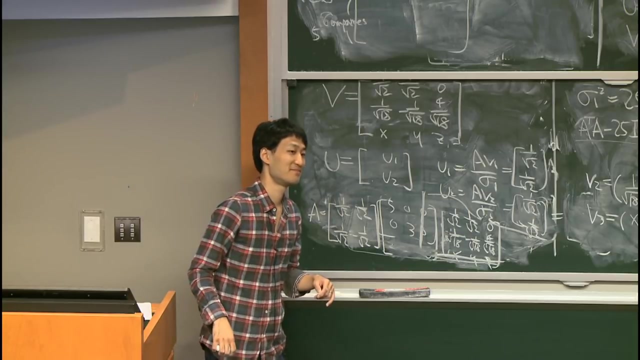 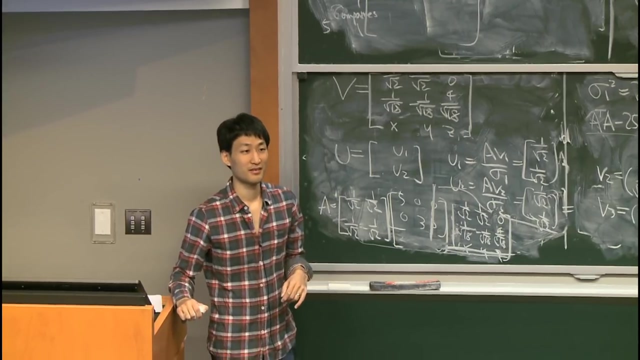 So I made a lot of mistakes. today I have one more topic, but it's totally irrelevant topic. So any questions before I move on to the next topic? Yes, Can you press it back to me, Mm-hm? 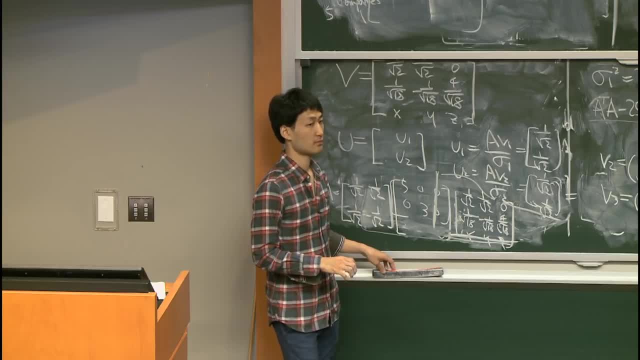 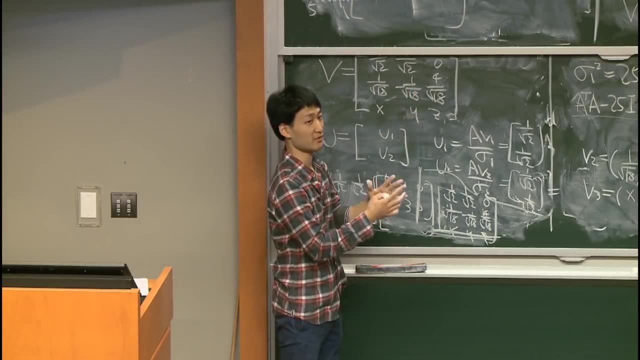 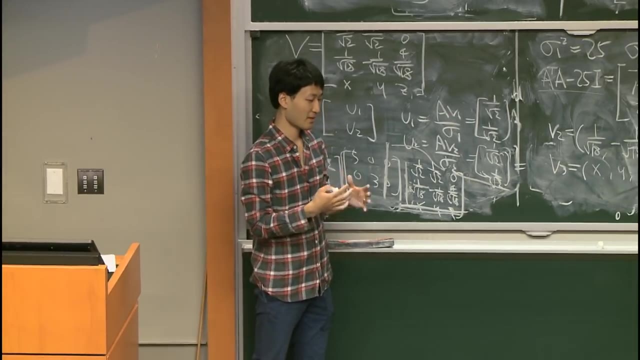 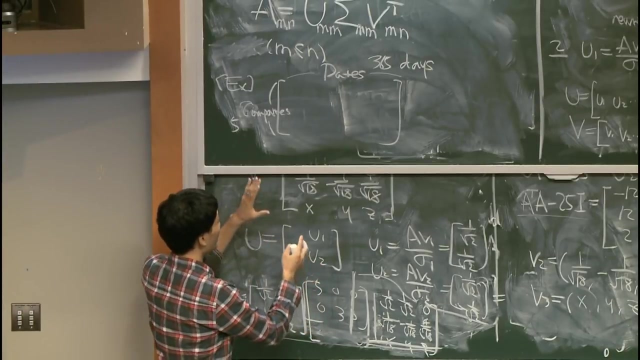 Oh, so in this data what it means. You're asking what the eigenvectors will mean over this data. It will give you some stocks, It will give you the correlation. So each eigenvector will give you a group of companies that are correlated somehow. 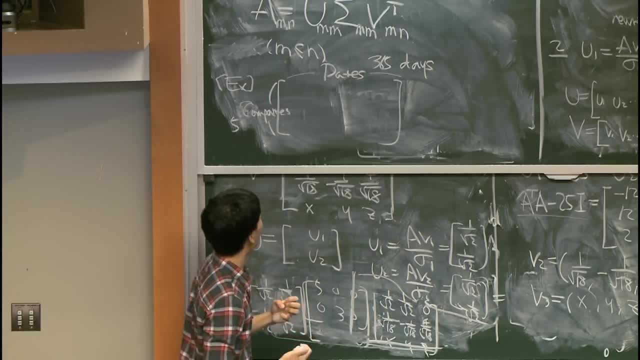 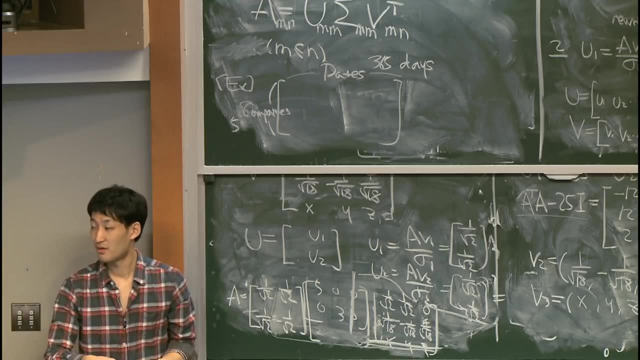 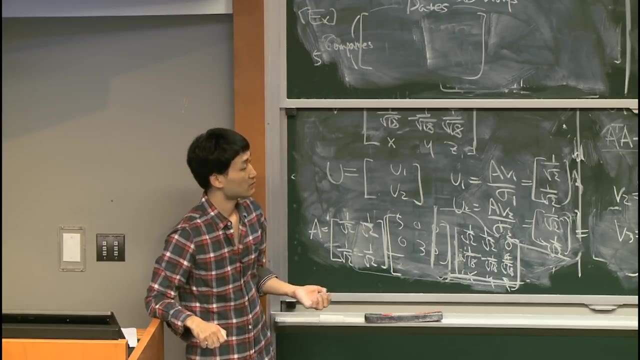 It measures their correlation. It measures the correlation with each other, So I don't have a very good explanation of what its physical meaning is. Maybe you can give us a little bit more. Possibly We will get into this in later lectures, But in the singular value, decomposition. 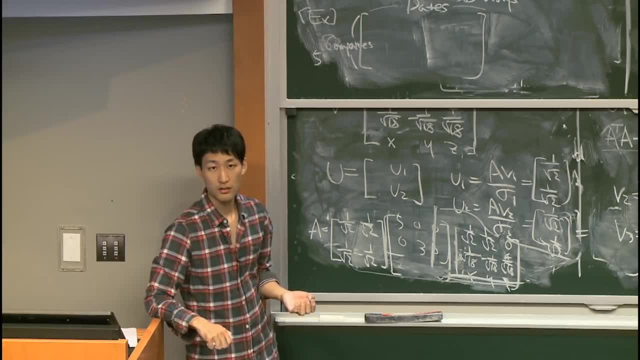 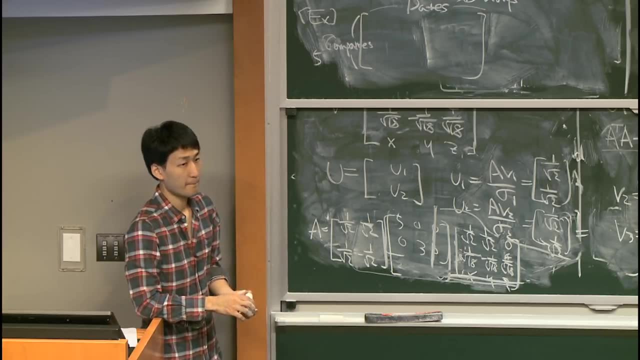 what you want to think of is, these orthonormal matrices are really defining a new basis, sort of an orthogonal basis. So you're taking the original, You're taking the whole coordinate system And then you're rotating it without changing or stretching or squeezing the data. 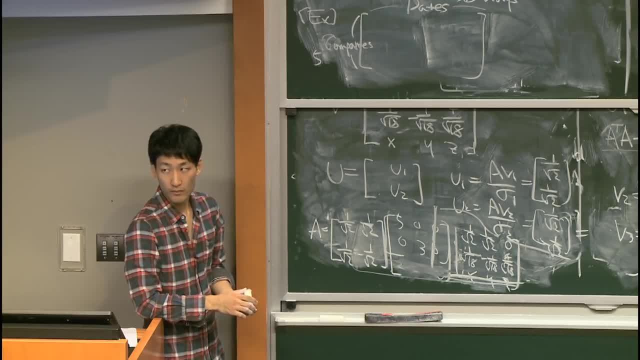 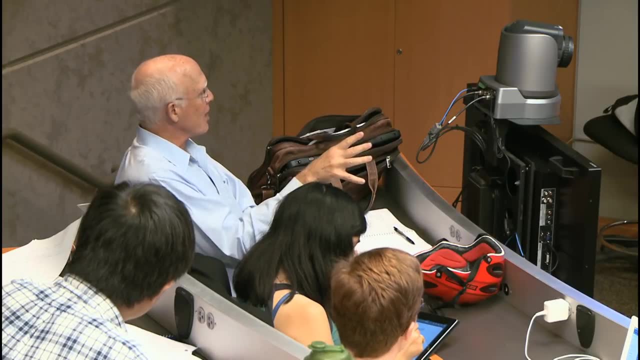 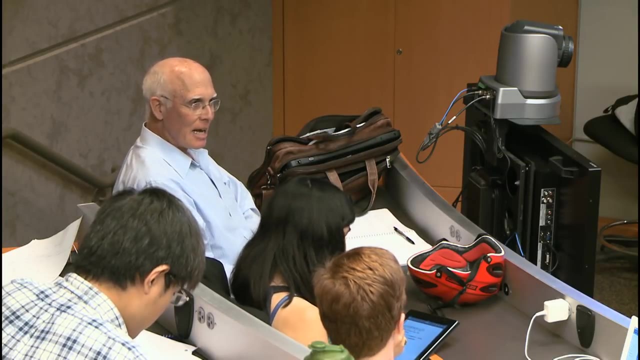 Or you're just rotating the axes, So an orthonormal matrix gives you the cosines of the new coordinate system with respect to the old one, And so the singular value decomposition, then, is simply sort of rotating the data into a different orientation. 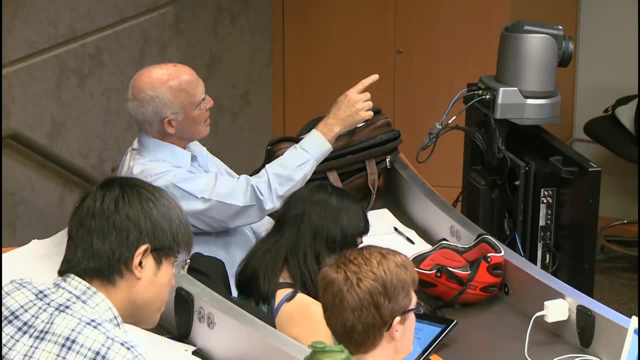 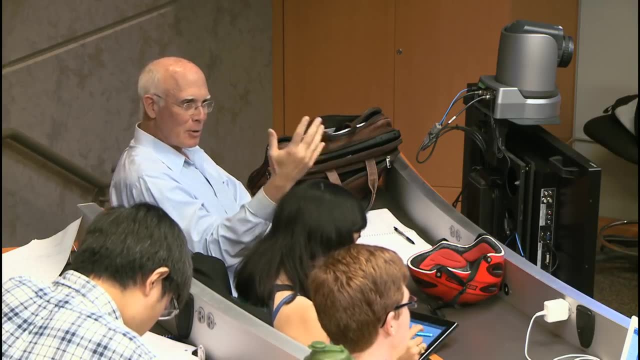 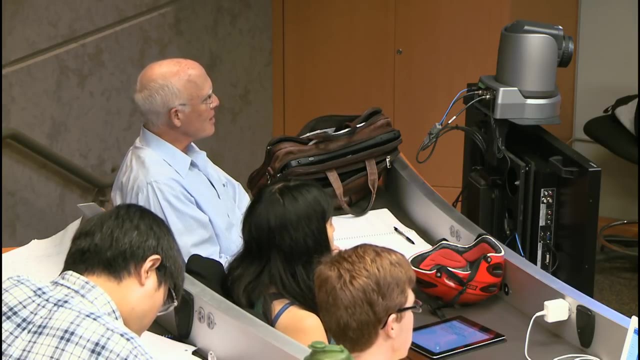 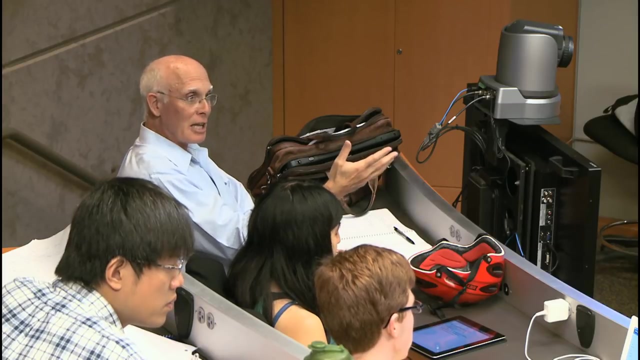 And the principle or the orthonormal matrix, orthonormal basis that you're transforming to is essentially the coordinates of the original data in the new, in the transformed system. So, as was commenting, you're essentially looking at a representation of the original data points in a linearly transformed space. 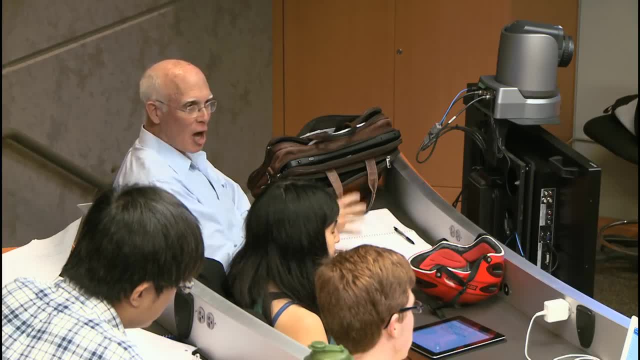 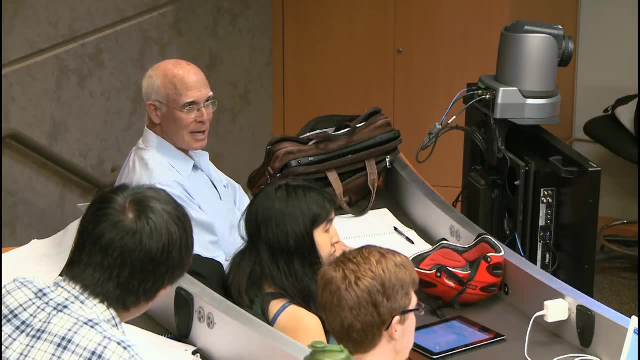 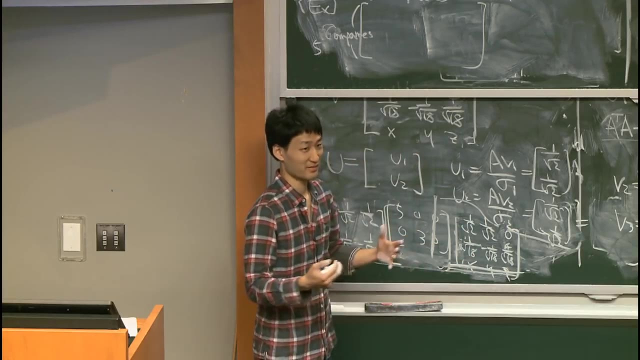 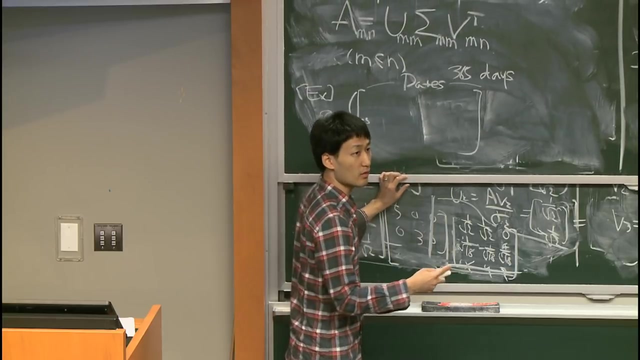 And the correlations between different stocks, say, is represented by how those points are oriented in the new. So you'll have to see real data to really make sense out of it. Yeah, But another way to think of it is where it comes from. 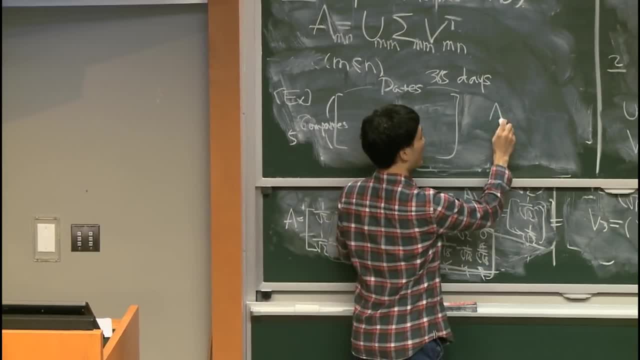 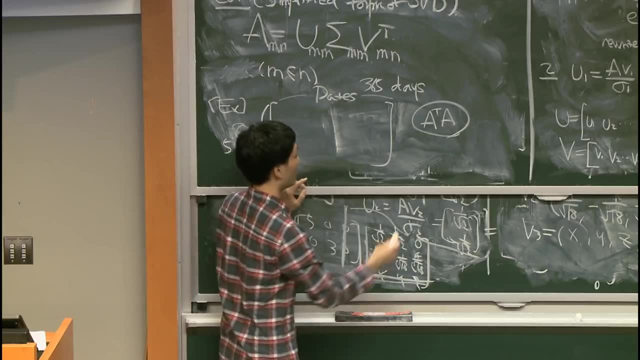 So all this singular value decomposition, if you remember the proof, it comes from eigenvectors and eigenvalues of A transpose A. Now if you look at A transpose A, I'll just say it's A transpose, A transpose, A times A transpose. 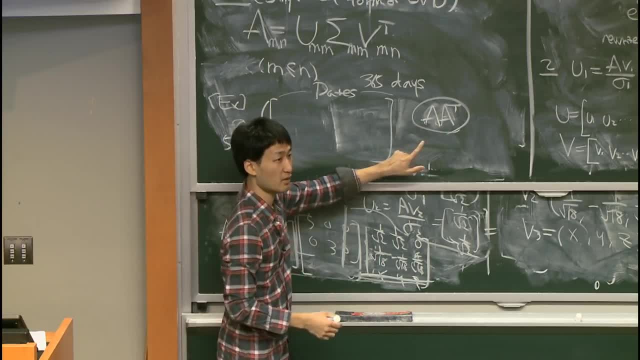 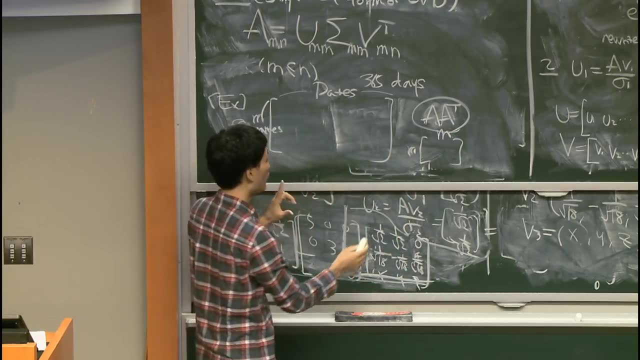 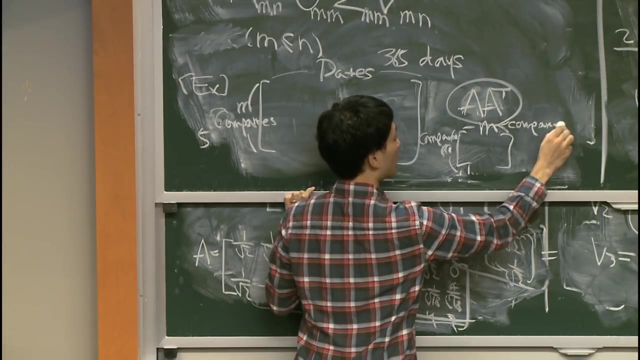 It's pretty much the same. If you look at A times A transpose, you're going to get an m by n matrix And it will be indexed both by these companies And the numbers here will represent how much the companies are related to each other. 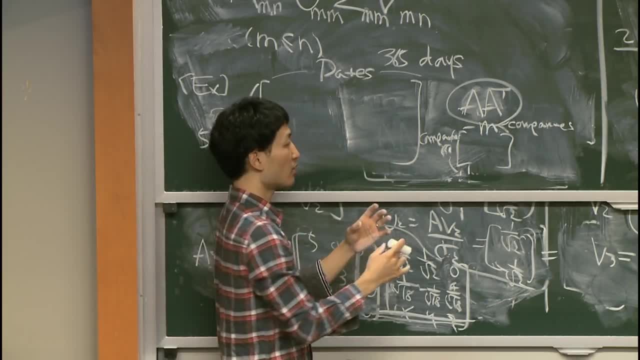 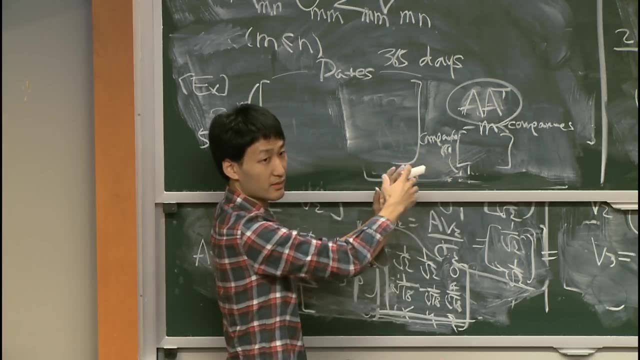 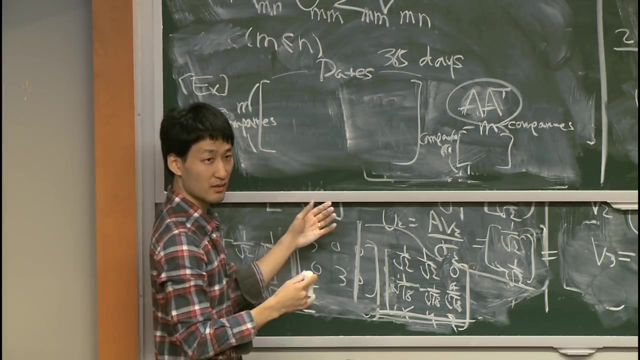 how much correlation they have between each other. So by looking at the eigenvectors of this matrix, you're looking at the correlation between these stock prices, let's say these companies' stock prices, And that information is represented inside the singular value decomposition. 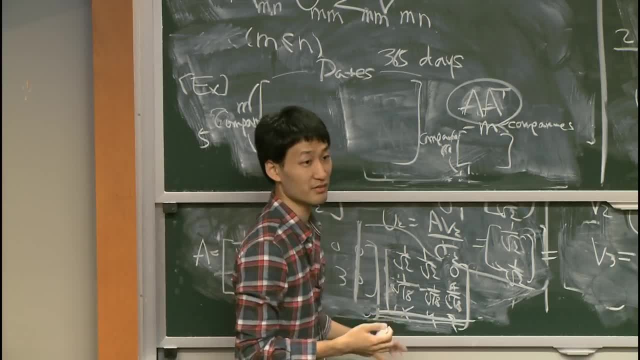 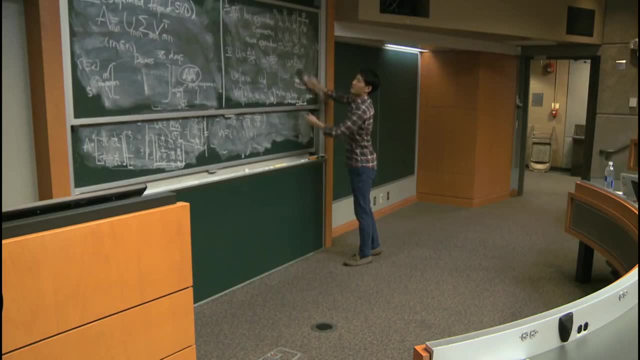 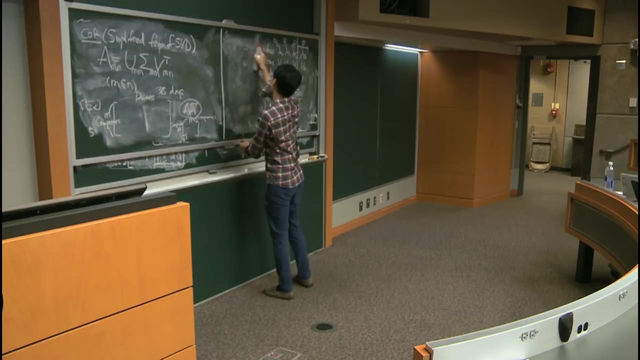 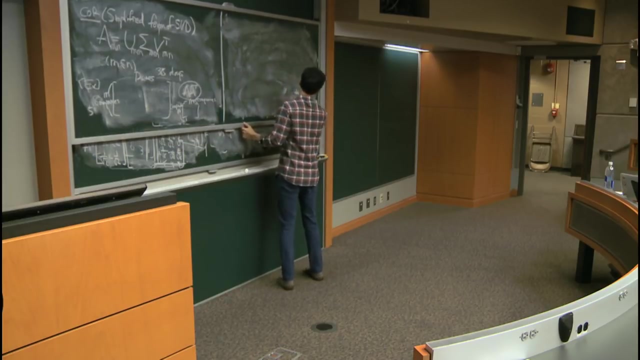 But again, it's a lot better to understand if you have real numbers and real data, which you will have later. So please be excited and wait. You're going to see some cool stuff. OK, so that was all for eigenvalue decomposition. 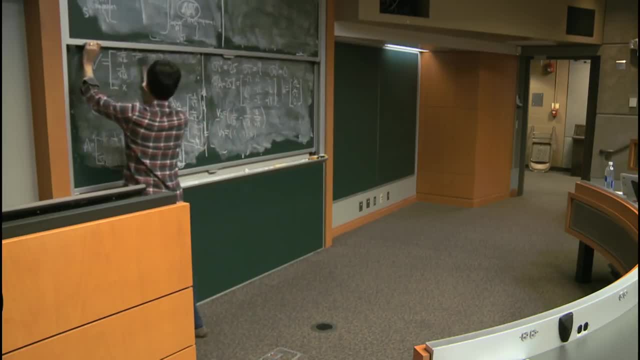 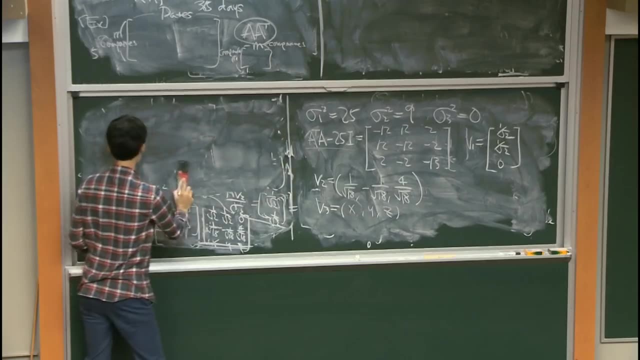 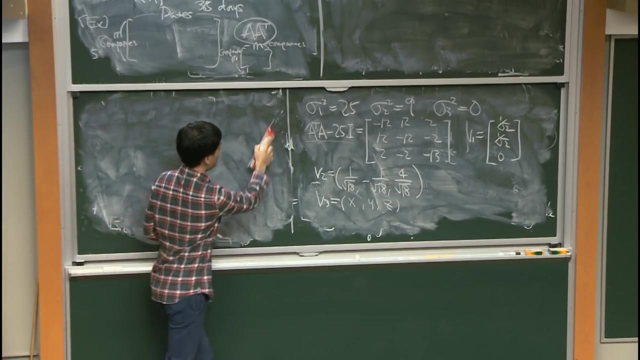 and singular value decomposition. And the last thing I want to mention today is something called Perron-Frobenius theorem. This one even looks a lot more theoretical than the ones I showed you, But surprisingly, a few years ago, Steve Ross, he's a faculty. 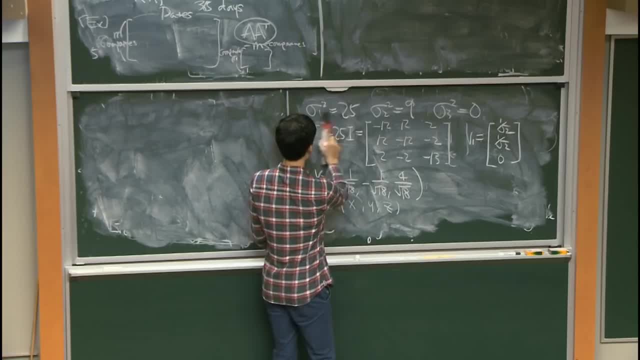 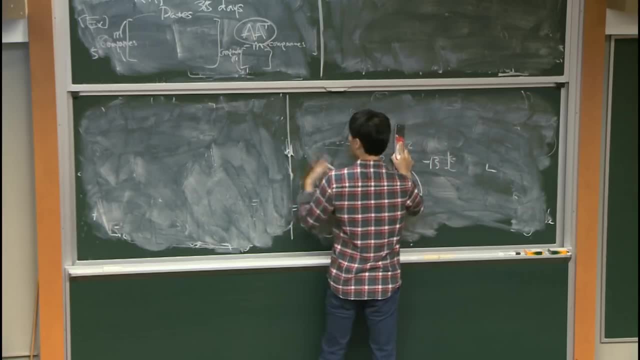 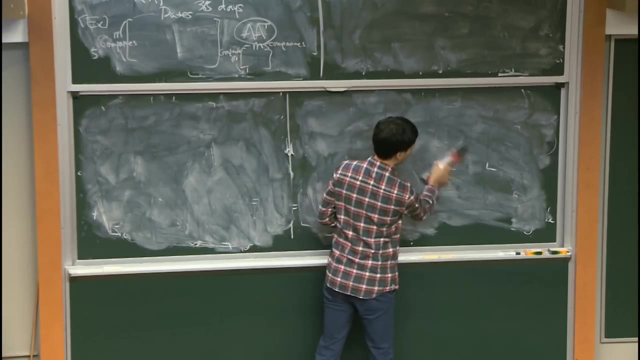 in the business school here found a very interesting result called Steve Ross Recovery Theorem that makes use of this theorem, so makes use of Perron-Frobenius theorem- that I will tell you today. Unfortunately, you will only see a lecture on Steve Ross. 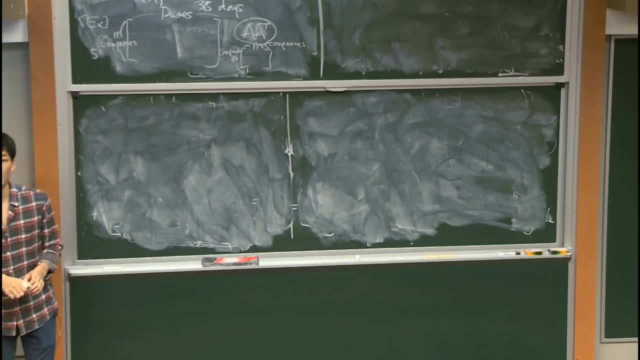 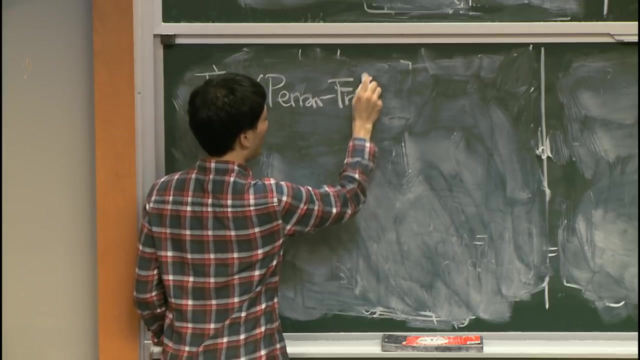 Recovery Theorem toward the end of the semester, So I will try to recall what it is later. But since we're talking about linear algebra today, let me introduce the theorem. This is called Perron-Frobenius And you really won't believe that it. 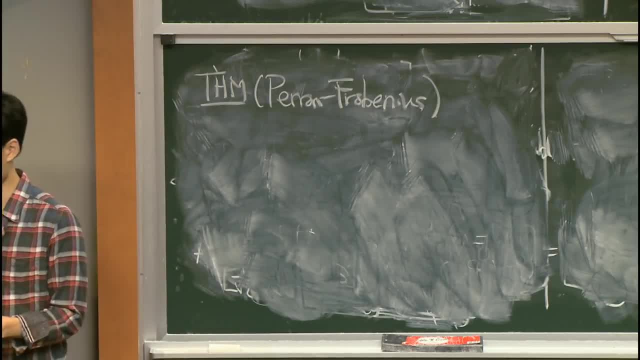 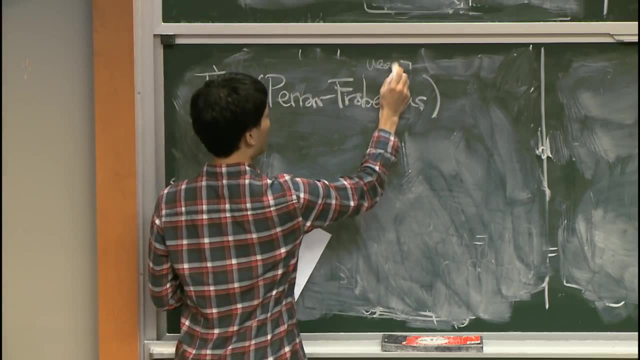 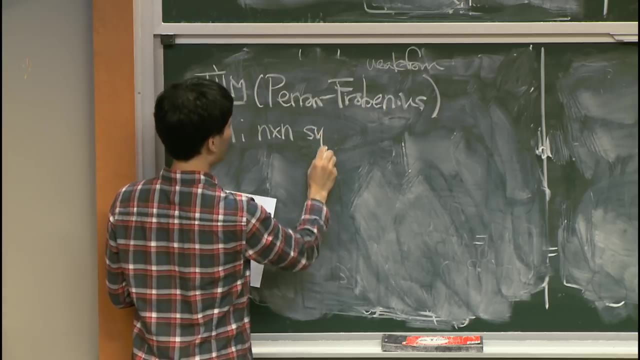 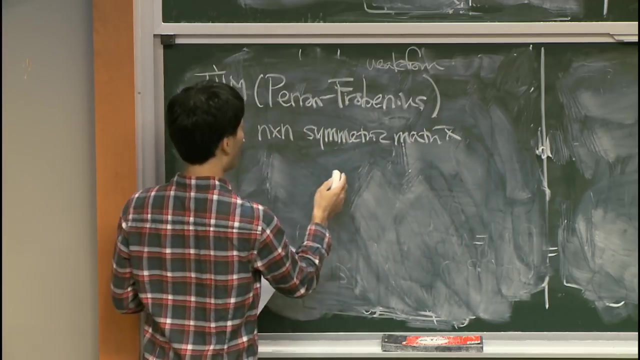 has any applications in finance because it just looks so theoretical. OK, I'm just stating a really weak form. Weak form. Let A be an n by n symmetric matrix. Let A be an n by n symmetric matrix whose entries are all positive, with positive entries. 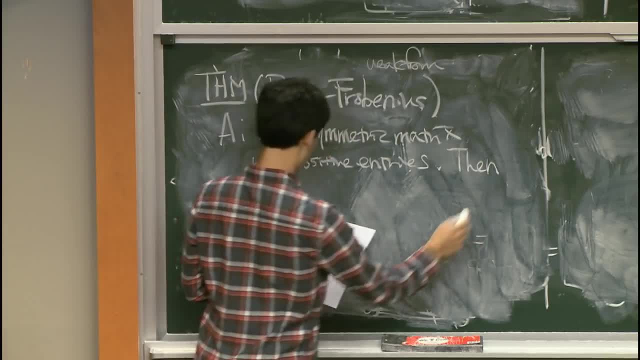 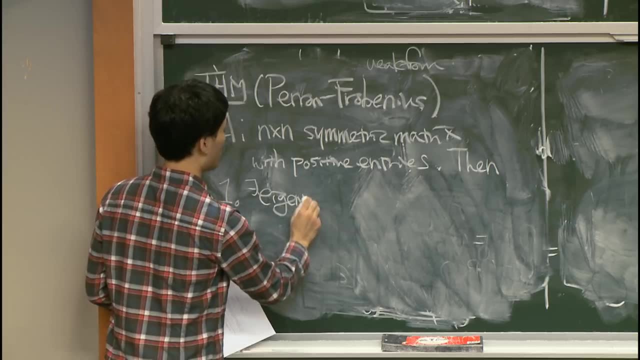 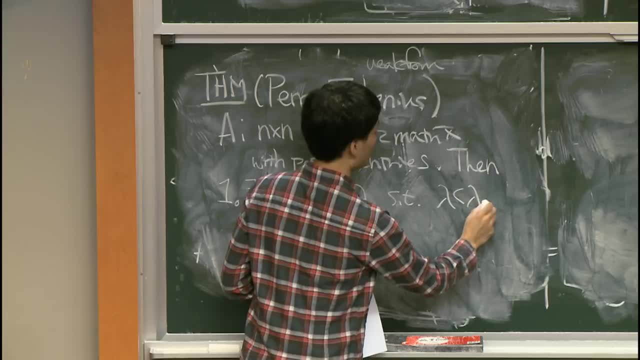 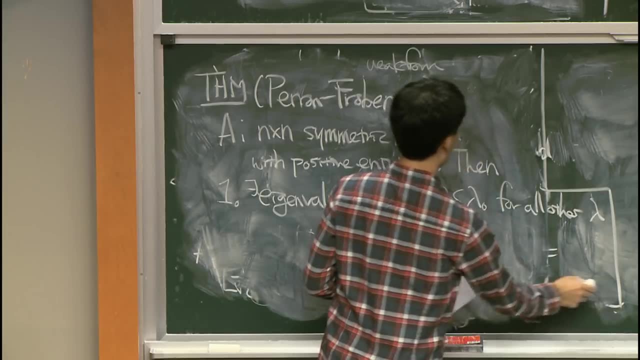 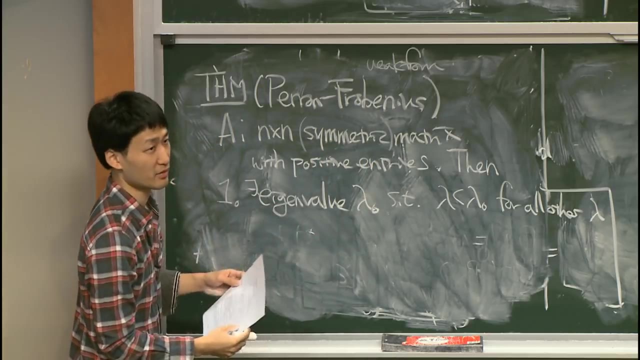 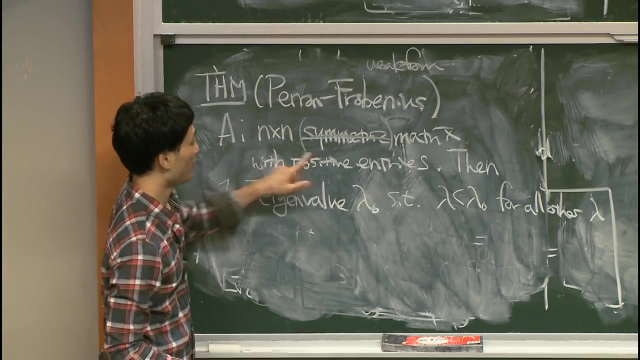 lambda 0.. lambda 0.. You can drop symmetric, but I'm just stating it because I'm going to prove only for this weak case. So think about the statement when it's not symmetric. So if you have an n by n matrix whose entries are all 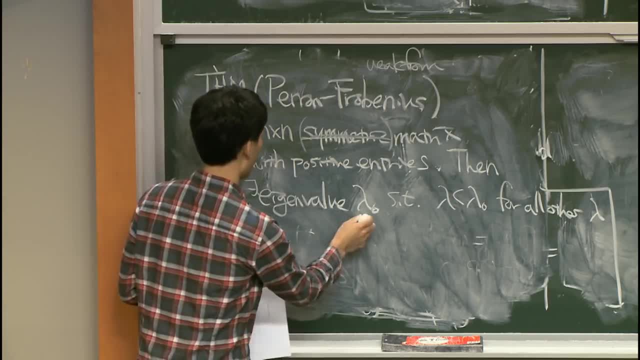 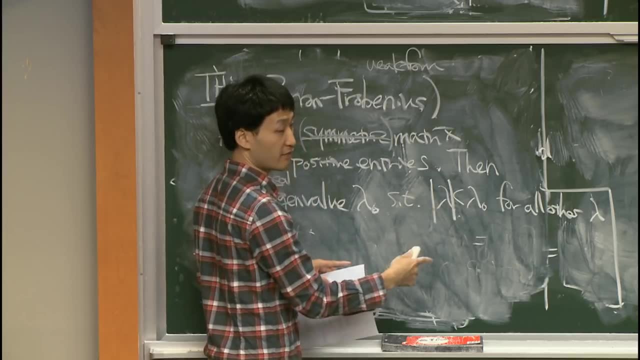 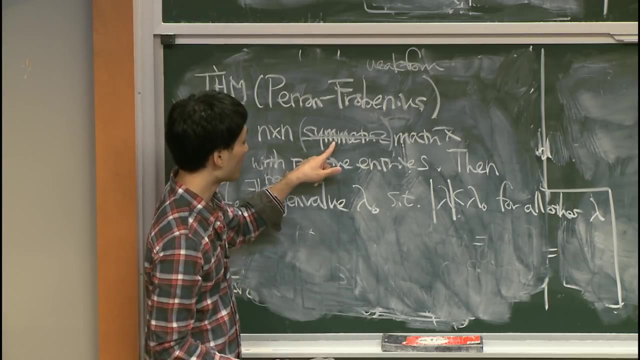 positive, then there exists an eigenvalue lambda- 0, a real eigenvalue, such that the absolute value of all other eigenvalues are strictly smaller than this eigenvalue. So remember that if it's not a symmetric matrix, they can be complex values. 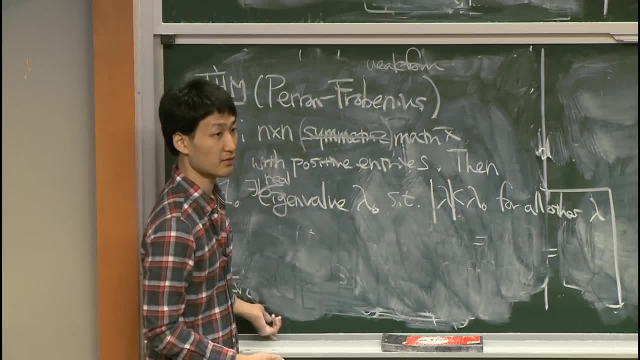 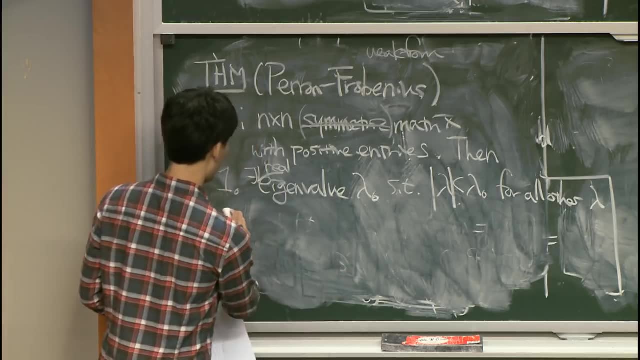 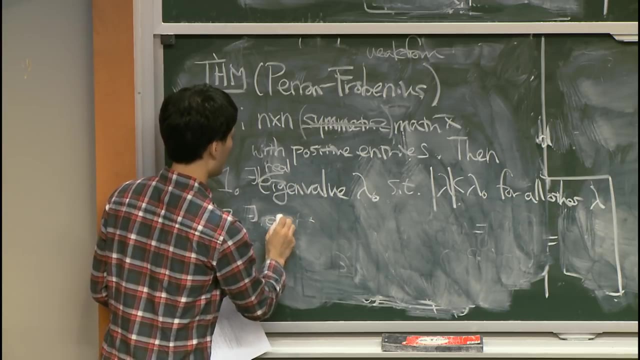 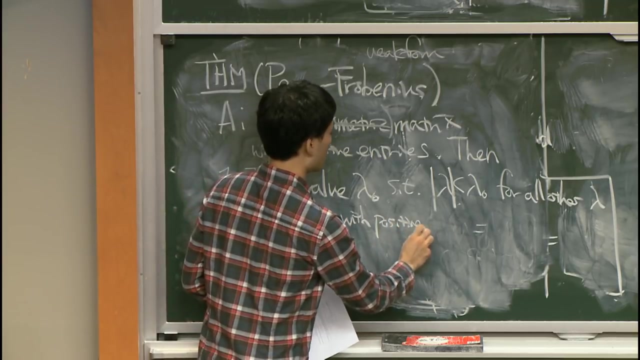 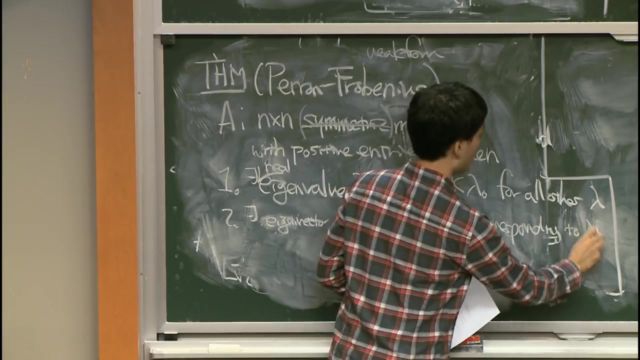 This is saying that there's a unique eigenvalue which has largest absolute value And, moreover, it's a real number. The second part: there exists a positive eigenvector with positive entries corresponding to lambda 0.. So the eigenvector corresponding to this, lambda 0. 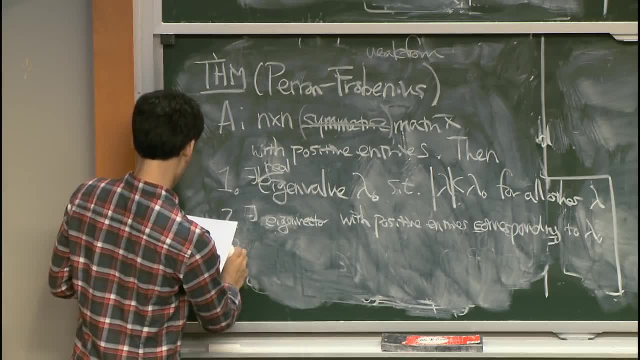 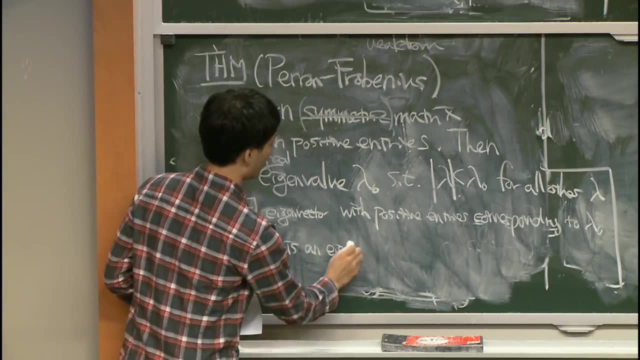 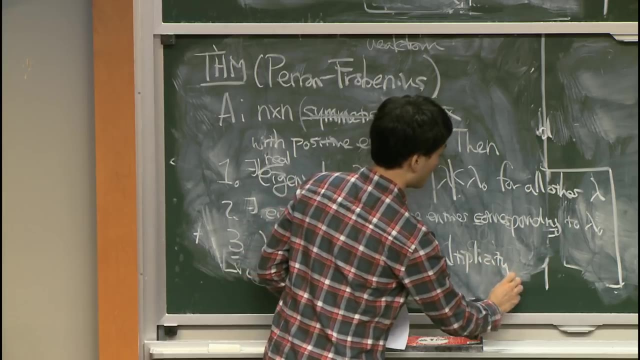 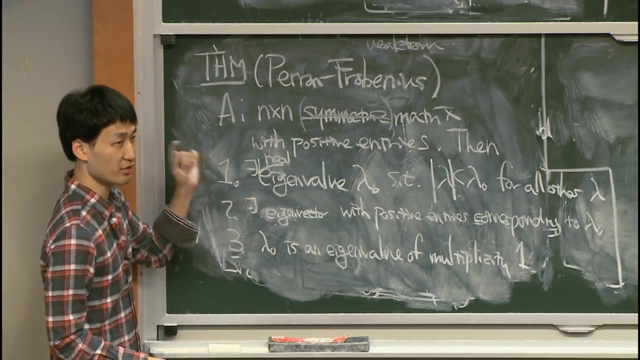 has positive entries, And the third part is lambda: 0 is an eigenvalue of multiplicity 1 for those who know what it is. So this really is a unique eigenvalue with a unique eigenvector, which has positive entries, And it's larger, really larger- than others. 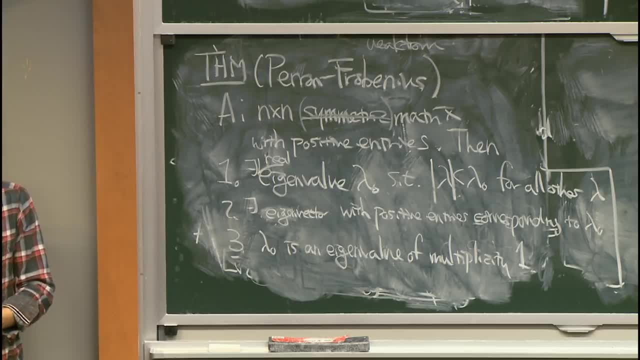 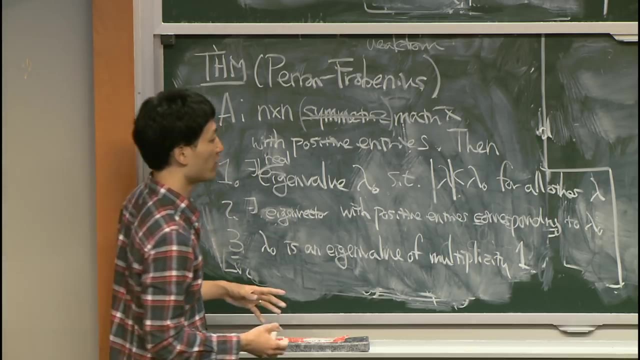 So that's our eigenvalue values. So from the mathematician point of view this has many applications. as probability theory. My main research area is combinatorics, discrete mathematics. It's also used in there. So from the theoretical point of view, 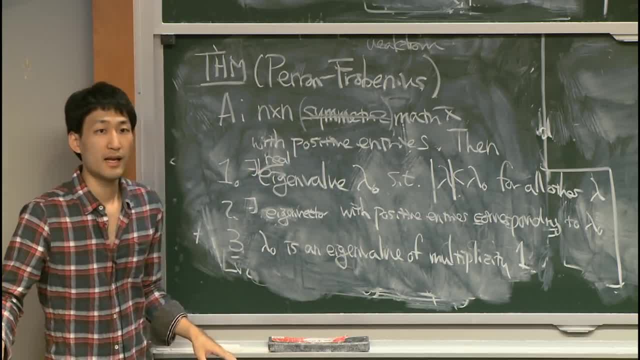 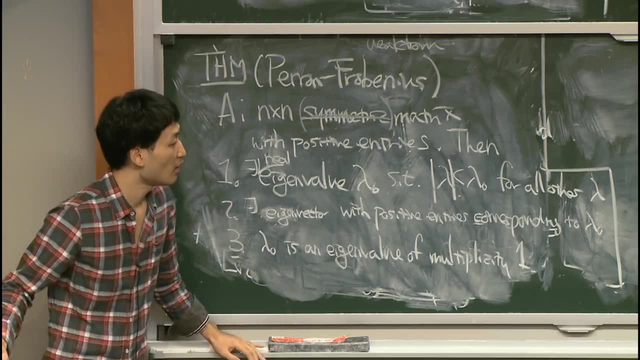 this has been used in many contexts. It's not a standard theorem taught in linear algebra, So I don't think probably most of you haven't seen it before, But it's used in many contexts. So, from the theoretical point of view, this has been used in many contexts. 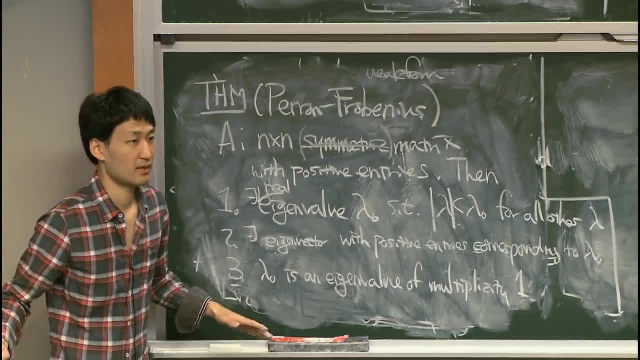 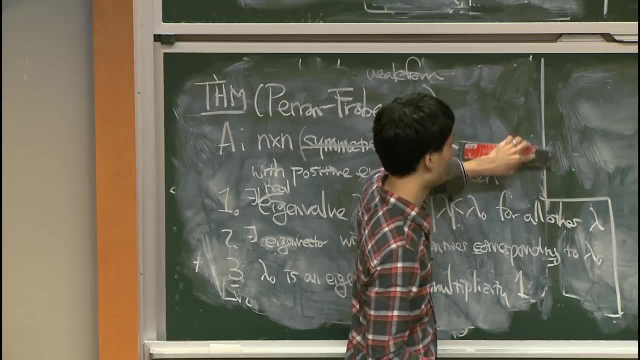 It's not a standard theorem taught in linear algebra, So from the theoretical point of view, this has been used in many contexts. It's a well-known result with many uses- theoretical uses, But you'll also see one used later, as I mentioned, in finance, which is quite surprising. 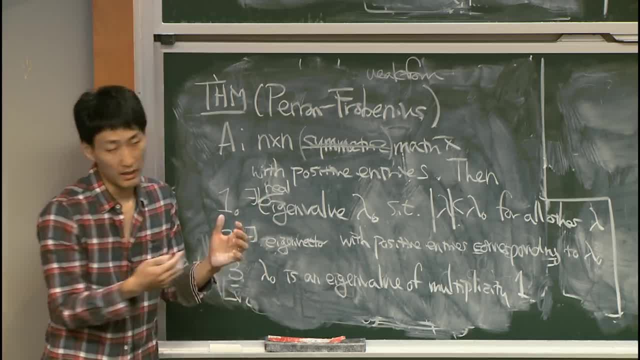 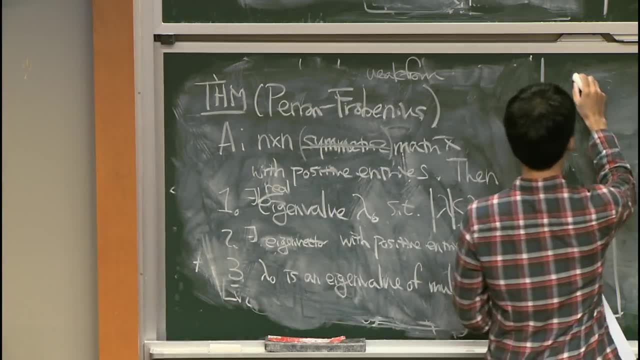 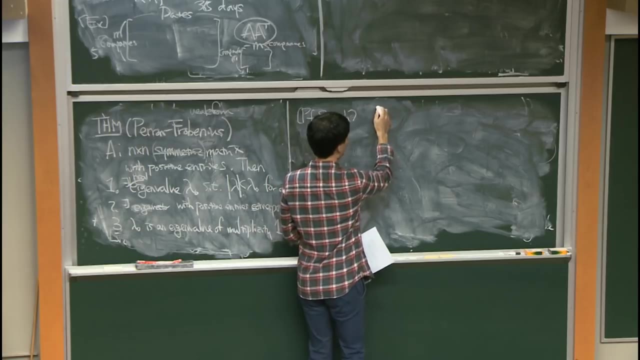 So let me just give you some feeling of why it happens. I won't give you the full detail of the proof, but just a very brief description. So it's a simple case of sketch when A is symmetric. So a simple case: A is symmetric. 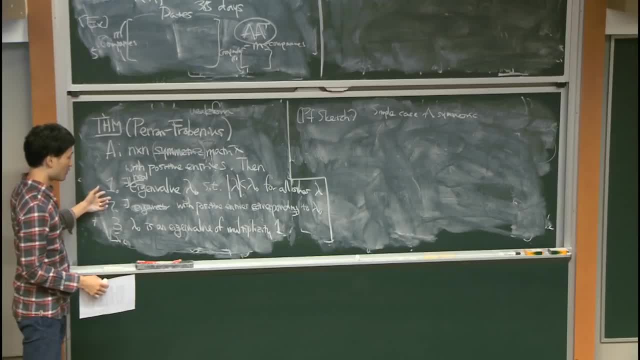 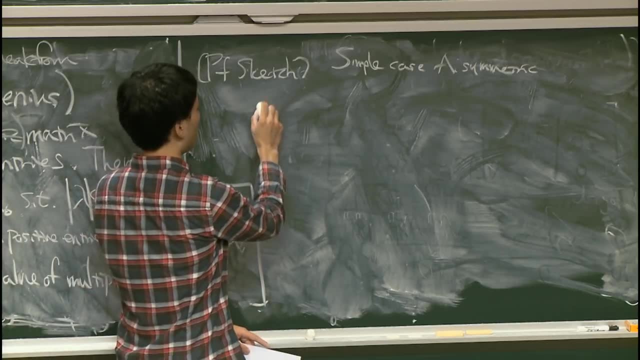 In this case, this statement: if you look at it first of all, A has to be equal to 0. So, if you look at it first of all, A has to be equal to 0. So it has real eigenvalues. 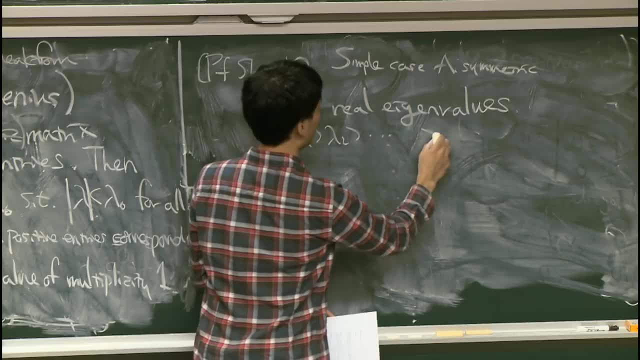 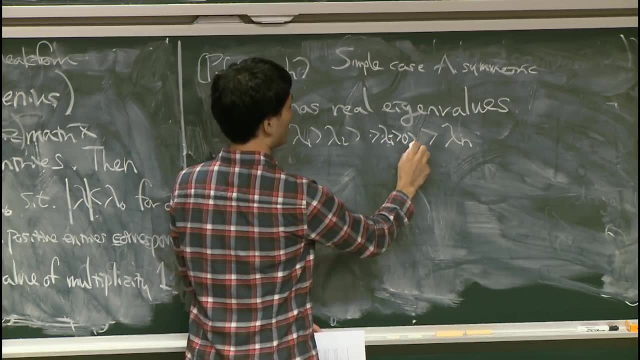 I'll say it's lambda 1, lambda 2, up to lambda n And at some point I'll say up to lambda i, it's greater than 0.. Afterwards, it's smaller than 0.. There are some positive eigenvalues. 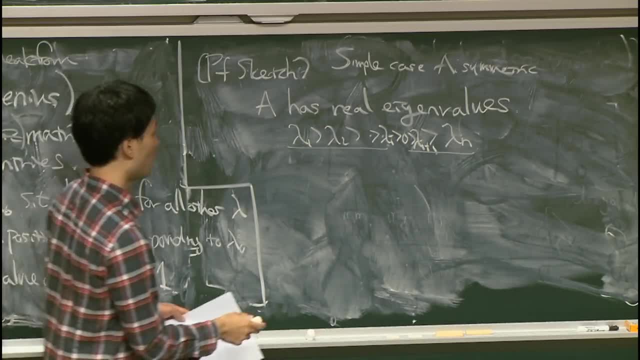 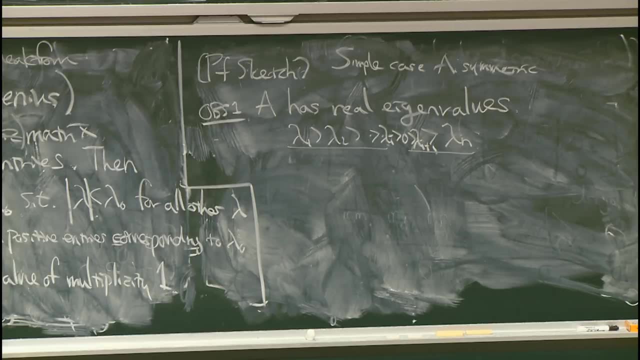 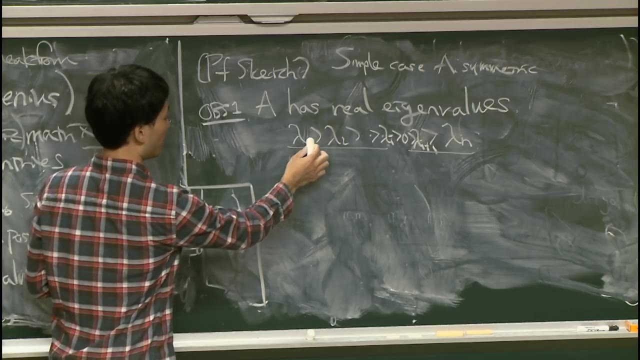 There are some negative eigenvalues. So that's observation one. Things are more easy to control because they're all real. The first statement says that Maybe I should have indexed it as lambda 0.. I'll just call this lambda 0 instead. 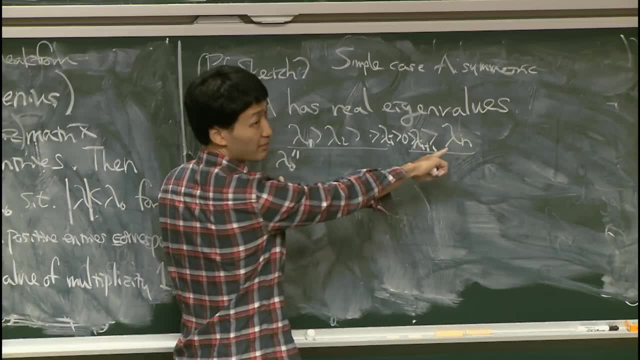 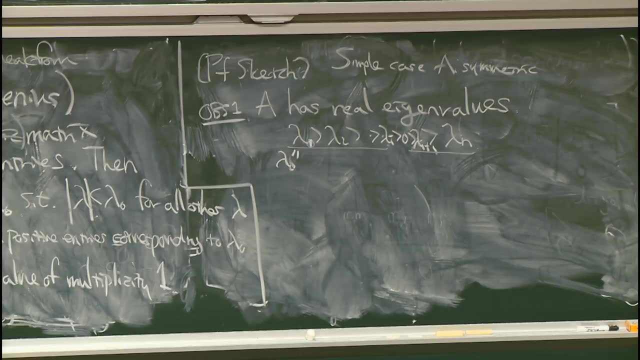 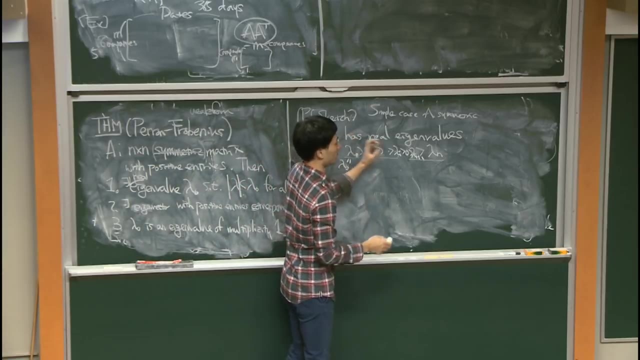 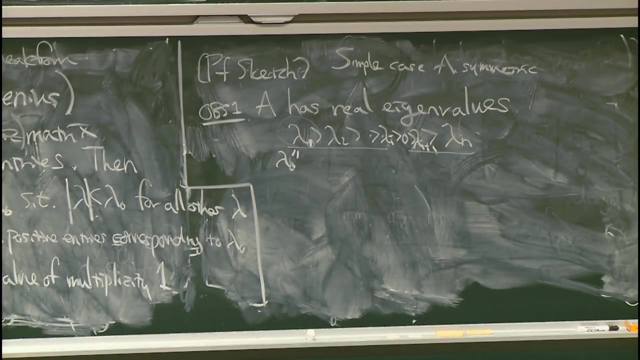 This lambda 0 is in fact larger in absolute value than lambda n. That's the content of the first bullet. So if they all have all positive eigenvalues, all positive entries, then the largest positive eigenvalue dominates the smallest negative eigenvalue, which yeah. 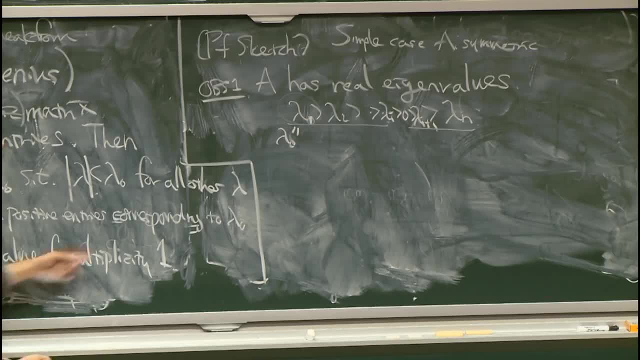 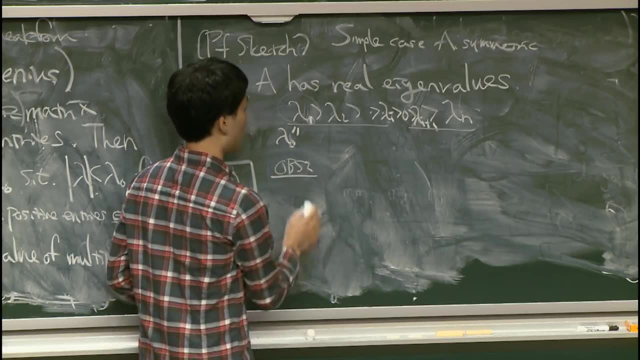 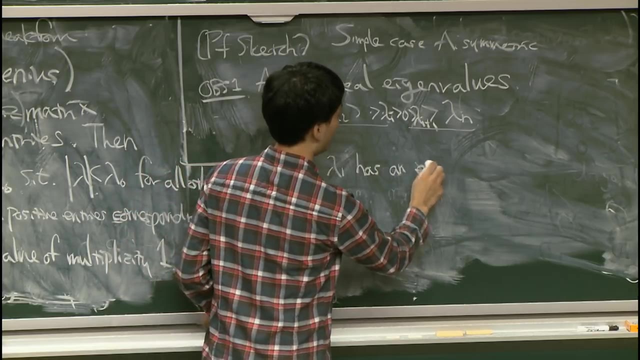 So why is that the case? First of all, to see that you have to go through different steps. So we go into observation two: Lambda 1.. So look at lambda 1. Lambda 1. Lambda 1 has an eigenvector with positive entries. 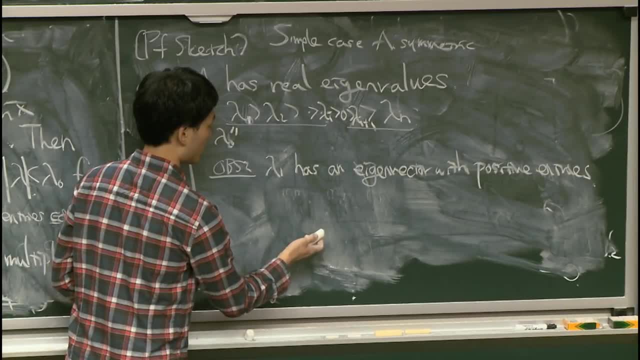 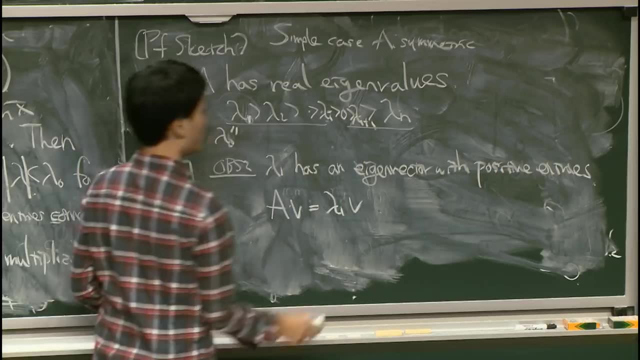 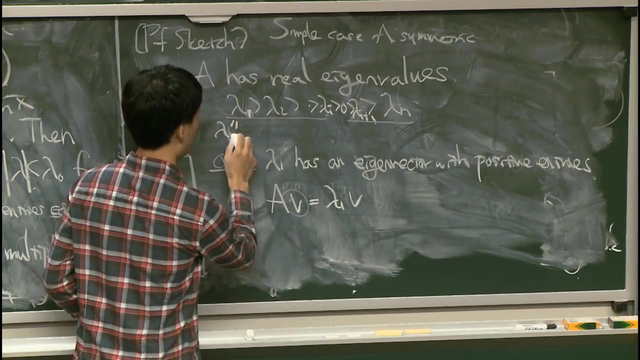 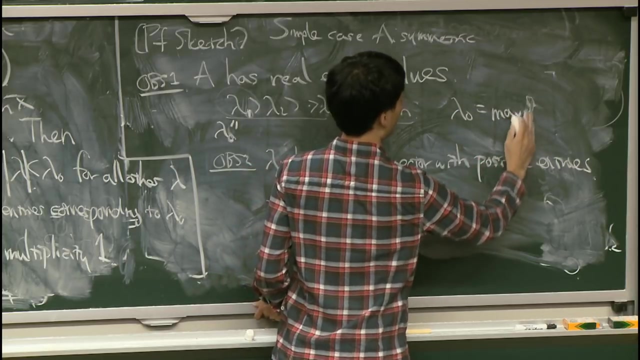 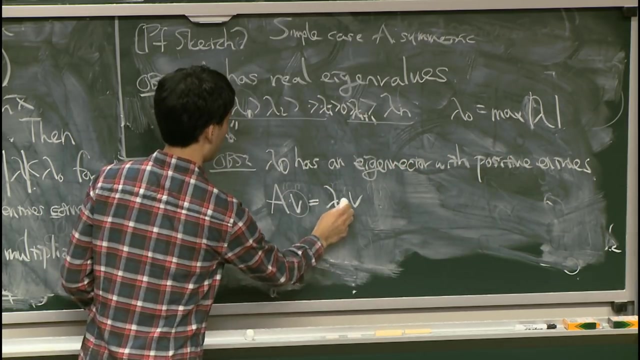 Why is that the case? That's because, if you look at, a times b equals lambda 1 times b. If v, let me state it this way- Lambda 0 is the maximum of all lambda Lambda 0.. OK, that's not entirely correct. 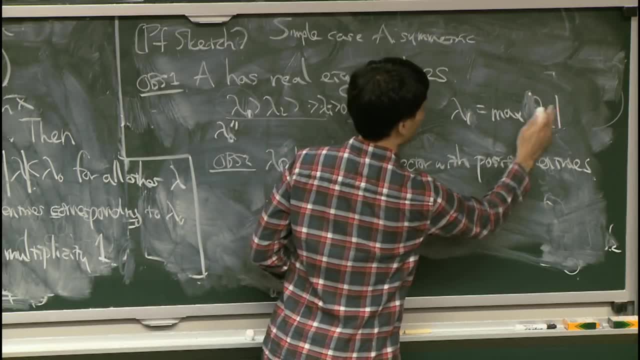 Lambda: 1. Lambda, 2. Lambda, 3. Lambda, 4. Lambda, 5. Lambda, 6. Lambda, 7. Lambda, 8. Lambda, 9. Lambda, 10. Lambda, 11. Lambda, 12. Lambda 13.. 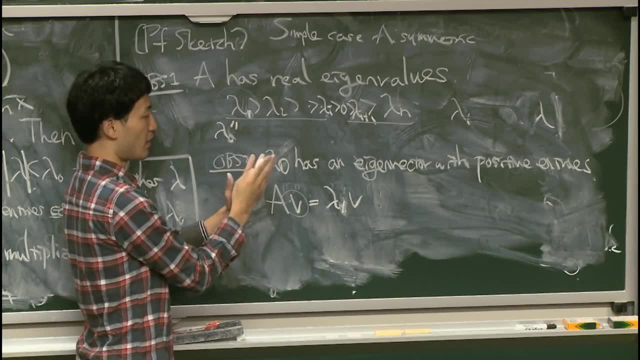 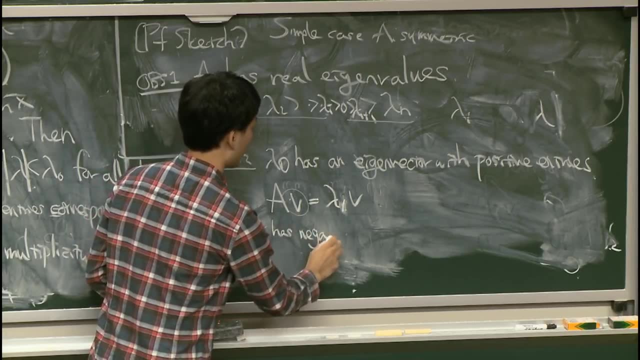 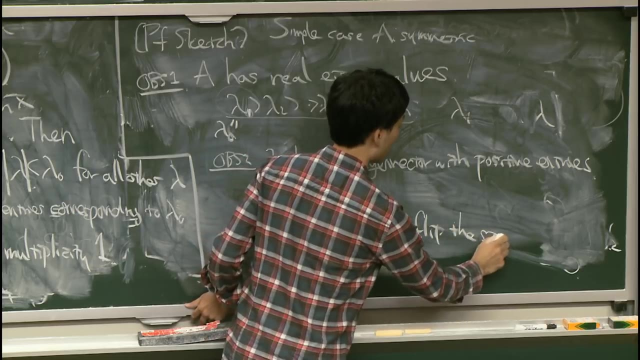 Lambda 14.. So, if you look at this, if v has non-positive entries, if it has a negative entry, if v has a negative entry, then flip it, flip the sign and in this way obtain new vector v prime. 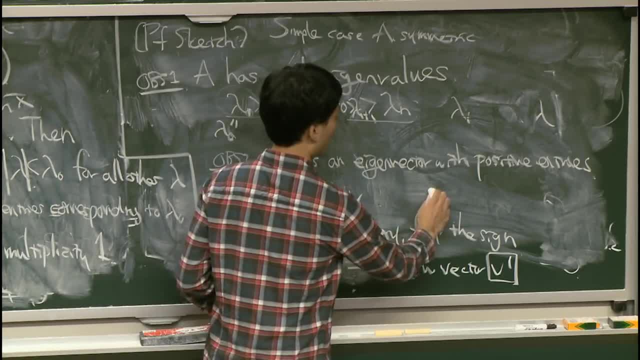 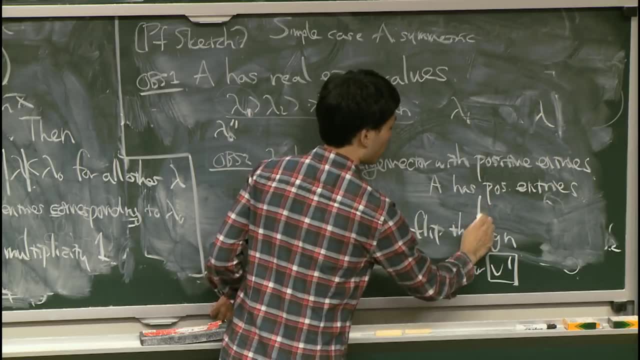 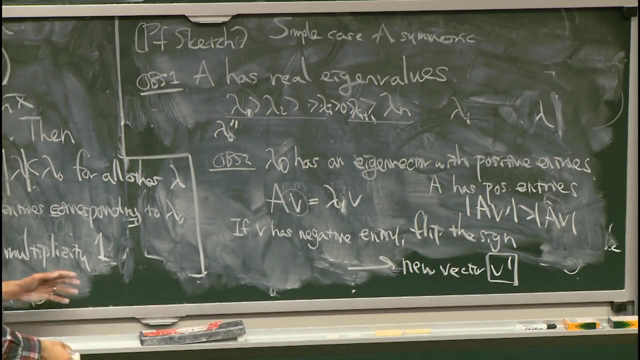 Since a has positive entries, a has positive entries, what we conclude is that a times v prime will be larger than a times v. You have to look, Think about it, because it has positive entries. If it has some negative part somewhere, the magnitude will decrease. 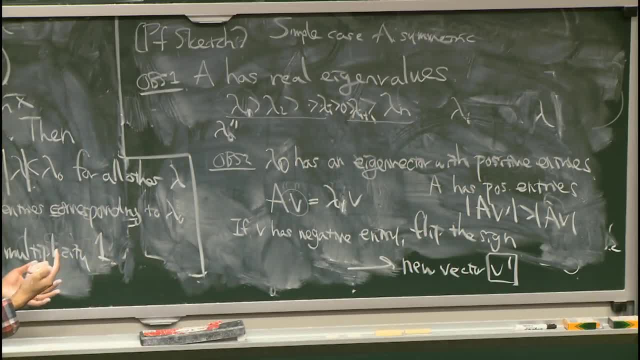 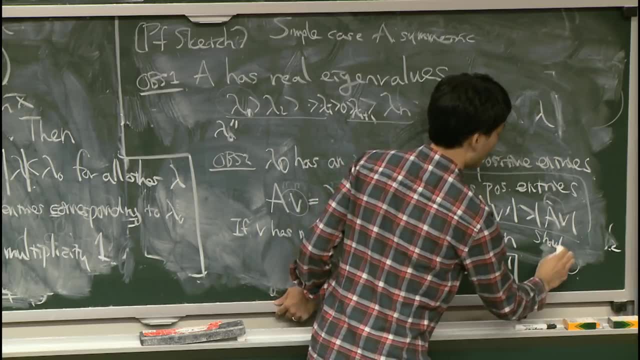 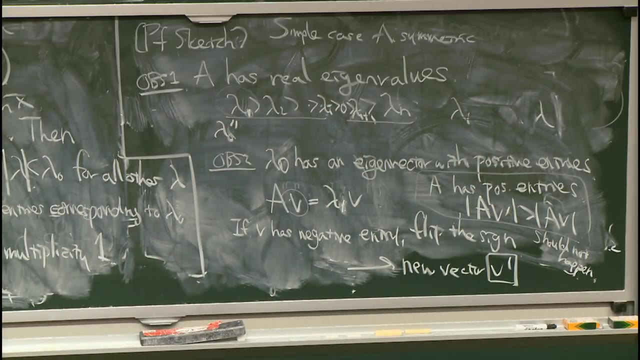 So if you flip the sign, it should increase the magnitude, And this cannot happen. This shouldn't happen. It should not happen. That's where the positive entries part is used. If you have positive entries, then the eigenvector should have positive entries as well. 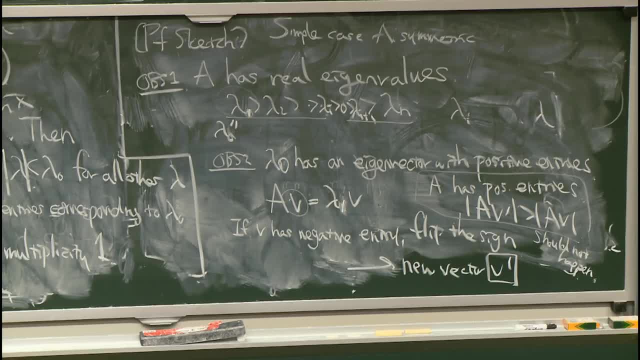 So I will not work through the details of the rest. I will post it on the lecture notes. But really, this theorem, in fact, can be stated in a lot more generality than this. I'm stating only a very weak form. 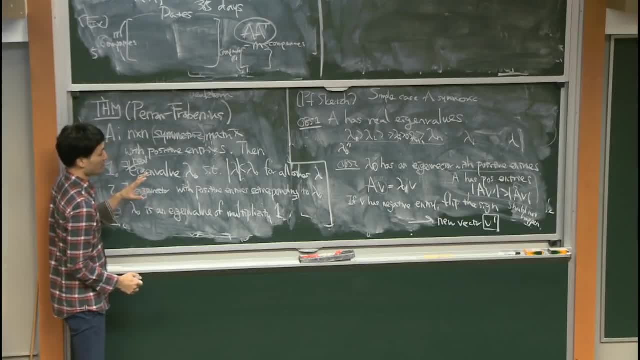 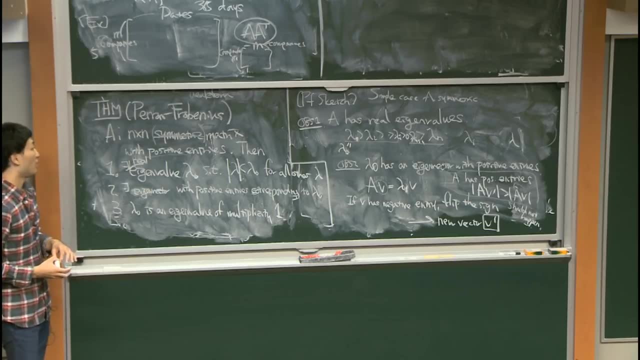 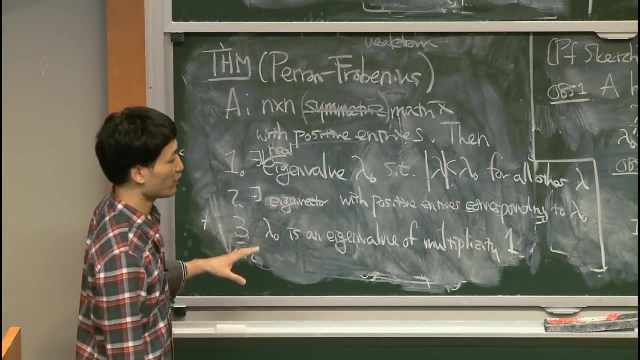 It doesn't have to have all positive entries, It has to only be something called irreducible, which is a concept from probability theory, from Markov chains. But here we will only use it in this setting, So I will review it later before it's really being used. 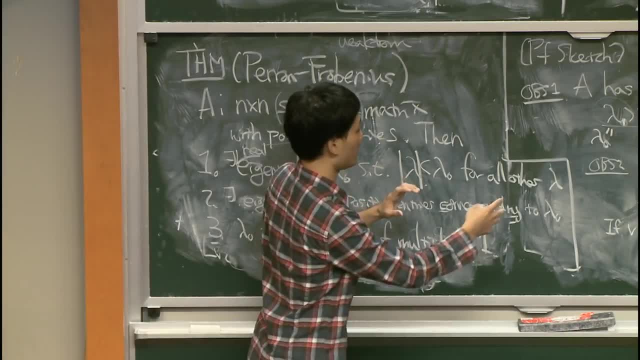 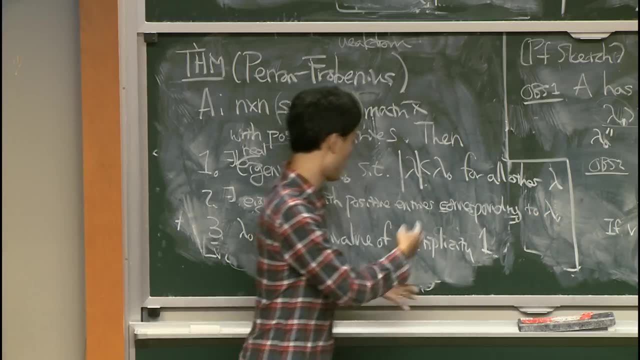 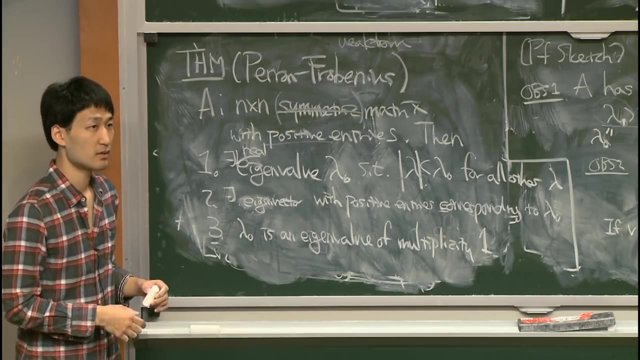 But just remember that, how these positive entries kick into this kind of statement where there is an eigenvalue, largest eigenvalue, why there has to be a vector which is all positive entries. Those will all come into play later. So I think that's it for today. 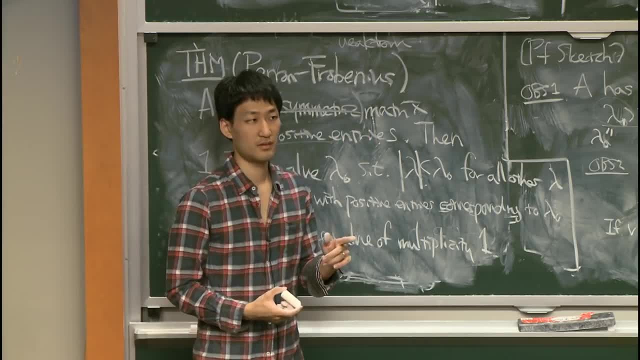 If you have any last-minute questions. if not, I will see you on Thursday. 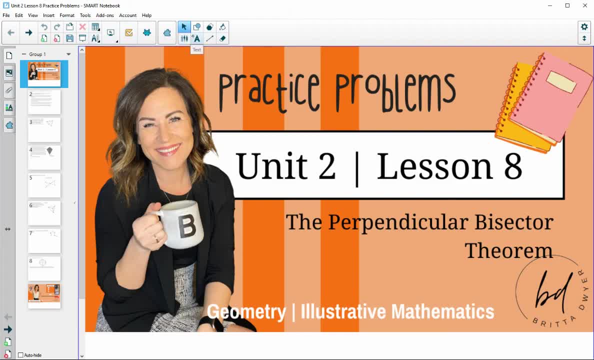 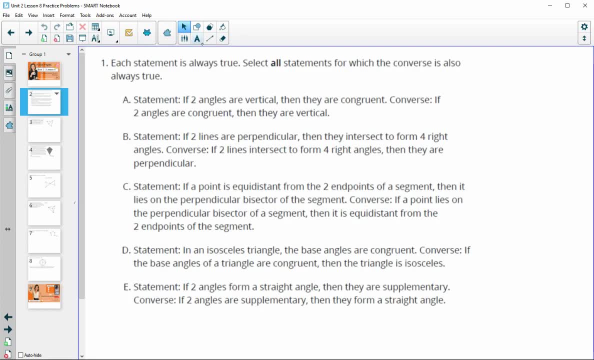 In this video we're going to look at the Unit 2, Lesson 8, practice problems. Number one says that each of the statements is always true. Determine whether the converse is true. So they're giving you a statement in each one. This is true. We're just reading the converse. 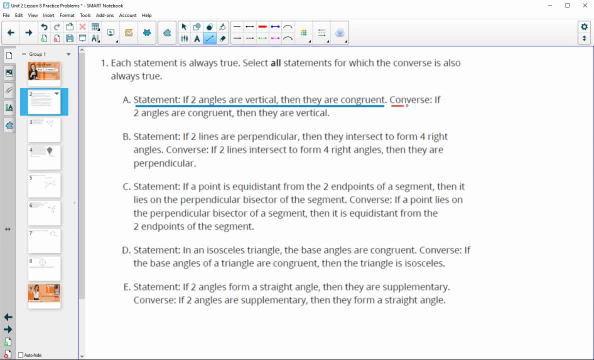 which is where we switch the end and the beginning and decide if the converse of the statement is also true. All right, so in this first one, the converse is: if two angles are congruent, then they're vertical. And that is not true, And we can provide a counterexample. 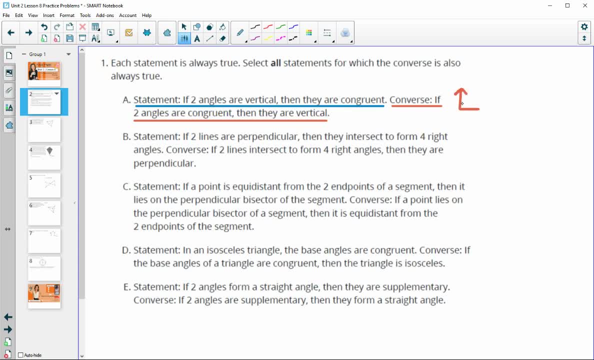 because vertical angles is where the two lines kind of cross each other. So here's a vertical angle like this, And vertical angles are always congruent. but congruent angles aren't always vertical, because we can draw congruent angles that aren't vertical angles. 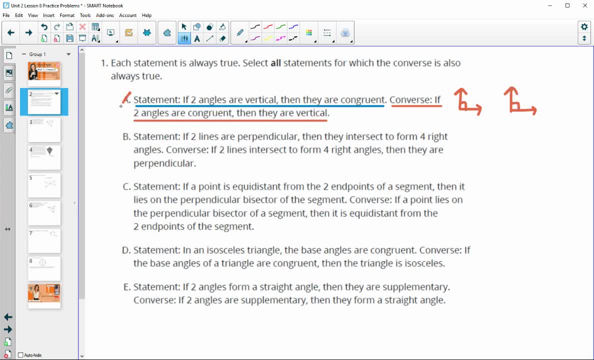 So these are two right angles, They're congruent, but they're not vertical. So this one would be false. The second one, the converse, says if two lines intersect to form right angles, then they are perpendicular. So if we have two lines crossing, 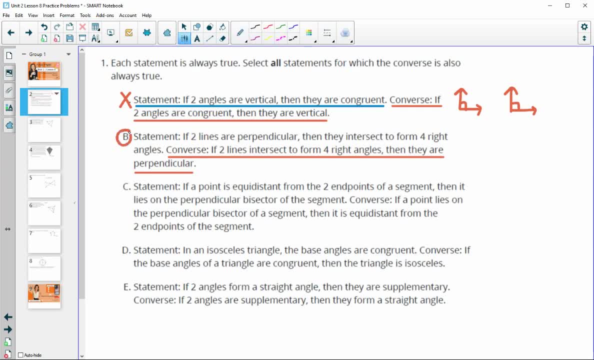 and they form right angles, then they're perpendicular. That is true. C. the converse says if a point lies on the perpendicular bisector of a statement, okay, so we have a perpendicular bisector of a segment, two points that are lying, or a point.